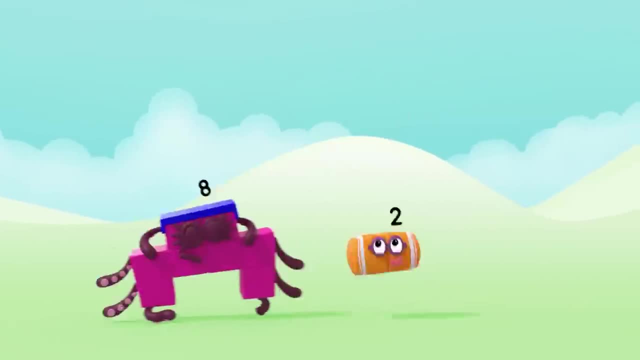 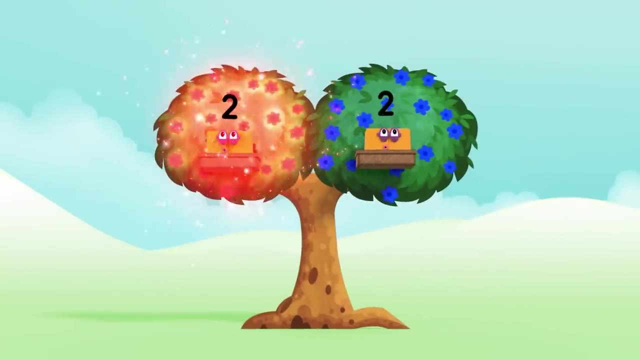 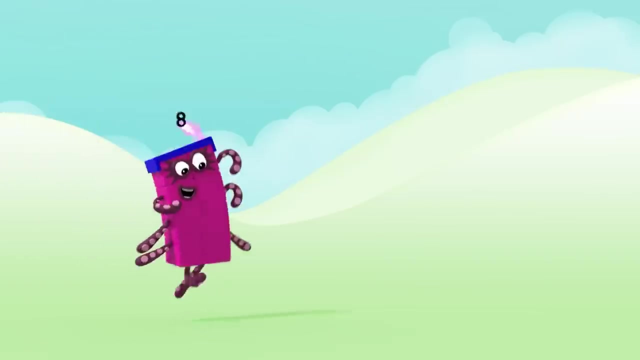 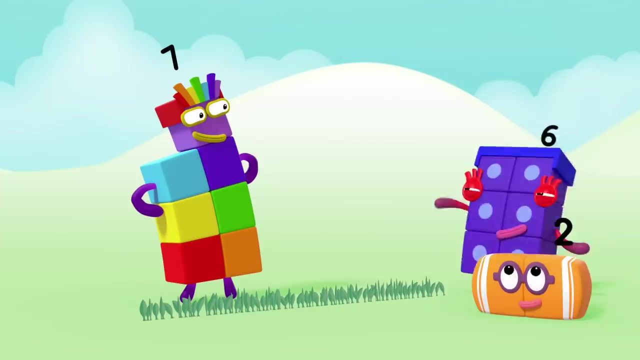 Er, Oh, Whee, Woo-hoo-hoo, Oi Whee. Two points each. Beginners luck, You're bigger, You start. Eight minus two Equals six. This game is nice. Let's roll the dice. 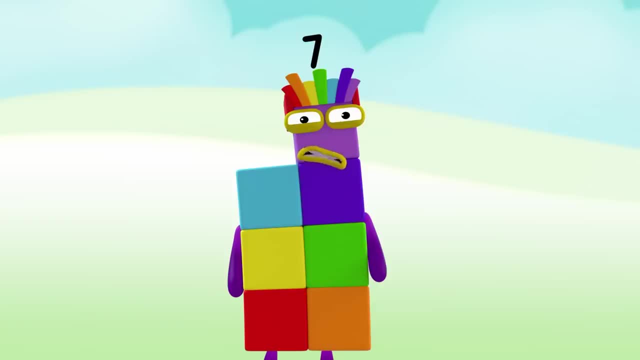 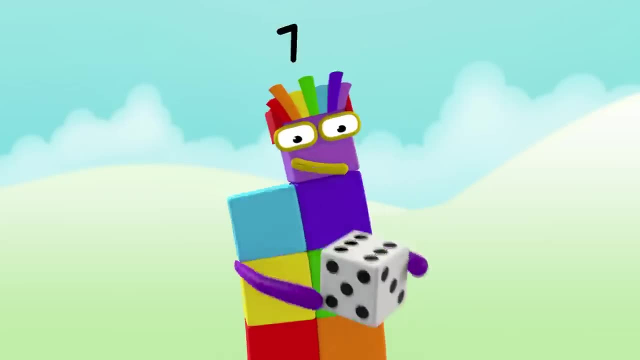 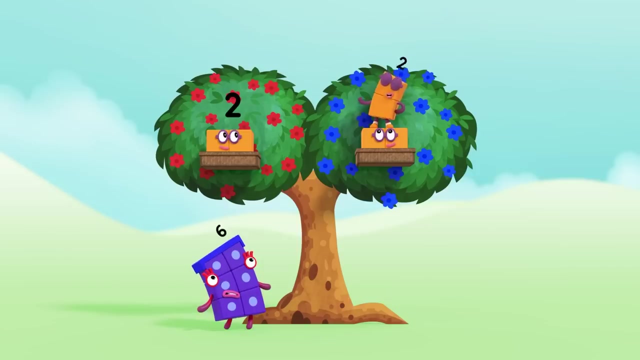 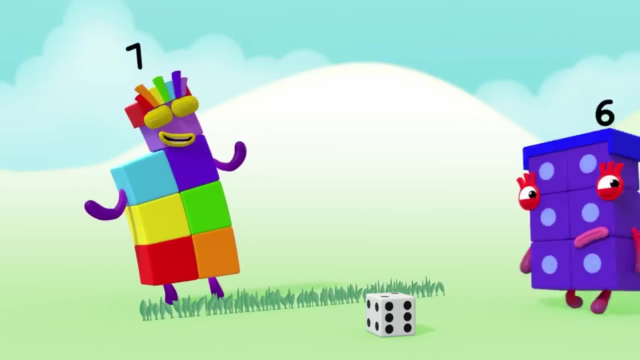 When it leaves my hand. how will it land? Um on six? Oh, lucky me, Lucky me. Penalty, unfair distraction, Which means Four, two. Better luck next time, Here we go. Seven minus two, Equals. 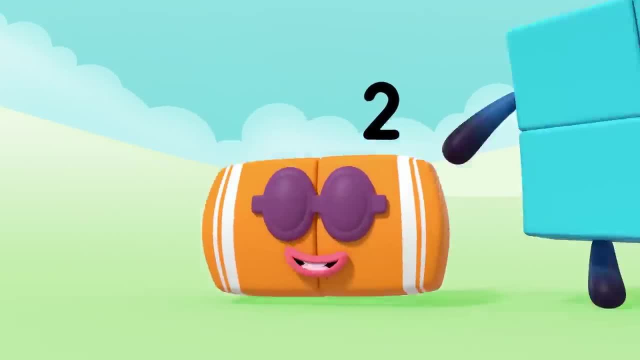 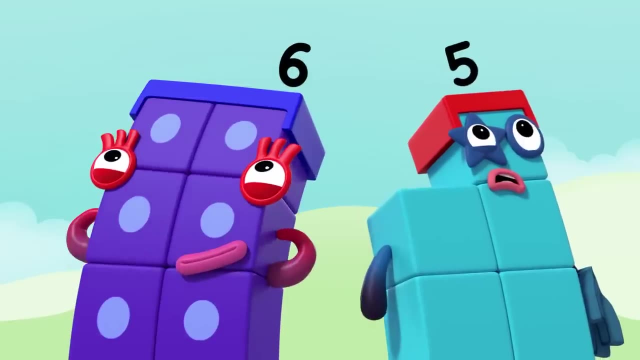 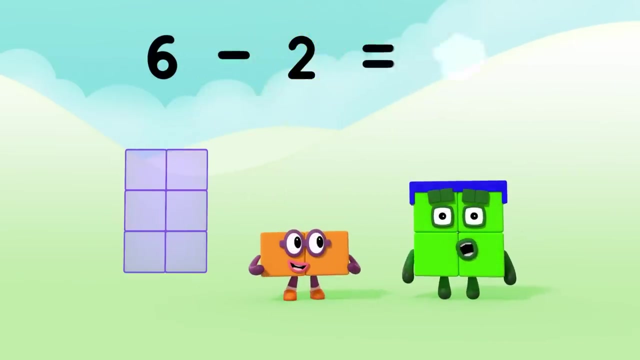 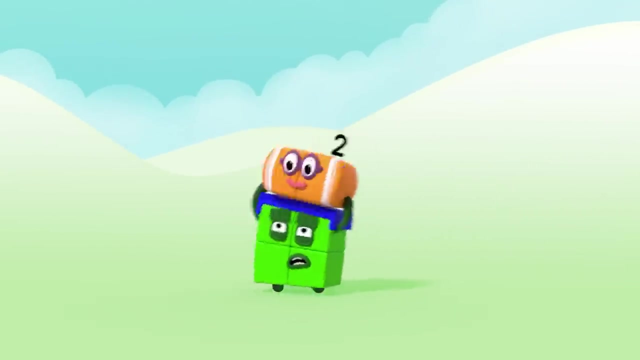 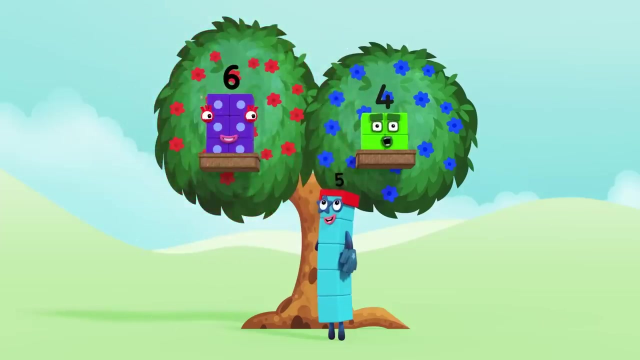 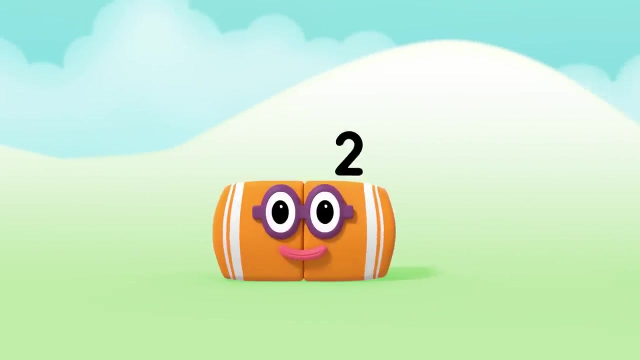 Five Four points each. Six Minus two Equals four. Four Three Whee Whee Whee Whee. Six four. Six Five minus two Equals three Whee Whee Whee. 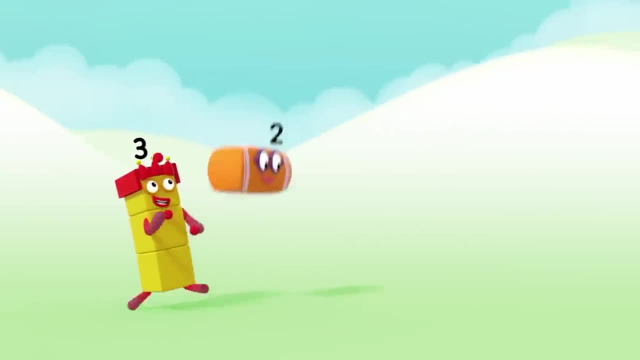 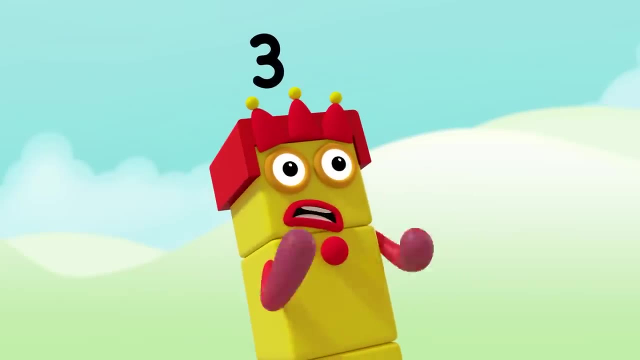 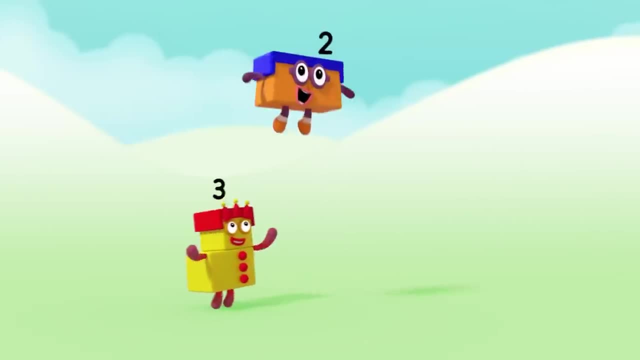 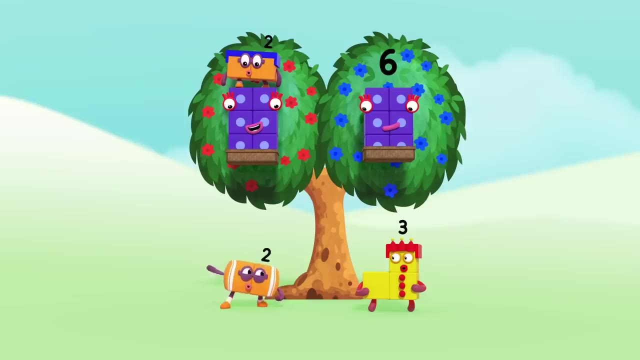 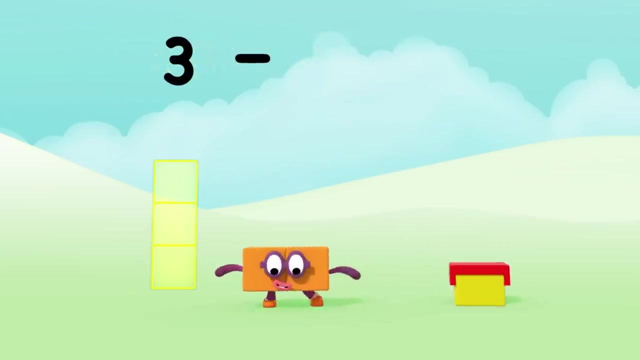 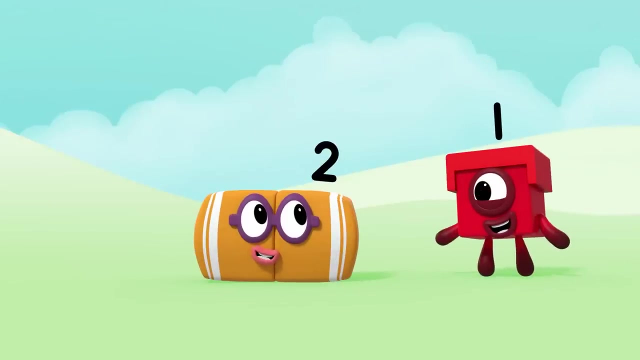 Whee Penalty round two, Oh Eight. Three Minus two Equals one Final round. Ready Go, Oh no, Oh no, Oh no, Oh Oh Bother. Let me lend a hand. 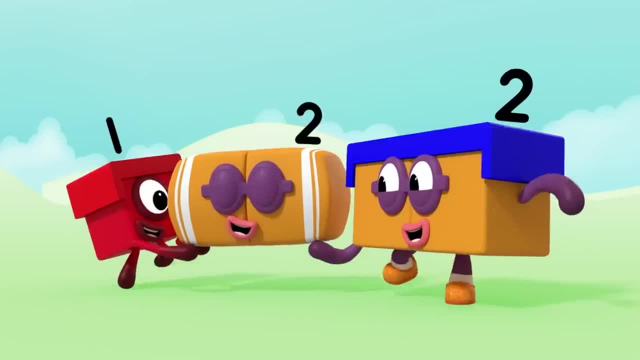 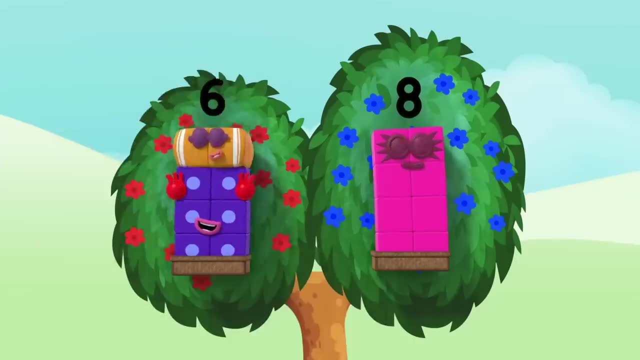 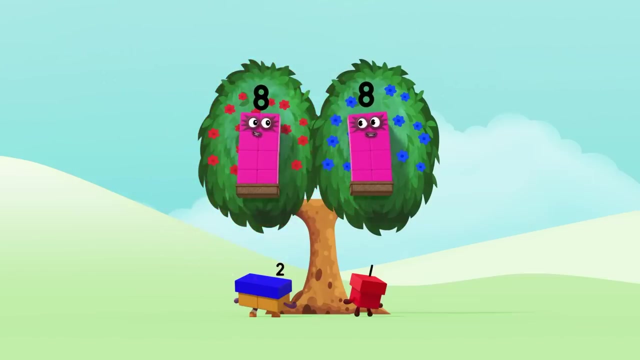 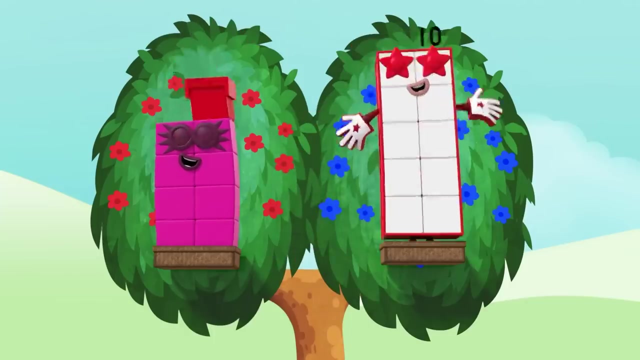 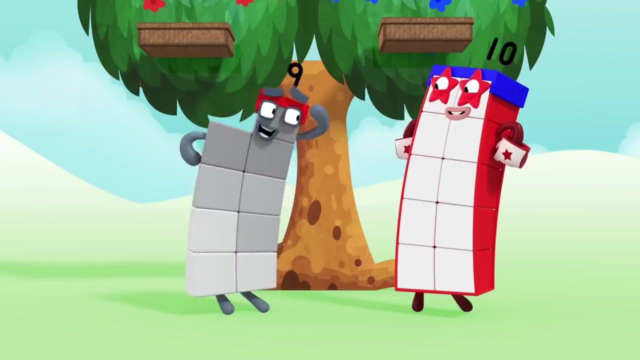 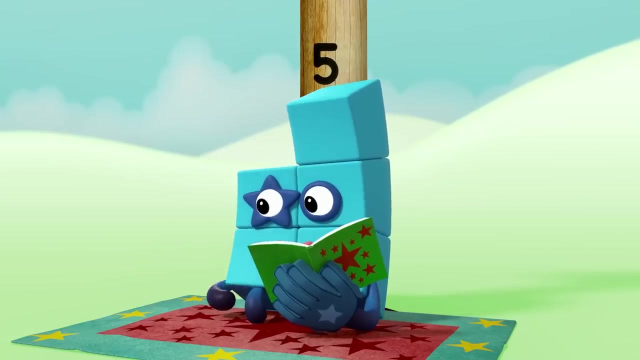 Or two, Six. Thanks, two Up there, please, One, two. Yay, There, Hang on Eight points each. It's a draw. Woo, That was fun. Same time tomorrow. Game on: Found you. 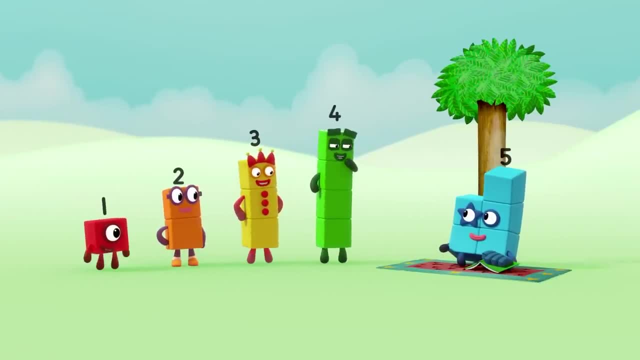 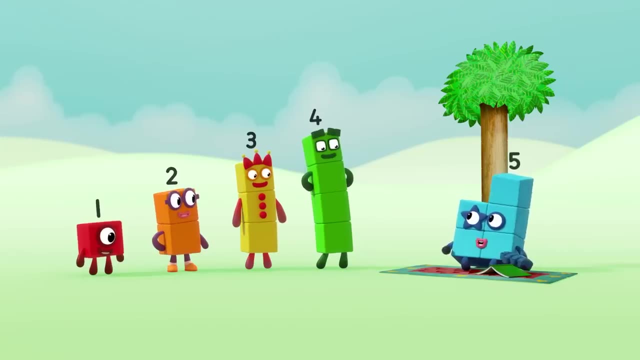 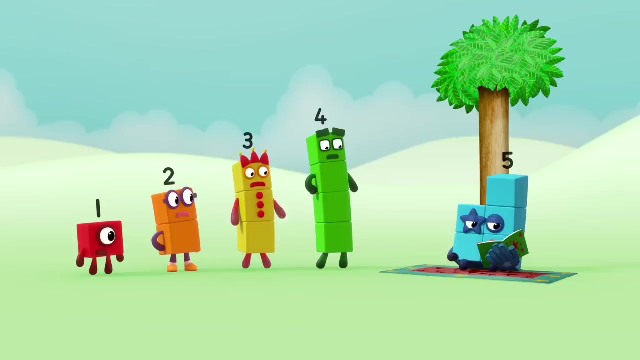 There she is. Hello, We're playing hide and seek. Want to join in? I would absolutely love to You hide, and I'll seek. Huh, You won't find us sat there. Oh, will I not now? I'm good at this game. 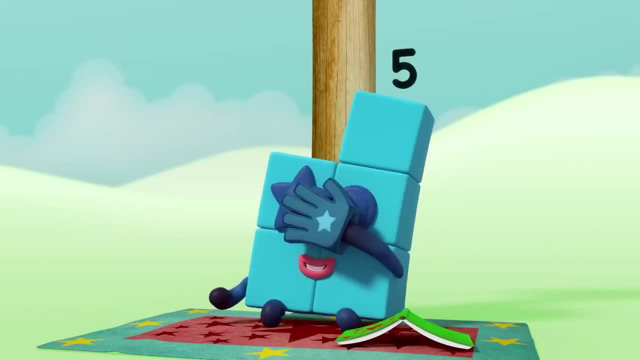 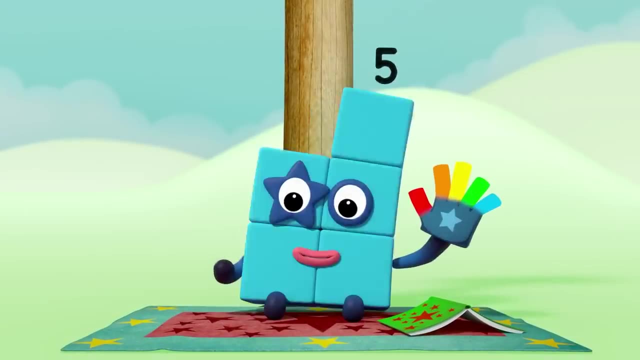 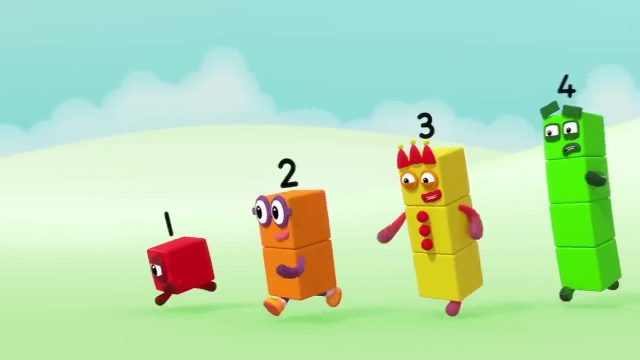 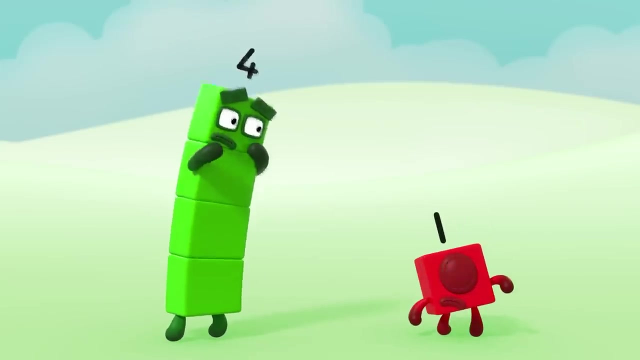 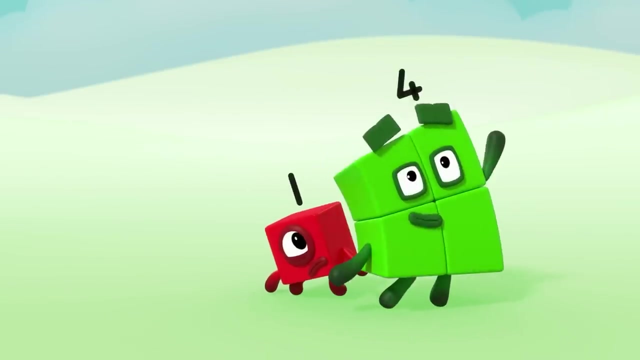 I'll find you and point you out. One, two, three, four, five, Ready or not, here I Get on with my book. Ooh, hey, hide behind me. Ha. Oh, Where can I hide? I know behind you. 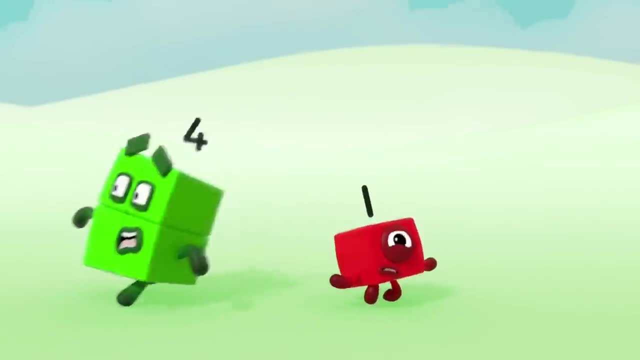 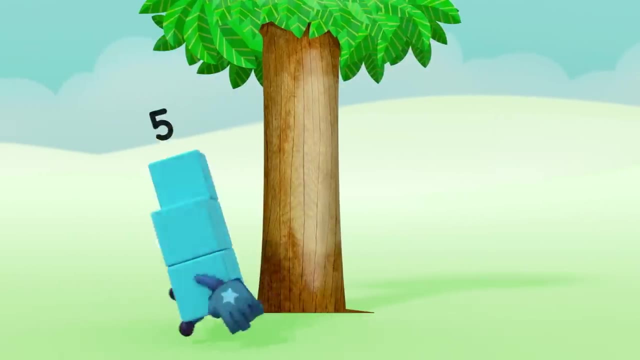 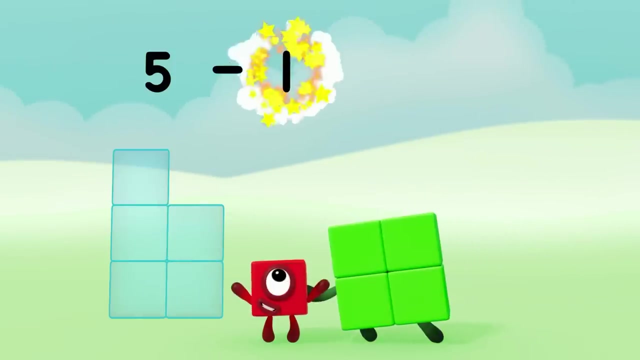 Four, Oops Huh, Four Plus one Equals five. Ready or not, here I come. Find you four, find you one, Ha-ha-ha. Five minus one Equals four. Look five, said she'd point us out. 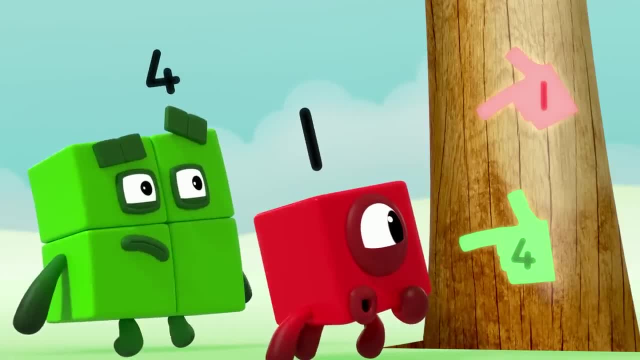 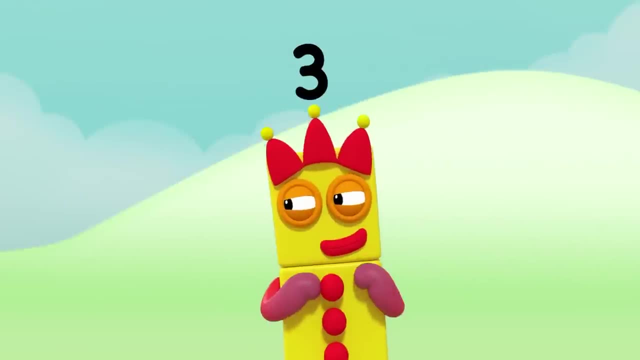 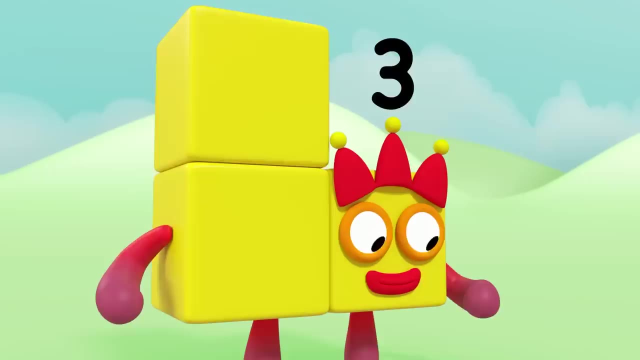 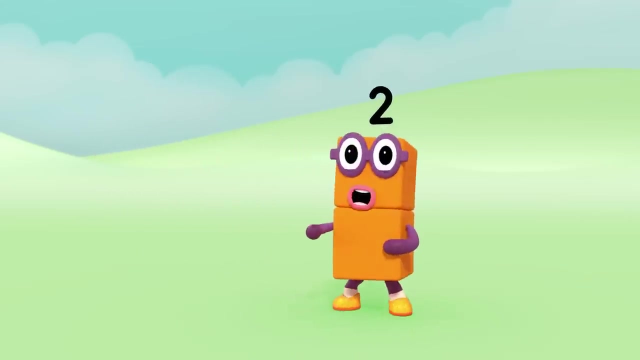 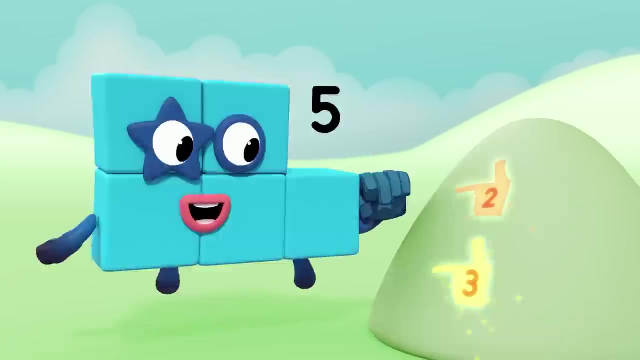 Five was right here. How I am. Three, Master of Disguise, Ah Shh Shh. Two Plus three Equals Five. Ready or not, here I be. Find you two, find you three. Five minus three. 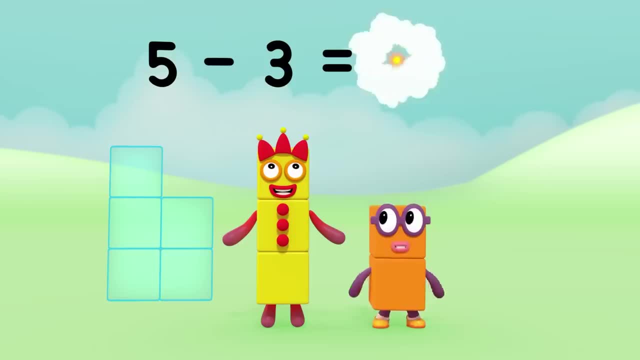 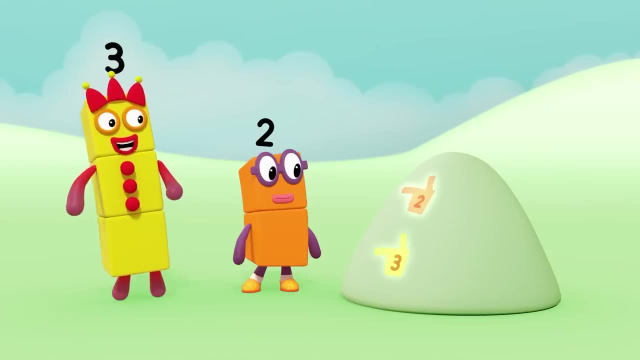 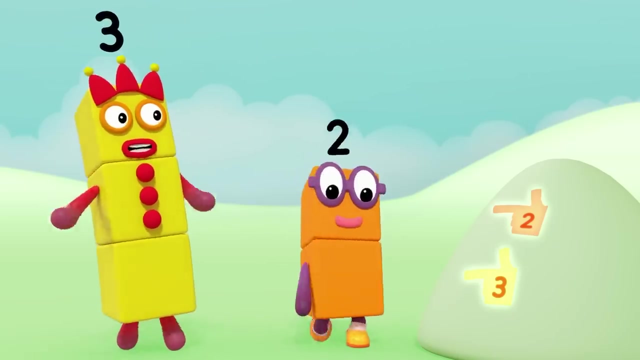 Equals two: A pair of pointing prints. Five found us, But but how? I don't know, I don't know How? Eh, Mm-mm-mm-mm-mm Five, You're here. How did you? Ha-ha-ha. 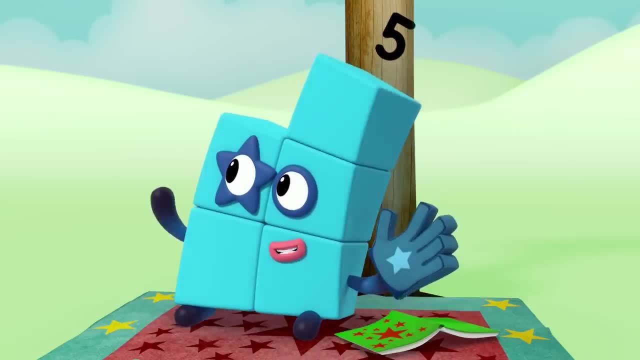 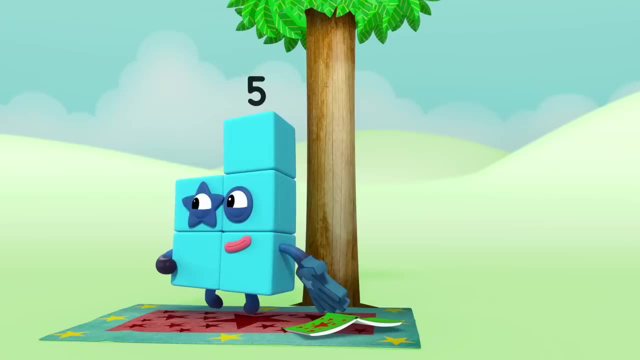 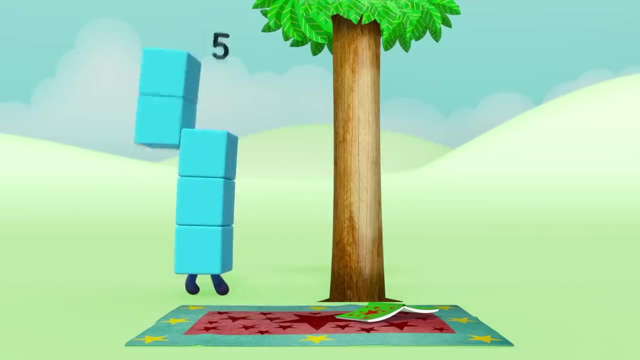 Told you I was good Ha. Now my turn to hide. All together, One, Two, Three, Four. Ready or not? Five, here we come, Ha-ha, Ooh, Ha-ha-ha, Ha-ha-ha. 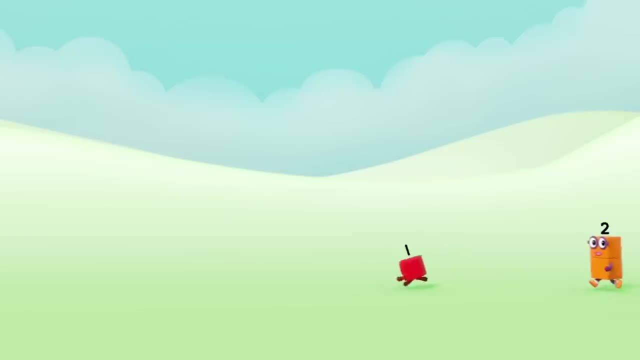 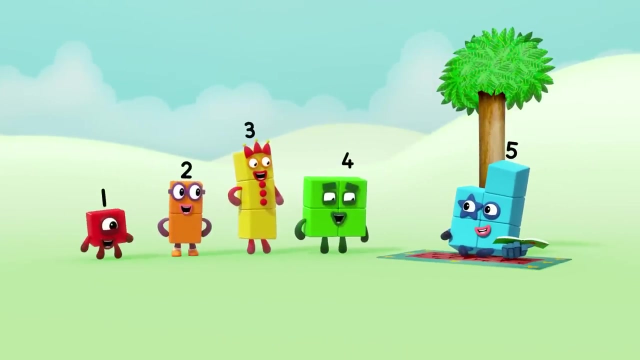 Rock One Plus four Equals Five. Found you. Amazing, Can you find me again? Five Minus four Equals one. Come on, Rock. Three Plus two Equals Five. Found you, Fantastic, Can you find me again? Five Minus two Equals three. Found you. You, stars, You all find me. 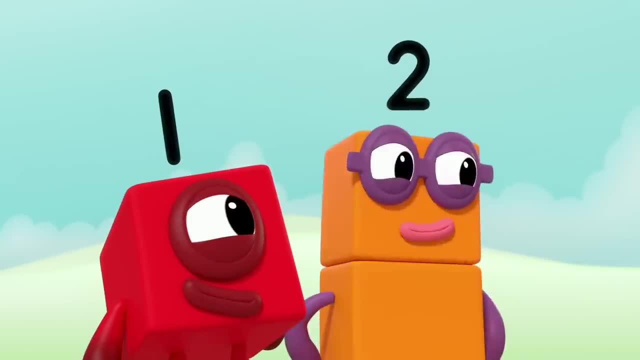 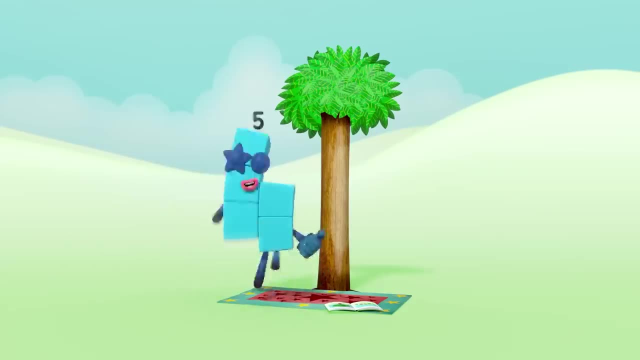 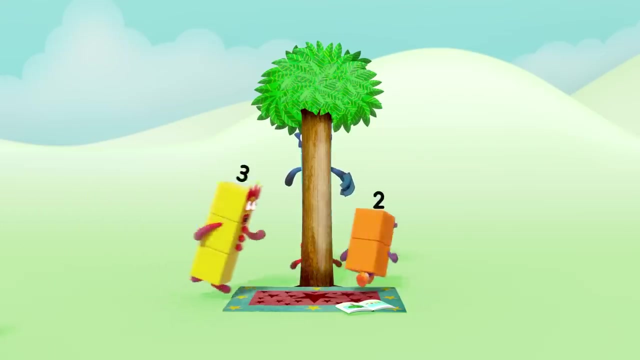 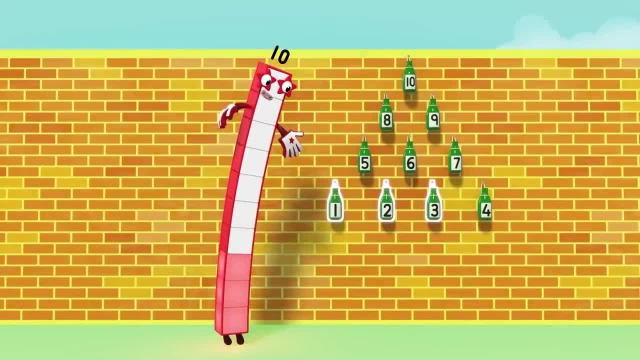 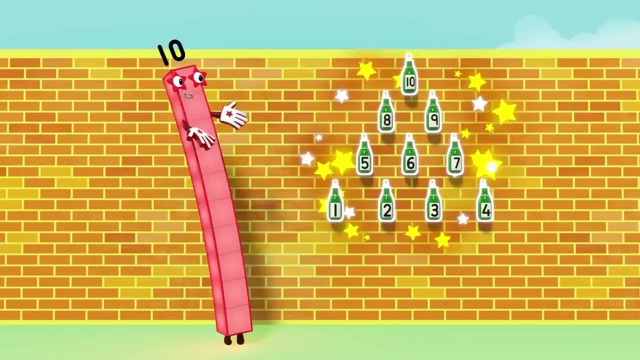 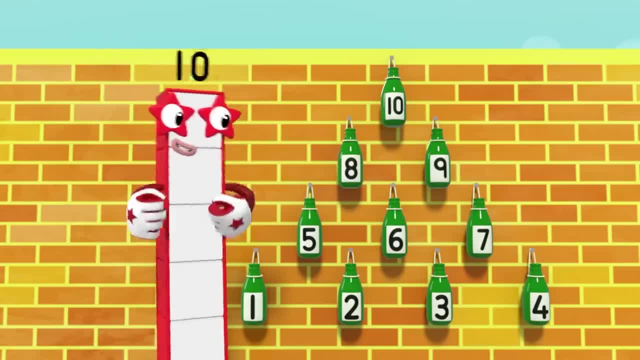 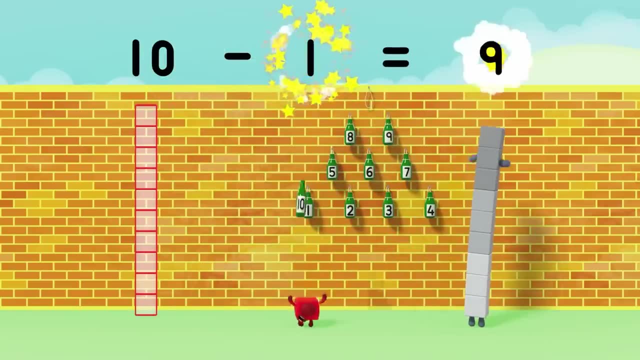 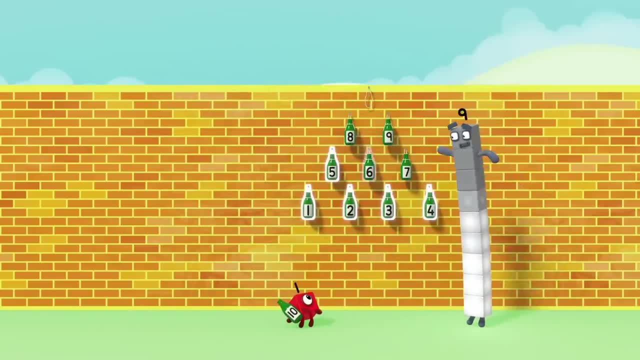 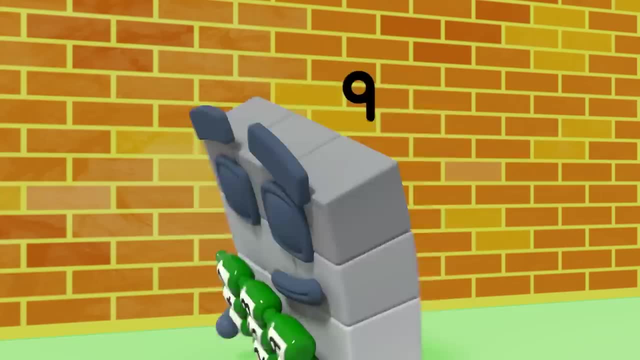 I'm going to try. I'm going to try. One, two, three, four, five, six, seven, eight, nine. Nine green bottles hanging on the wall. Better move these nine before they fall. They're not safe up there. Nine green bottles safely on the floor. 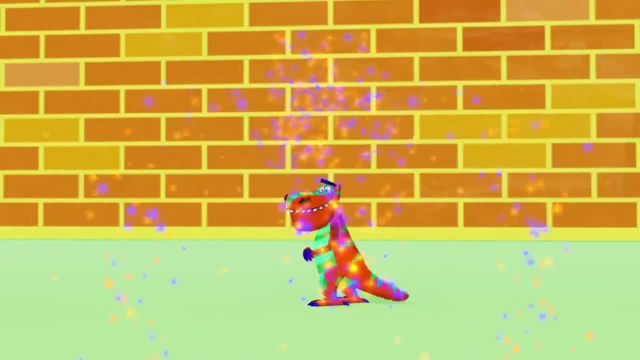 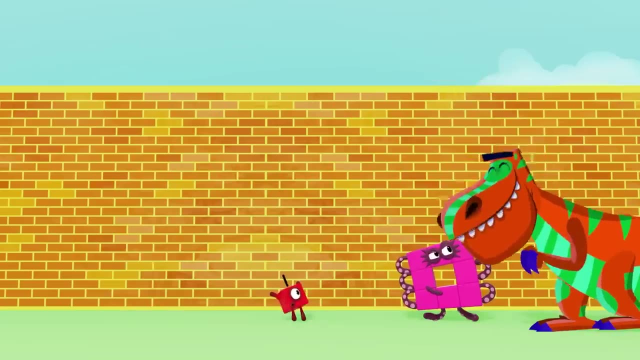 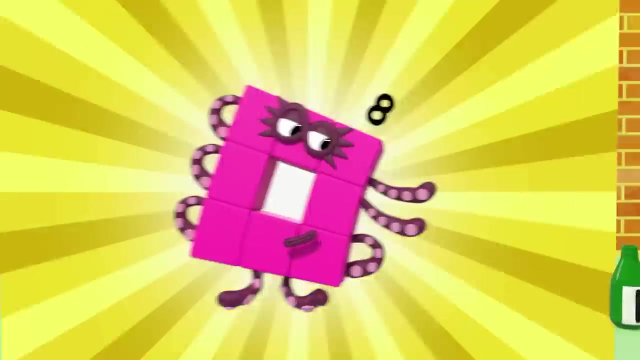 Nine green bottles safely on the floor. Oh, Oh, Ah, Oh Ah Achoo. But if one green bottle becomes a dinosaur, There'll be one, two, three, four, five, six, seven, eight, Eight green bottles not safe on the floor. 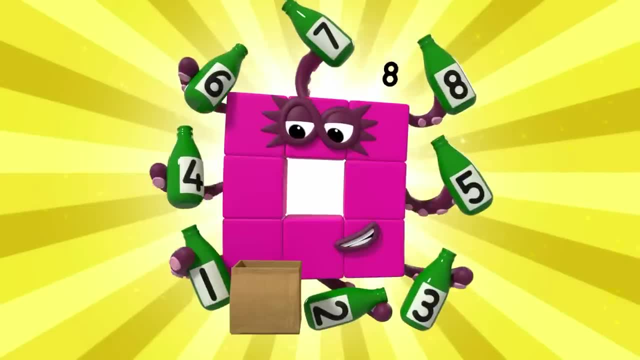 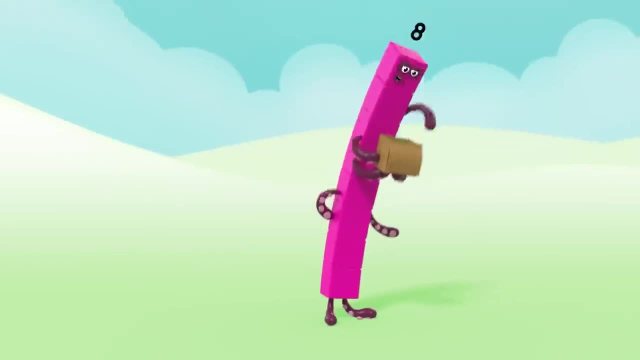 Octoblock hide One, two, three, four, five, six, seven, eight. hide Eight green bottles hiding in a box. Eight green bottles hiding in a box. But if one green bottle is stolen by a fox, Hey. 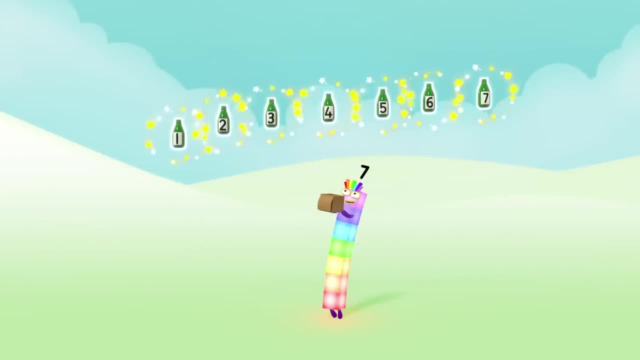 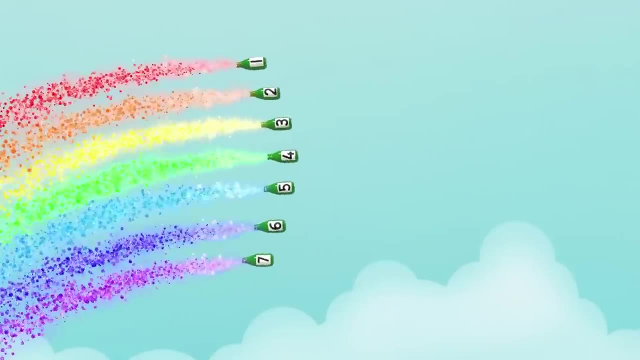 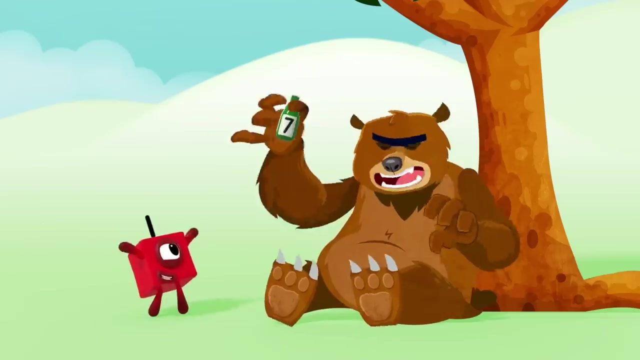 There'll be one, two, three, four, five, six, seven, Seven green bottles hiding in a box. That was lucky. Oh, Seven green bottles flying through the air. Seven green bottles flying through the air. But if one green bottle should wake a grizzly bear. 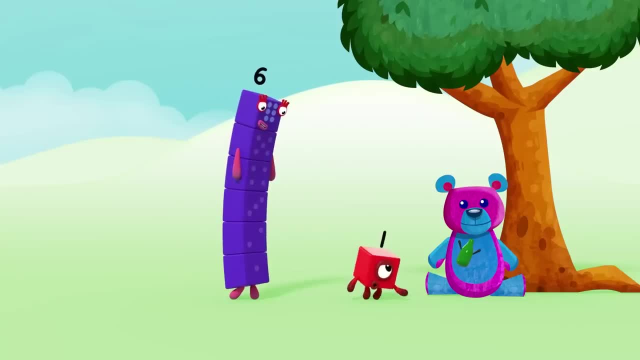 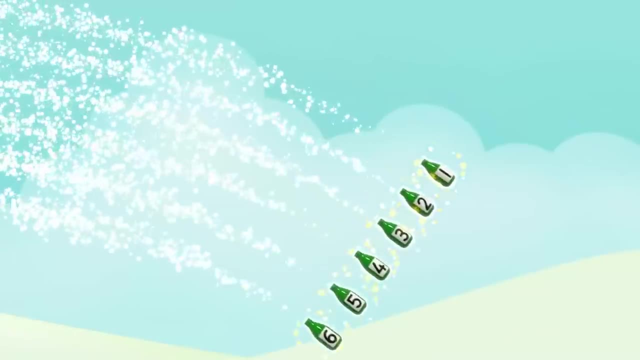 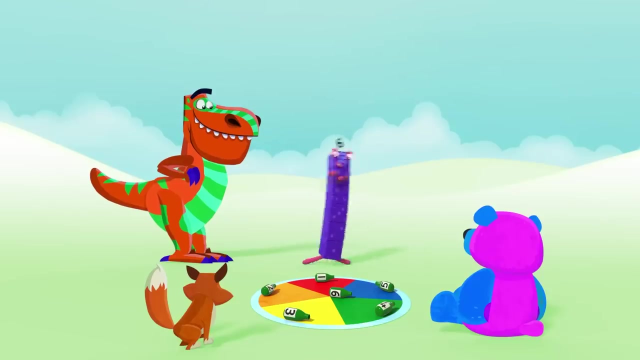 What I mean. hug a teddy bear. Phew, There'll be one, two, three, four, five, six, Six green bottles falling through the air. Six is my name. Let's play a game, And this game goes like this. And this game goes like this. 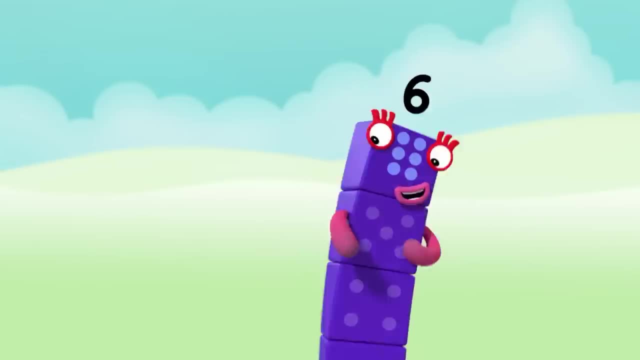 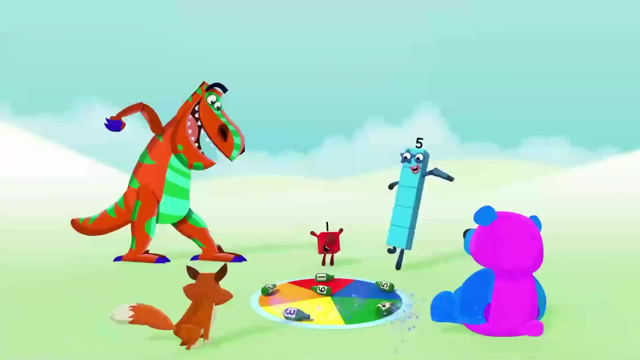 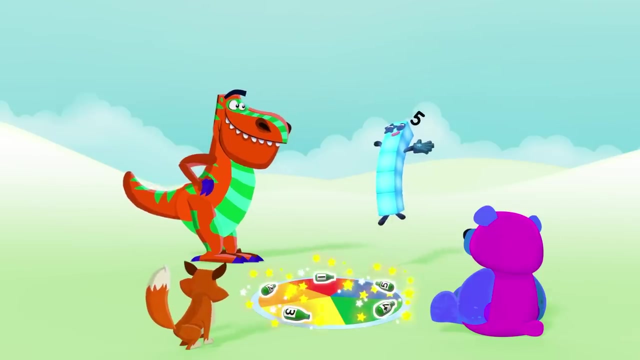 Six green bottles lying on the ground. Six green bottles lying on the ground, And if one green bottle spins around, Whoa, You win. There'll be one, two, three, four, five, Five green bottles lying on the ground, Yeah, Yeah. 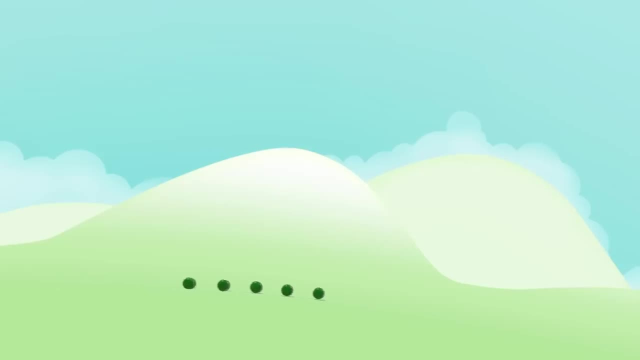 Yeah, Yeah, Yeah, Yeah Yeah. Five green bottles rolling down the hill. Five green bottles rolling down the hill, Yeah, And if one green bottle should grow a dapple-dill, There'll be one, two, three, four, four, four green bottles rolling down a hill. 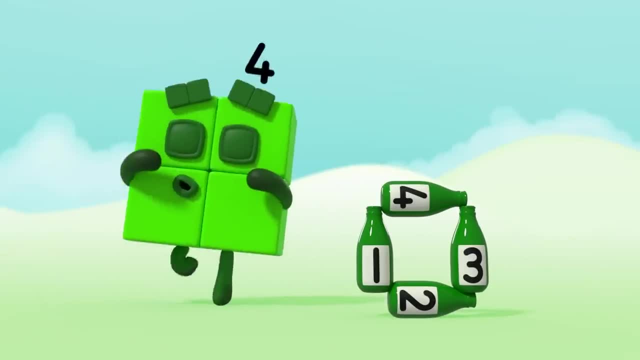 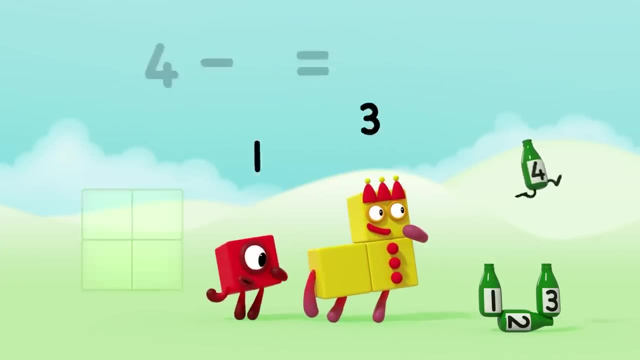 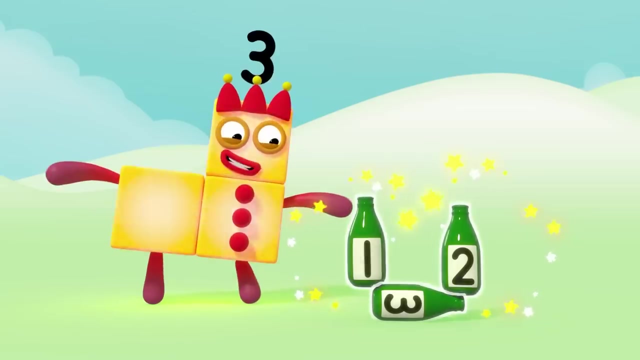 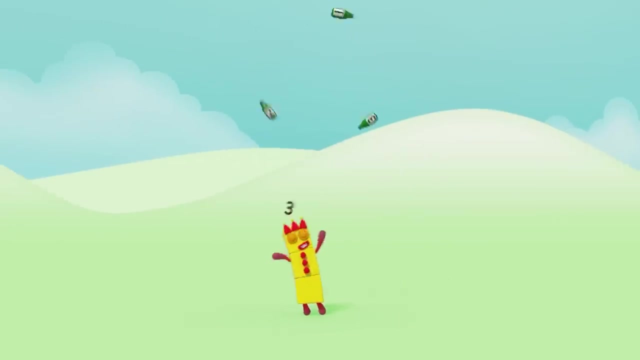 Four green bottles standing in a square. Four green bottles standing in a square, But if one green bottle should run to the bear, There'll be one, two, three, three green bottles Standing in a triangle. One, two, three, Three green bottles spinning in the sky. 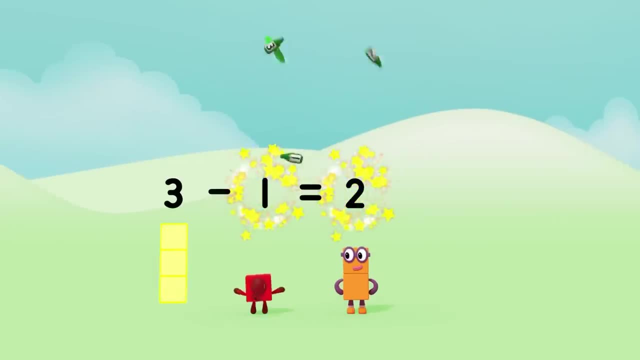 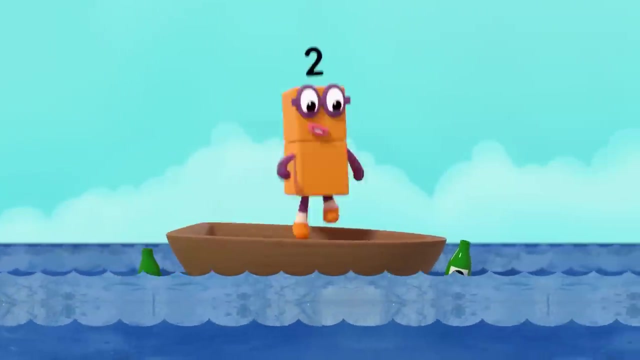 Three green bottles spinning in the sky, But just one green bottle shall pop its wings and fly. There'll be one, two, three green bottles spinning in the sky. Come back. Two green bottles floating out to sea. Two green bottles floating out to sea. But if one green bottle should learn to watch a sea, 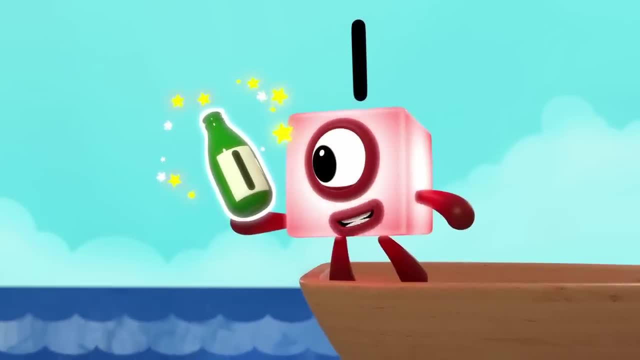 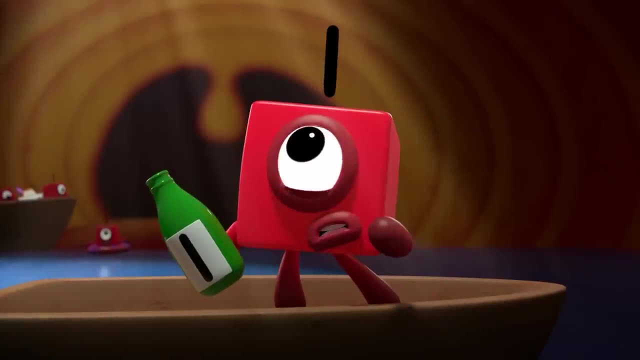 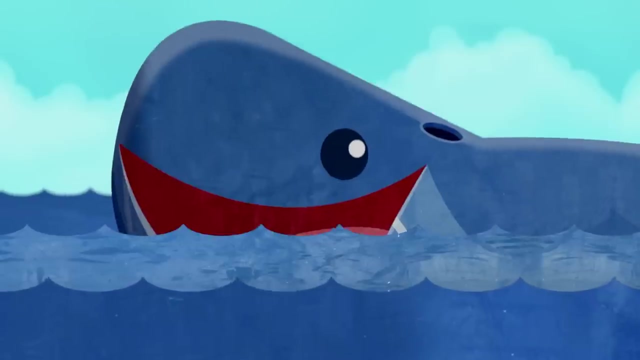 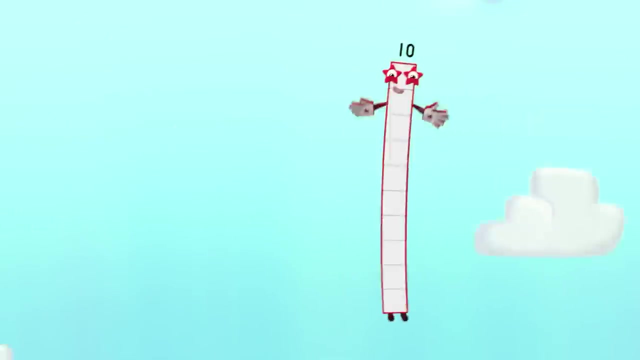 There'll be one one green bottle floating out to sea, One green bottle swallowed by a whale, One green bottle swallowed by a whale. But if that green bottle should grow a tickly tail, There'll be no green bottle swallowed by a whale. Ten green bottles hanging on a wall. 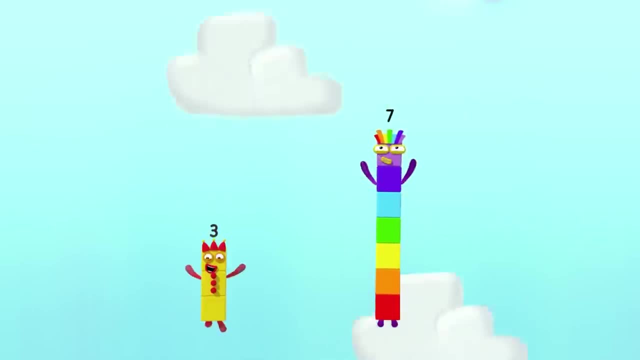 Safely on the floor, hiding in a box, Flying through the air, lying on the ground, Ten green bottles rolling down a hill, Standing in a square, spinning in the sky, Floating out to sea, swallowed by a whale. But if one green bottle should accidentally fall, 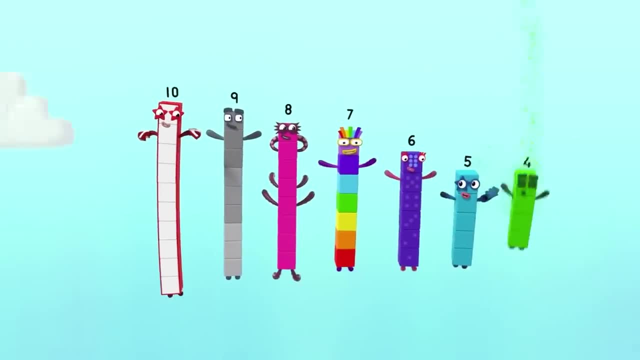 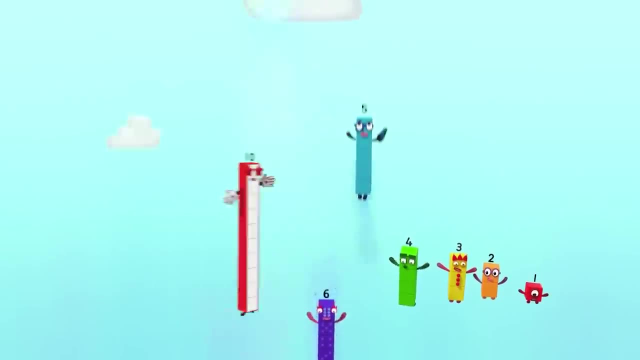 Become a dinosaur. wake up to sleep there, Spin around up a hill, fly between some flies, Learn to watch a sea grow a tickly tail. There'll be one, two, three green bottles spinning in the sky. Nine, eight, seven, six, five, four, three, two, one. 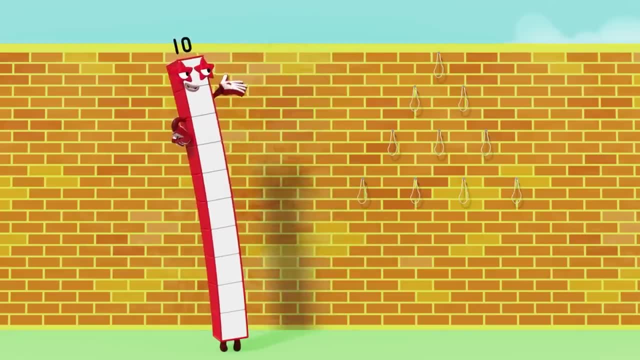 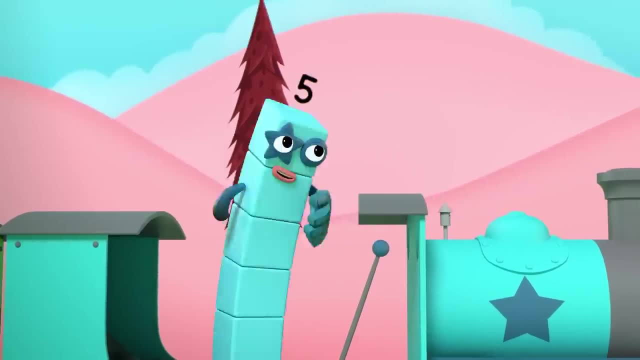 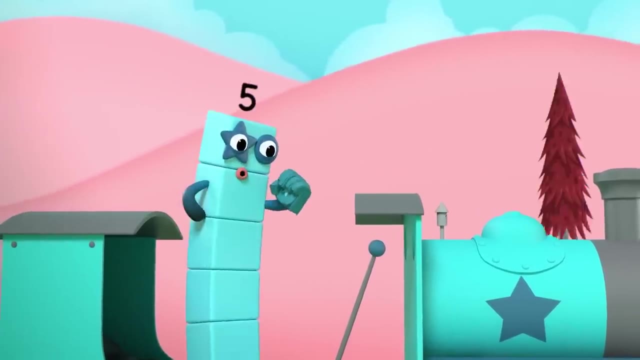 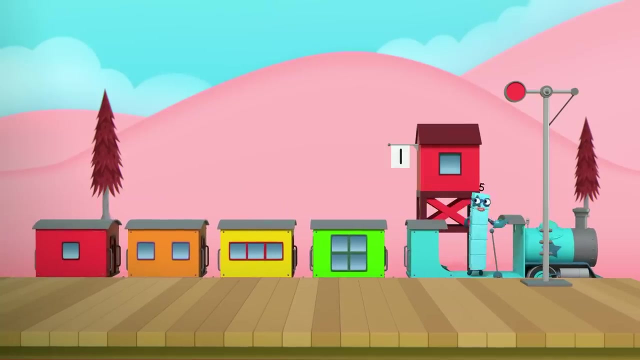 No green bottles hanging on the wall. I am five. I feel alive Whenever I can drive my train. Only five, no more, no less, Can drive the number black, six, brick, Woo-hoo. No one getting on the train. Let's be on our way again. 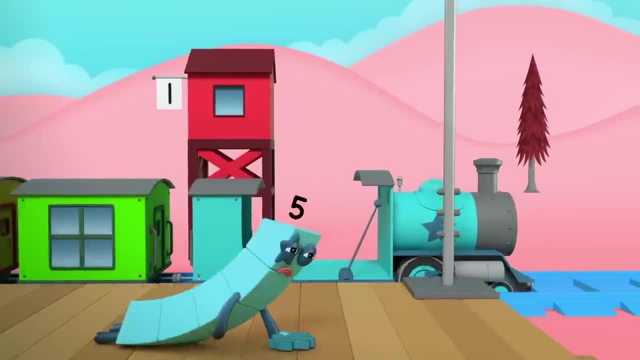 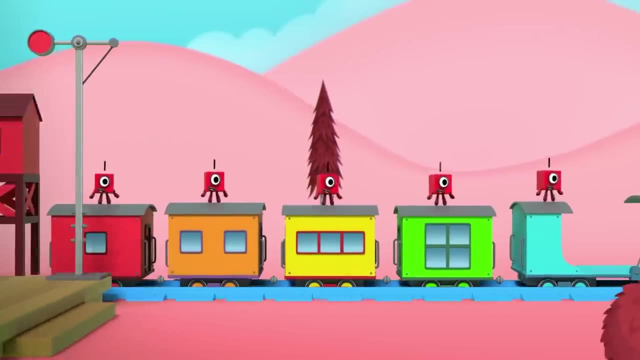 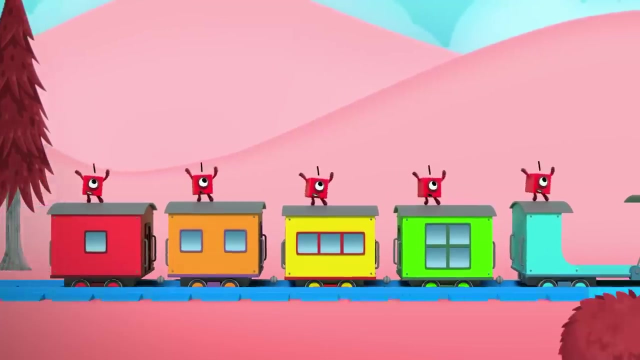 Woo-hoo, We have to get the train to stop. So hop, hop, hop, hop, hop on top. Only five can stop the train. So how do we make five again? Only five, no more, no less, Can stop the number blocks express. 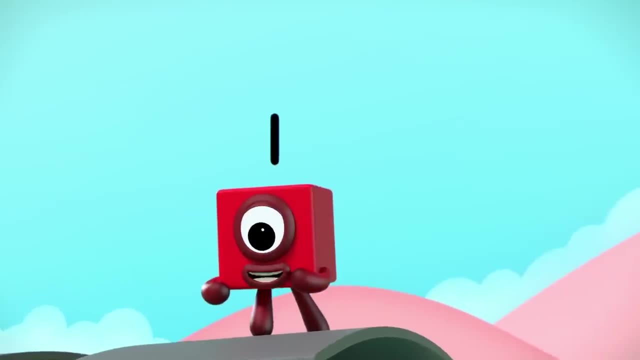 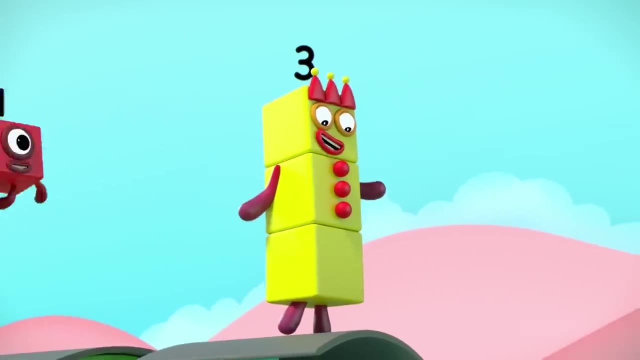 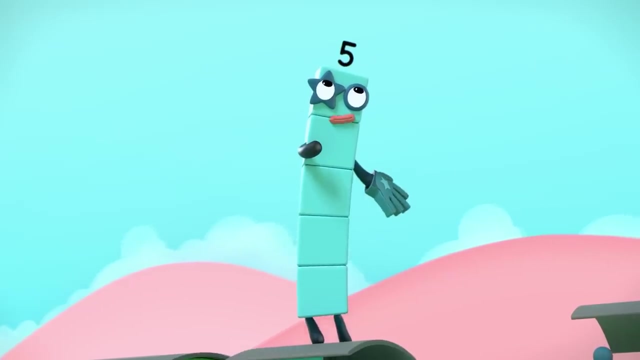 Woo-hoo, I think I know what must be done. Let's stop the train by adding one. One plus one equals two. Two plus one equals three. Three plus one equals four. Four plus one equals five. Only five can stop the train, And I am back to five again. 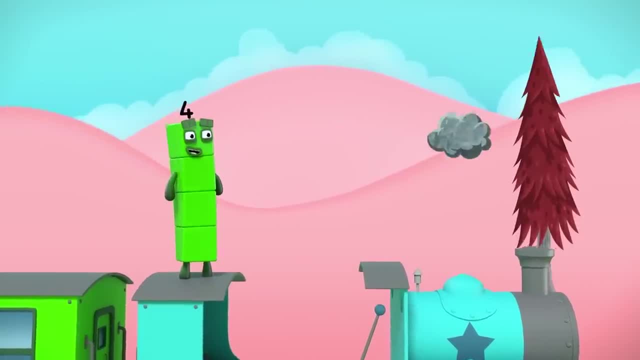 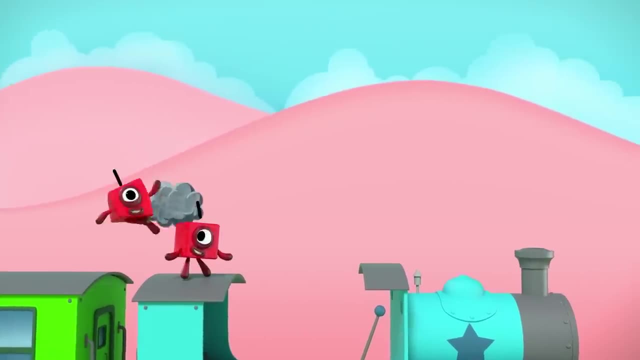 Woo-hoo, Five minus one equals four. Woo-hoo, Four minus one equals three. Woo-hoo, Three minus one equals two. Woo-hoo, Two minus one equals one. Woo-hoo, Woo-hoo. Can you help us, pretty please. 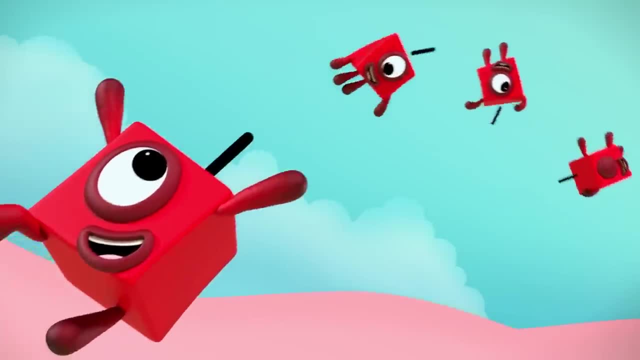 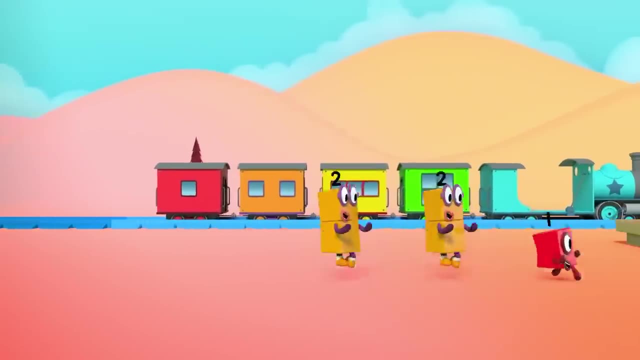 Can you help us, pretty please? We need to get back on the way. Only five can stop the train. So how do we make five again? Only five, no more, no less, Can stop the number blocks express. Woo-hoo, We know what we have to do. 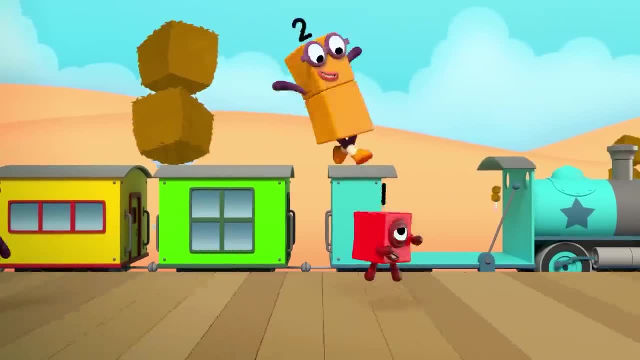 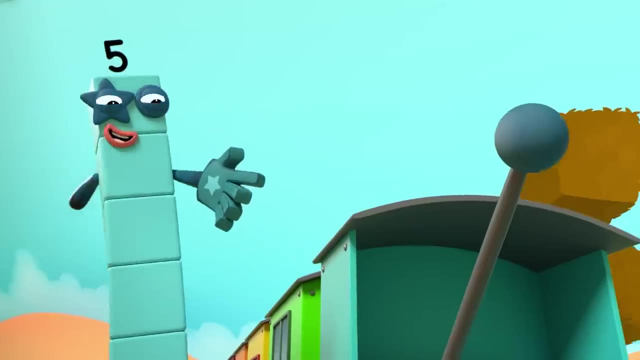 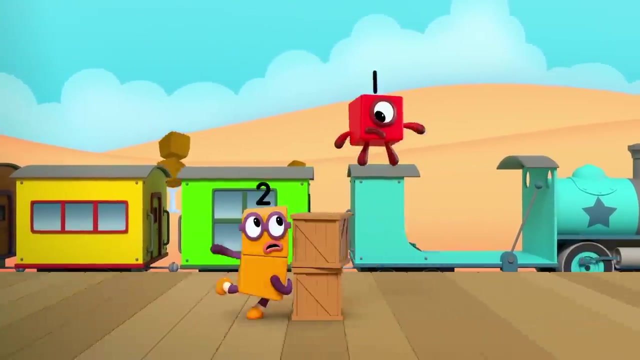 Stop the train by adding two. One plus two equals three. Three plus two equals five. Only I can stop the train. So I am back to try again. Woo-hoo, Five minus two equals three. Three minus two equals one. Ouch Ow, Come on twos. 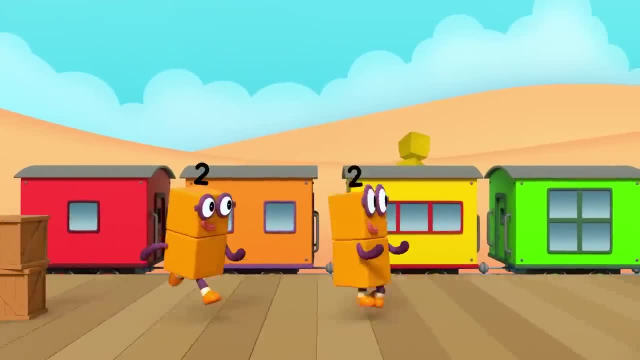 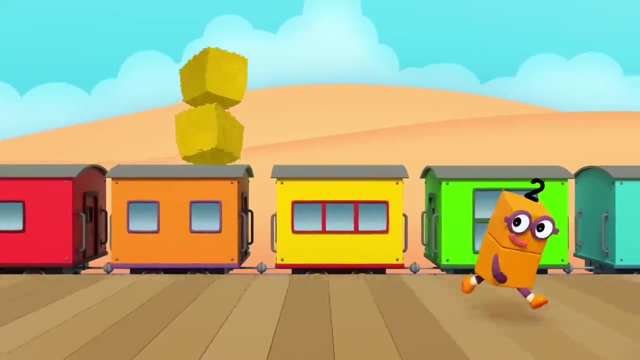 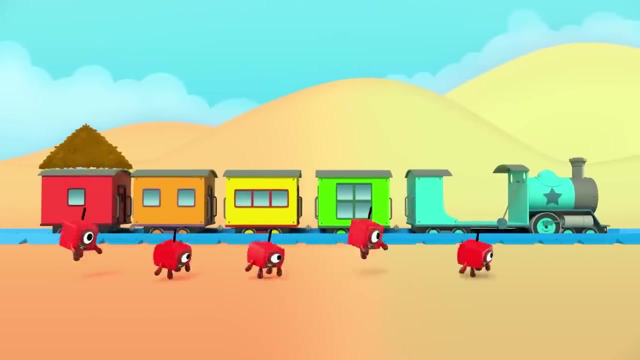 Time to act like kangaroos: Hop, hop, hop, hop. Two plus two equals four. Four minus two equals two. Only five can stop the train. So how do we make five again? Woo-hoo. Okay, friends, leave this to me. I'll stop the train by adding three. 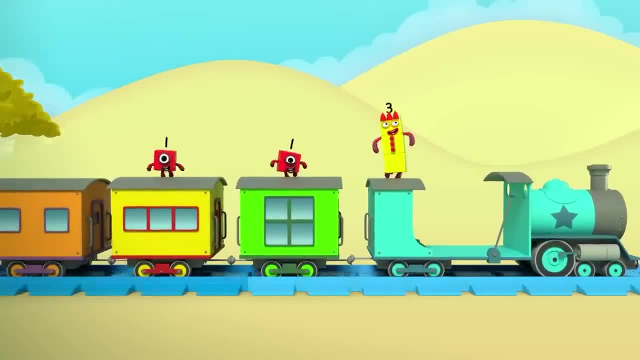 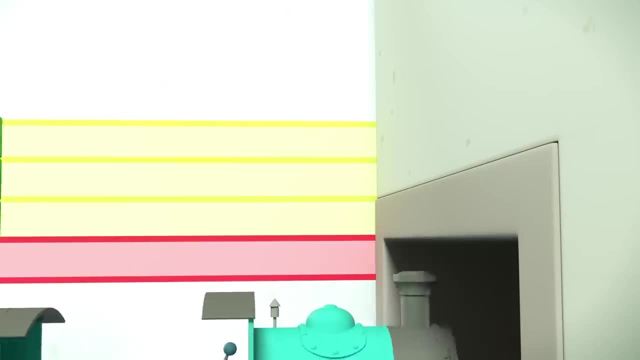 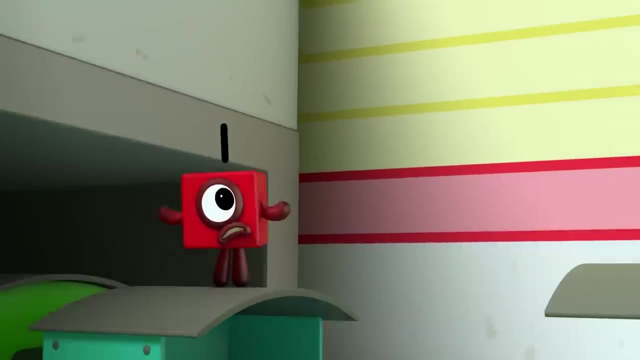 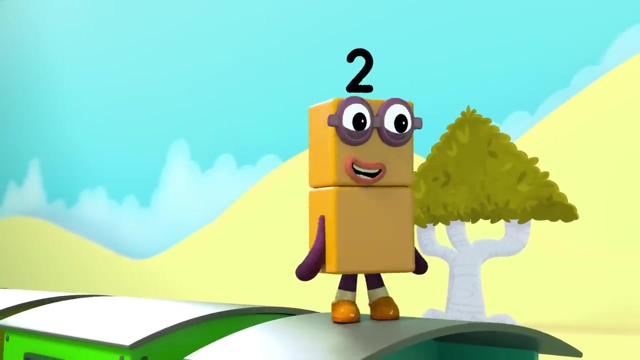 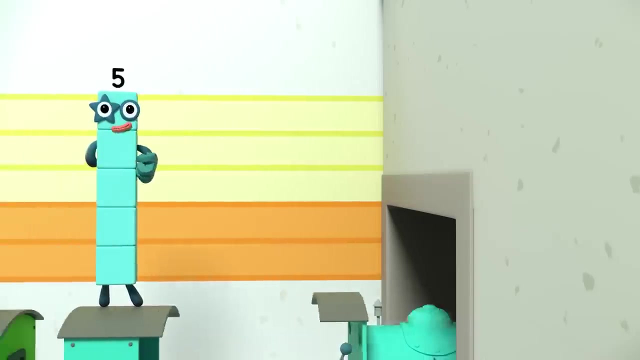 Hop, hop, hop on top. One plus three equals four. What does that mean? I'm not quite sure. I don't think I've seen that before. Minus three equals one. Hey, Two plus three equals five. Only I can stop the train And I am back to five. 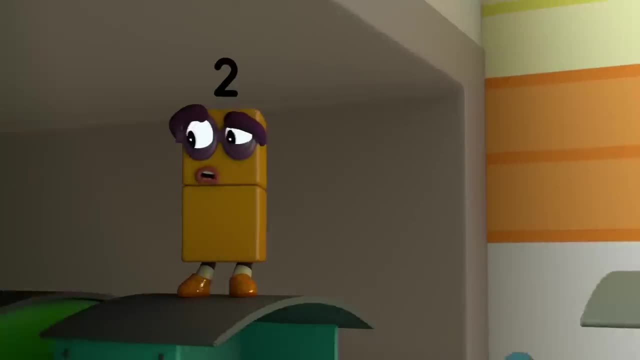 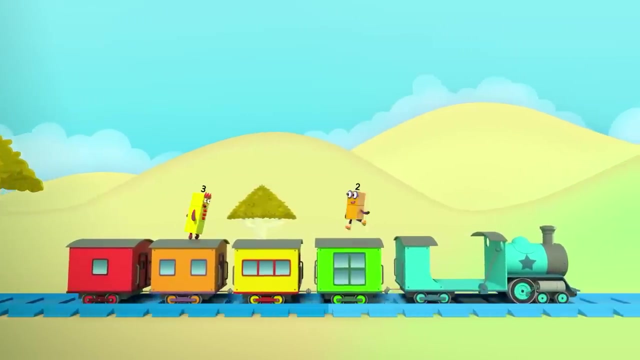 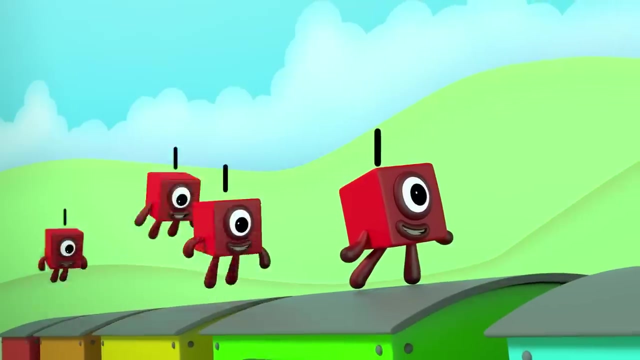 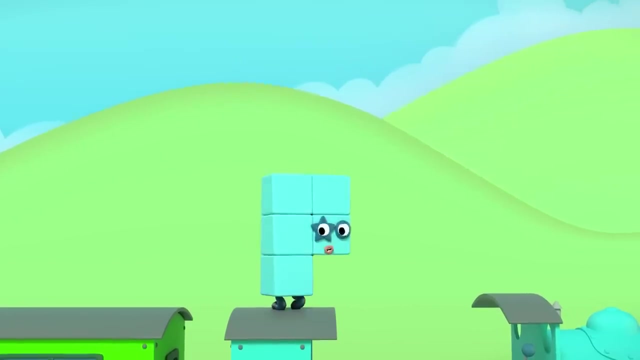 Minus three equals two. Hey, Only five can stop the train. So how do we make five again? I am square, you be war. Let's stop the train by adding four. One plus four equals five. Only I can stop the train. So here I am to try again. 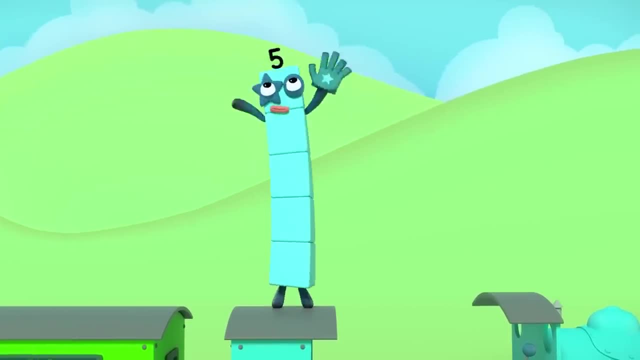 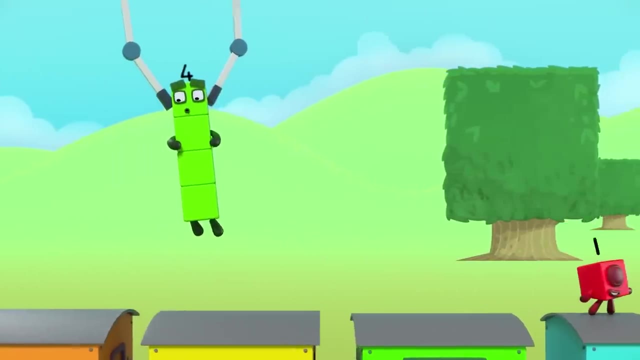 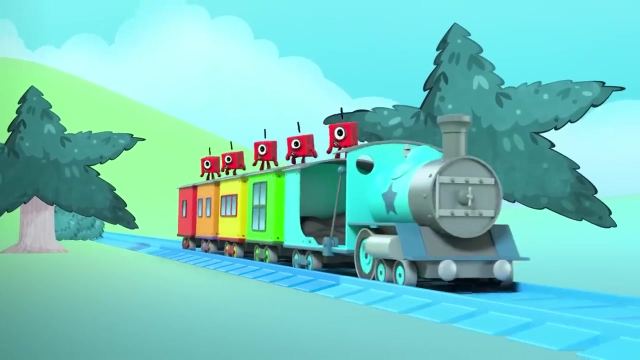 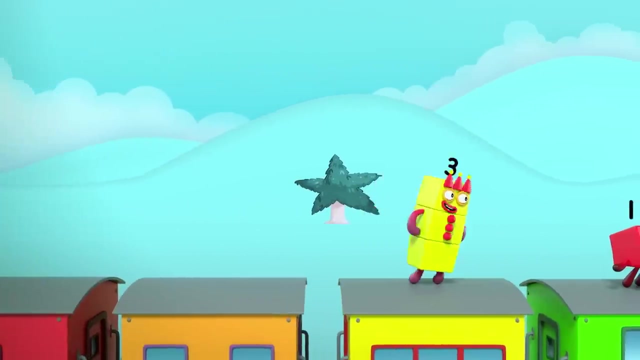 Only five, no more, no less, Can stop. the number blocks express Woo-hoo. Five minus four equals one. Only five can stop the train. So how do we make five again? One, two, three, four. Hey, Only five can stop the train. 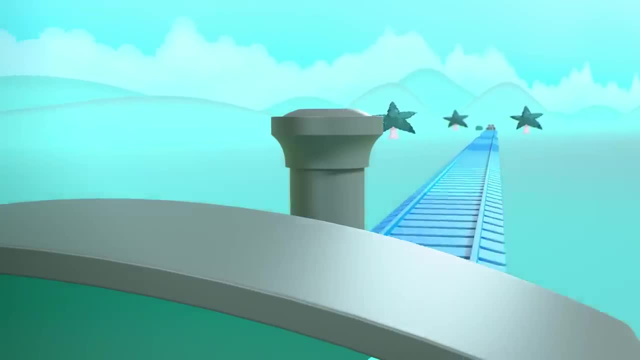 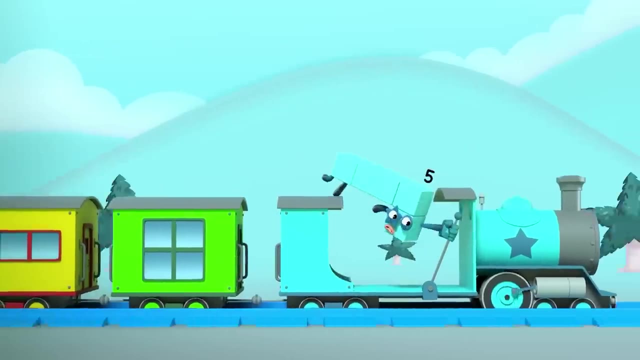 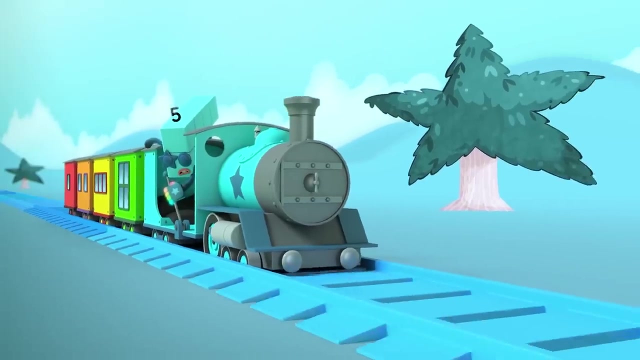 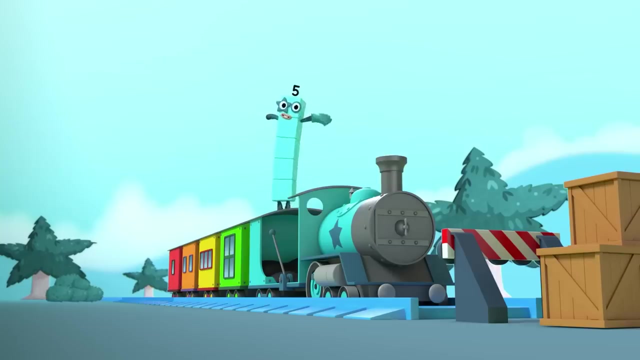 So here I am to try again. Uh-oh, no, we're in a mess. Stop the number blocks express. One, two, three, Four, five, High five. Success, I stopped the number blocks express. Woo-hoo Yeah. 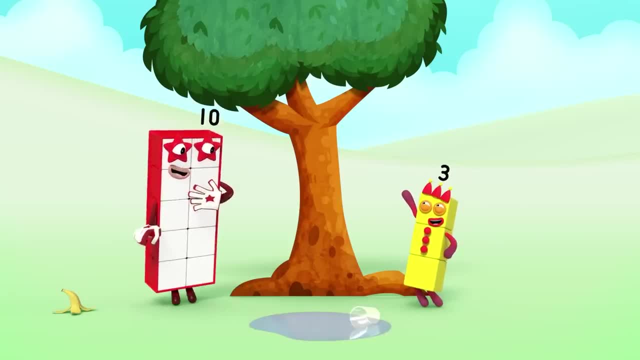 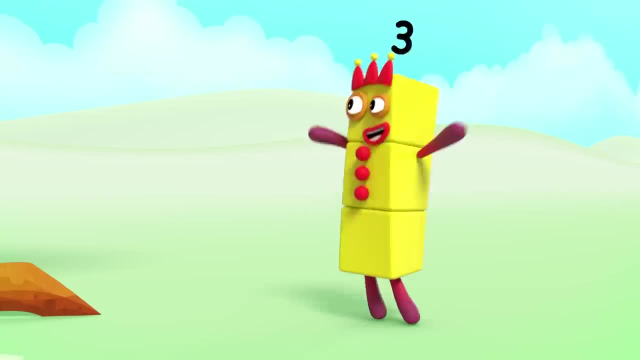 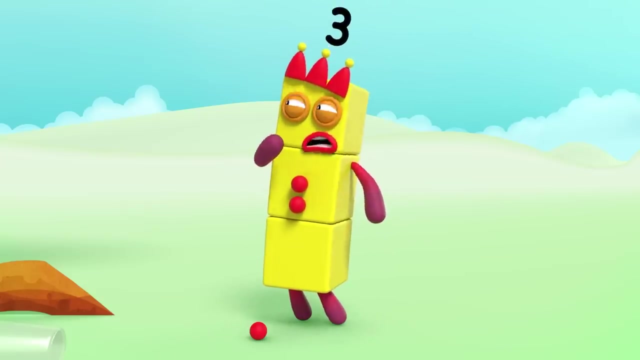 Bum-bum-bum Three, Oh sorry, Ten. I'm just so excited to show you my new trick. Look at this. Oh, Is that it? No wait, I'm not having much luck with mine today, Oh no. 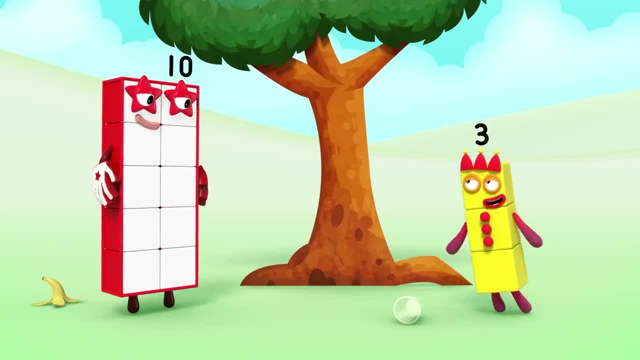 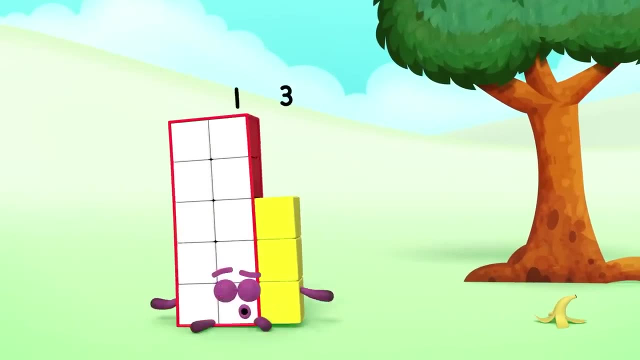 My new trick: Ready, steady go, Oh unlucky. Oh hi, Who am I? I'm one, two, three, four, five, six, seven, eight, Nine, ten, eleven, twelve, thirteen, Whoa. 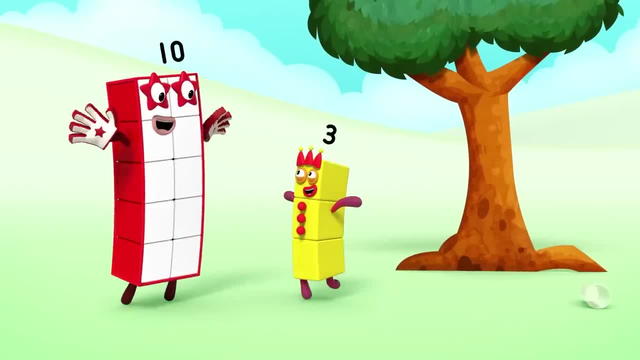 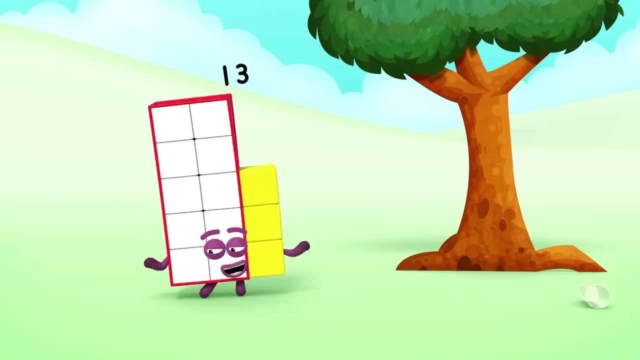 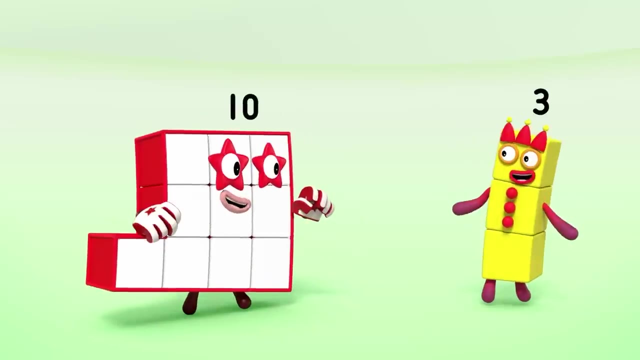 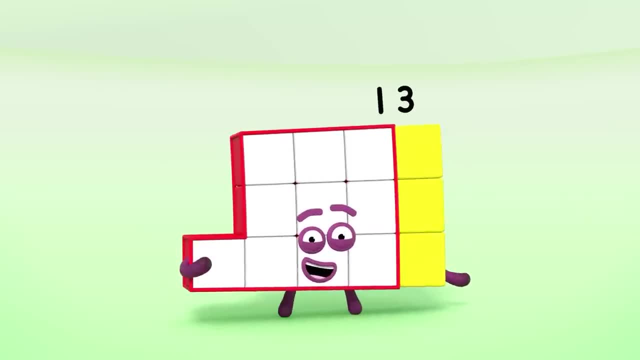 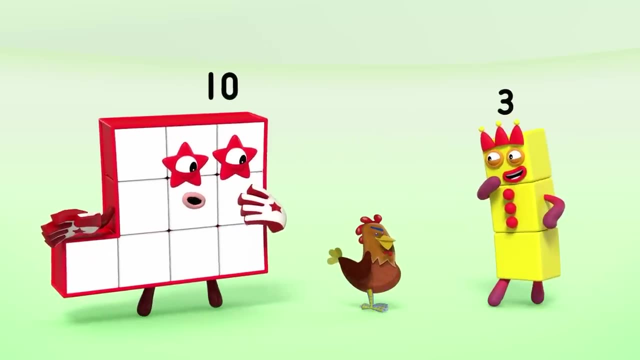 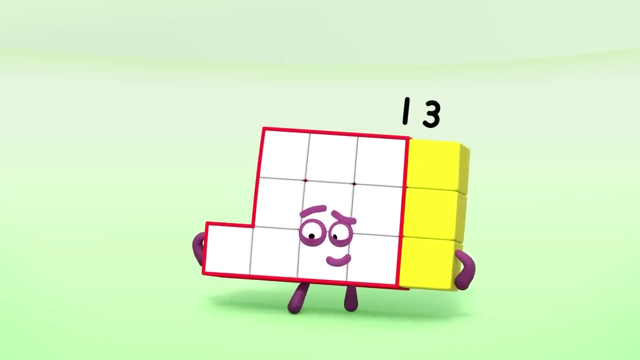 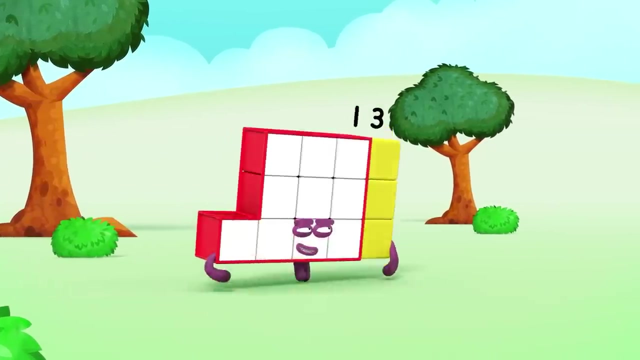 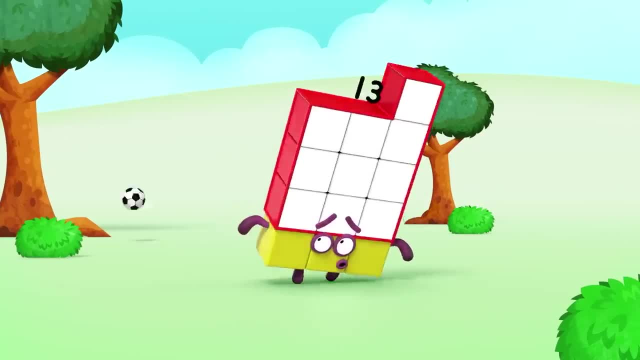 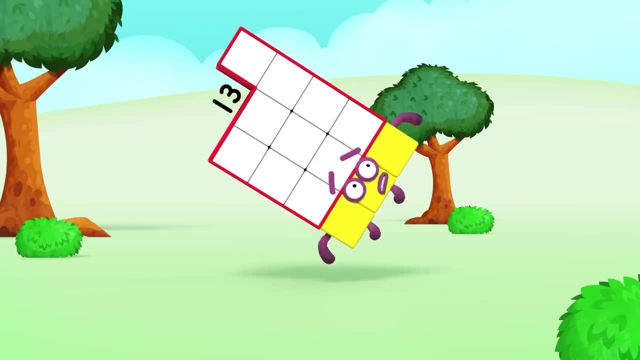 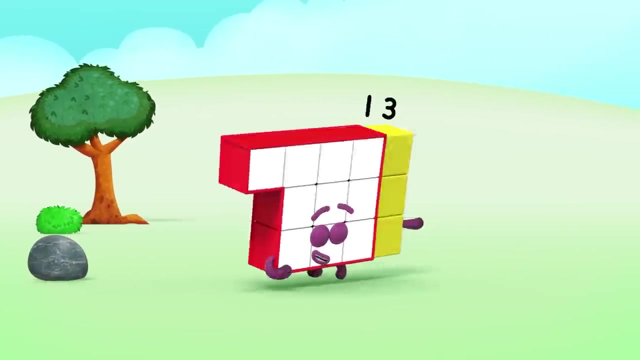 Expecting to run out of luck. Sorry, It's all jolly japes. When I get into scrapes I'm always coming. I'm the clumsiest number you've ever seen. Unlucky number 13. It's happened again. a three and a ten. 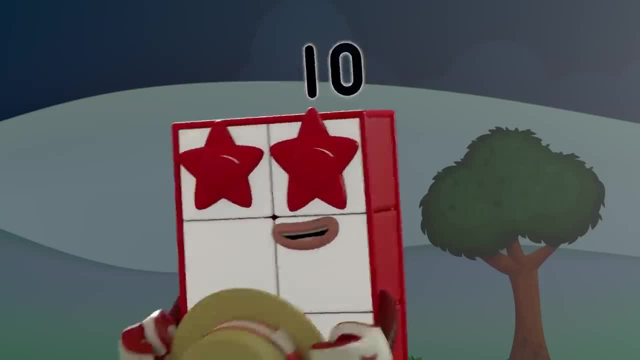 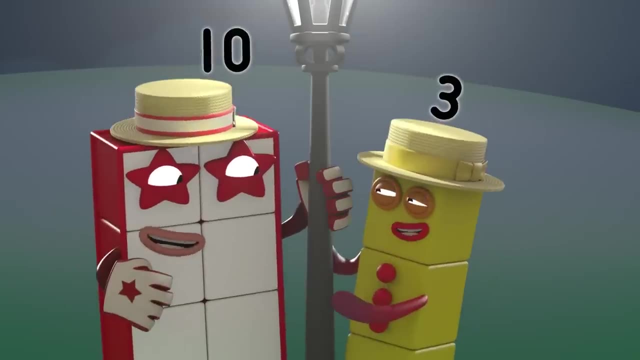 Somebody should tell him that it's happened again. I don't have the heart to be fussy or picky, But he's falling apart. he's a bit unsticky. It's happened again and no one knows when. Somebody should tell him that it's happened again. 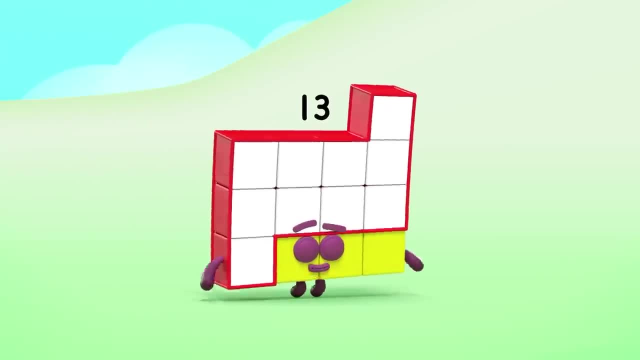 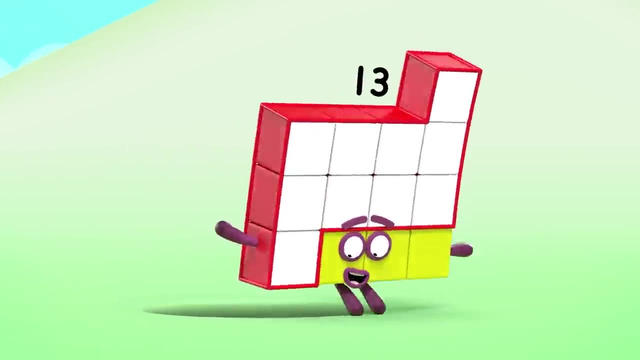 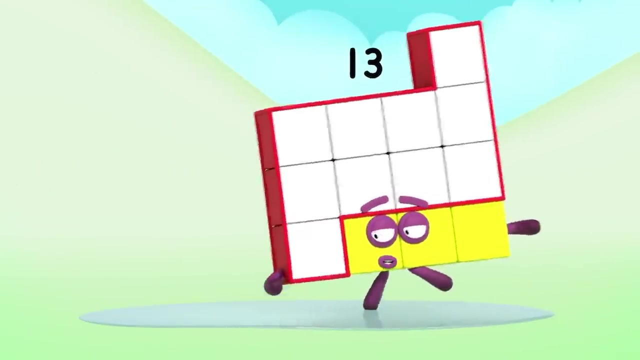 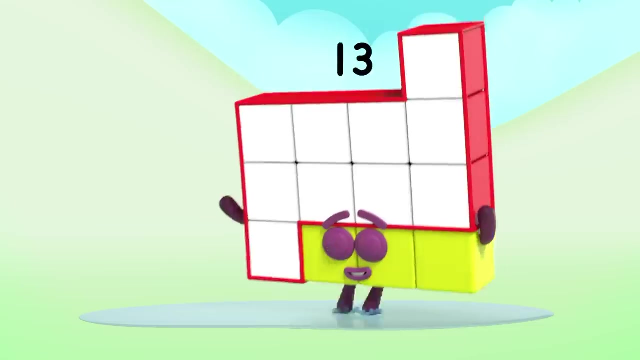 Me again, three and ten, Expecting to fall down a hole. I jump through a hoop and step in the puddle. That seems to sum up my role, And wherever I end up, I make a scene. Unlucky number 13. Unlucky number 13. 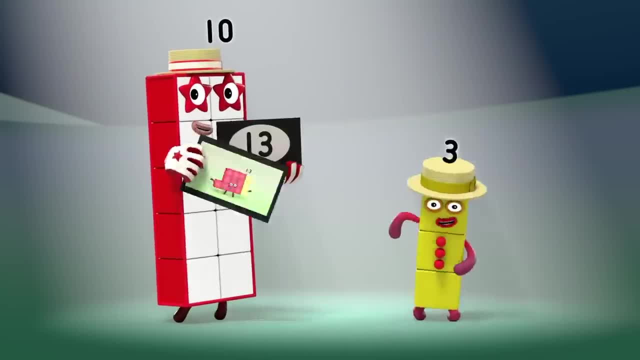 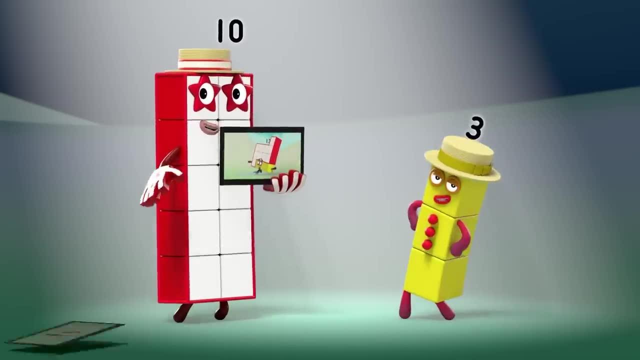 Unlucky number 13. It's always the same when he says his name, Somebody should tell him that's the name of the game. It's happened before a total disaster, But he's going to need more than a sticking cluster. It's always the same. we know what to blame. 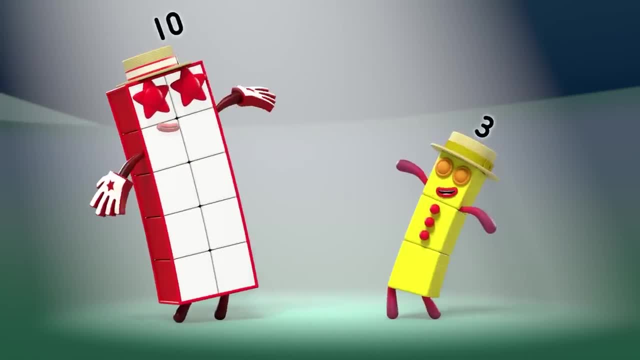 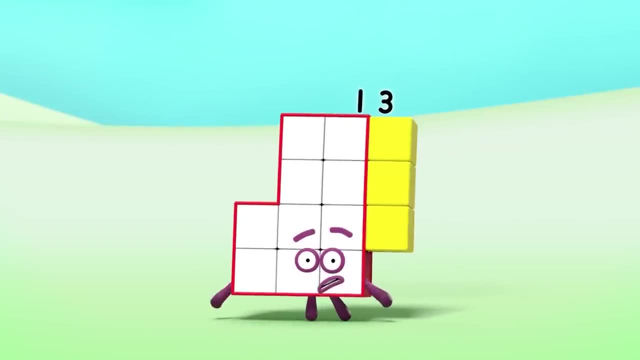 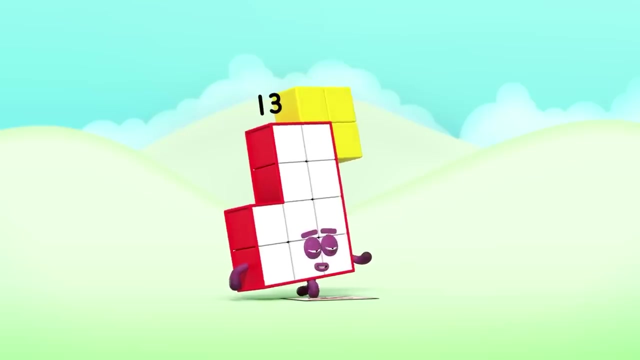 Somebody should tell him not to mention his name. It's getting routine. I say I'm 13, Keep it together. keep it together. This is absurd. You know what I mean? I say it's 13 And took my tether to say that word. It's always the same. it's getting routine. 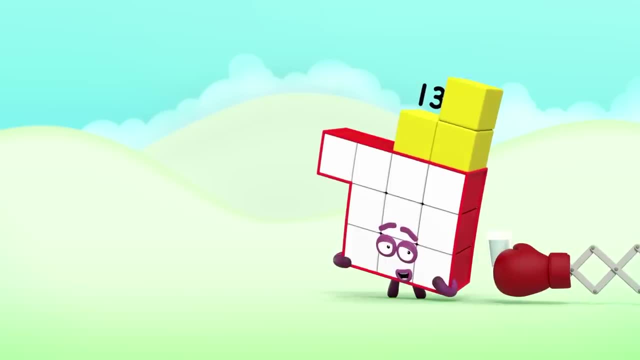 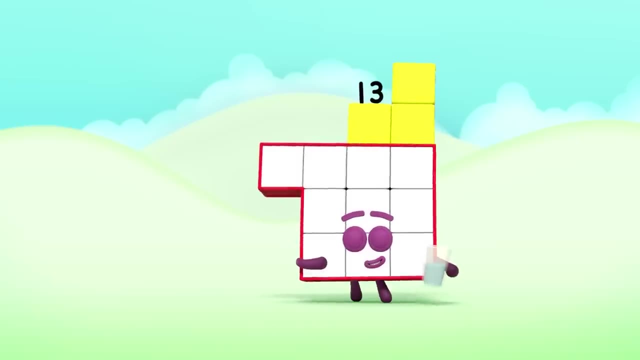 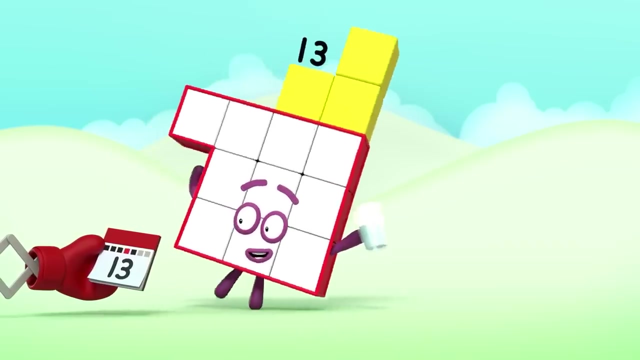 They ask me my name, I say I'm thir. Thirsty, I say I'm thirsty. They ask me my number. you know what I mean. And I always say it's a Thirsty. I always say it's Thursday. 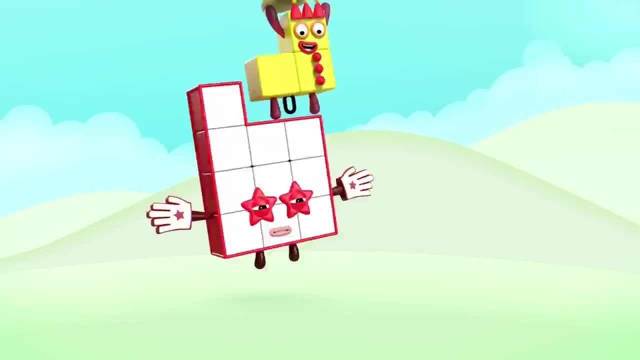 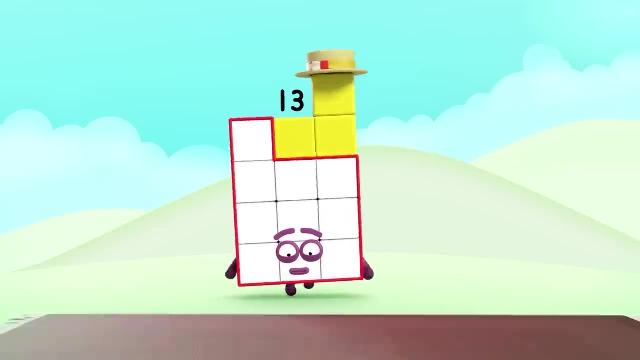 And he's joking. it's their time. This is me, 10 and 3, Turning this into a game. I'm changing my luck. I won't come unstuck As long as they don't say my name. Call me one more than 12 or 10 and 3. 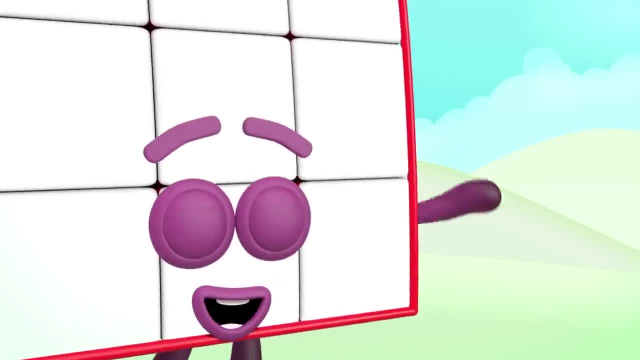 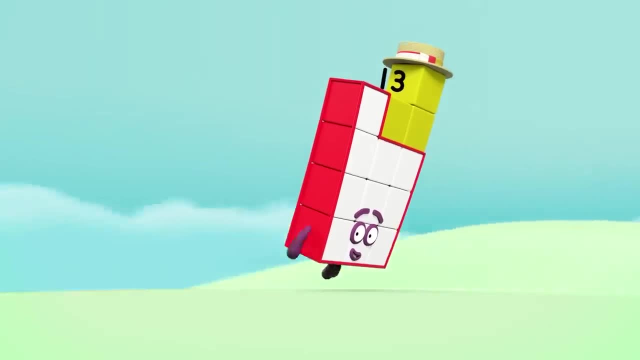 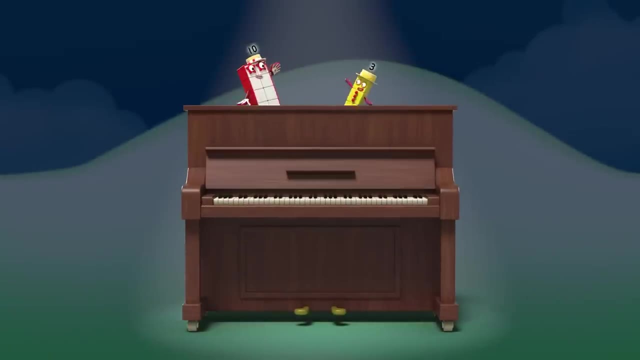 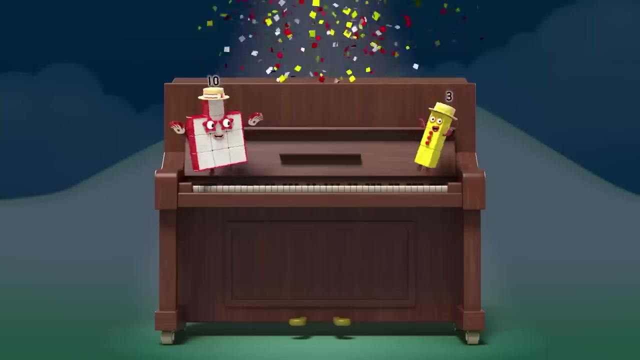 Whatever you call me, I'm still me. I'm the happiest number you've ever seen So lucky. I'm the happiest number you've ever seen To be unlucky. Number 13: Thirteen, Thirteen, Thirteen, Thirteen, Thirteen, Thirteen, Unlucky me. 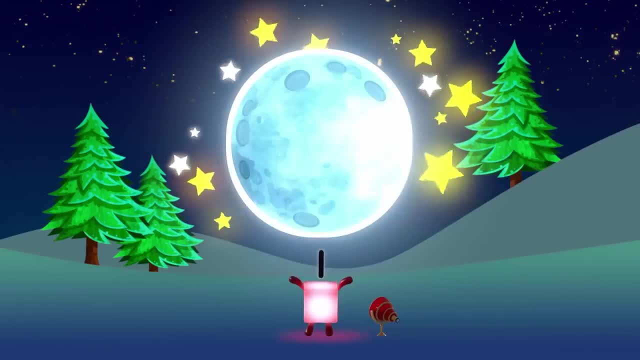 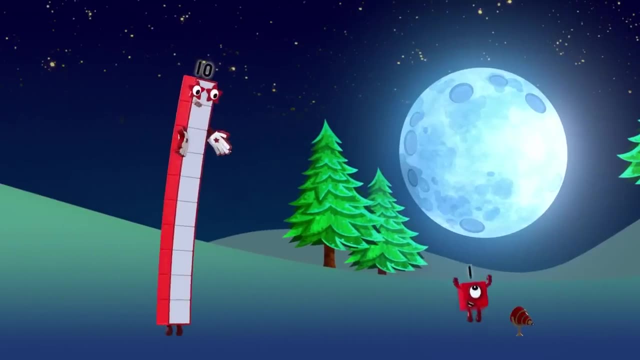 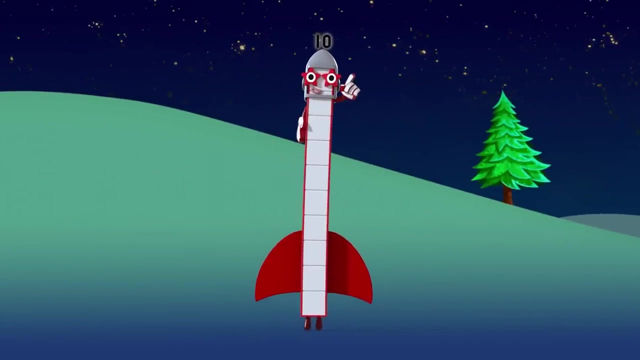 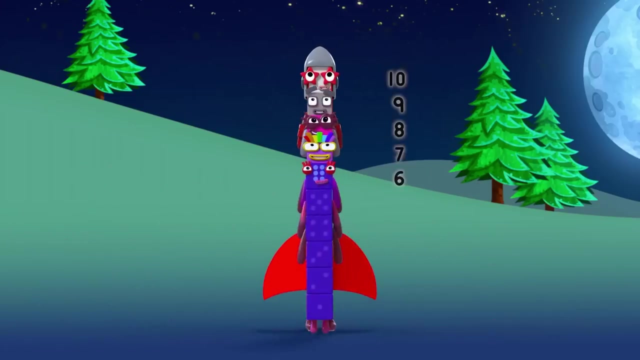 One, one marvelous moon. One day I'll go into space. Ha, You'll never get to the moon that way. one Just count down from ten to one. Ready, Oh, Ten, Nine, Eight, Seven, Six, Five, Four, Three, Two, One Blast off Huh. 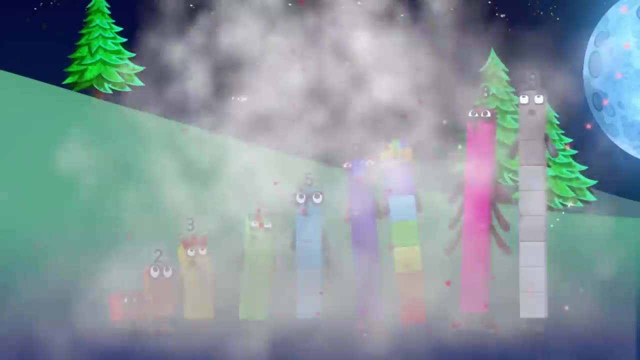 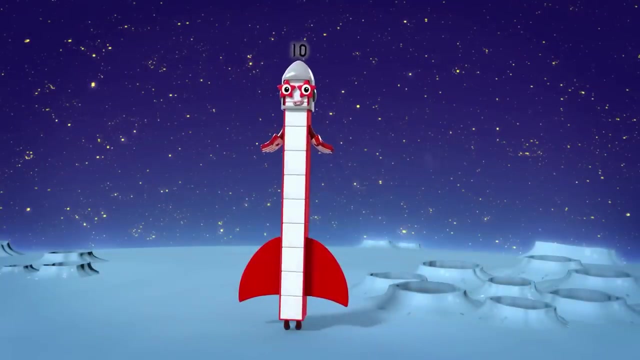 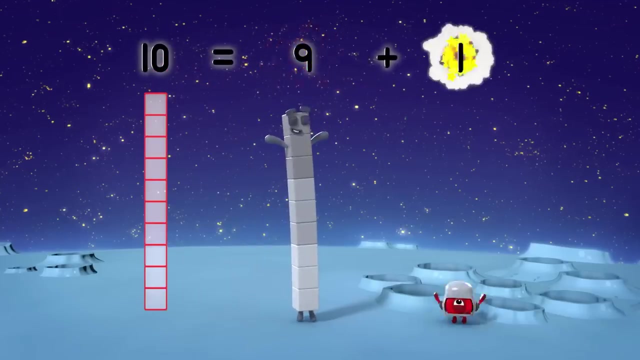 Four, Three, Two, One. Blast off Huh. Two, Three, Two, One And one Number ten up on the moon, And my friends will be here soon. Ten equals Nine Plus one. One small step for a number, One giant hop for number kind. 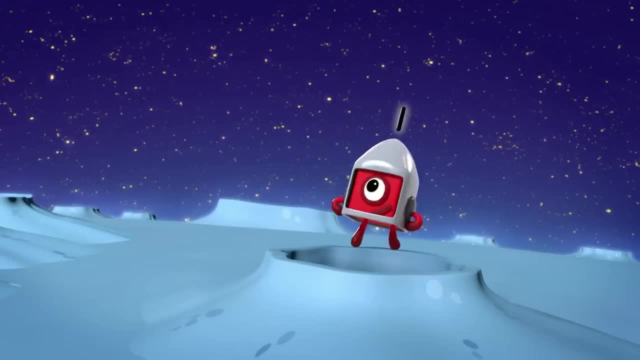 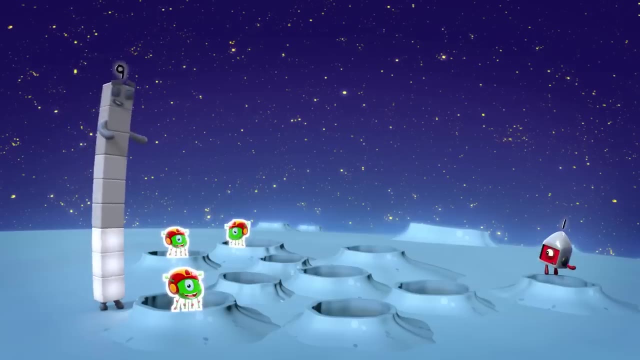 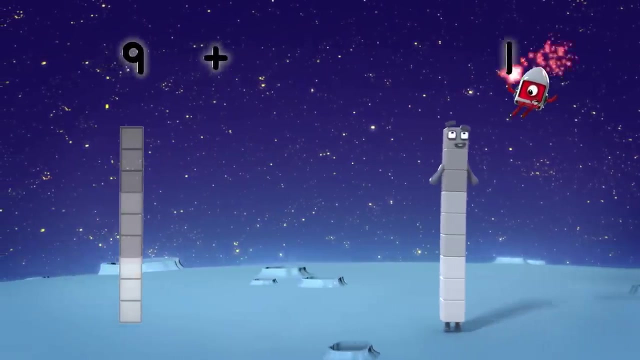 We're on the moon. Nine And one. That was easy, This is fun. One, Two, Three, Four, Five, Six, Seven, Eight, Seven, eight, nine, Nine aliens. One more is ten. Nine plus one equals ten. Number ten: back on the moon. 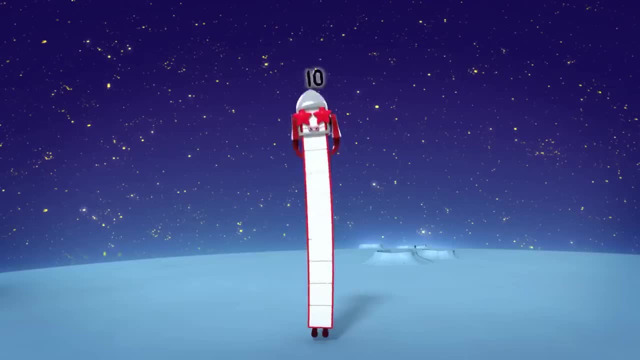 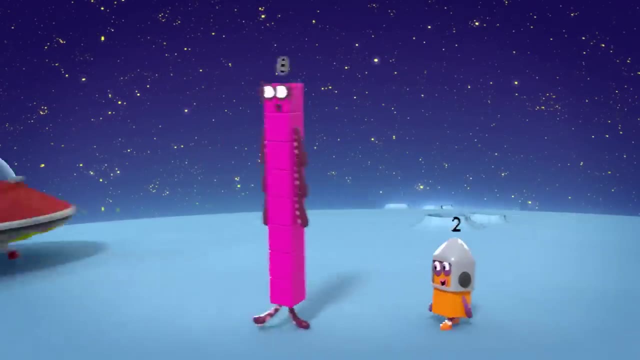 Two more friends will be here soon. Ten equals eight plus two. We're on the moon. Eight and two. How did we get here? Haven't a clue? One, two, three, four, five, six, seven, eight. 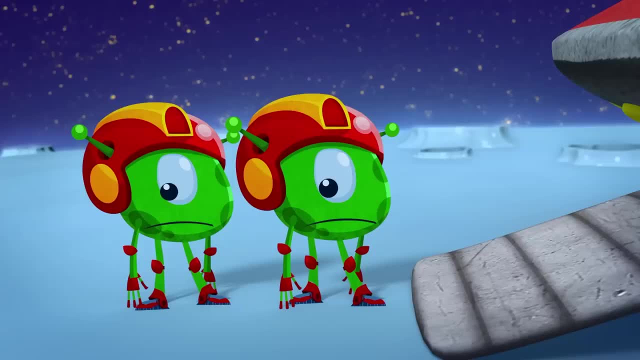 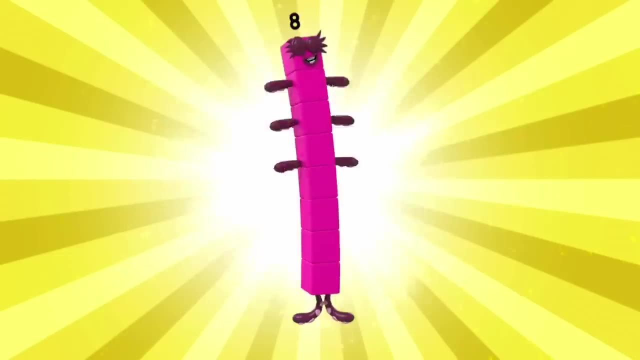 Eight aliens all heading home. Oh no, There's no room for those two, Never fear. Octoblock is here. Octoblock build One, two, three, four, five, six, seven, eight Build. 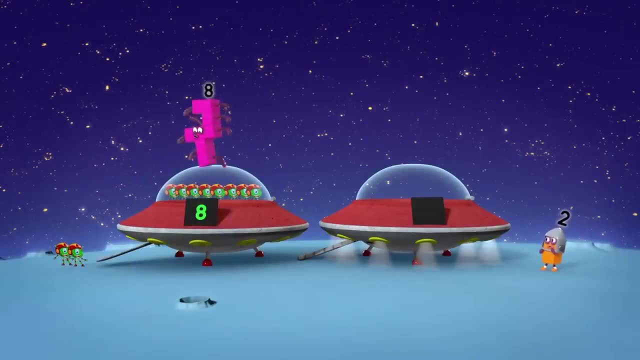 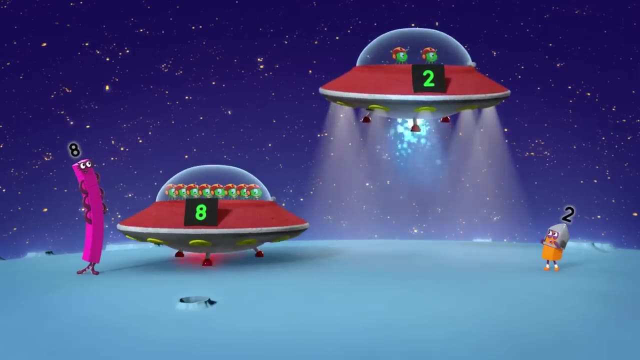 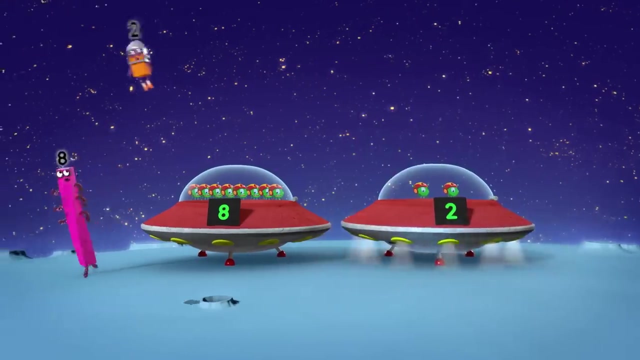 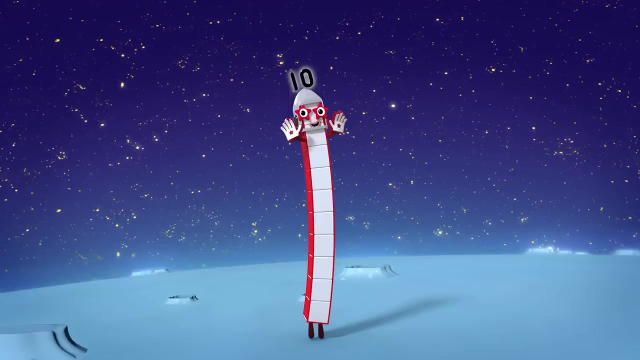 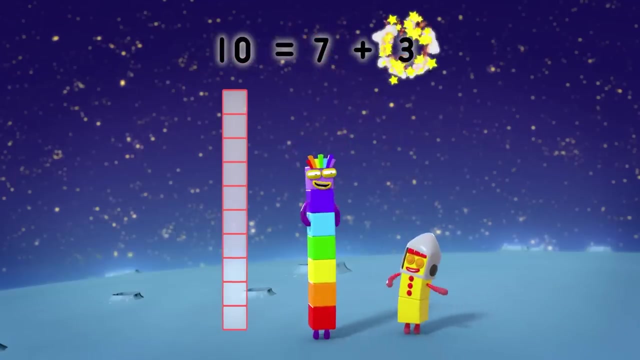 Build Two flying saucers. Good work, Oh, come back, It's not starting, Whoa. Eight plus two equals ten. Here I am. number ten. Time to make some friends again. Ten equals seven plus three. We're on the moon. 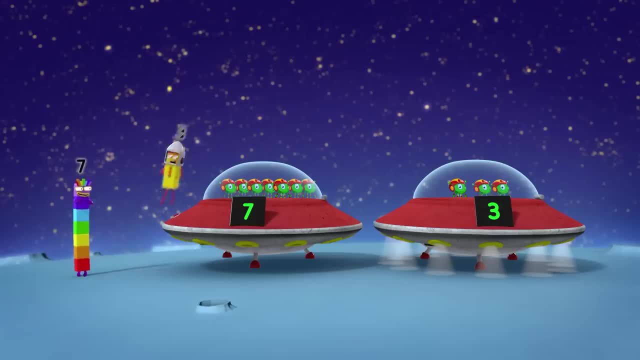 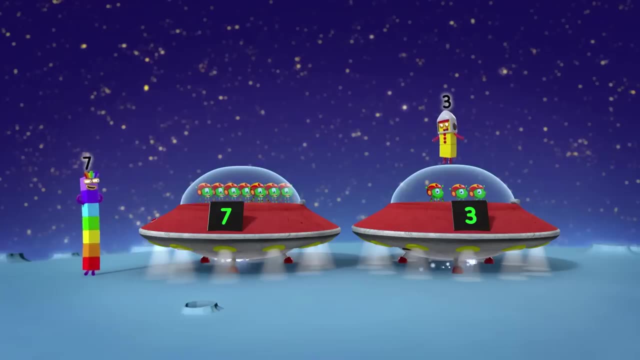 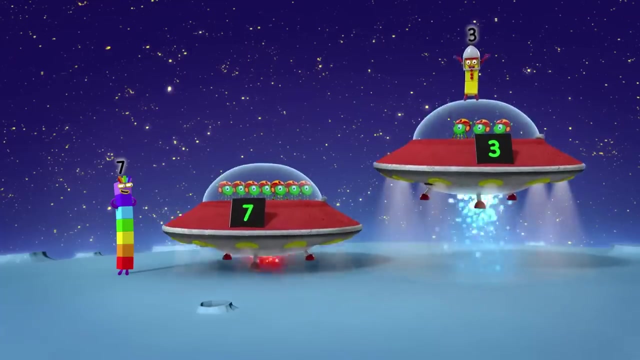 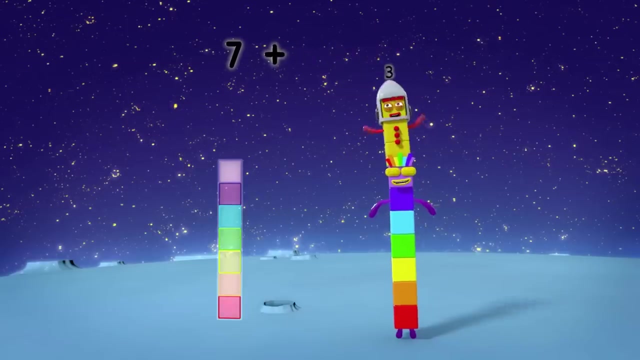 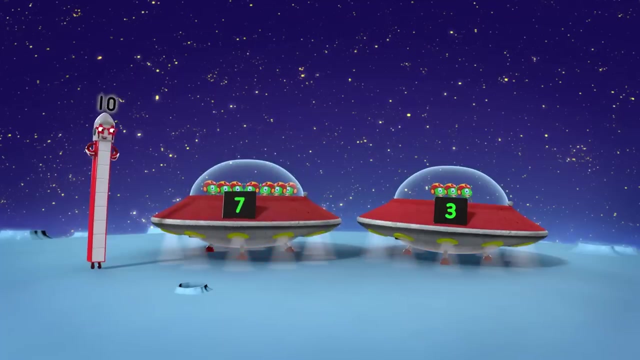 Seven and three. We're so lucky. Look at me, Look at that. There's the on button. That was lucky, Ready, steady, Blast off, It's too heavy. Seven plus three equals ten. It's ten again. Wait and see who my next two friends will be. 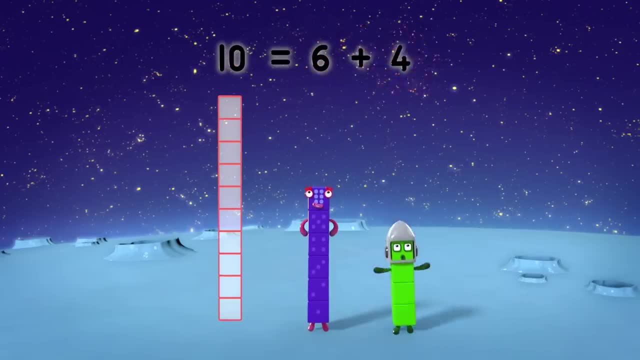 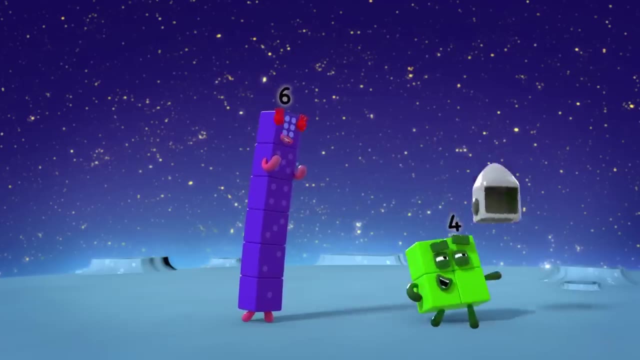 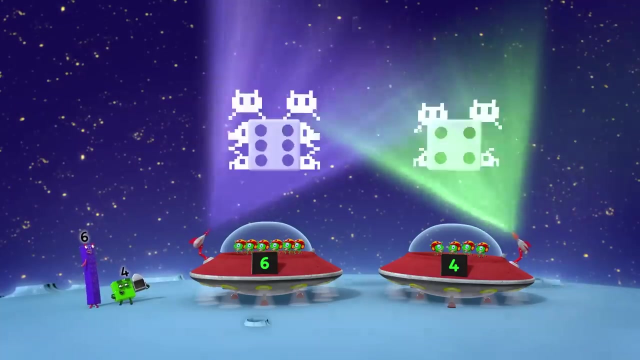 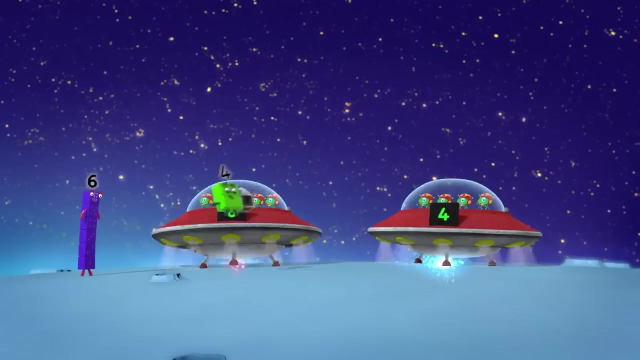 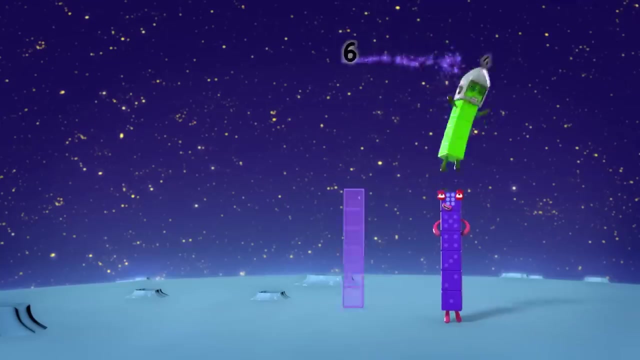 Ten equals six plus four. We're on the moon. Six and four. We really couldn't ask for more. Let's play a game: Roll the dice. and Oh, That was so cool, Still too heavy. Six plus four equals ten. 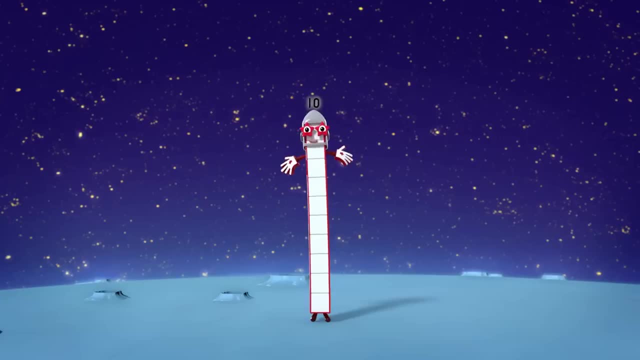 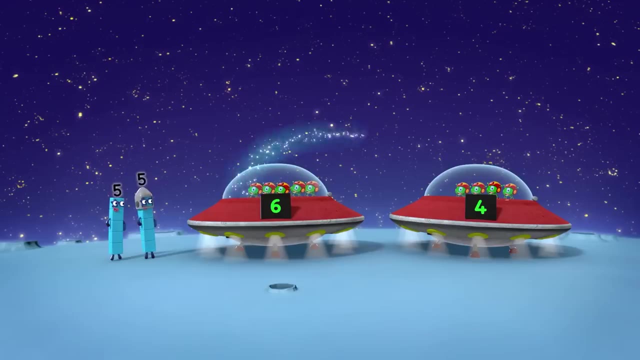 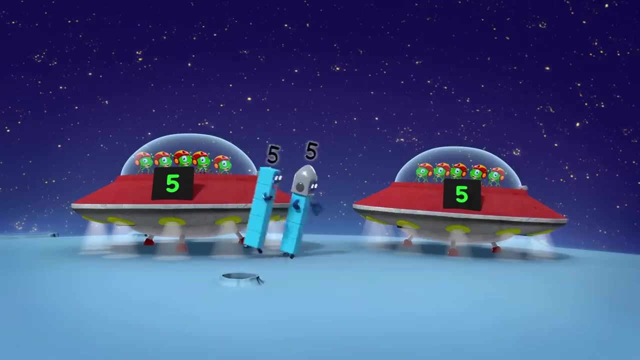 Quick before our visit ends. We've just got time for two more friends. Ten equals five plus five. We're on the moon. Five and five. It sure feels great to be alive. Let's give them a hand. High five, Come on. 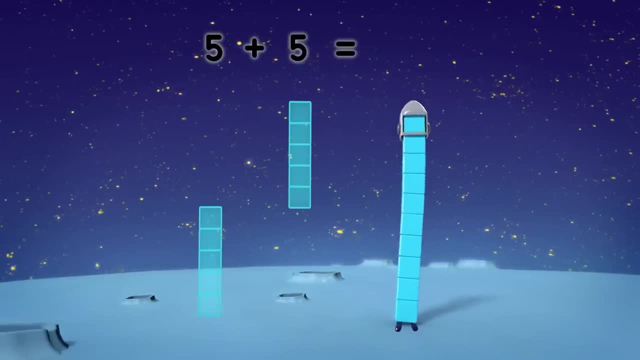 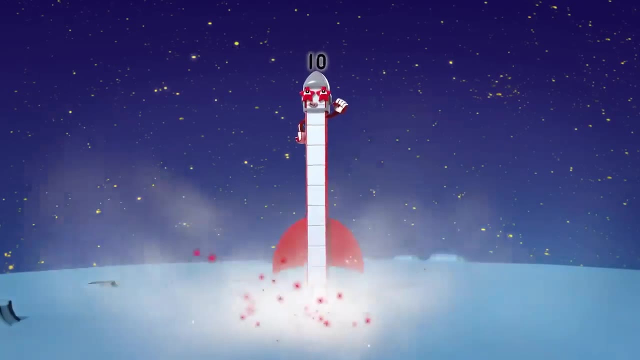 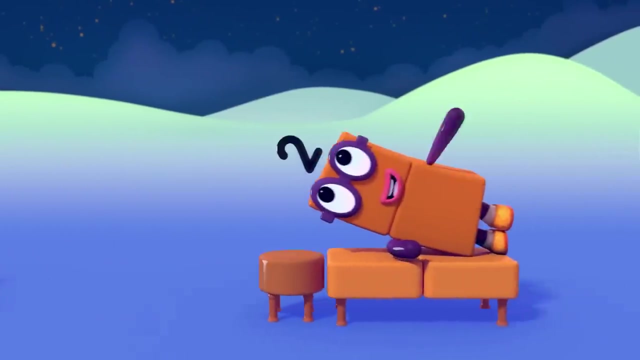 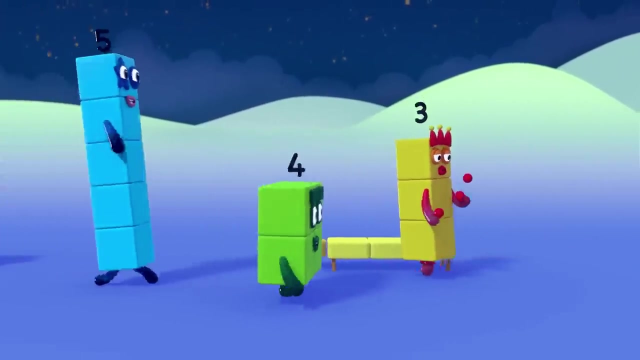 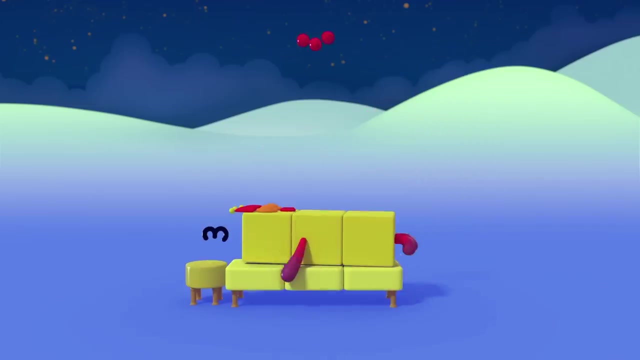 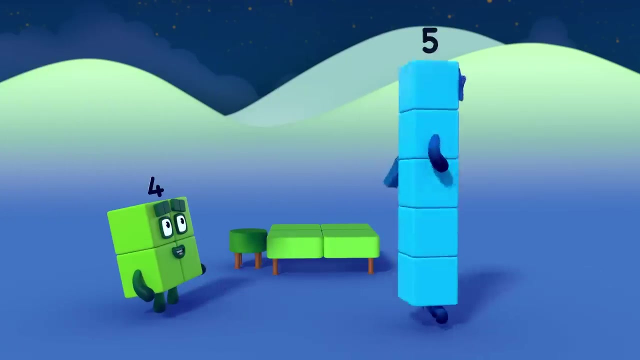 Five plus five equals ten. The number blocks from one to ten. went to the moon and home again. Night night. It's time for bed Boar, But I'm not tired. Stay up, Go to bed, Make up your own mind. 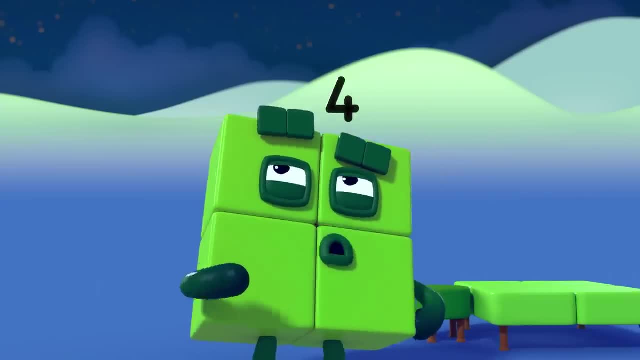 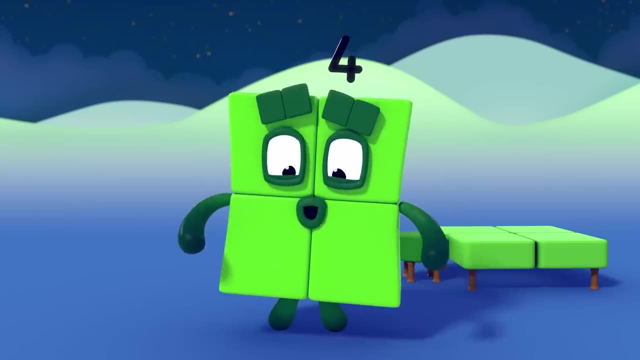 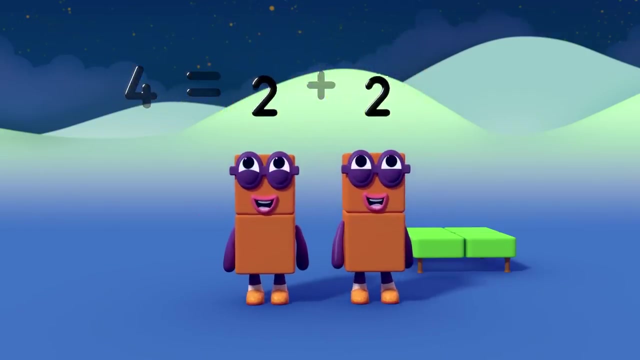 Stay up or sleep. Stay up or sleep. I can't do both. He can, No, no, no, no, Not you two. Four equals two plus two. Ha ha, ha, ha, ha ha. You look like me. 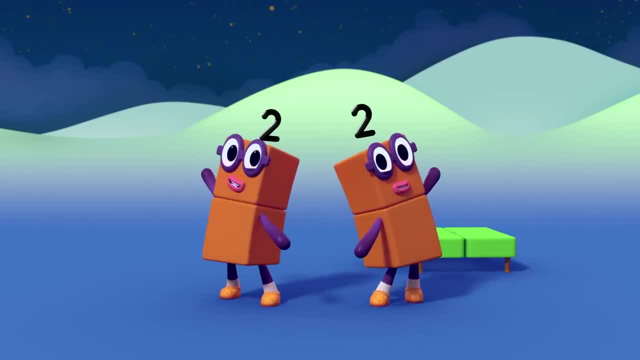 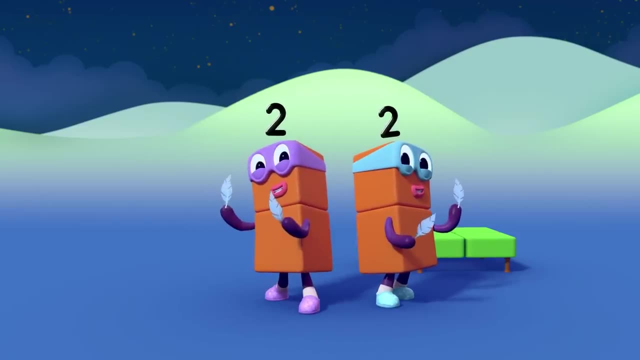 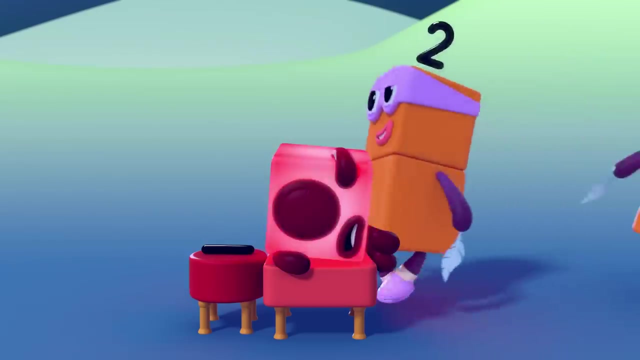 I look like you. We're two of a kind, We're the Terrible. Twos, Yeah, Two. lots of two feathers. It's tickling time, Hooray. One, two, one, two, Tickle, tickle. 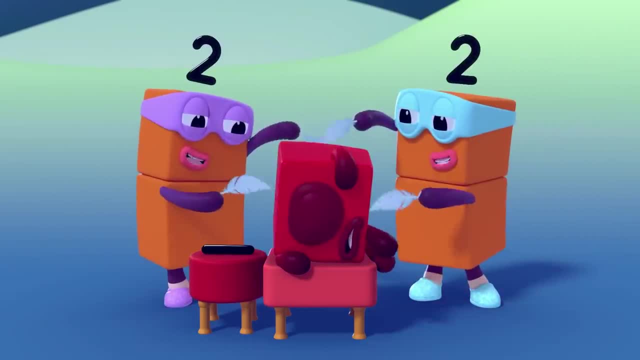 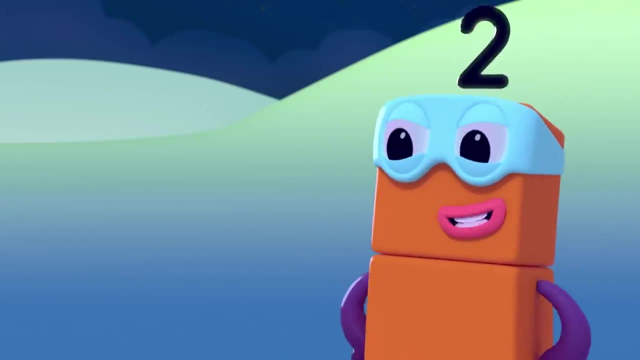 Tickle, tickle, Oh, is someone there, Not someone, Some twos, And we're both here to say boom, That was fun, Let's do it again. Yeah, Oh, oh, Oh, oh, Oh oh. 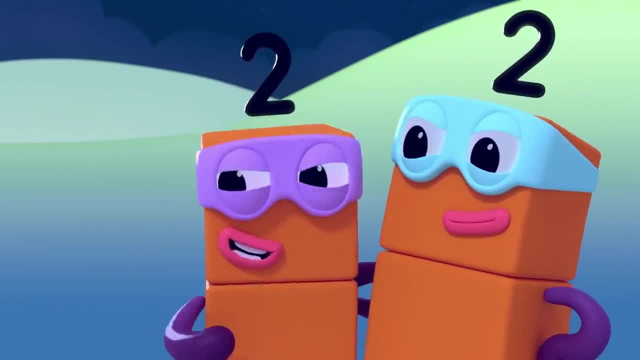 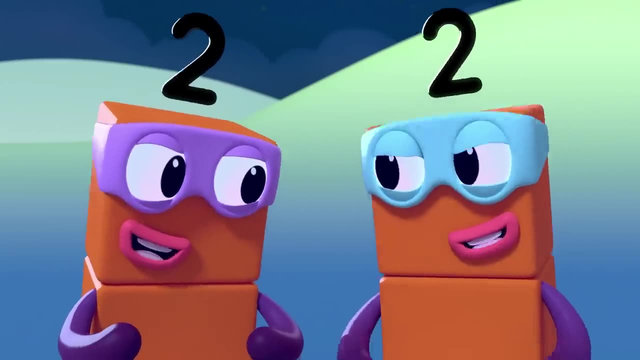 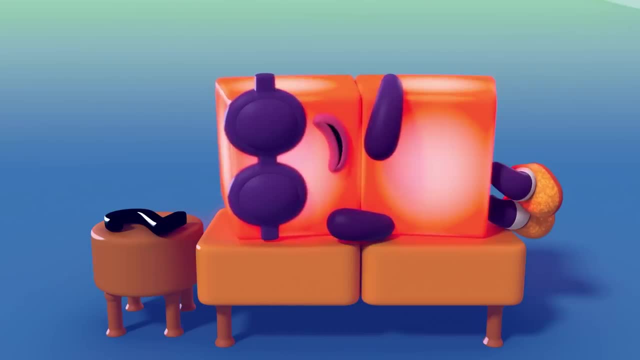 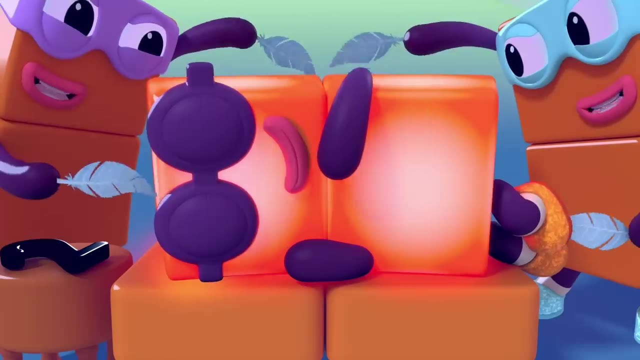 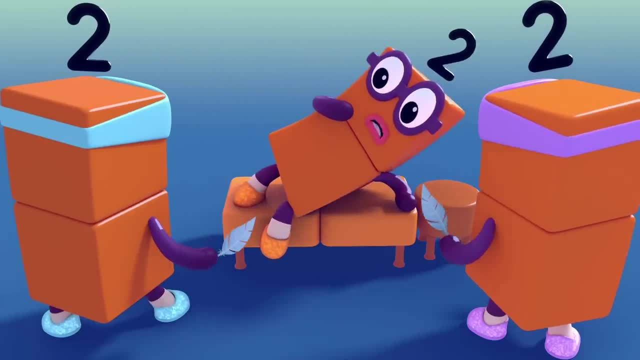 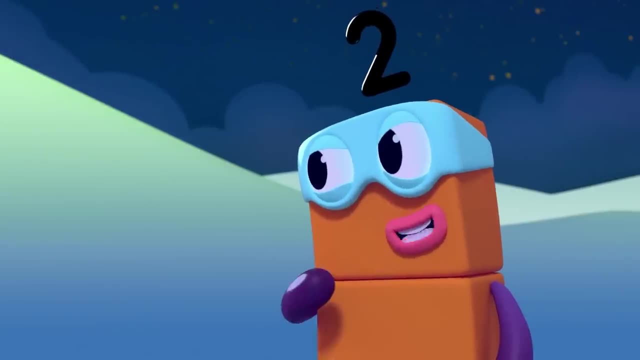 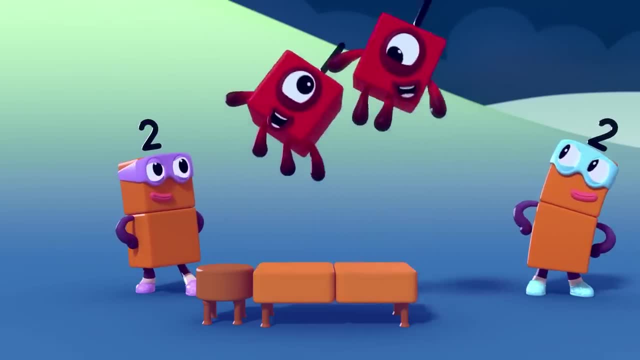 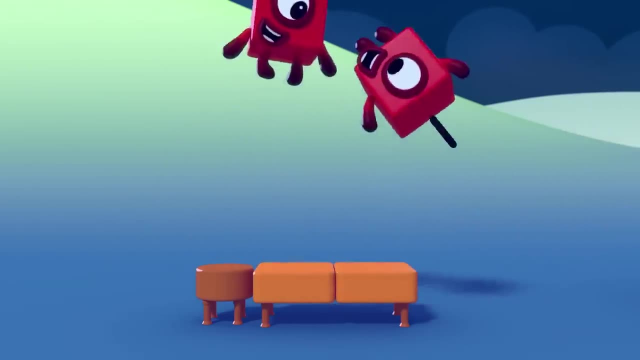 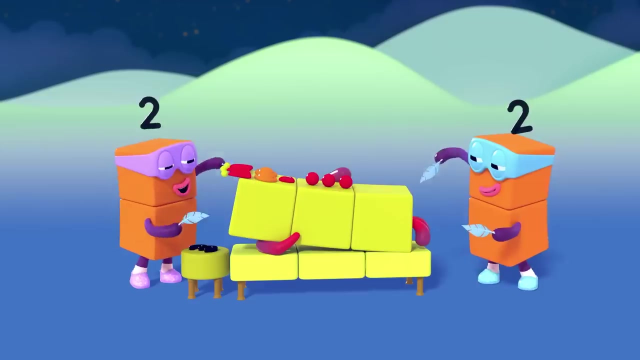 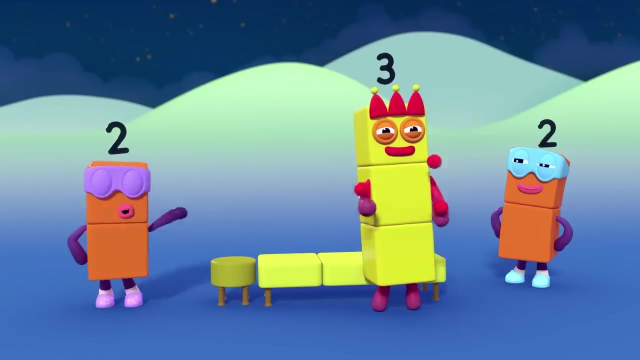 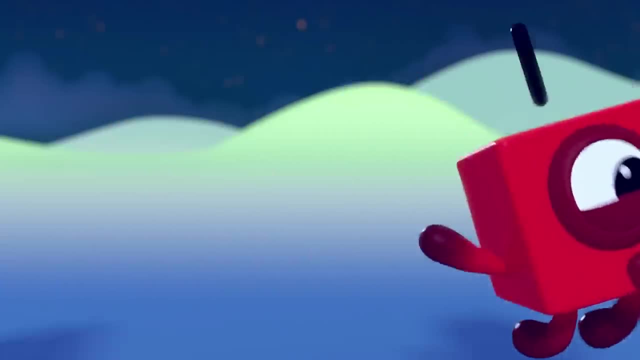 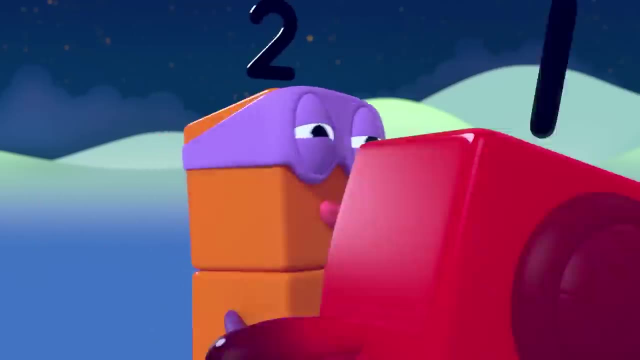 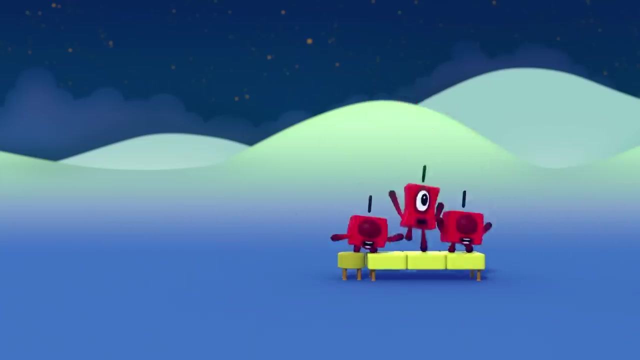 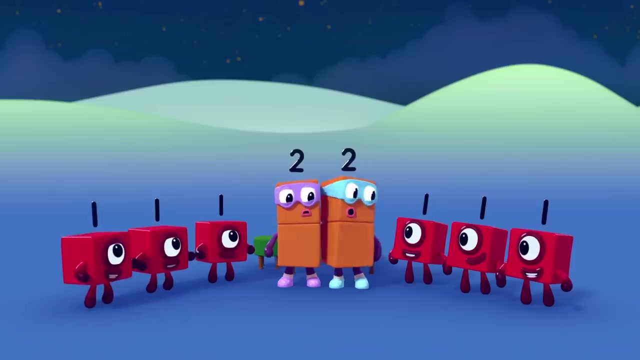 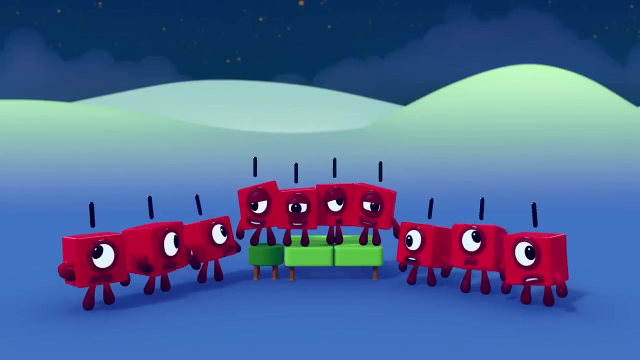 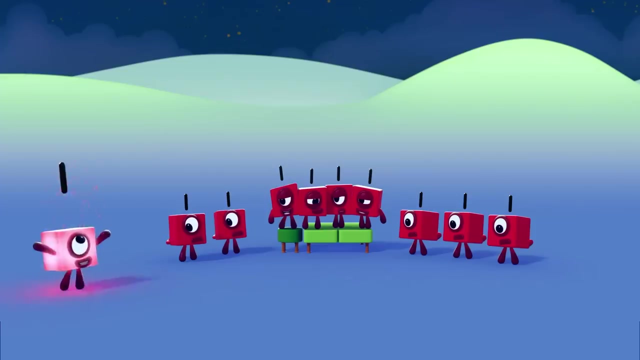 Ah You, Hey, Stop A terrible Tuesday Toodle-oo. We've only one thing to say: Boom, Everyone, pull yourselves together. One one block. One plus one equals two. Two is two ones. One plus one plus one equals three. 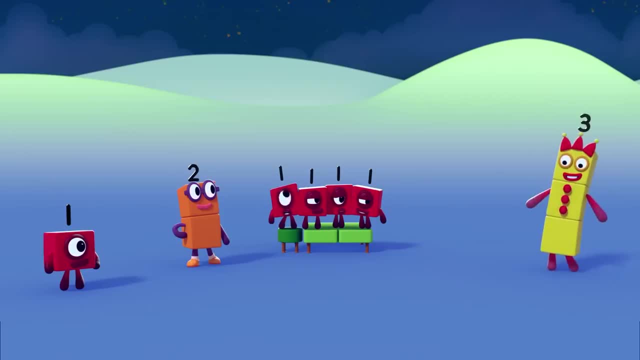 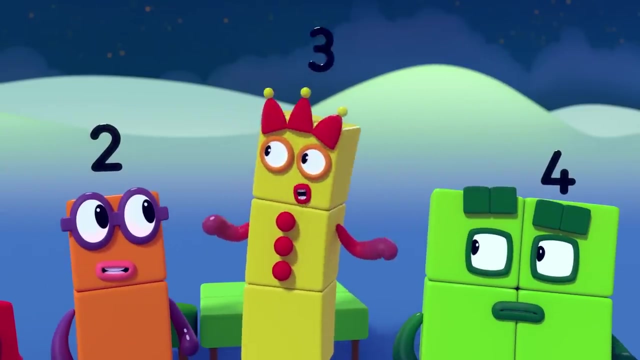 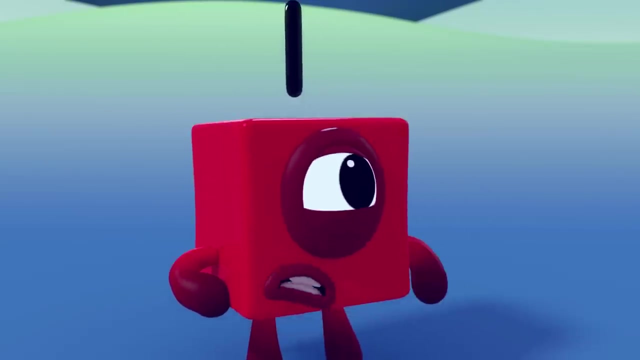 Three is three ones. One plus one plus one. Three plus one equals Four. Four is four ones. Where are they? Where did those terrible twos go? Don't look at me. What's all of the noise? The terrible twos are playing tricks on us. 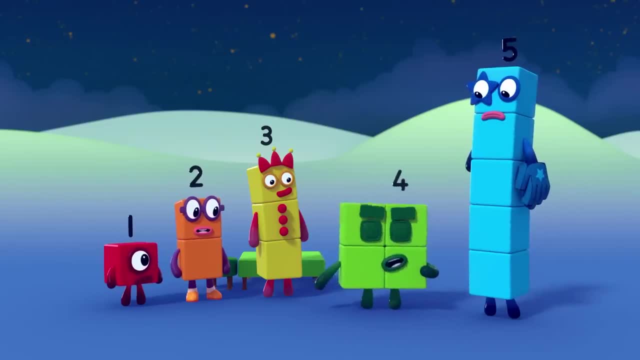 And where are they now? I have to be square with you. They made me. What did they make you? You can tell us four. No, They made me. No, They made me. Well, I made them. Then they made me. 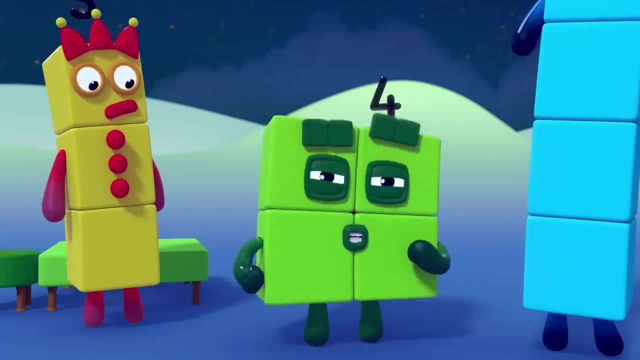 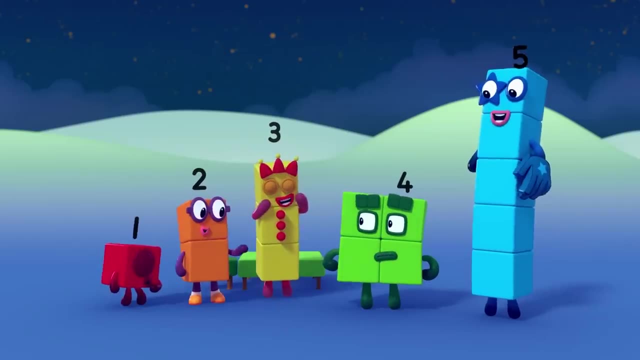 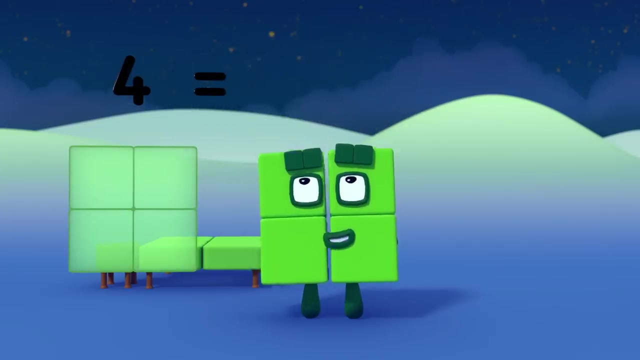 Huh, I'm the terrible twos. I'm four lots of one, But I'm also two lots of two. You're so funny, Don't be silly. That's a very funny joke. Four equals two plus twos. The terrible twos. 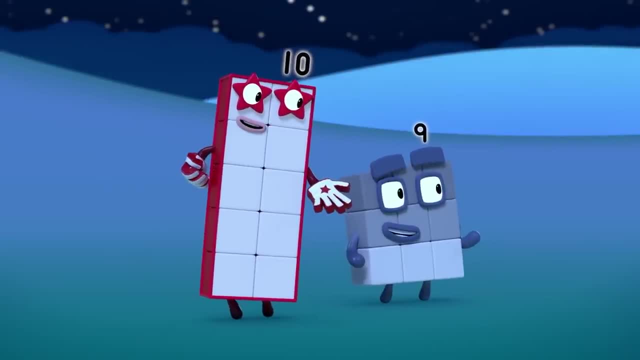 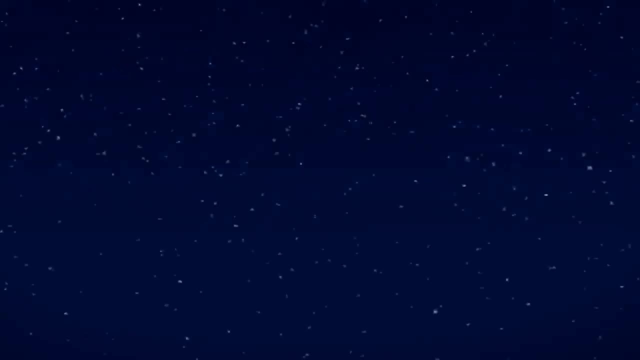 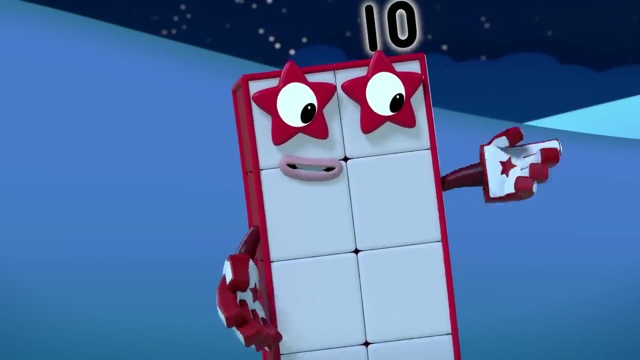 Shh. Now there's something you don't see every day: An alien Up Up. Ah, Whoa Is that where you live? Up, up, Up up. Don't worry, fellow space cadet, I can rocket you home. 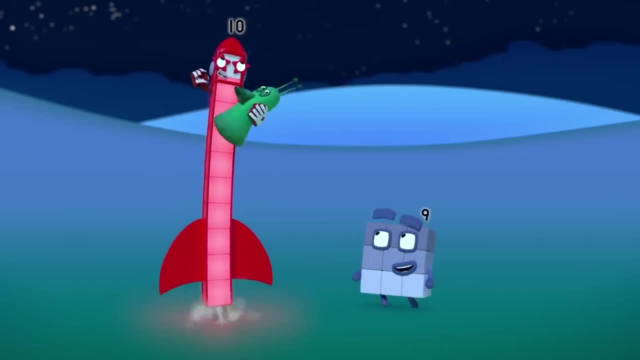 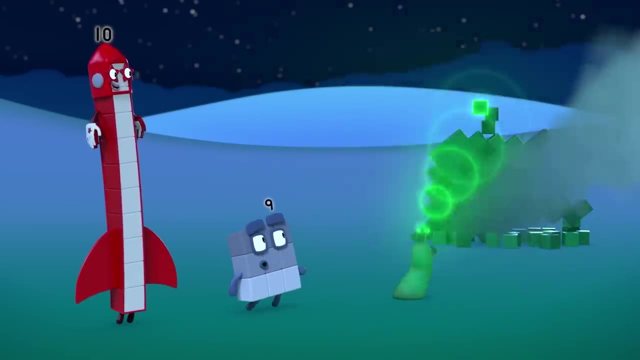 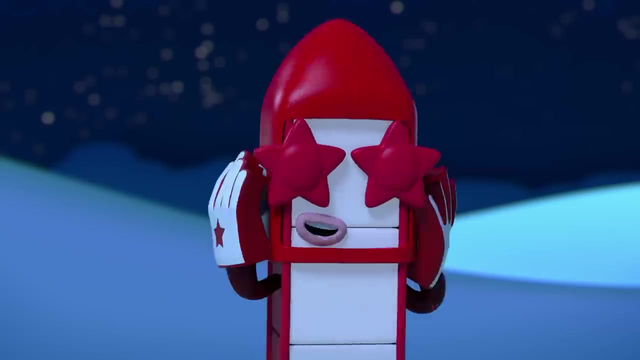 Hold on tight. Ten, nine, eight, Oh, Ah, Uh-oh, Uh-oh, Uh-oh. I think she's building a tower. Hmm, Up, Oh, Um. I think you'll need more blocks than that. 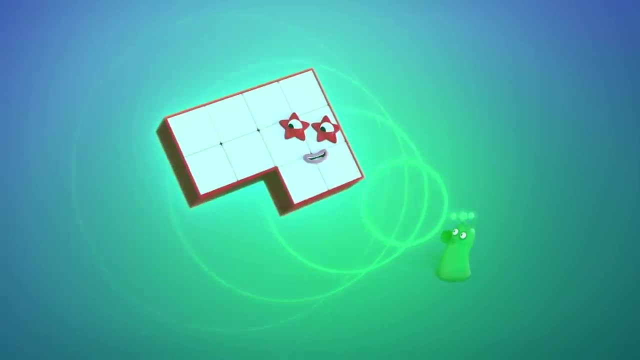 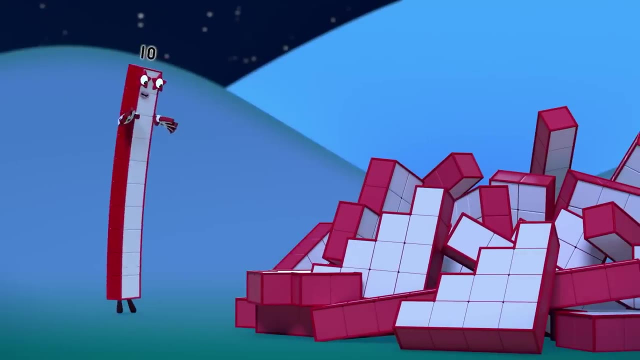 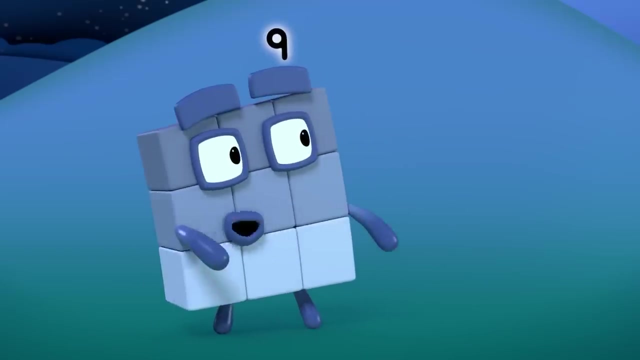 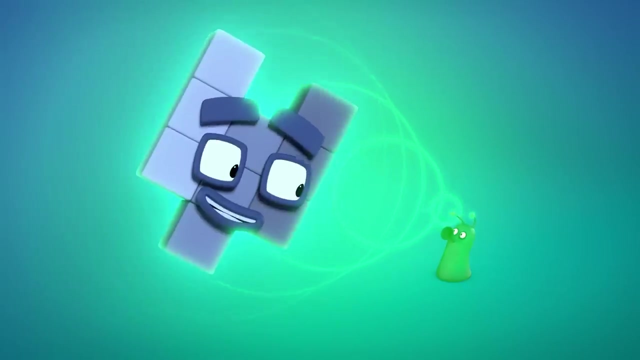 Whoa, Stop That tickles. Oh, Ha-ha-ha, Let's build a tower, My turn. That looks like fun. Oh, that looks fun. Oh, Oh, Ha-ha, Ha-ha-ha. 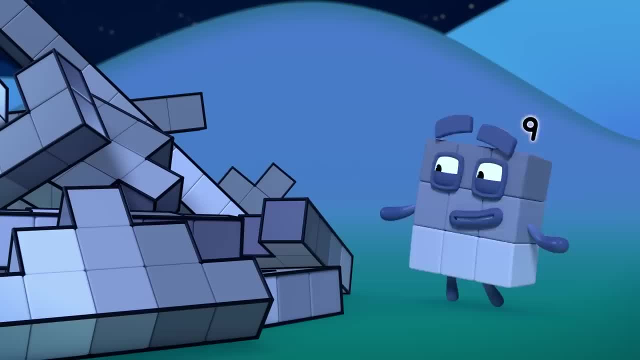 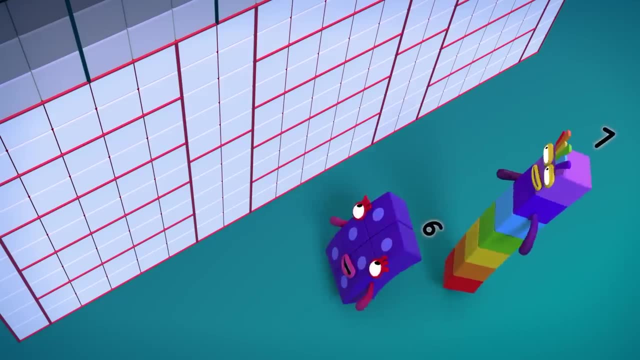 Oh, Oh, Oh, Ha-ha, Ha-ha, Oh, Ha-ha, Ha-ha, Ha-ha, Ha-ha, Ha-ha-ha, Ha-ha, Ha-ha-ha, Ha-ha. 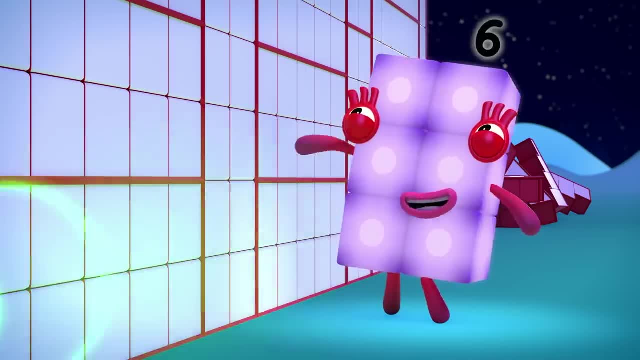 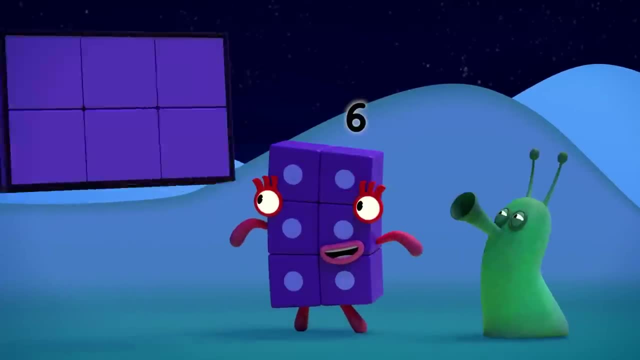 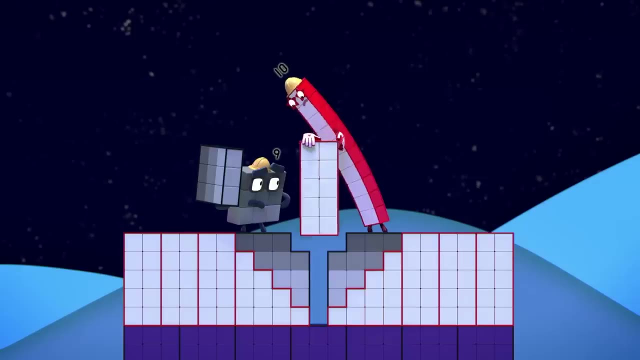 Ha-ha-ha, Oh, I didn't even know I could make that shape. Hey Say: Can I play? Oh, lucky me Woo. This doesn't fit, Or this Or that. Try this Yay. 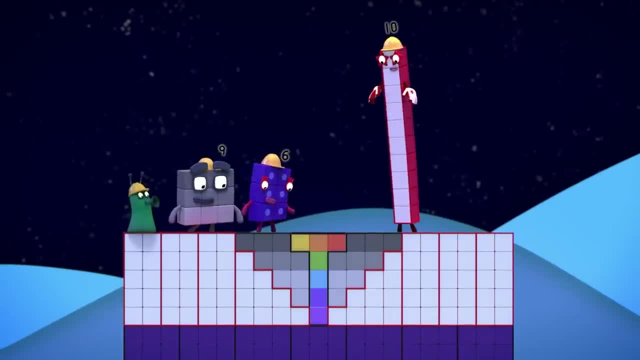 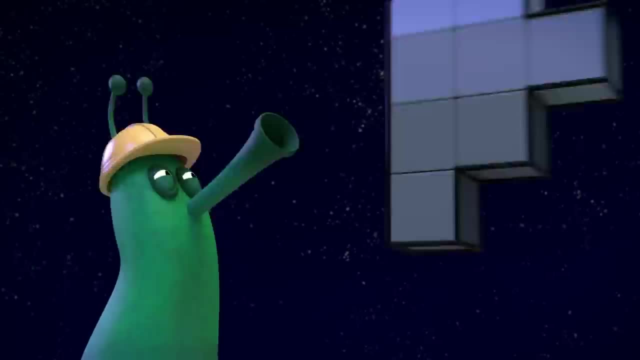 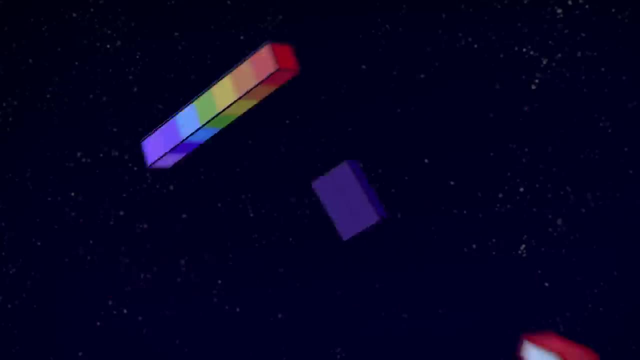 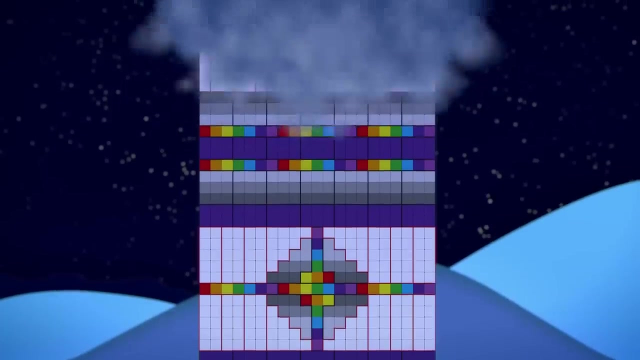 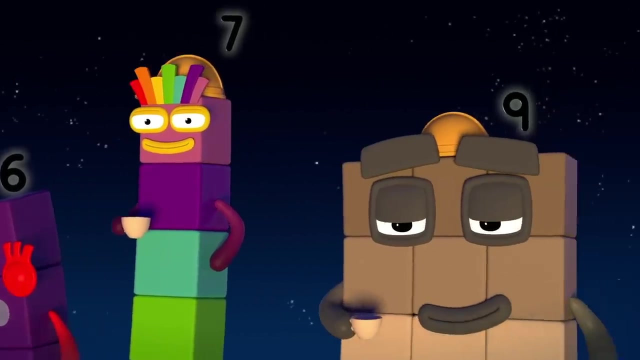 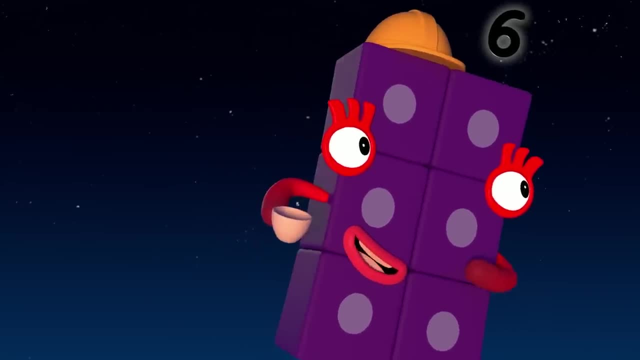 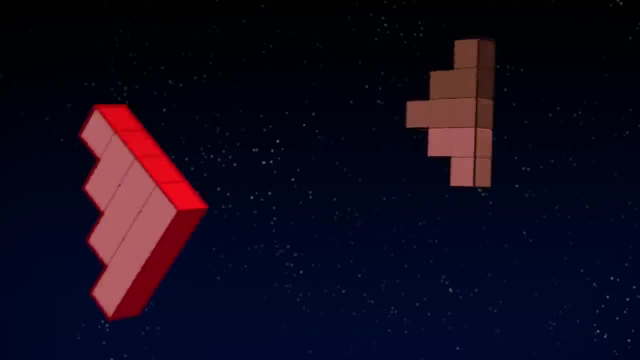 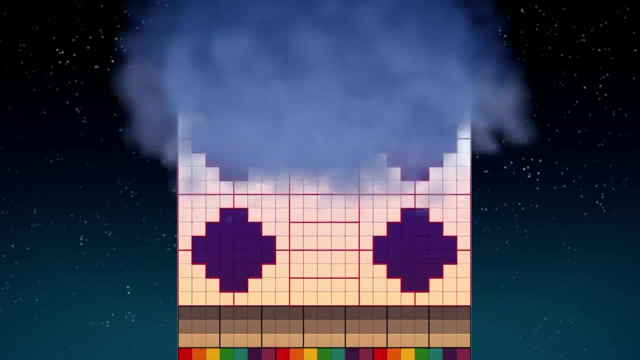 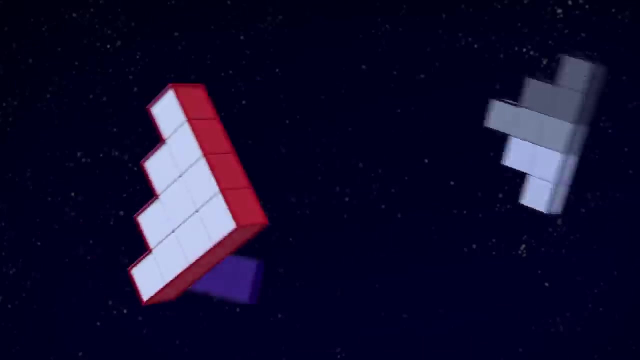 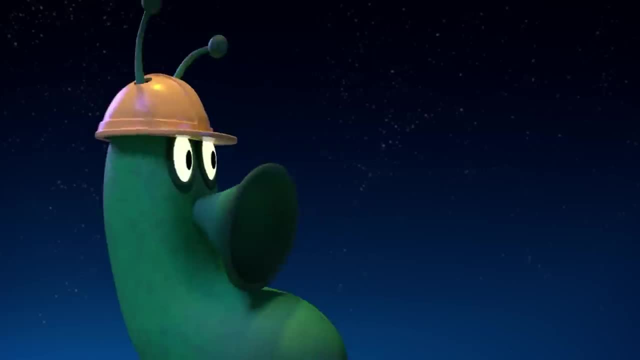 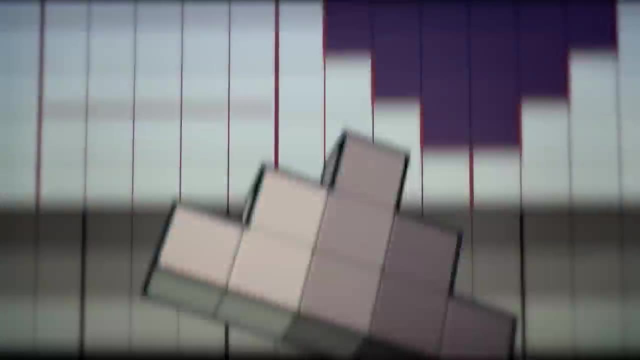 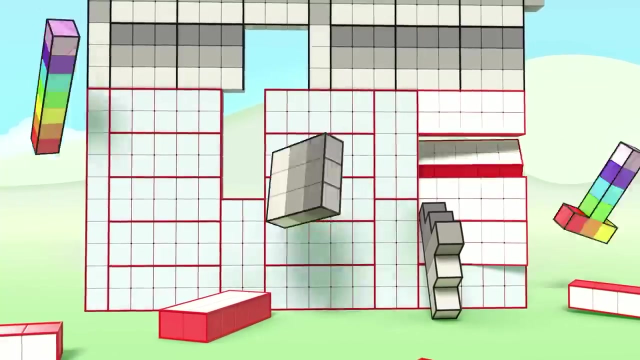 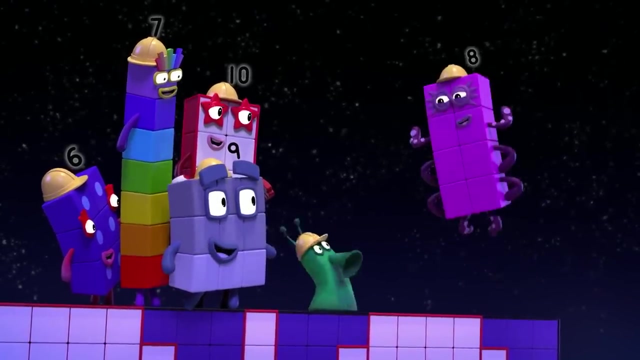 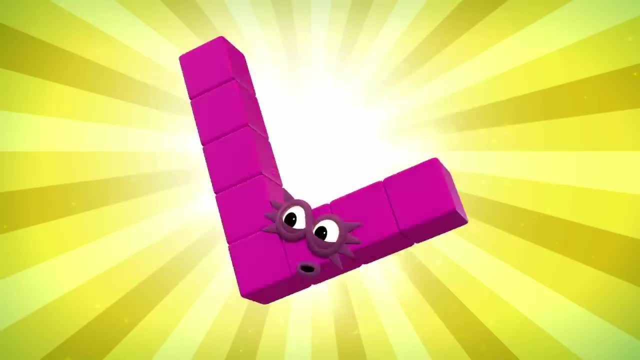 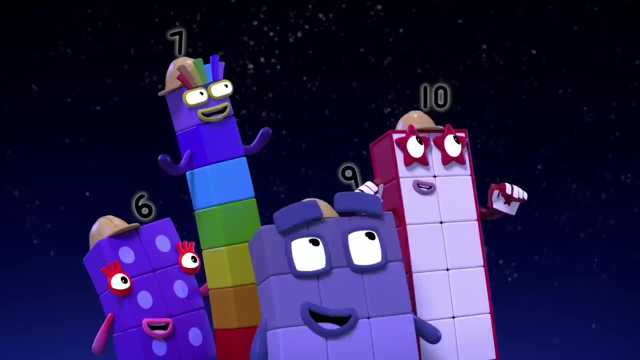 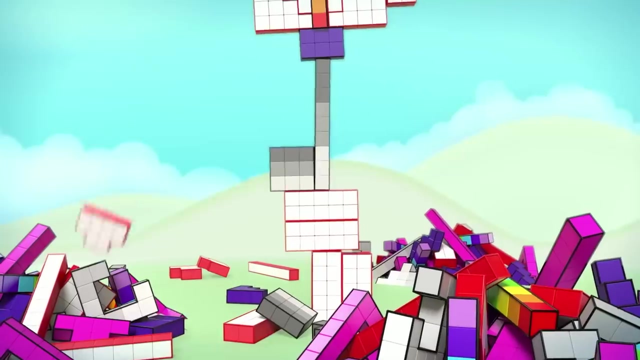 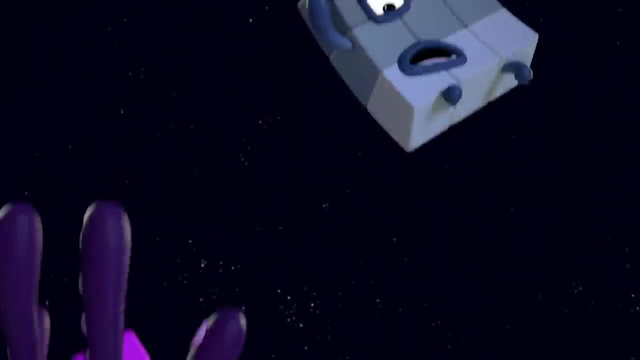 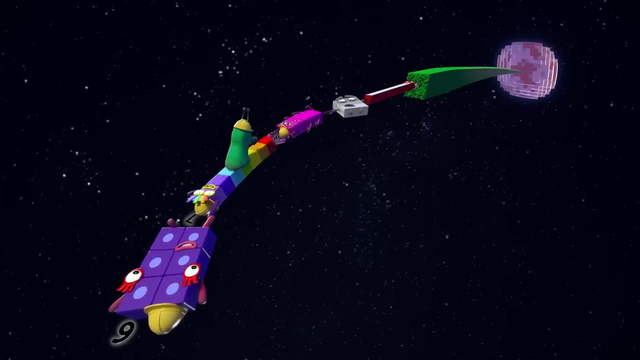 Oh, Oh Oh. Did somebody say help Octoblock to the rescue? Oh Oh, Octoblock built One, two, three, four, five, six, seven, eight Timber. Whoa, You go up, we'll go down. 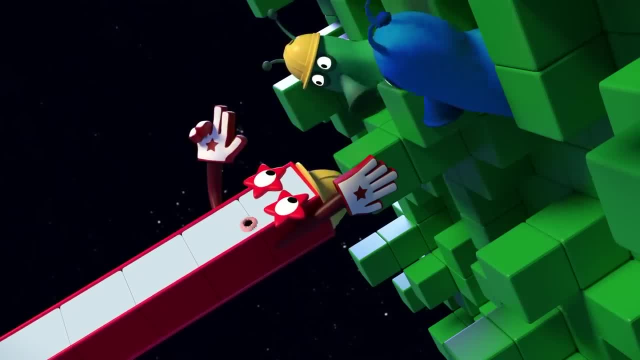 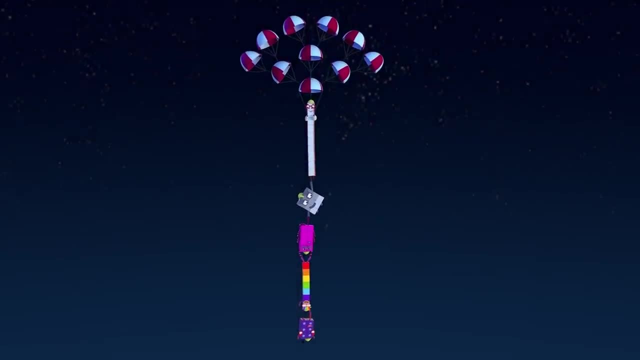 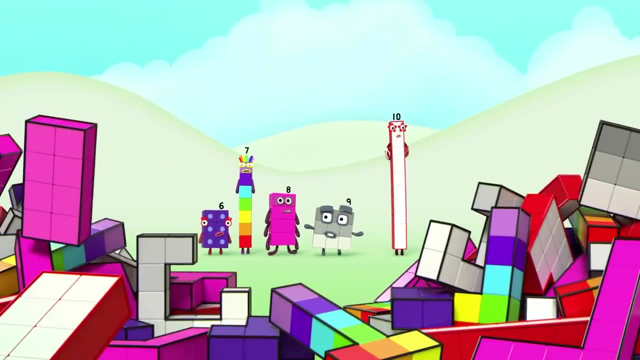 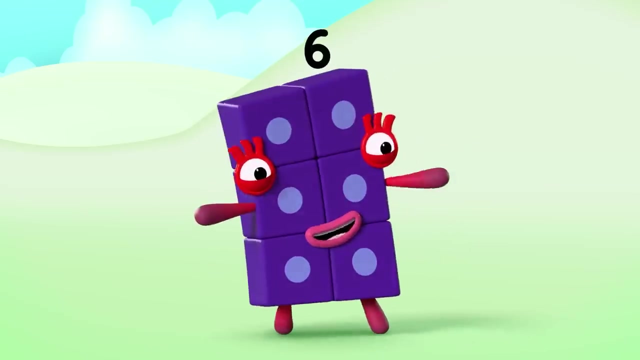 Goodbye, fellow space cadet. Yay, Well done crew. A successful mission, Well, mostly successful. We helped our friend get back to space, but now our tower's all over the place. That's lucky We get to build something else. 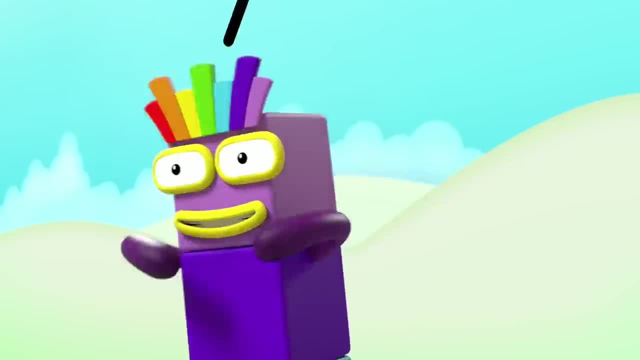 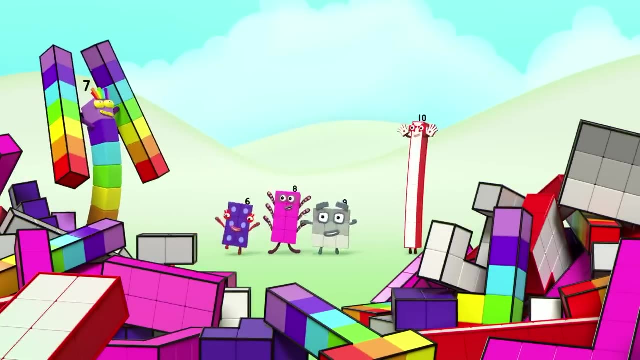 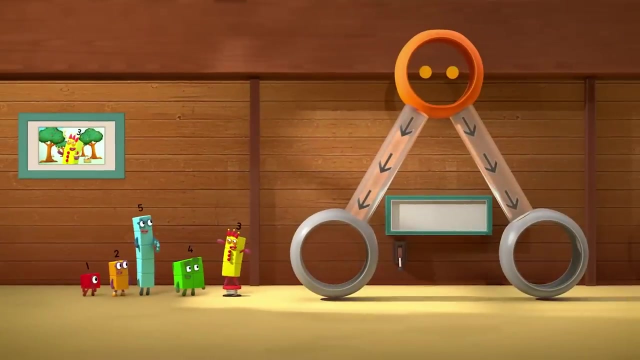 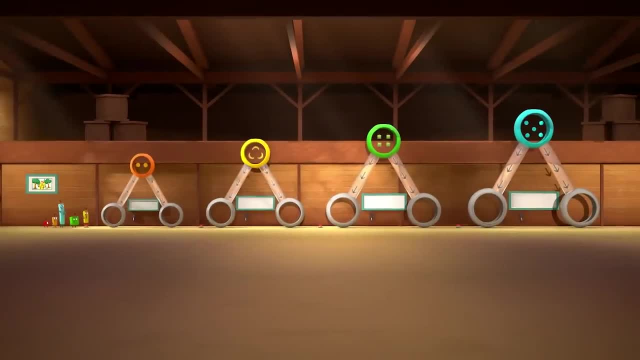 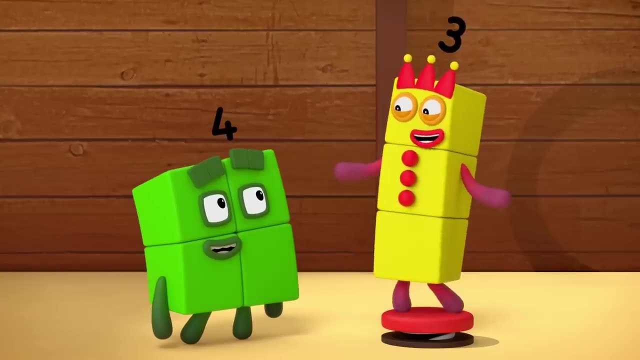 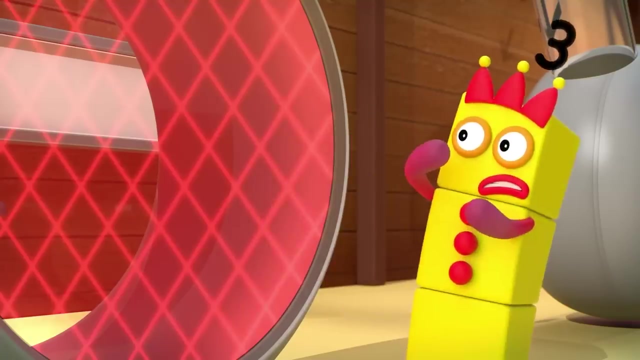 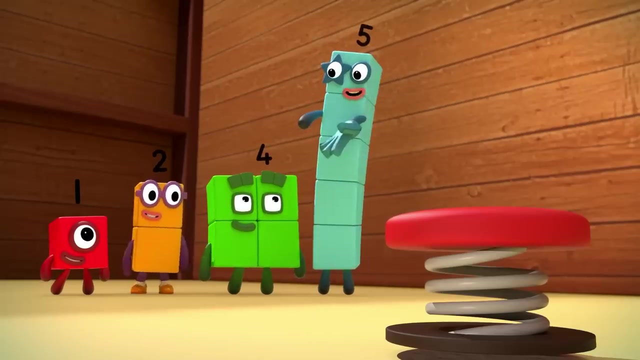 where we serve up fresh fruit all day. Wow, How do they work? Oh, easy peasy: lemon squeezy, Obviously I just Silly thing's broken. There are two oranges in there. Maybe if two tries it. 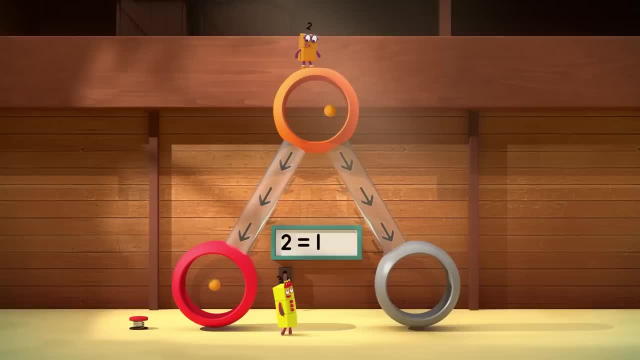 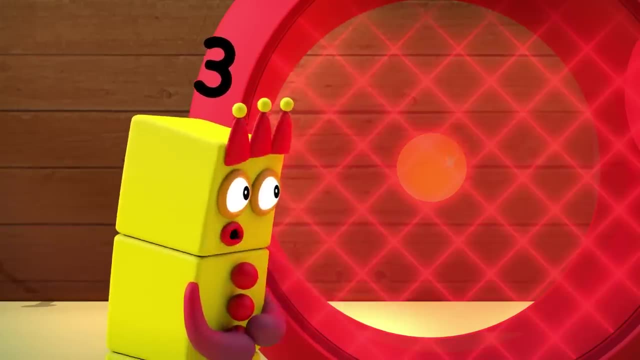 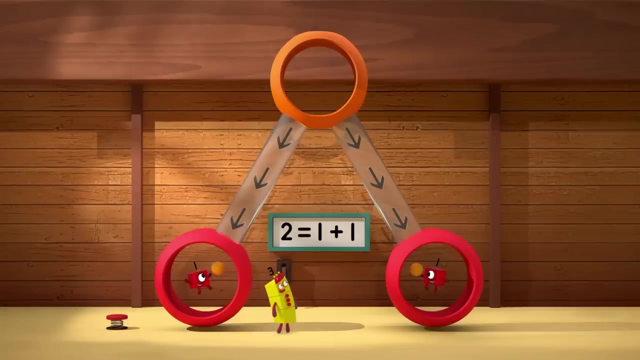 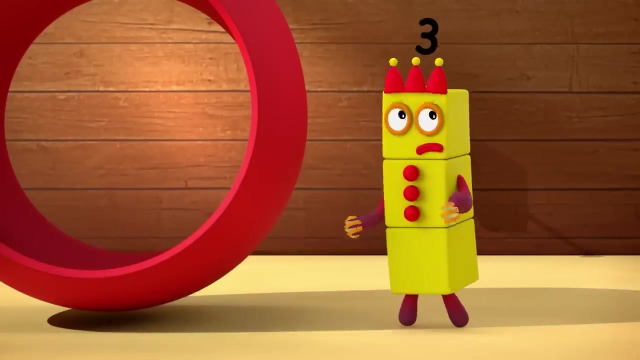 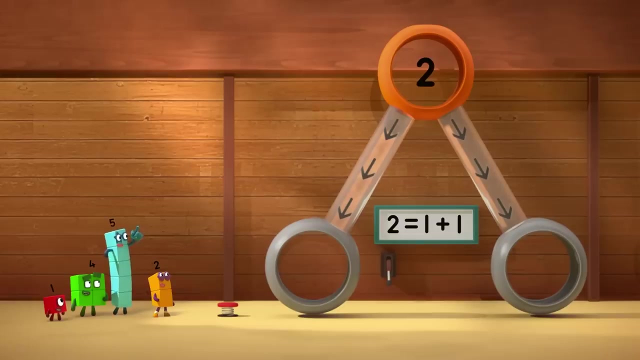 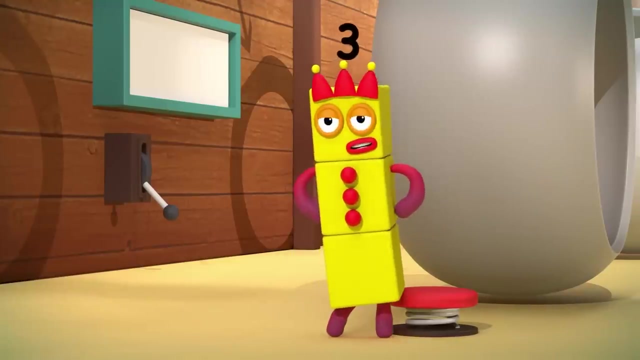 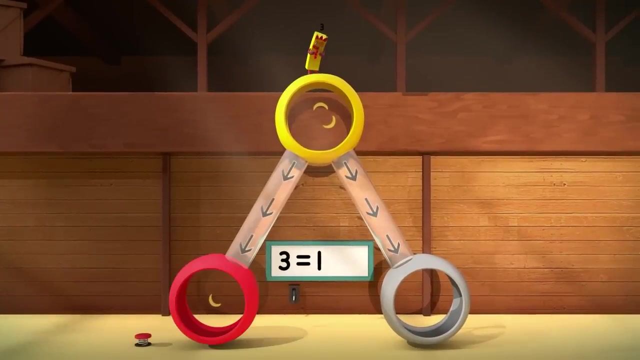 Two equals one plus one. How do I? Two equals one plus one, Yum Ta-da, Look. Two at the top splits into one and one at the bottom. I want fruit. It's my turn. Three equals one plus two. 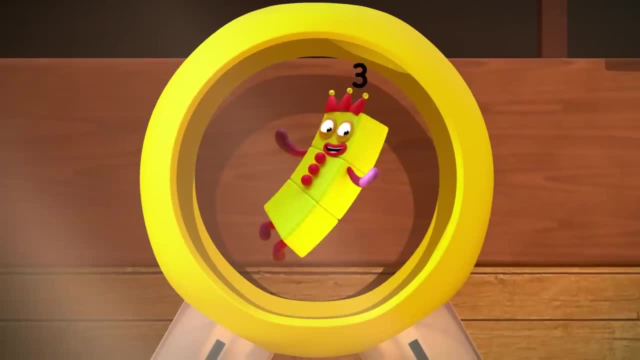 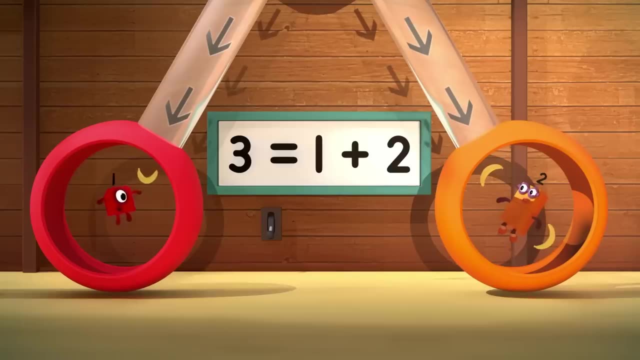 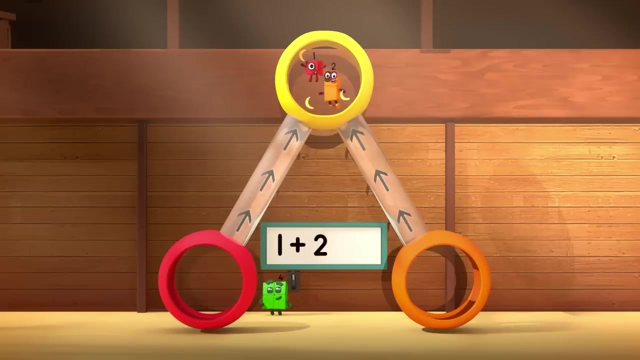 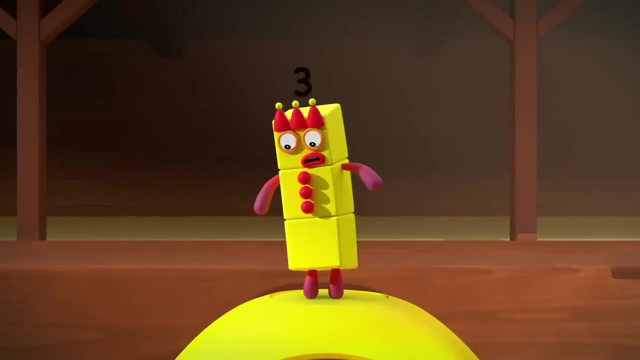 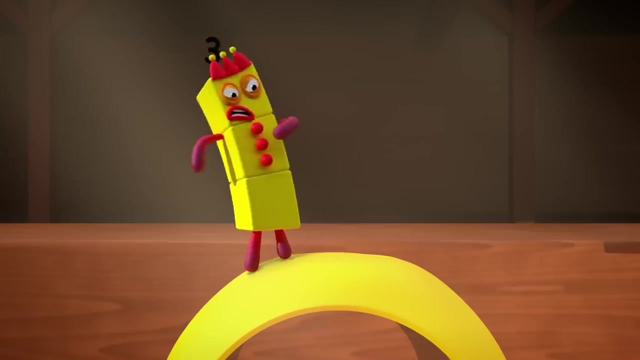 Yum, Yummy, yummy, yummy. Three equals one plus two. Oh, Where's three? Let's try this lever: One plus two equals three. Oh, it works both ways. Oh, Hey, Hey, Those are mine. 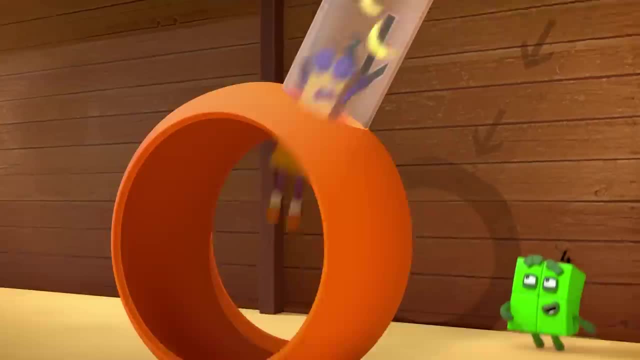 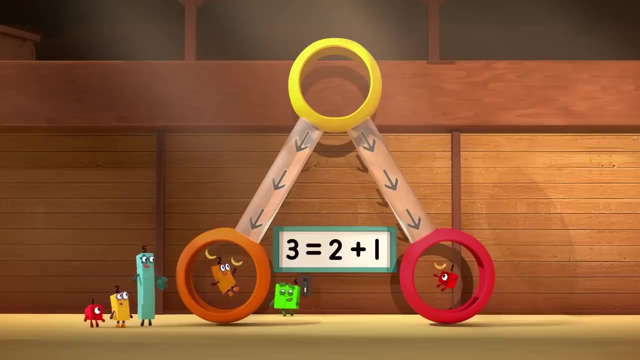 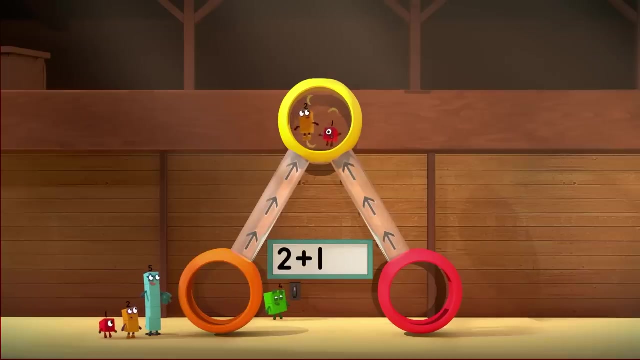 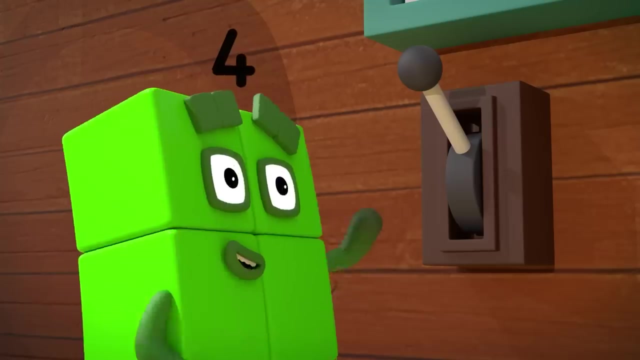 Three equals two plus one. Now there's two over here and one over there, But three doesn't get her bananas again. Two plus one equals three. Hey, I'm still hungry. Oh, Mmm, Look Apples Square. 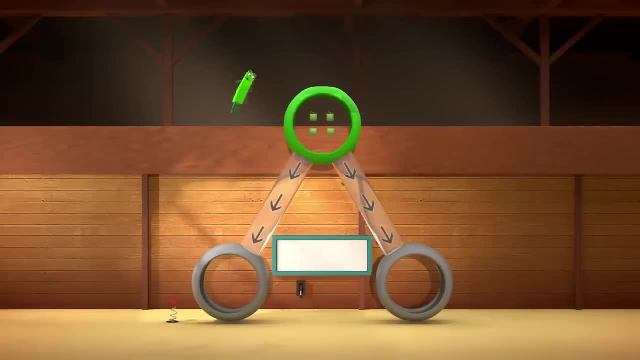 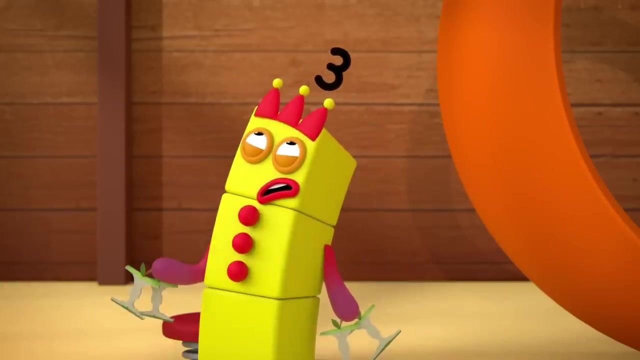 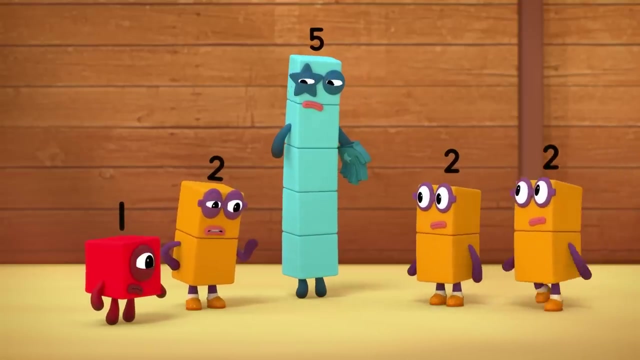 Apples. Apples Four equals two plus two. Yum yum, Yum yum. No, no, no, you silly machines, Poor three. We need to find a way to make three apples come out. Look, Four new apples. 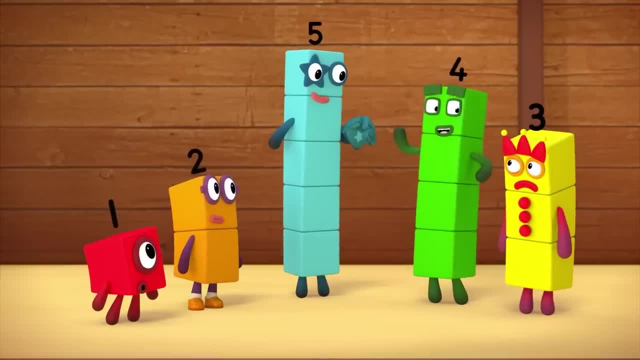 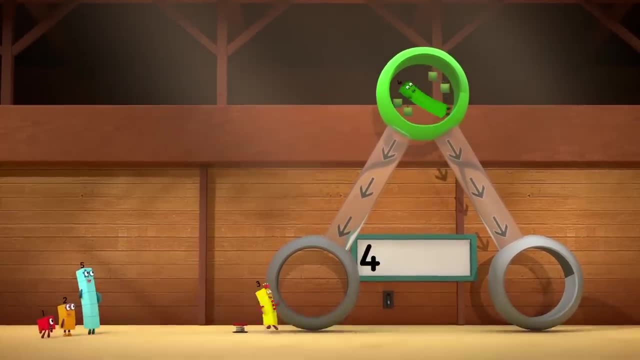 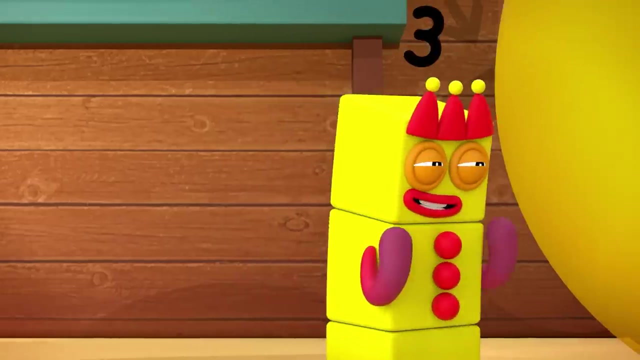 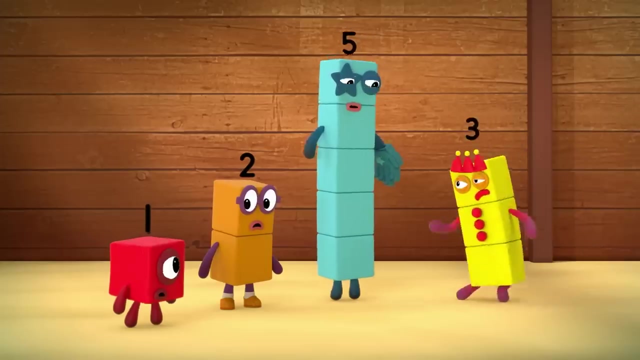 Four new apples, Apples at the top. I know how to make three, Here I come. Four equals one plus three. Yes, yes, yes, No, no, no, No, Oh, Mum, Oh, Oh Oh. 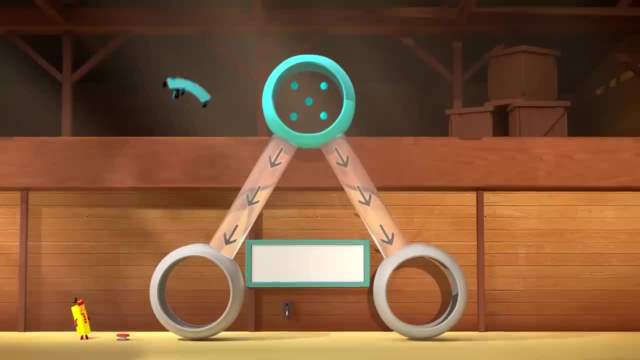 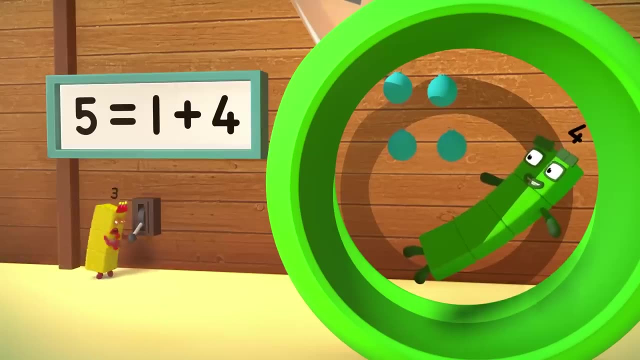 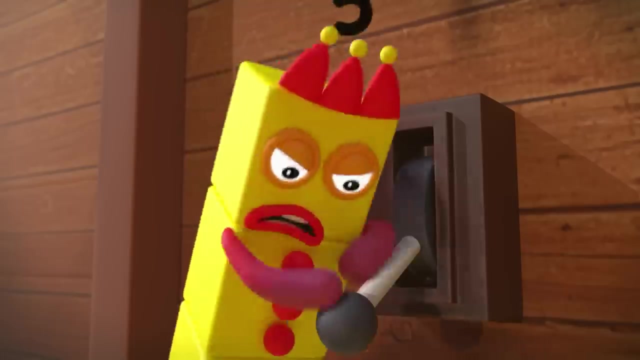 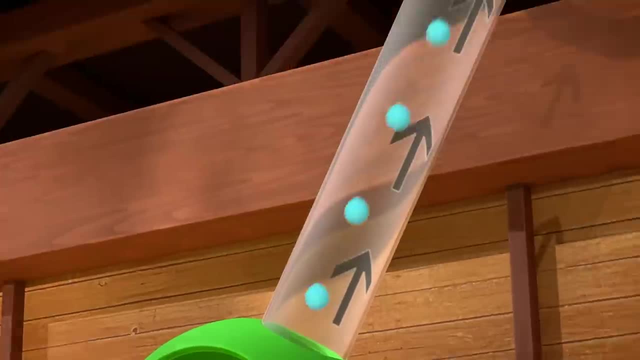 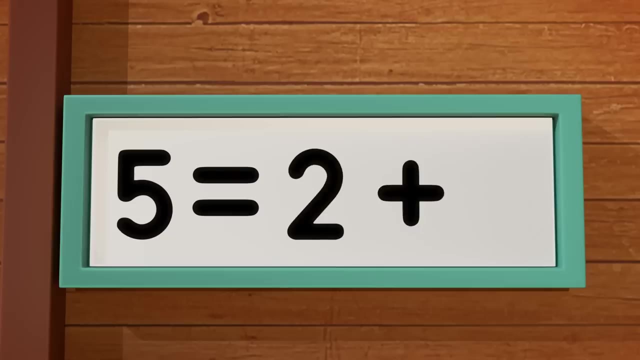 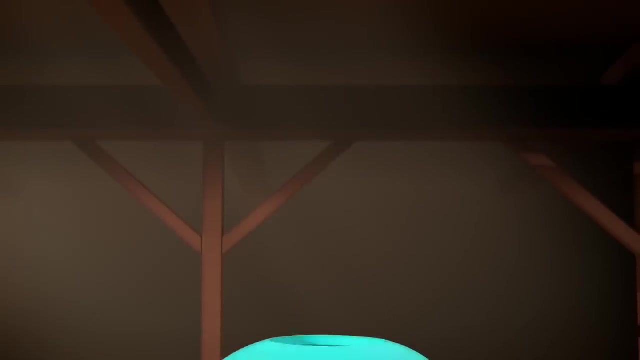 5 equals 4 plus 1.. 4 plus 1 equals 5.. 5 equals 2 plus 1. 2. Two plus three equals five. It's going far too fast. Five equals three. correct: One, two, three. 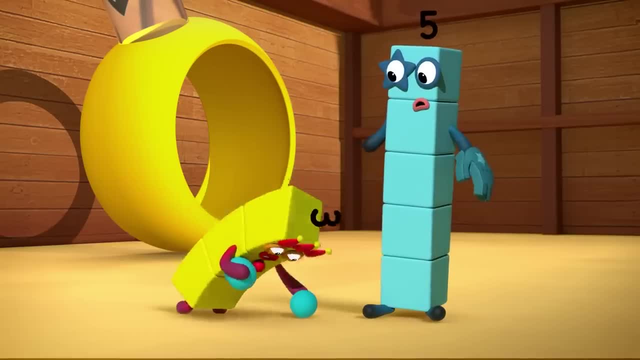 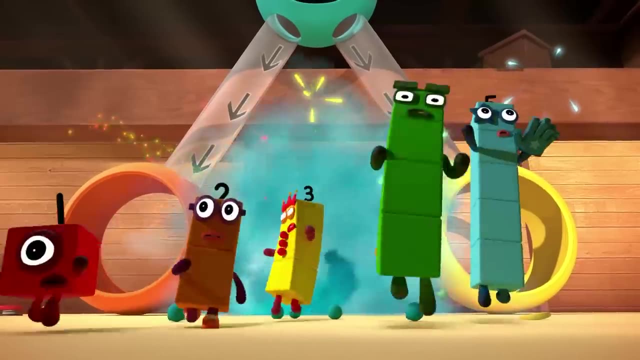 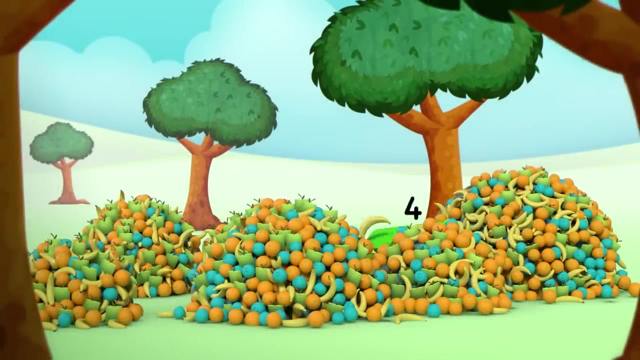 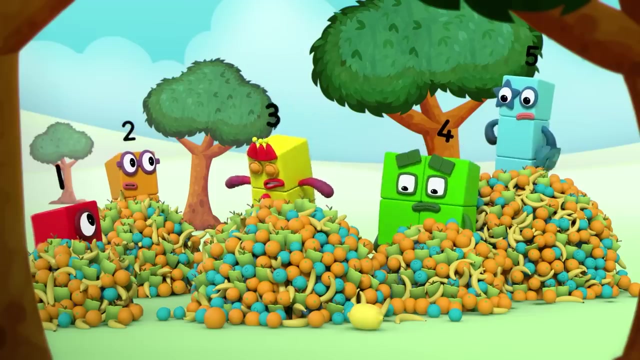 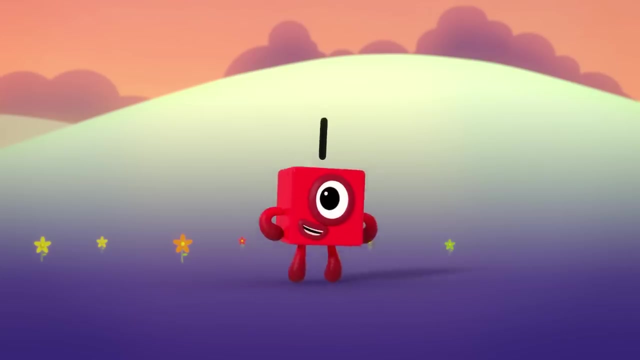 Three blue birds Run. I told you Easy peasy, lovey dovey. I told you: Easy peasy, lemon squeezy. I'm number one And this is fun. I've got one block to play with and the whole of me is one. 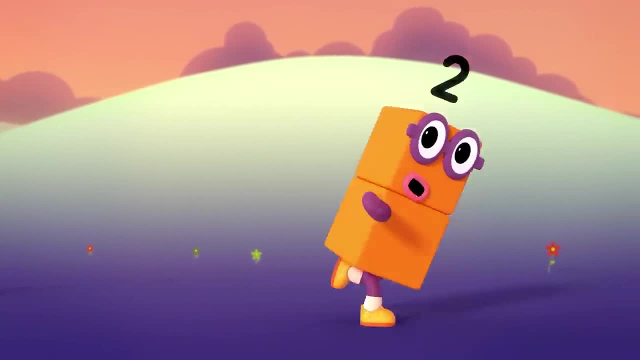 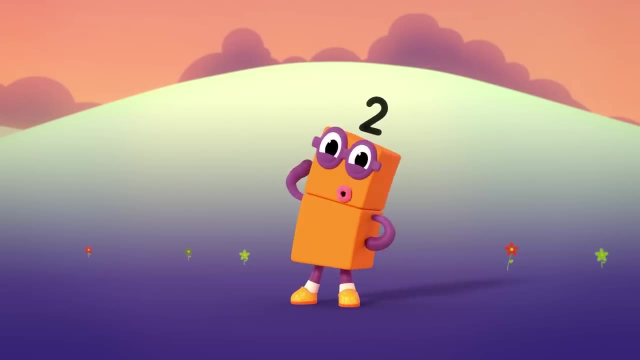 One, One, two, one, two. I'm number two. How do you do? I've got two blocks to play with and the whole of me is two, One, two. One is a part of me and one is a part of me. 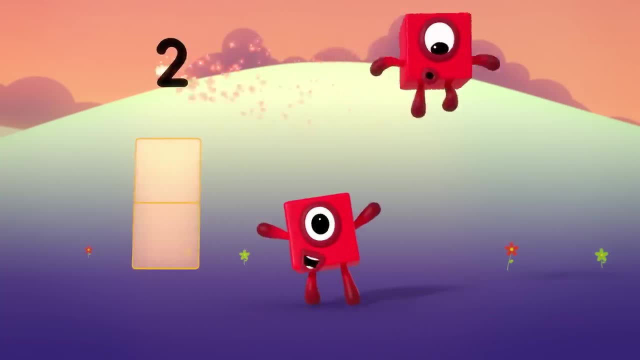 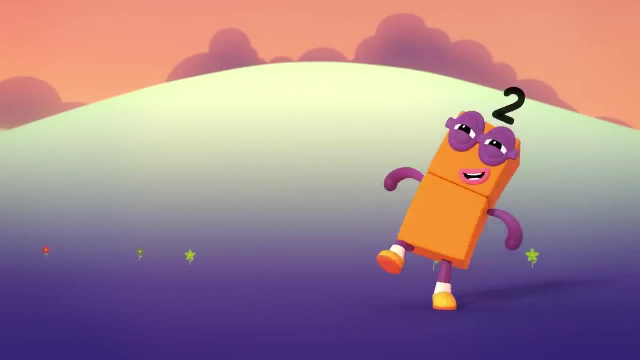 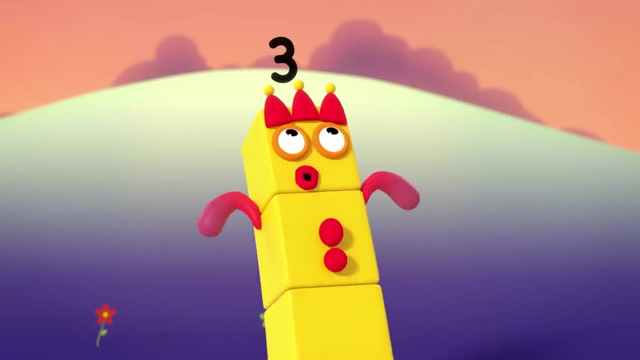 and the whole of me is two. Watch, I'm one and I'm a part. I'm one and I'm a part, And the whole of me is two, One, two, three, One, two, three, One, two, three. 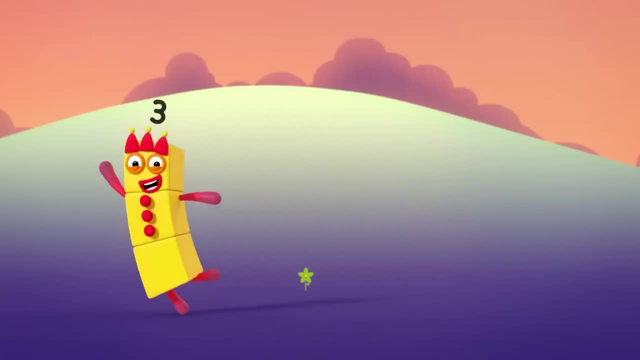 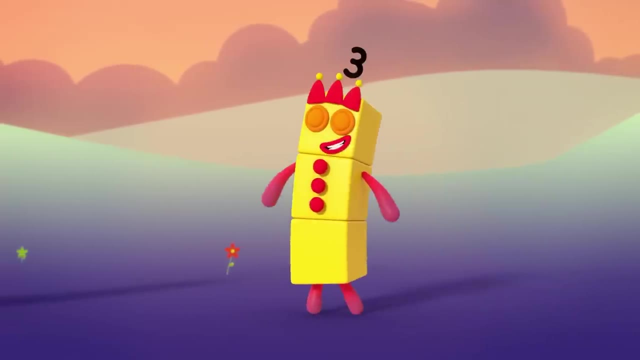 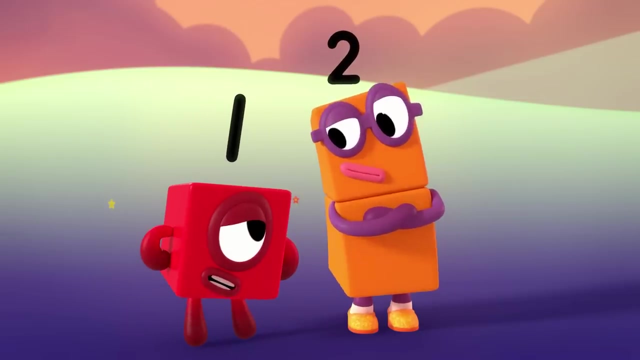 I'm number three. Now look at me. I'm the best of all the number blocks, as you can plainly see. The whole of me is amazing. The whole of me is so great. The whole of me is Sorry. Three, Try again. 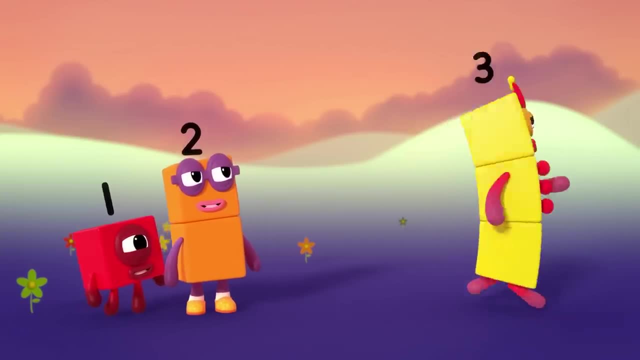 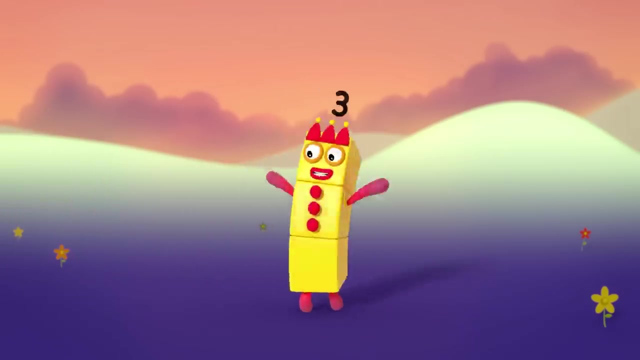 Okay, I'm number three. Yes, look at me. I'm the best of all, the number. Oh, you can't do it like that. You can't do it like that. I am, I'm number three. Now, look at me. 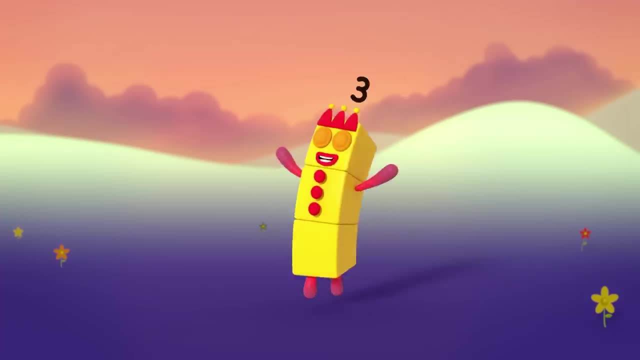 I've got three blocks to play with and the whole of me is three: One, two, three. One is a part of me and two is a part of me, and the whole of me is three. Watch, I'm two and I'm a part. 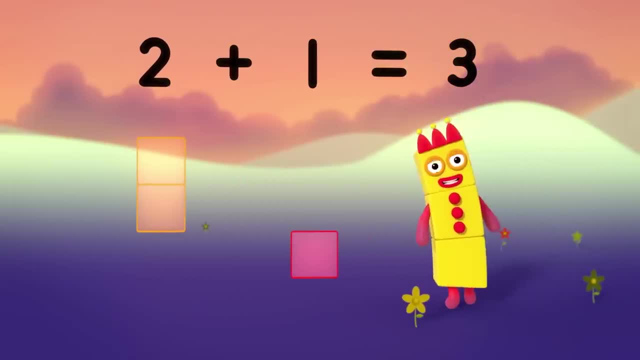 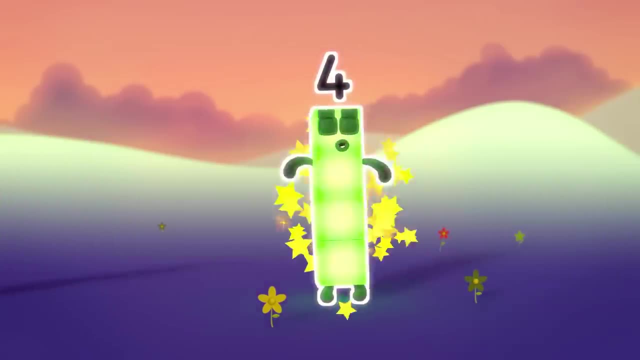 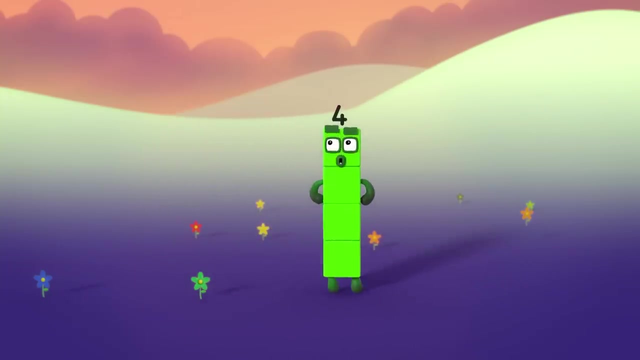 I'm one and I'm a part, And the whole of me is three. One, two, three. I'm number four and I am sure that I've got four blocks to play with, and the whole of me is four. One, two, three, four. 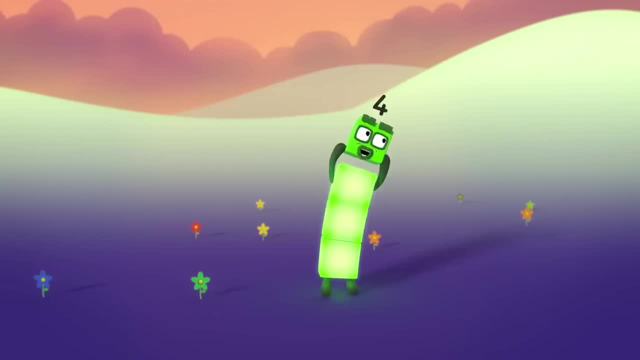 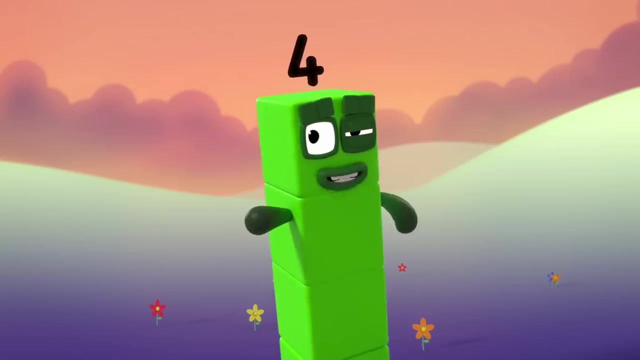 One is a part of me and three is a part of me, and the whole of me is four. Watch, I'm three and I'm a part, I'm one and I'm a part, And the whole of me is four. Now, here is something more. 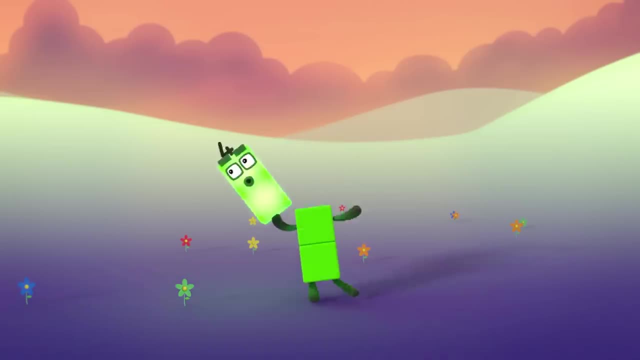 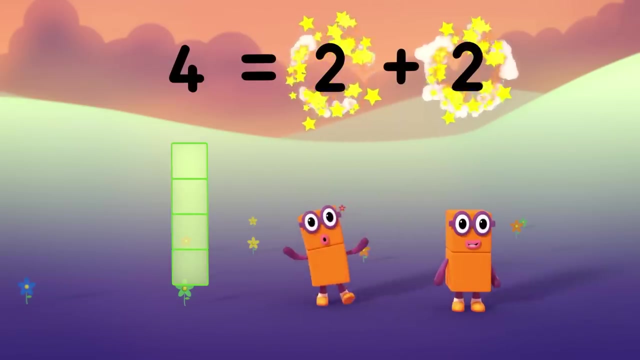 that's different from before. Two is a part of me and two is a part of me, and the whole of me is four. Watch, I'm two and I'm a part. I'm two and I'm a part, And the whole of me. 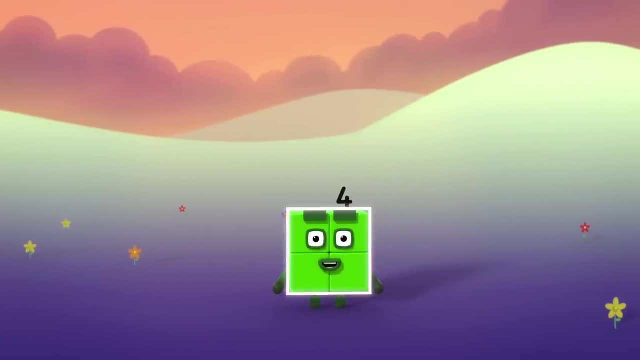 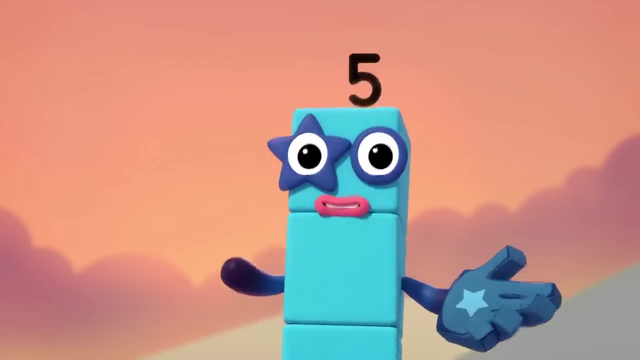 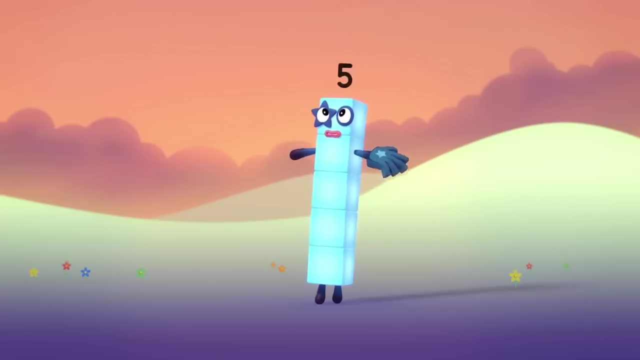 is four. I'm a square. look. Four sides, four corners. I'm number five. I am alive. I've got five blocks to play with and the whole of me is five. One, two, three, four, five. 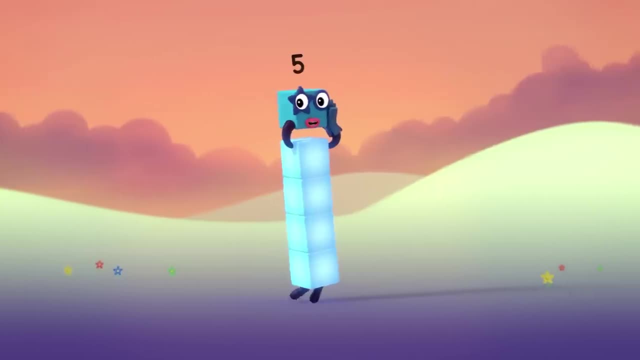 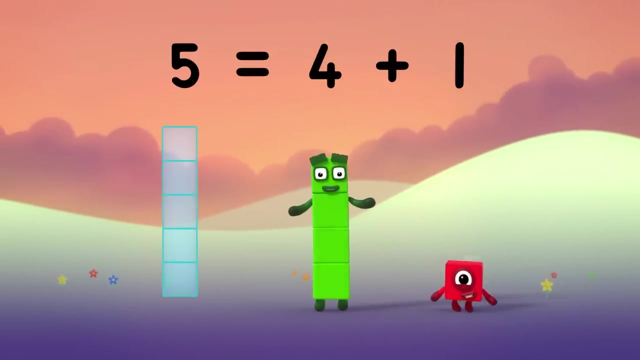 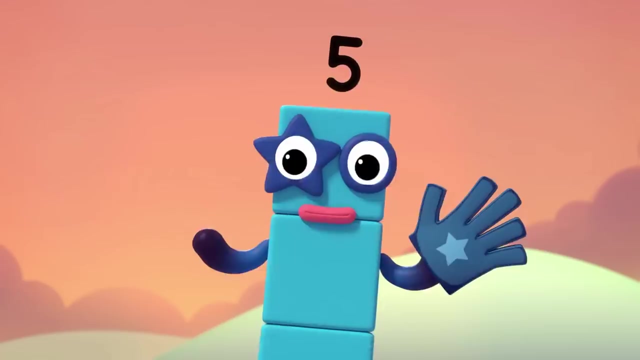 One is a part of me and four is a part of me, and the whole of me is five. Watch, I'm four and I'm a part. I'm one and I'm a part And the whole of me is five. But now I feel alive. 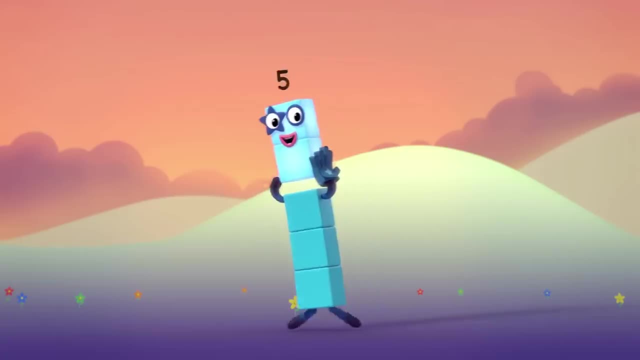 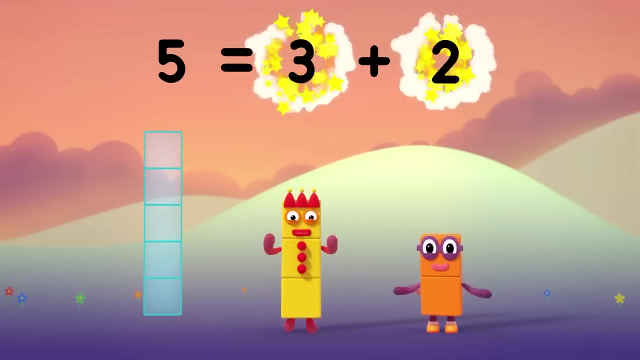 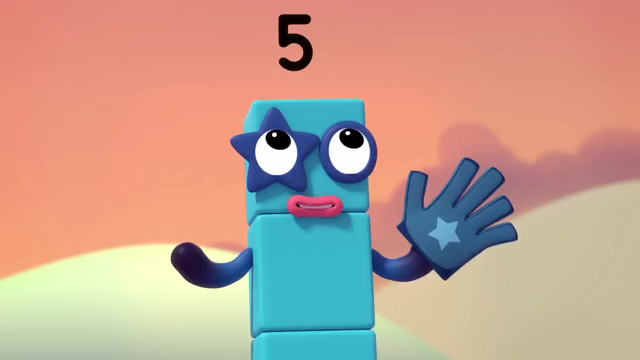 going into overdrive. Two is a part of me and three is a part of me, and the whole of me is five. One and three and I'm a part, I'm two and I'm a part, And the whole of me is five. 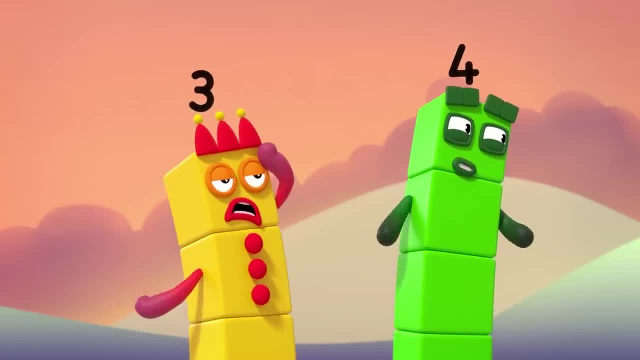 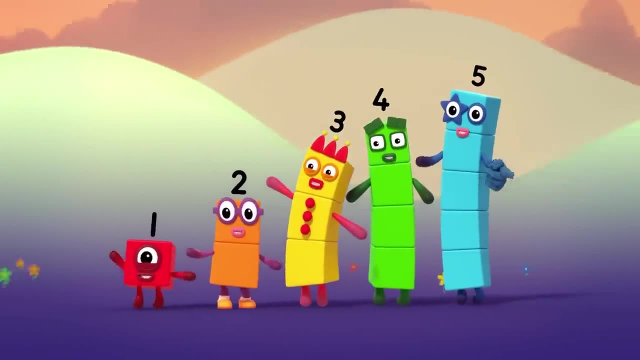 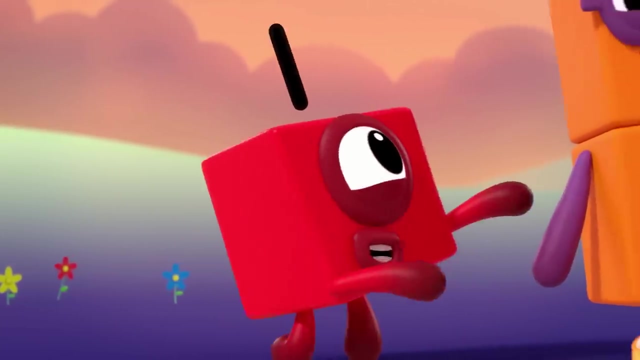 High five: Making friends is easy when you can come apart. Splitting up is not so hard. It's just we have lost control. A whole is made of whole parts and the parts they make are whole. Just remember that One is a part of me. 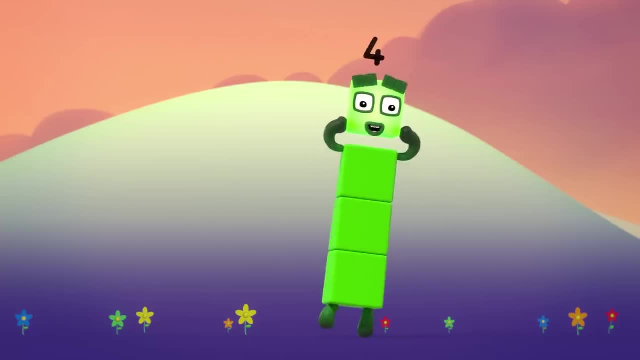 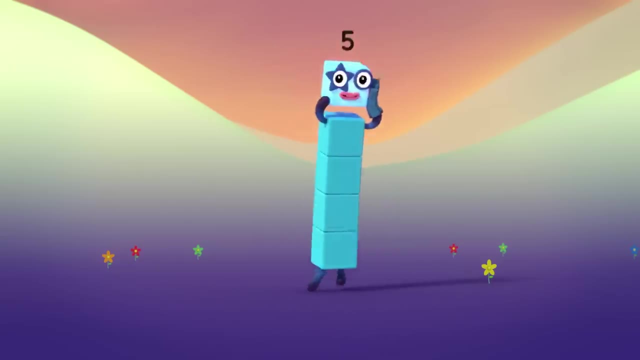 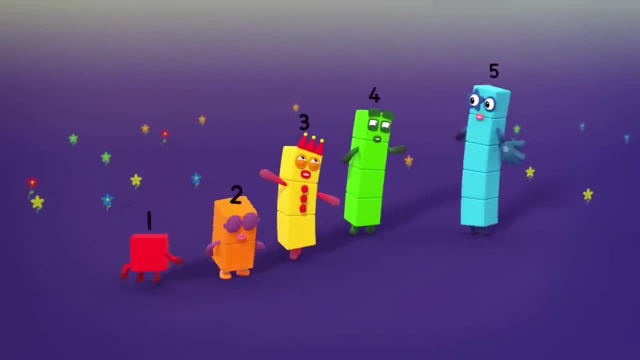 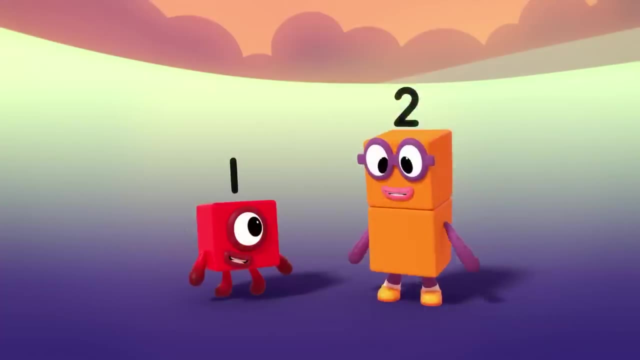 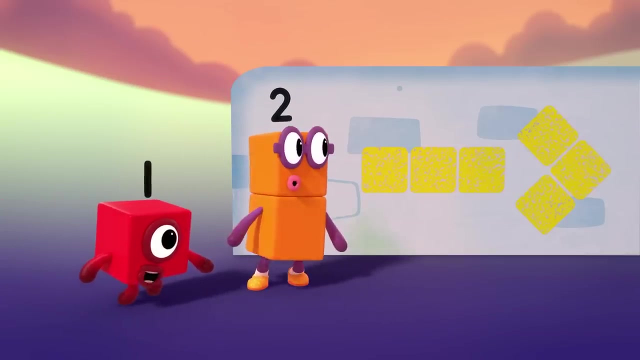 And the whole of me is one, two, four, five, One, two And again One, two. Your turn One. I can't do it. What was that That way? Come on, Wait, Looks familiar. It's pointing to the sounds Quick. 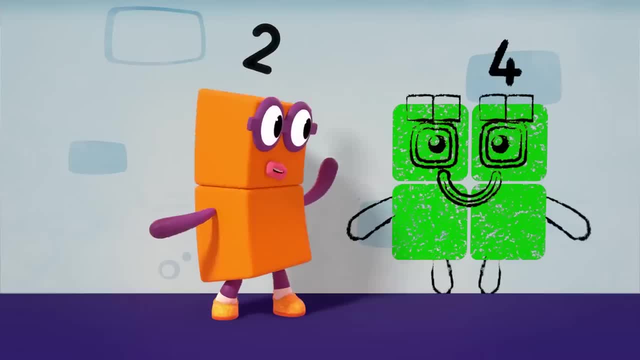 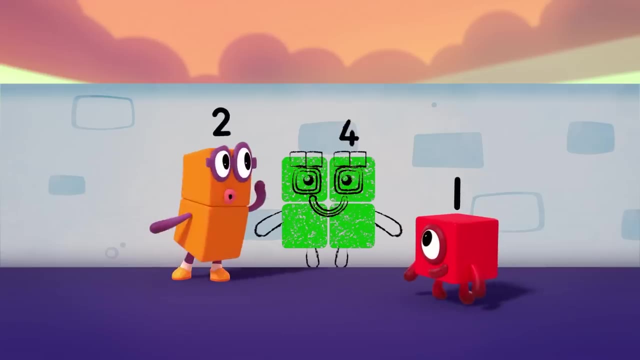 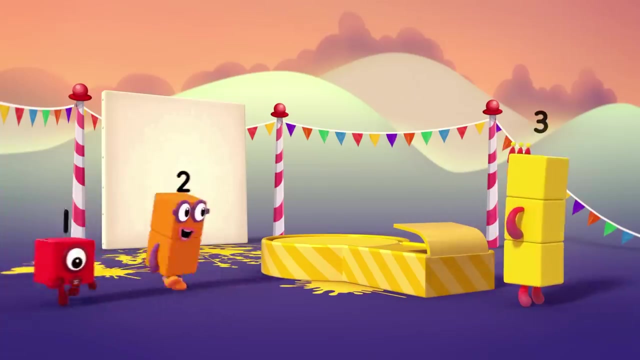 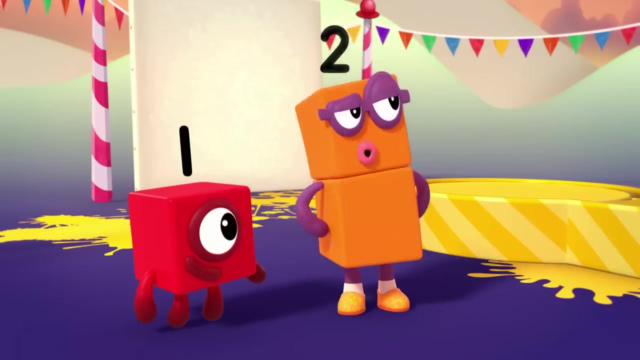 Hey, it's four, Four, Four. Are we playing musical statues? A painting, A painting of four. I knew that, But what's that? Welcome, welcome, welcome to my new stampoline park. Don't you mean trampoline? 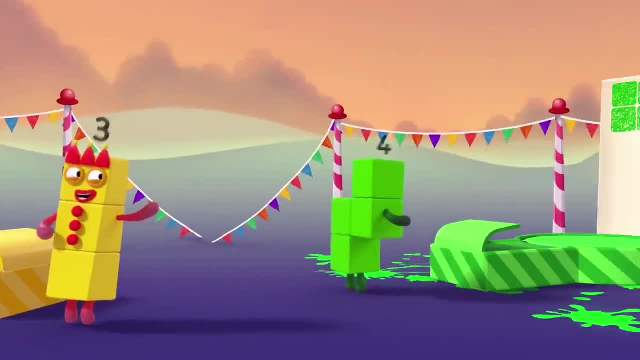 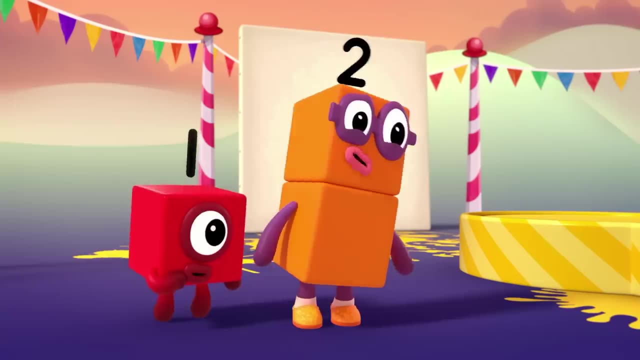 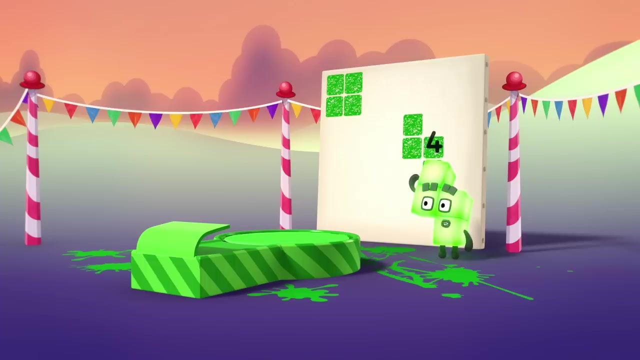 No, no, no, Look, That was fun. Four, Is that you? Of course. it is One, two, three, four, Four blocks, See, Whee. Whatever way round I go, I'm still four, Whee. 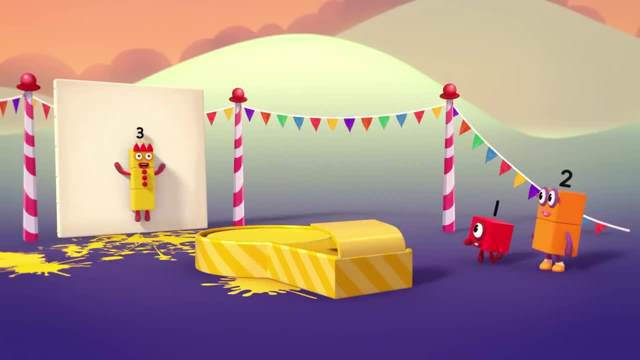 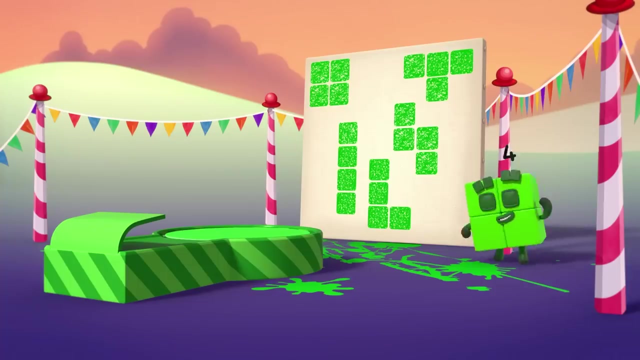 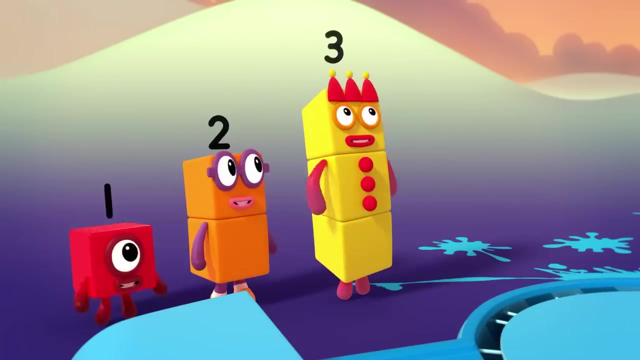 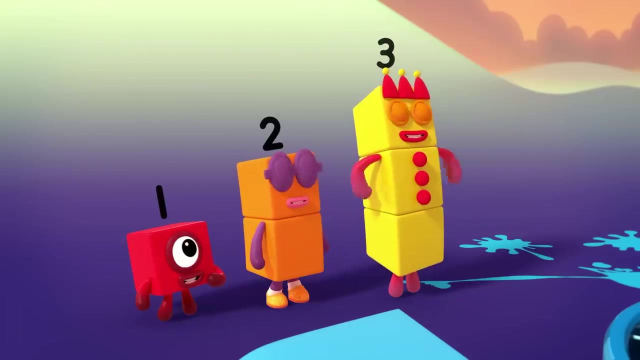 Look at me. Whee, I'm still three. Whee, Not bad. You should see. five Hou five. Did you make all these shapes? I did So. the more blocks you have, the more shapes you can make. 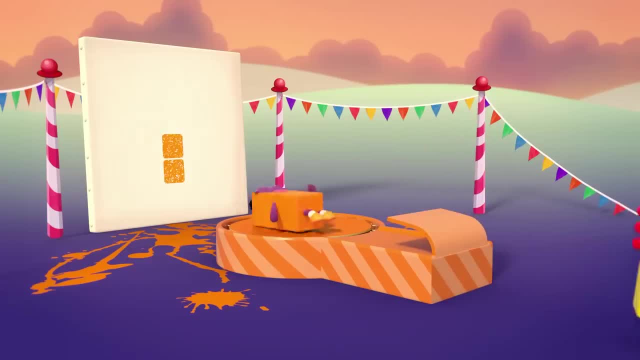 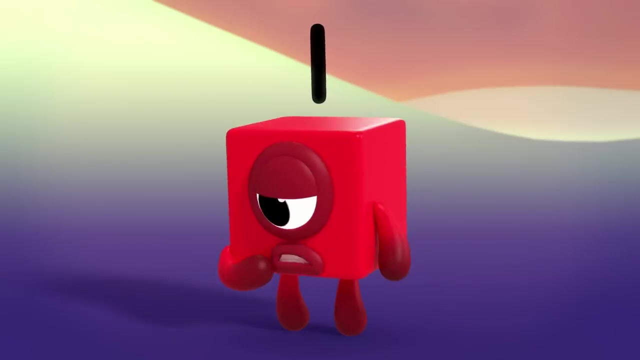 Hen. Oh, My turn In. Not bad two, Of course. they're not really different shapes, are they? It's the same shape, one going up and one going across. Oh, it's still better than me Look. 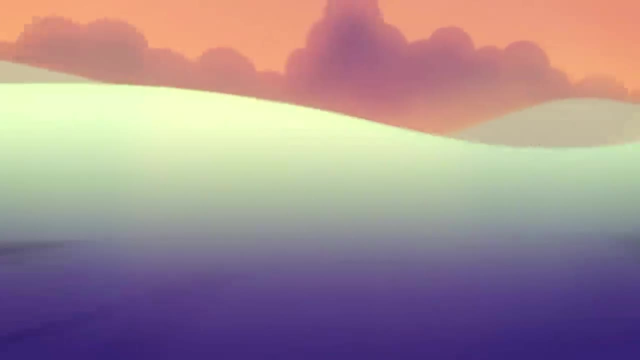 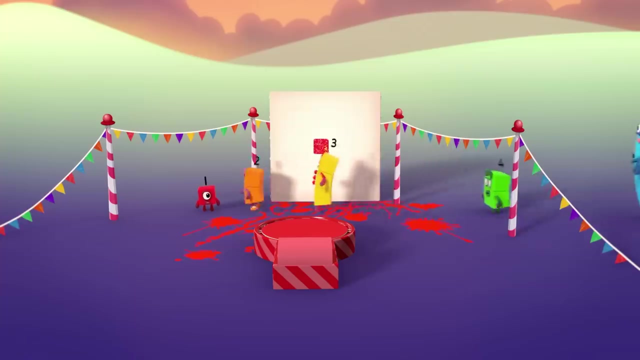 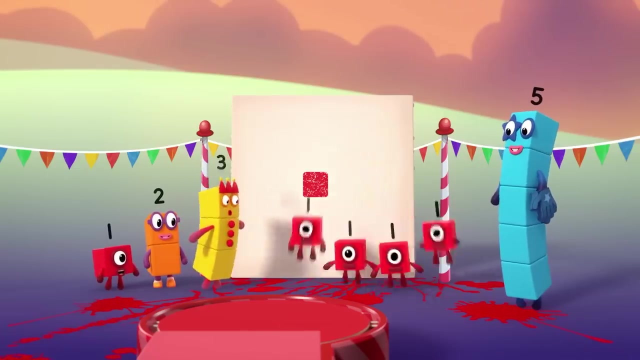 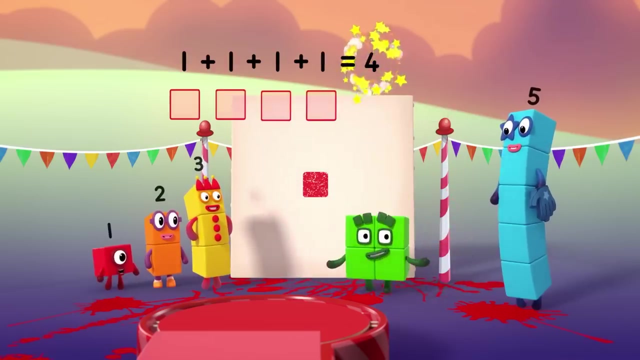 That's all One shape. Not very exciting compared to all of you Now. now, now You're forgetting something. One, two, three, Boom, Hey. One plus one plus one plus one equals four. Every big shape is made up of lots of little ones. 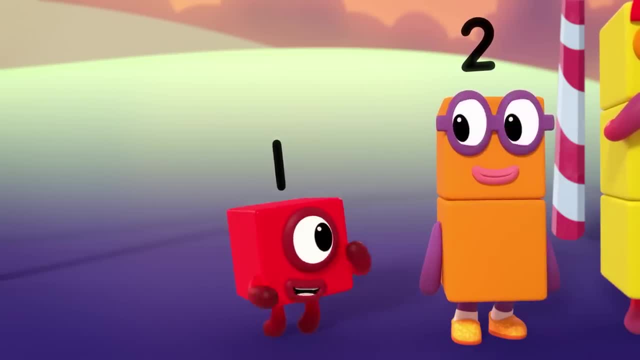 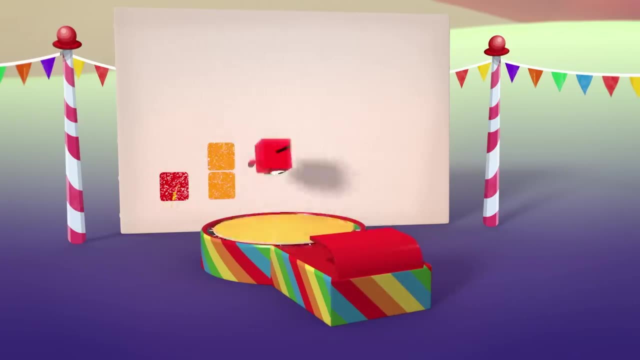 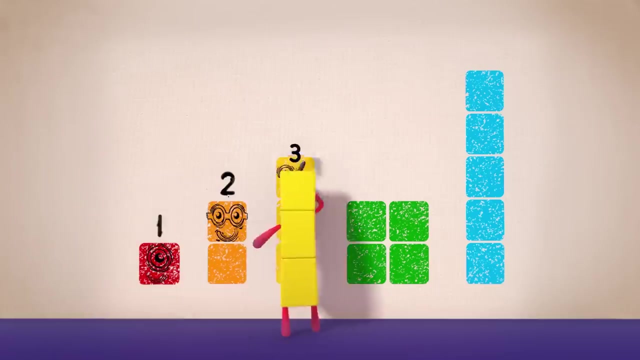 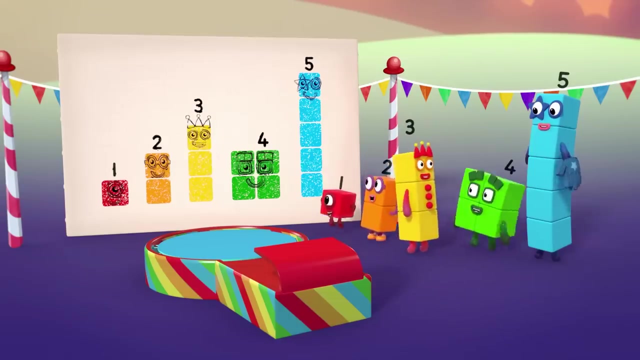 So lots of little ones can make every big shape. Look what I can do. Hooray, You made all of us Hooray. Well done, And just in time for the grand finale, What better way to celebrate opening my new park? 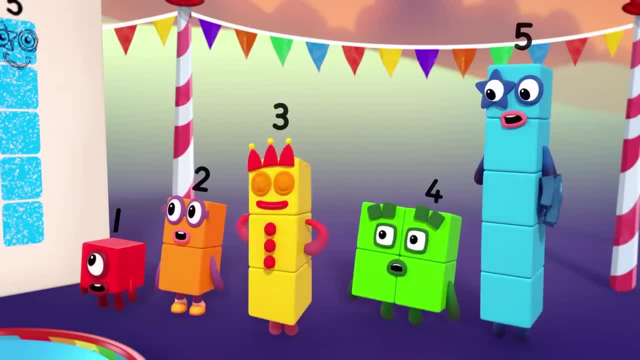 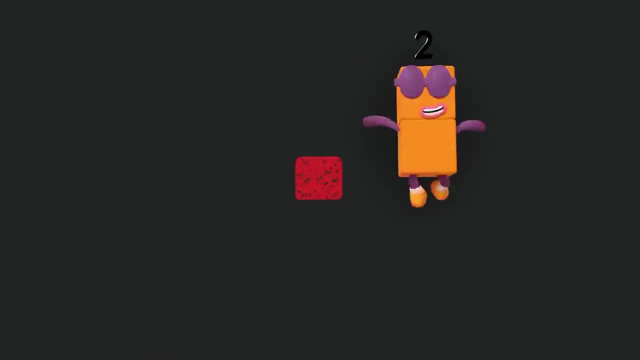 than with fire. Oh, May I present the Sky At Nut Woo Yay, Woo-hoo, Yay, Woo-hoo, Yay, Yeah, Woo-hoo Hooray, Woo-hoo, Yeah, Hooray. 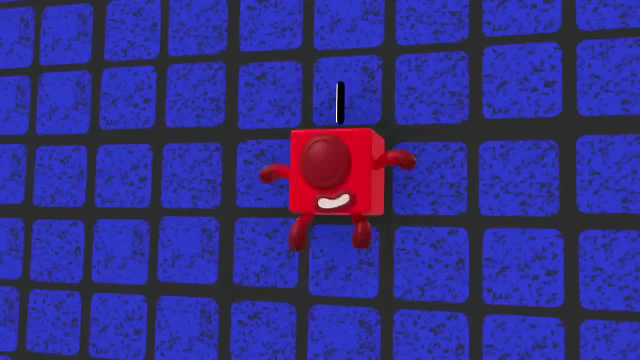 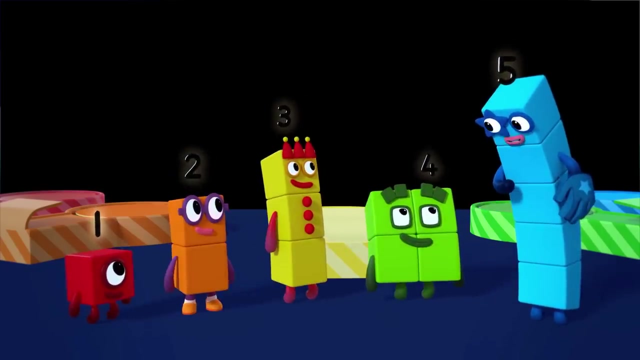 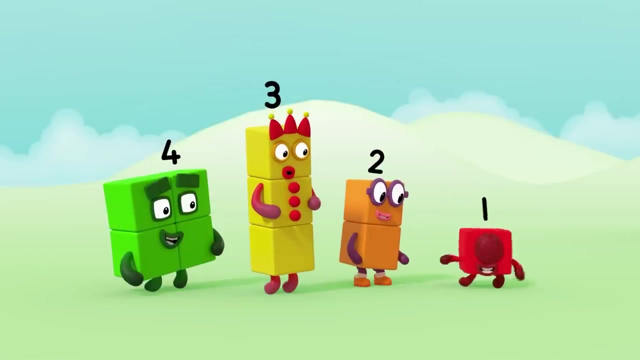 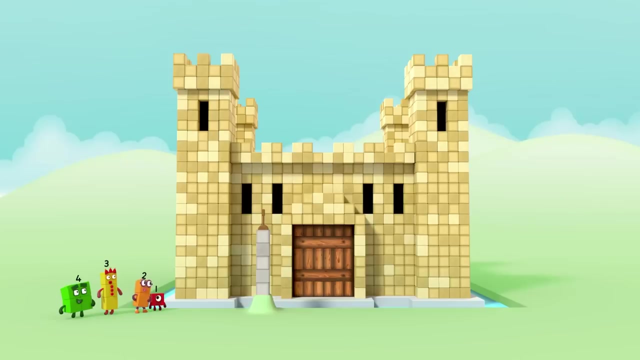 Yeah, Woo-hoo, Woo-hoo, Woo-hoo, You see one. When we all work together, the sky's the limit. Hooray Time for adventure. to Number Block Castle: Great, How do we get in? Hmm, Maybe if we pull that handle. 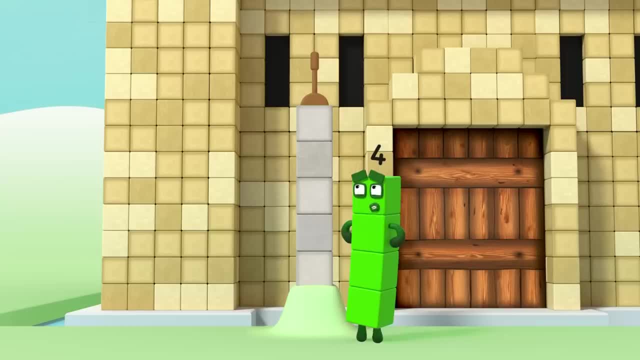 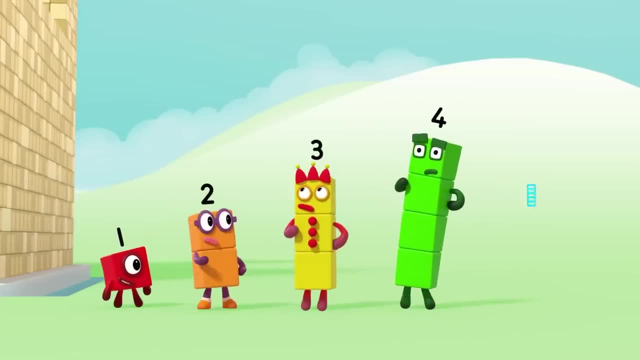 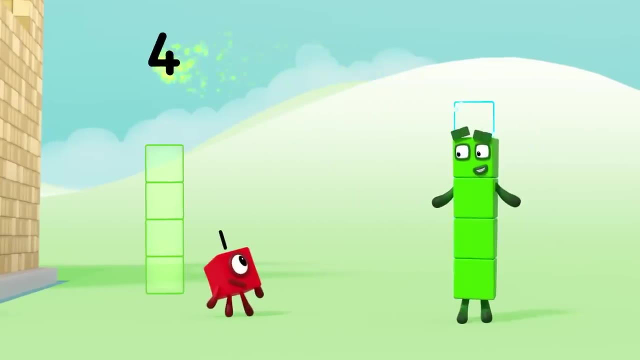 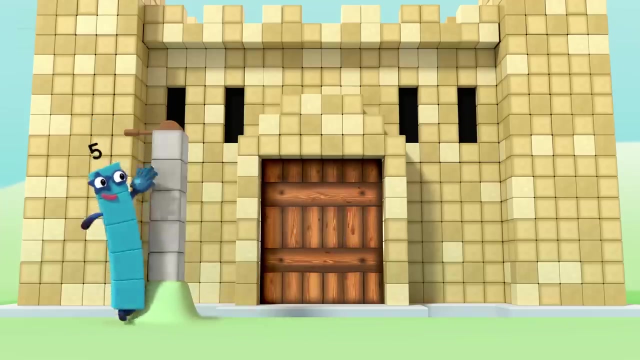 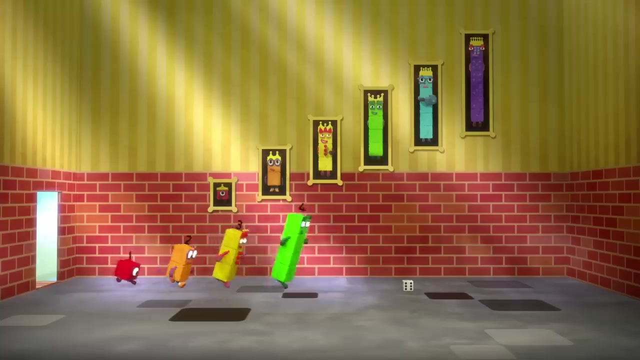 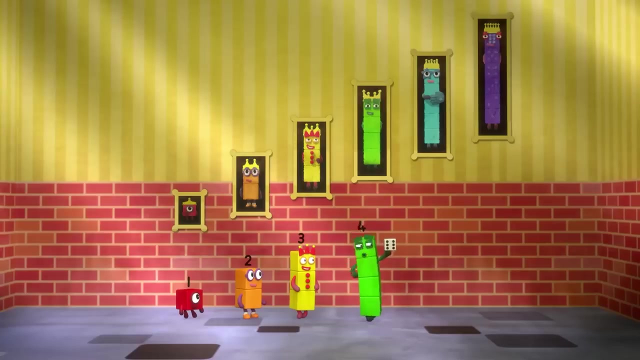 Oh, oh, If only I was a little bit taller. Five's taller than four. So how do we get five? Four plus one equals five. Oh, Hooray, Ah, Dead end. Six is good with dice. 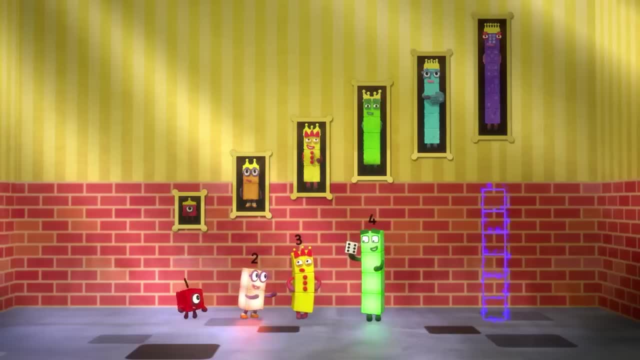 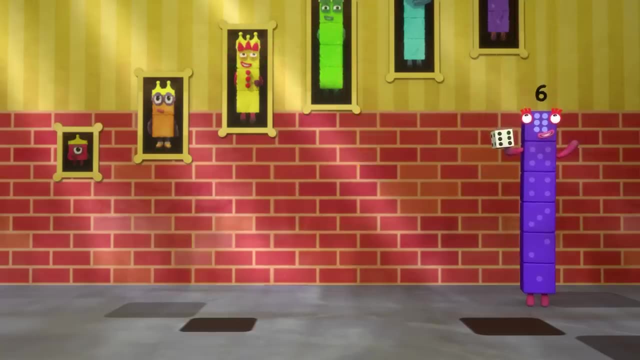 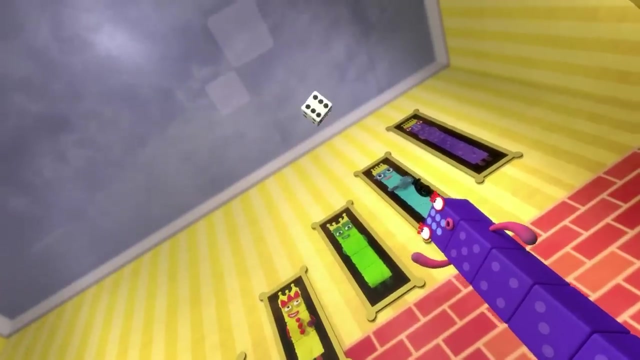 How do we get six? Four plus two equals six. Hello friends, Here's my advice. It's time for me to roll the dice. Watch me give a little throw and you'll know which way to go. 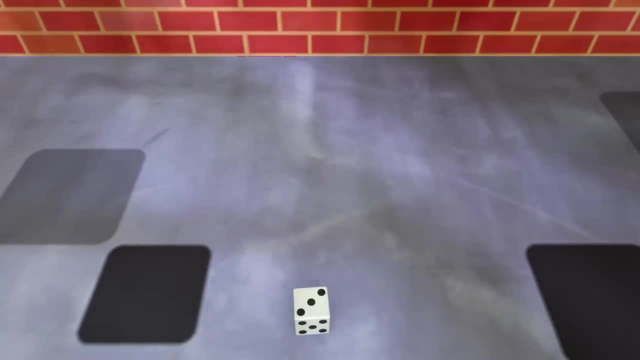 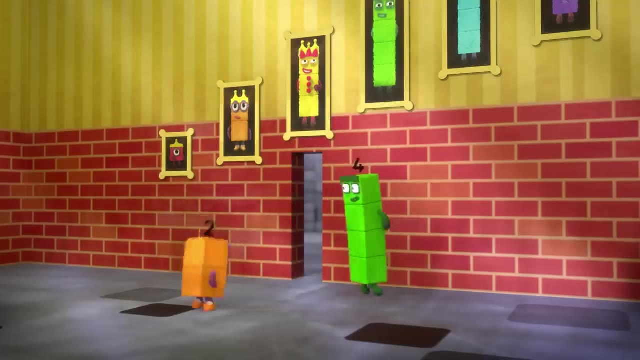 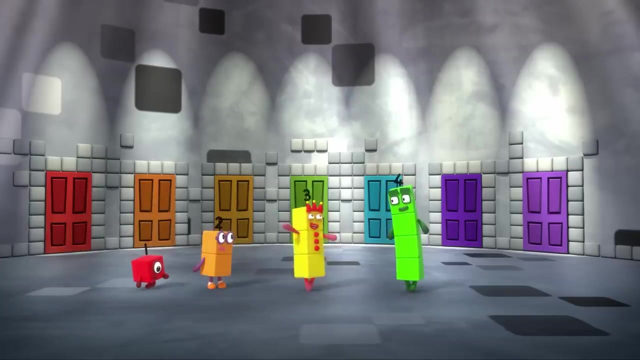 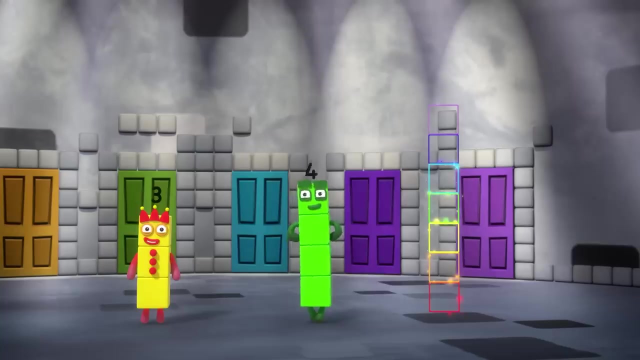 One, two, three, One, two, three, One, two, three. Follow me. Seven doors. Which door is right? Maybe seven can help. How do we get seven? Four plus three equals seven. 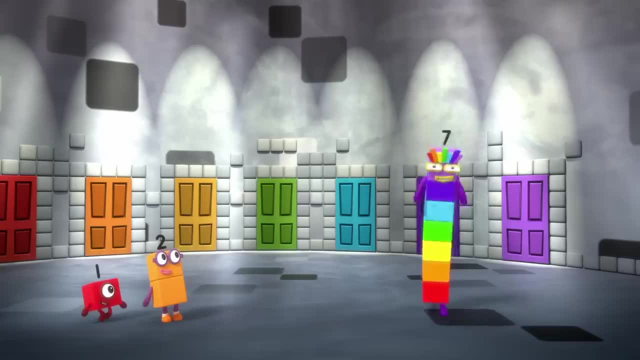 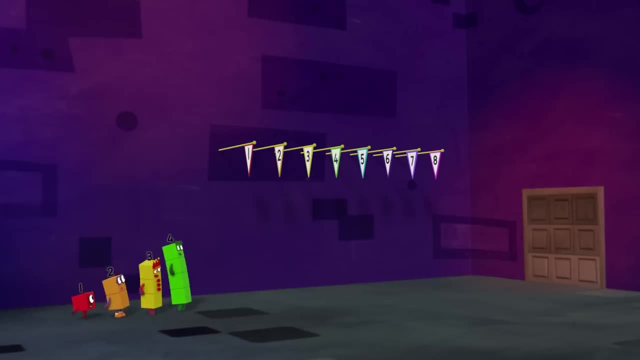 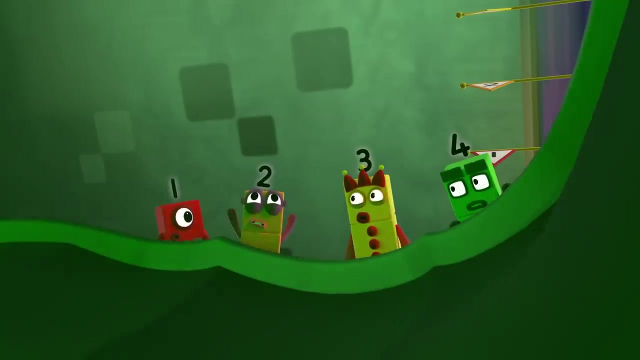 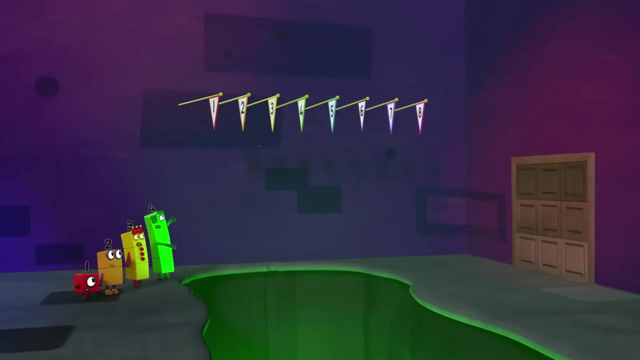 Oh, Seven, Oh, I feel lucky, Whoa. Oh, This way, Easy-peasy, Look-a-mazy. Oh, We're stuck. No, we're not. We could swing from the flagpoles. We'd need someone with very long arms to stretch that high. 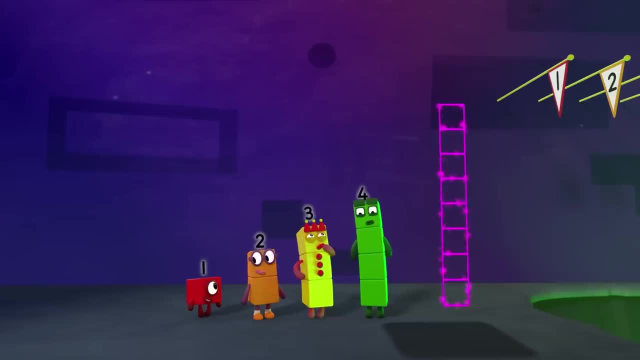 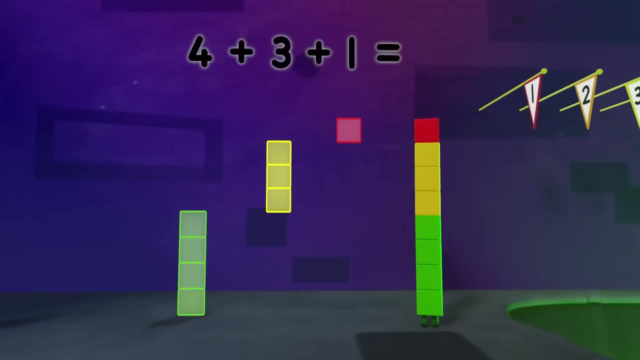 Eight. How do we get eight? Oh Yeah, Four plus three plus one equals eight. Octoblock swing Hooray. One, two, three, four, five, six, seven, eight. 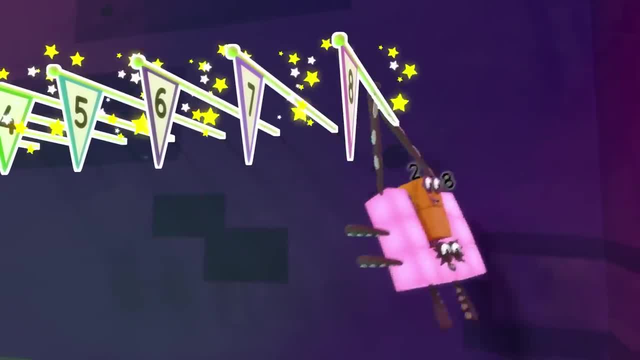 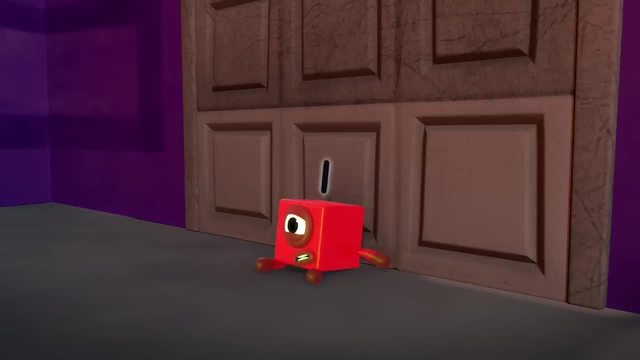 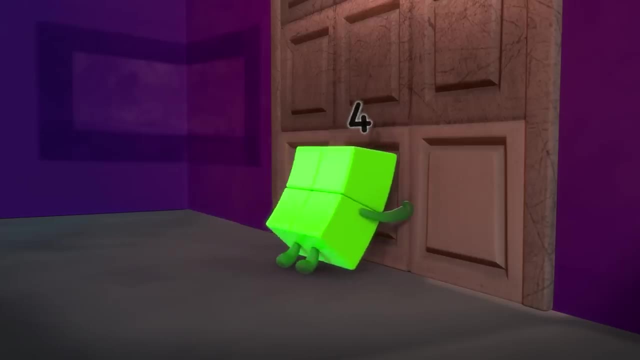 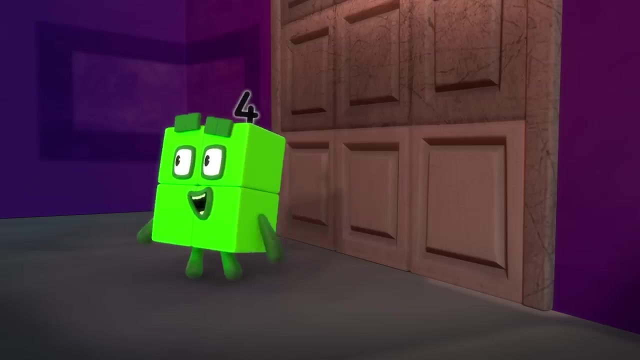 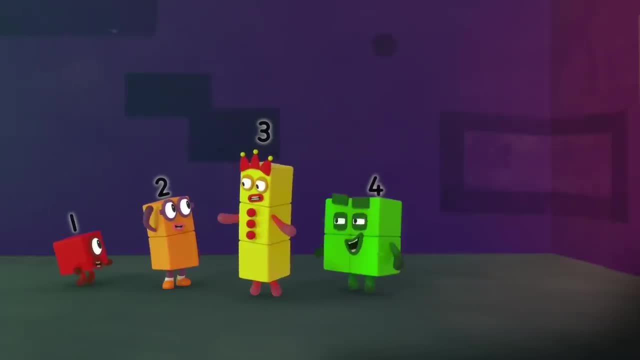 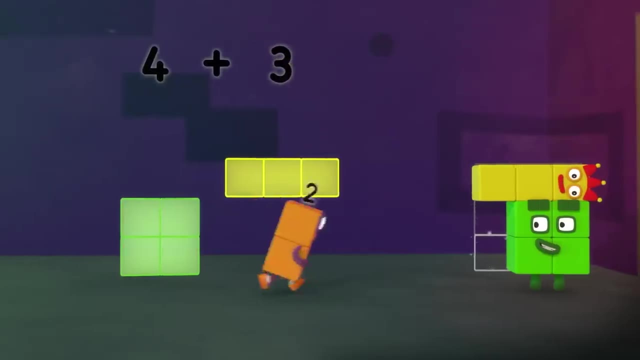 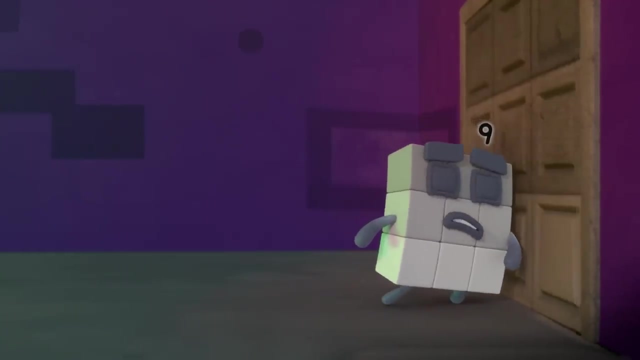 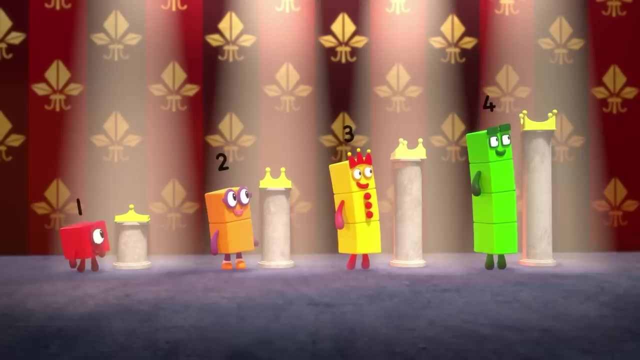 Nine. How do we get nine? Four plus three plus two equals nine. Ha-ha, Ooh, Ah, Ooh, Oh, Ooh, Thanks, Oh, Ha-ha-ha-ha-ha. 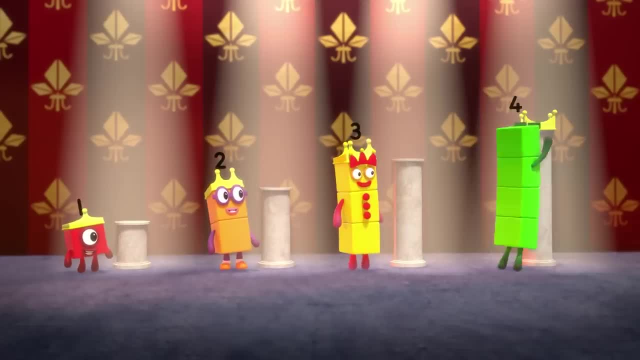 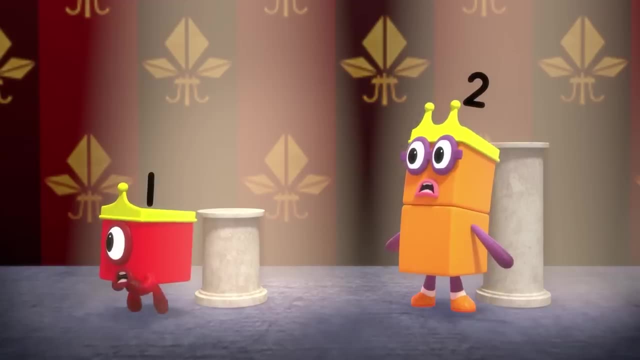 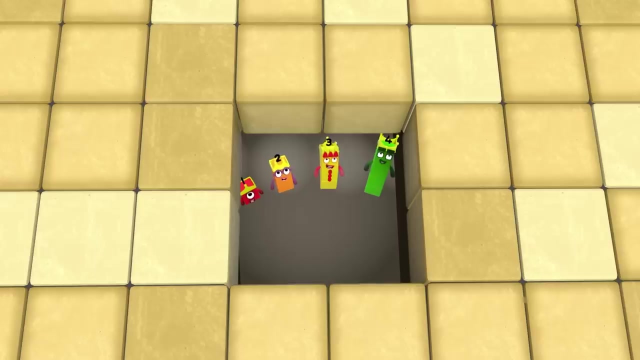 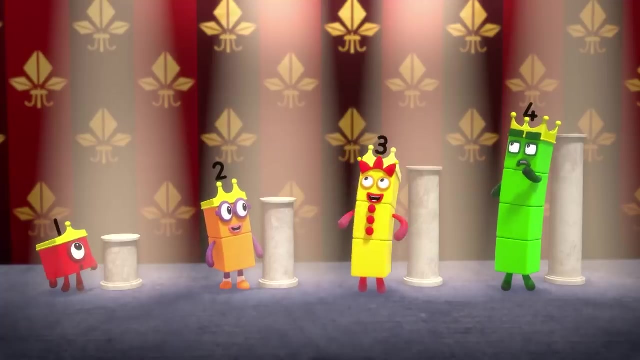 One, two, three, four, Four crowns. Hoo, Oh-oh. How are we gonna get out? Ha-ha-ha-ha-ha-ha-ha. Ah Ooh, If ten was here, we could rocket out through there. 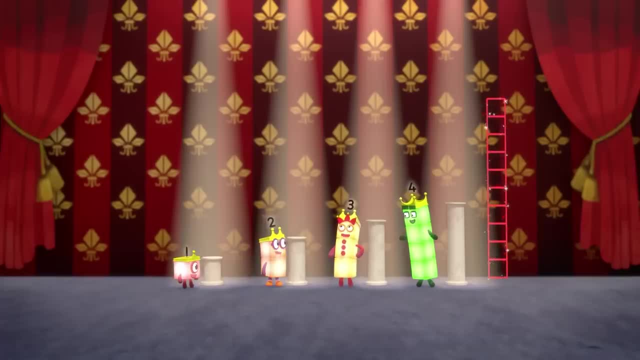 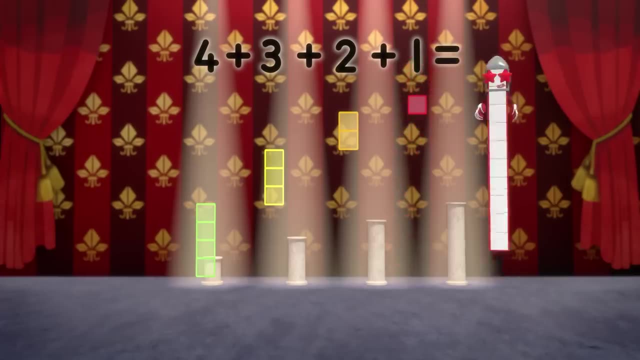 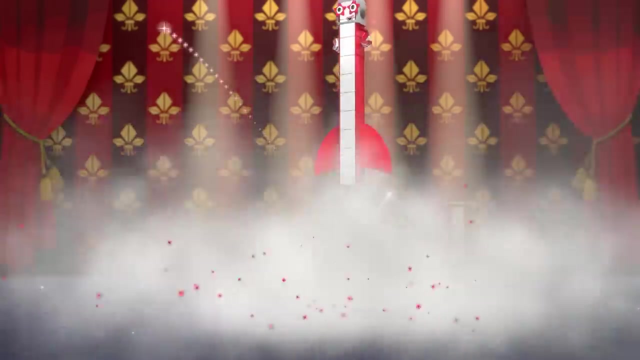 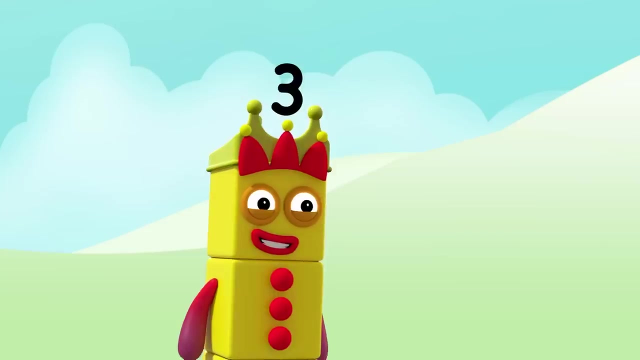 How do we make ten? Ooh, All together now, Four plus three plus two plus one equals ten, Ten, nine, eight, seven, six, five, four, three, two one. Blast off Four, three, two, one. 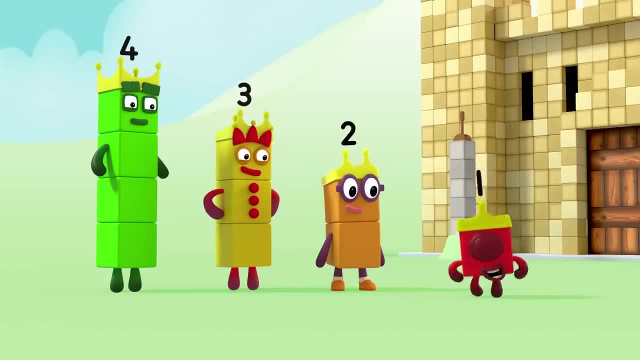 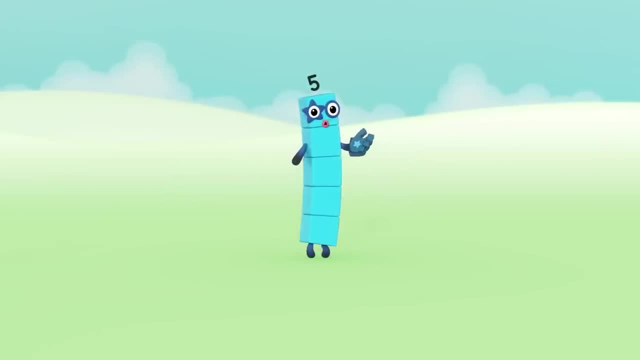 What an adventure. We may be little numbers, but when we work together, we're still the kings and queens of the castle. Let me tell you a story. Once upon a time, there were Three Ha-ha-ha-ha-ha. 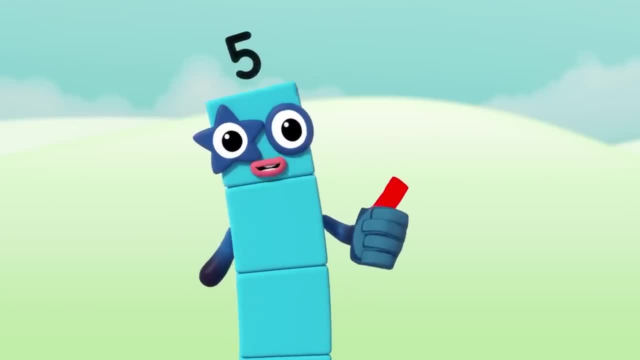 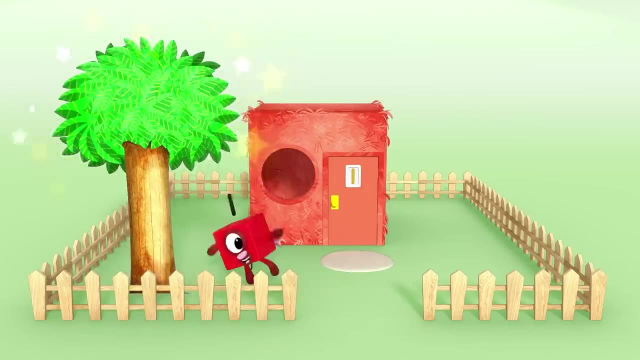 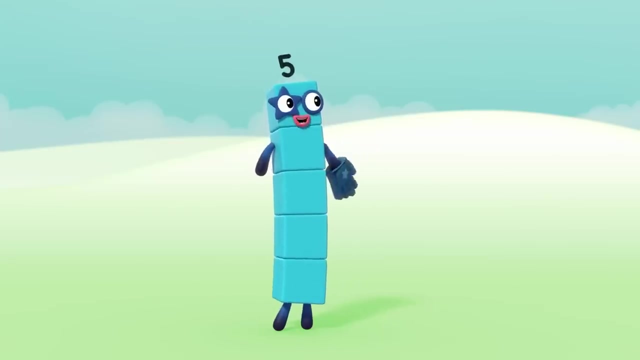 little pigs. The first little pig had a house with one room. Look, It has one one window and one one tree in the garden And there's a number one on the door. But then came Ha-ha. 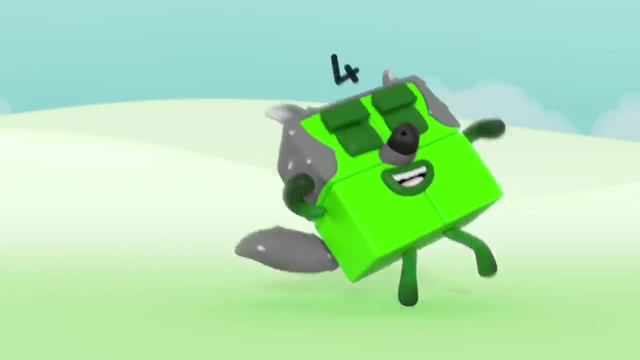 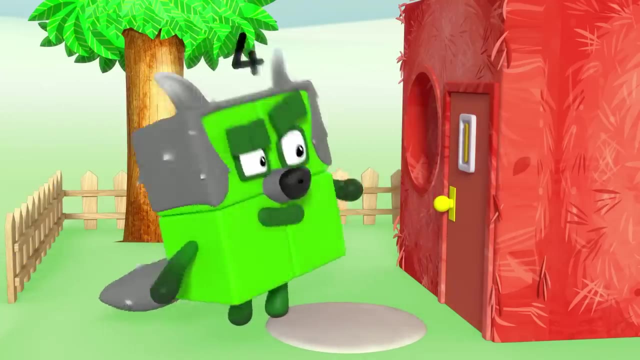 The big barred squirrel Roar, Ha-ha-ha-ha-ha, Little pig, little pig, let me in. let me in, Ha-ha-ha-ha-ha, Not by the head or my chin. 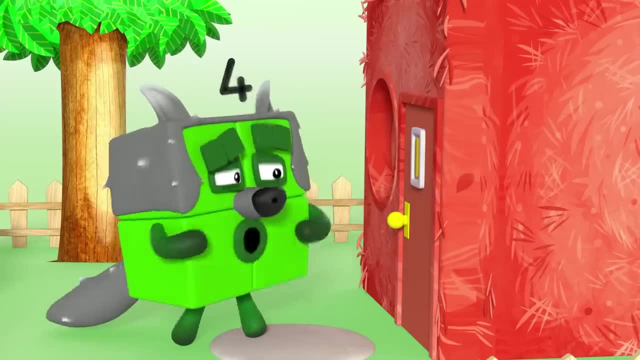 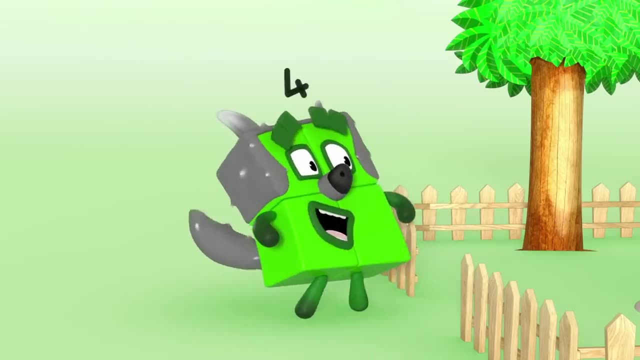 Then I'll hoof and I'll poof and I'll blow your house in Ha-ha-ha-ha-ha. Shame, That's so square. Ha-ha-ha-ha-ha, Ha. Oh, Whoa. 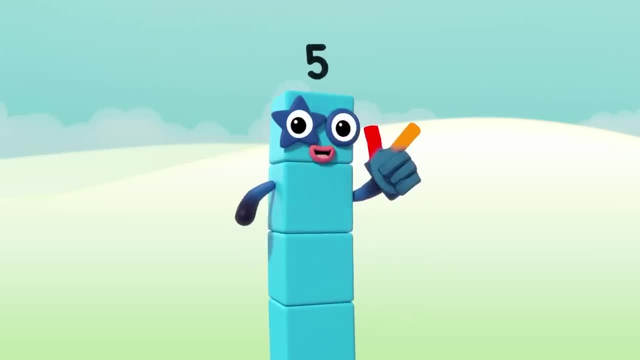 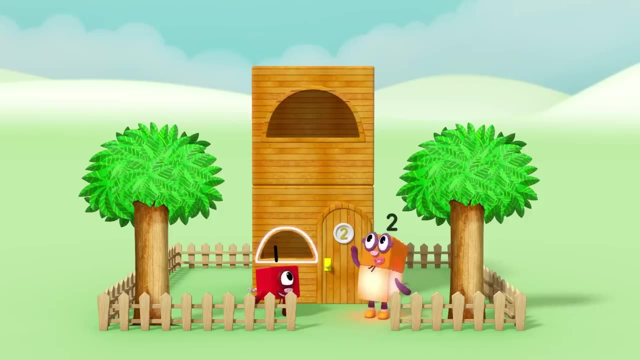 Whoa Ha-ha-ha-ha-ha. Luckily, the second little pig had a house with two rooms: Room for two, me and you. It has one two, two windows and one two, two trees in the garden. 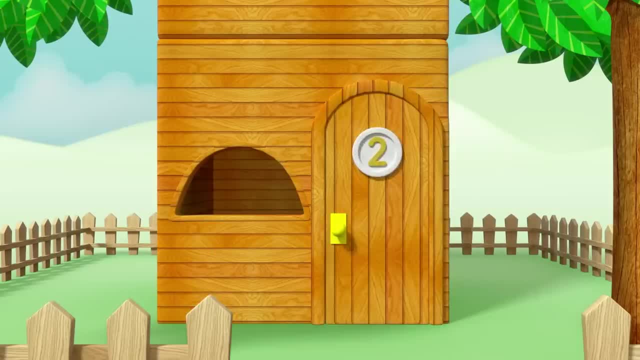 And there's a number two on the door: Ha-ha-ha-ha-ha, Ha-ha-ha-ha-ha, Ha-ha-ha-ha-ha, Ha-ha-ha-ha-ha. Tea for two and two for tea. 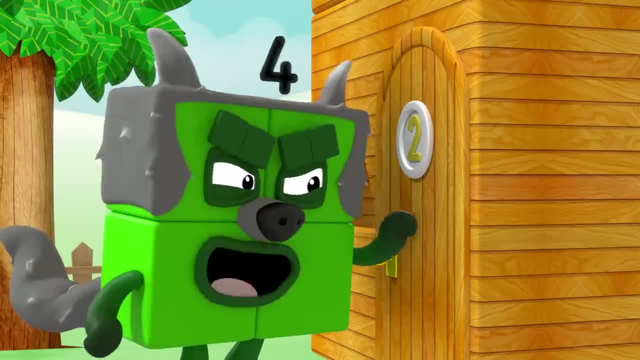 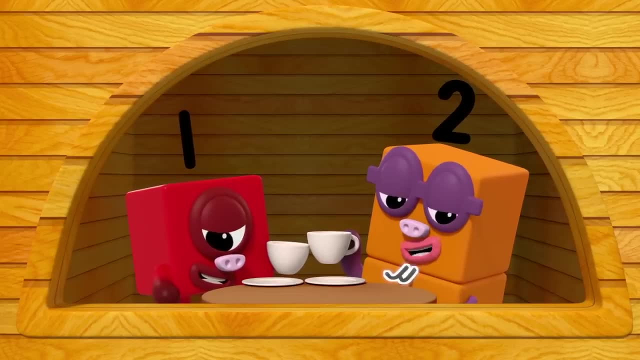 Ha-ha-ha-ha-ha, Little pig, little pig, let me in. let me in, Not by the two hairs on my chinny chin. Ha-ha-ha-ha-ha, Then I'll hoof and I'll poof and I'll blow your house in. 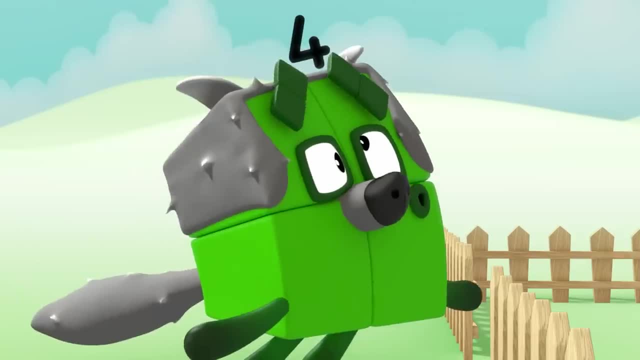 Ha-ha-ha-ha-ha, Ha-ha-ha-ha-ha, Ha-ha-ha-ha-ha, Ha-ha-ha-ha-ha, Ha-ha-ha-ha-ha, Ha-ha-ha-ha-ha. 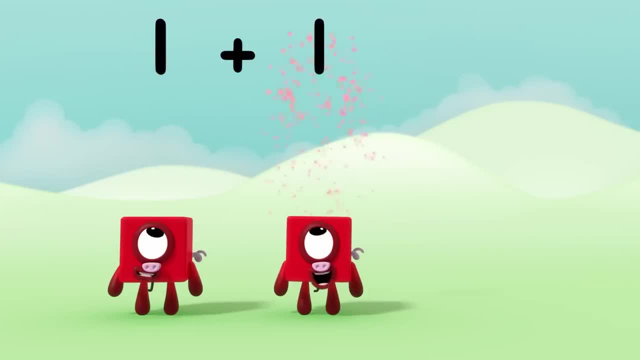 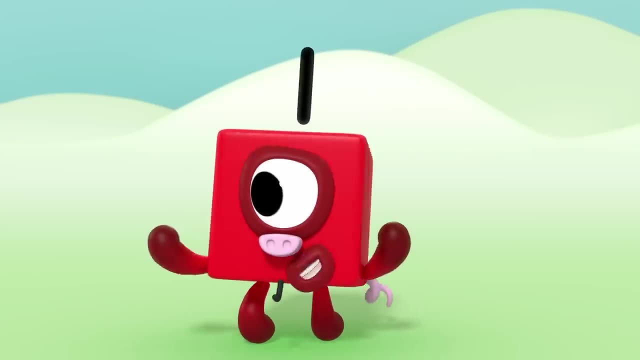 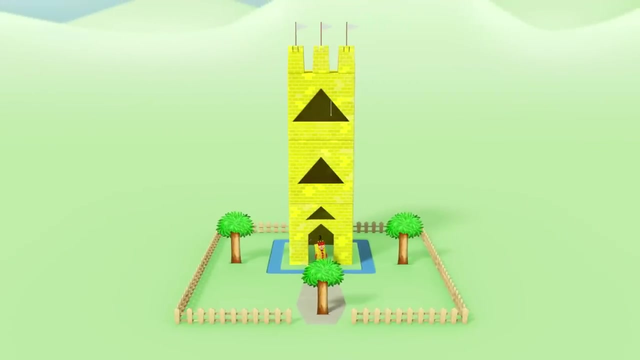 Sorry, two One plus one equals Two. No worries, It's only pretend, But where will we live now? Luckily, the third little pig- Oh, that's me Busy, busy, busy- had a house with three rooms. 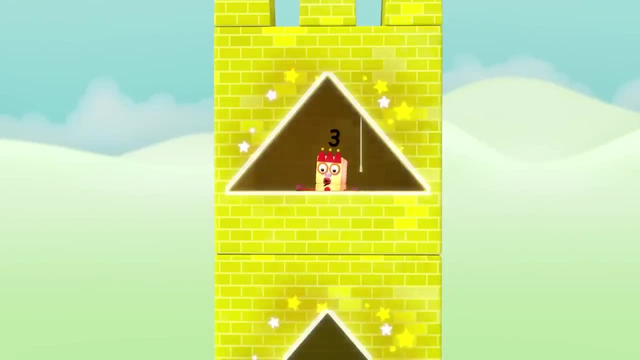 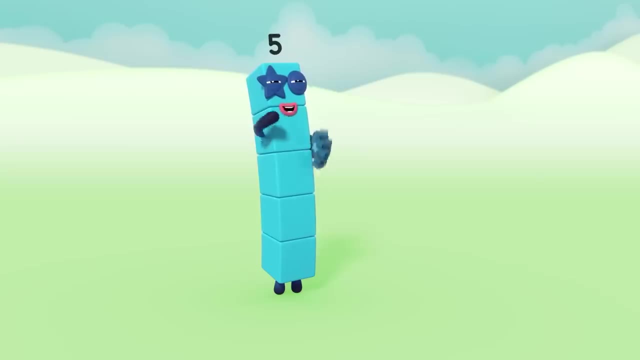 And one, two, three, three windows, And one, two, three, three turrets, And one, two, three, three flags. And, yes, yes, thank you three Oh, Room for a couple more Sure. 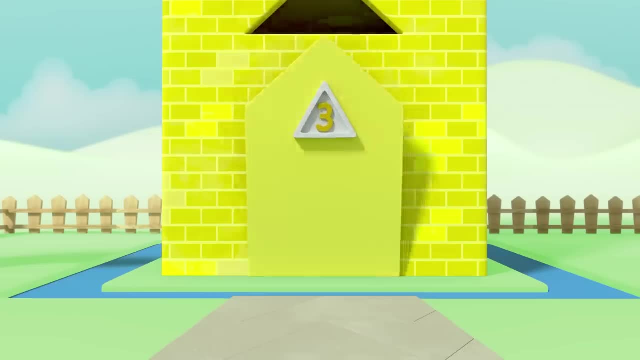 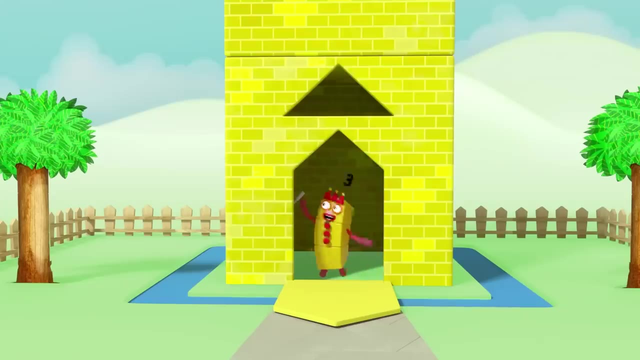 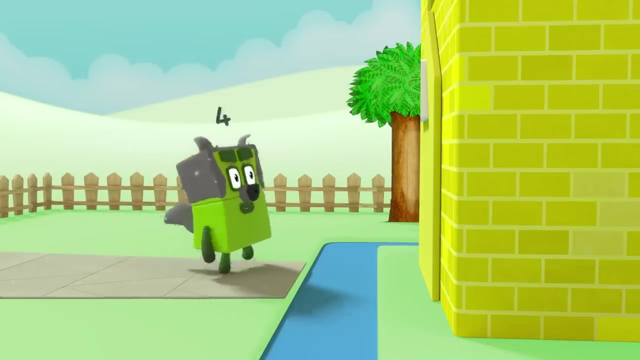 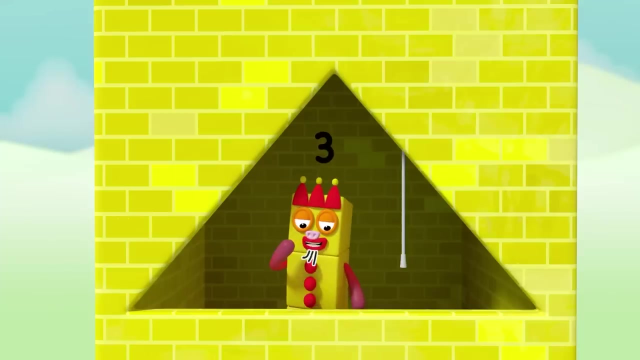 Two's company and three's a party. Oh, Keeping that big bad square out is as easy as one, two, three. Little pig, little pig, let me in, Let me in, Not by the three hairs on my chinny-chin-chin. 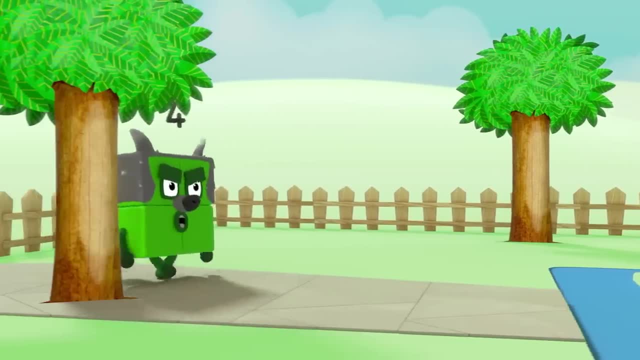 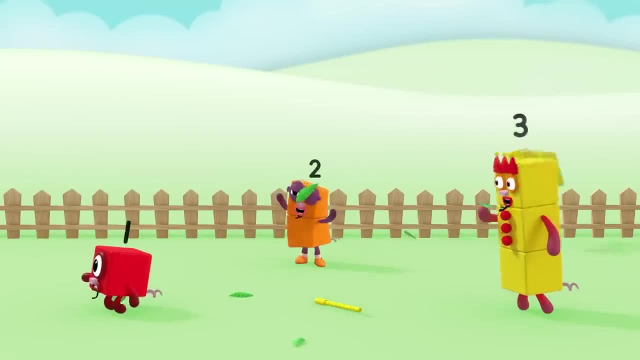 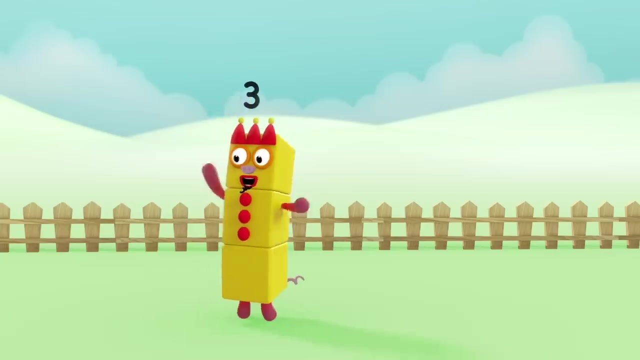 Then I'll huff and I'll puff and I'll blow your house in GASP POOF, POOF, OUCH, OUCH, What, But how? Just a little huff, GASP POOF. 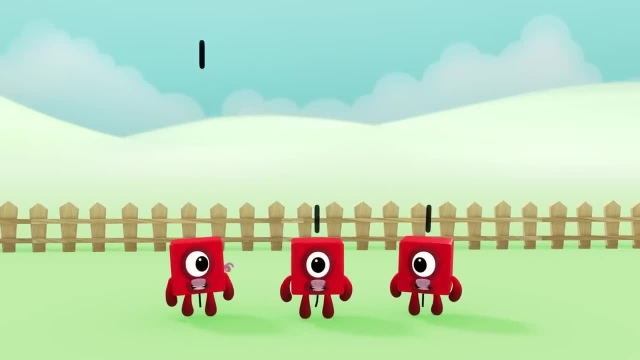 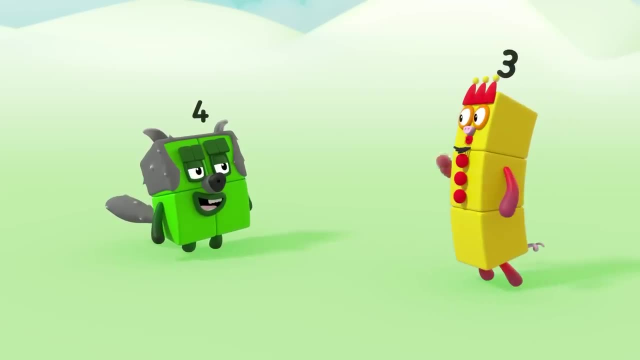 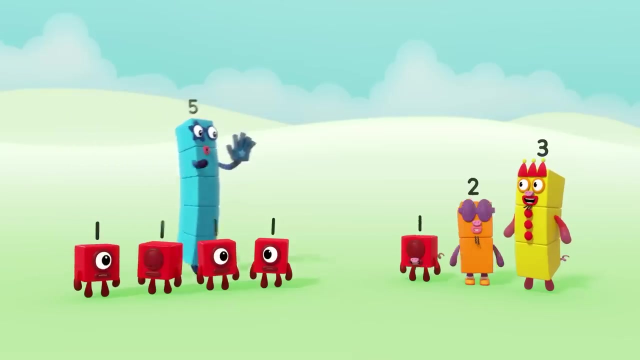 OUCH, GASP. Hey, One plus one plus one Plus one Equals three. See how you like it. GASP, GASP, OUCH, OUCH, OUCH. Stop. This isn't how the story goes. 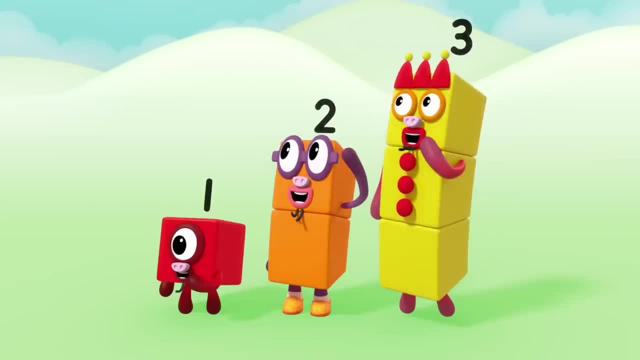 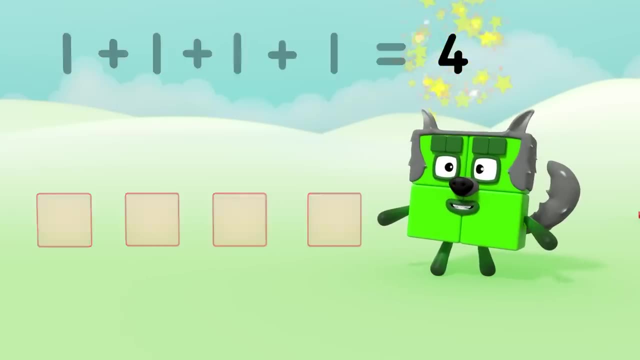 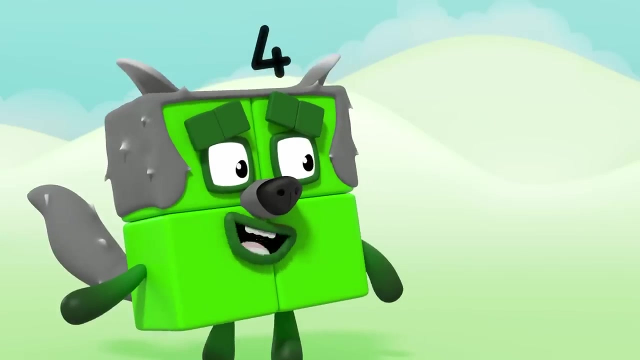 The third house doesn't get blown down. OUCH, One plus one plus one plus one equals Four GASP. No, Where will the three live? Where will the three little pigs live? now? There's always my house, GASP. 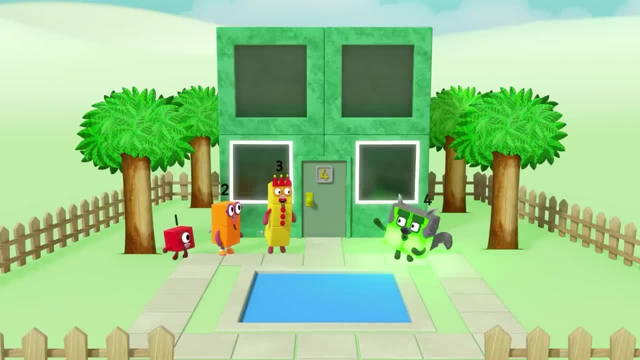 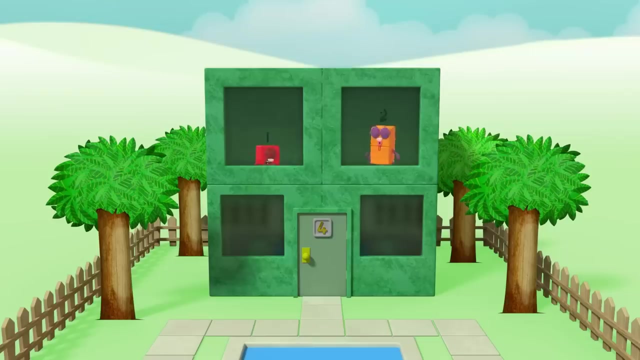 It's got four rooms With one, two, three, four, Four windows, And one, two, three, four, Four trees And a number four on the door: GASP, GASP. One, two, three, four. 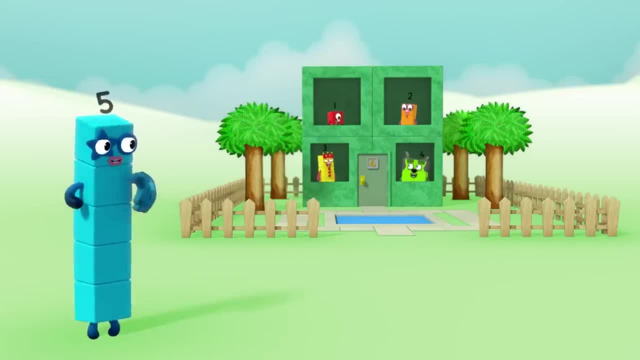 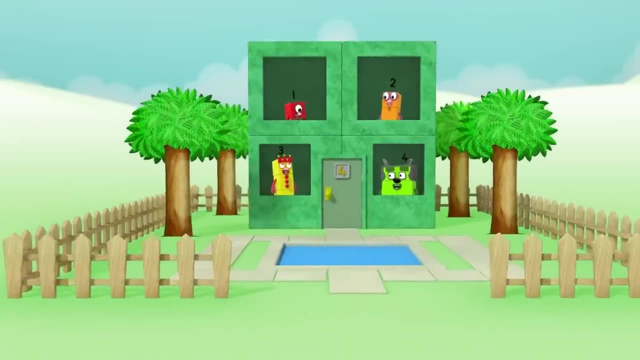 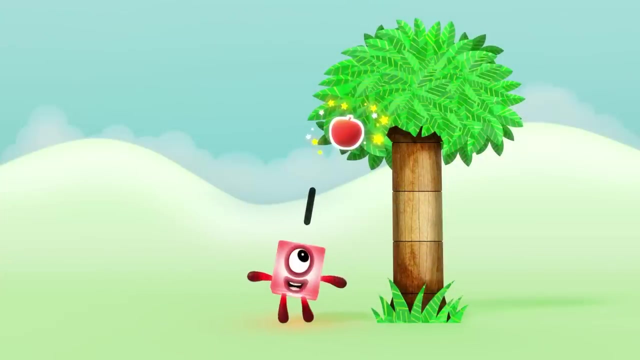 One, two, three, four, Four windows, Four farms, Two farms, One pig-hand. Once upon a time there were three little pigs And a big bad square, And they all lived happily ever after The end, YAY. 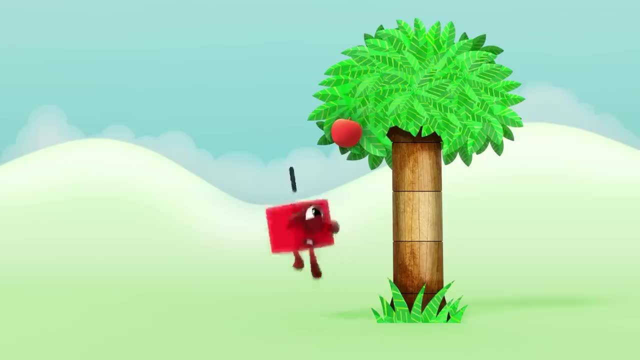 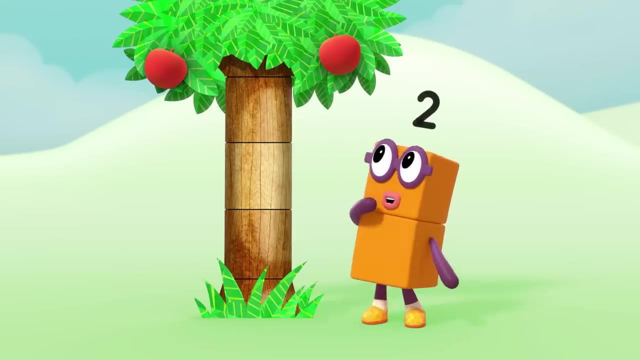 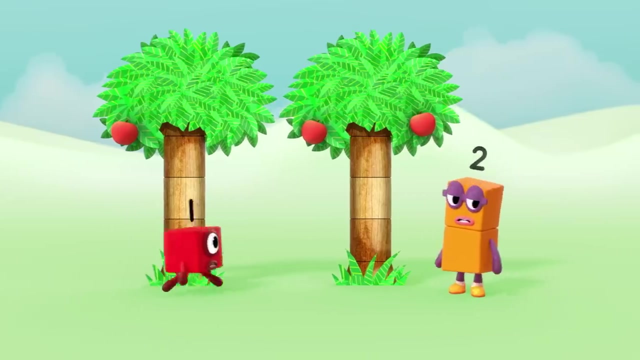 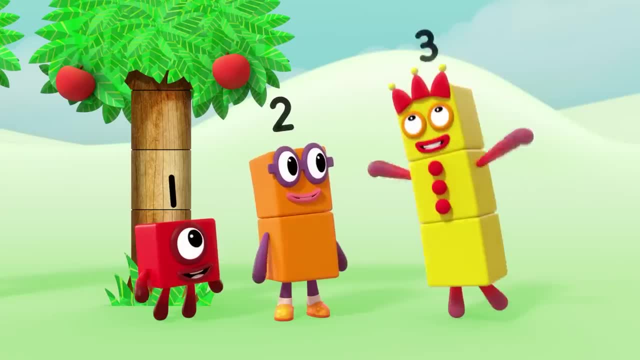 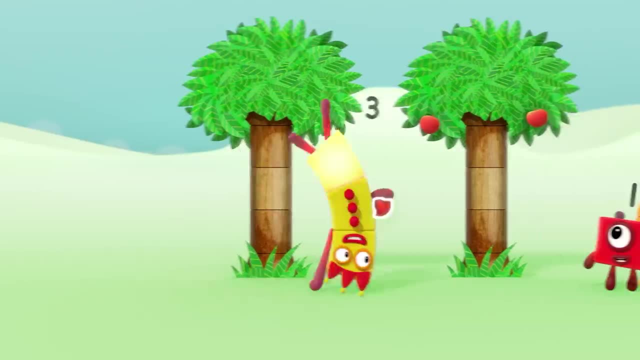 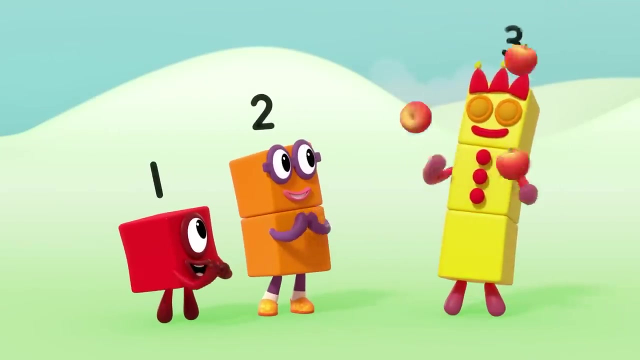 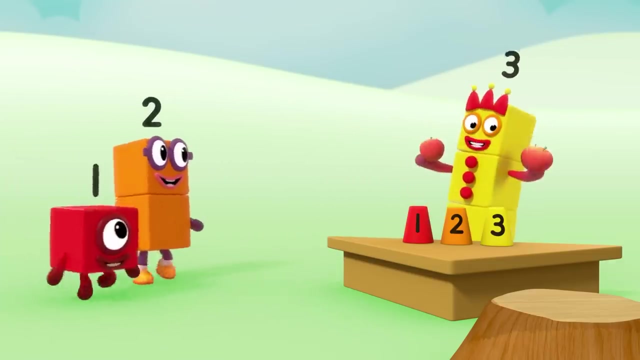 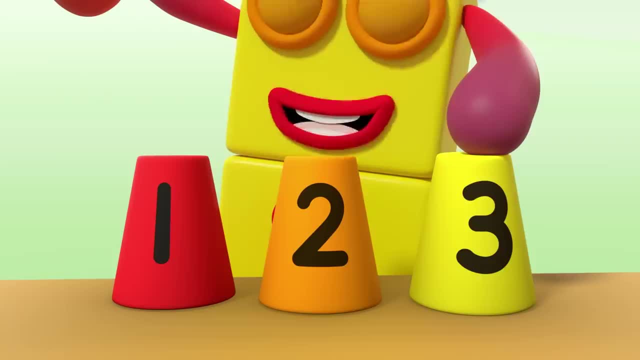 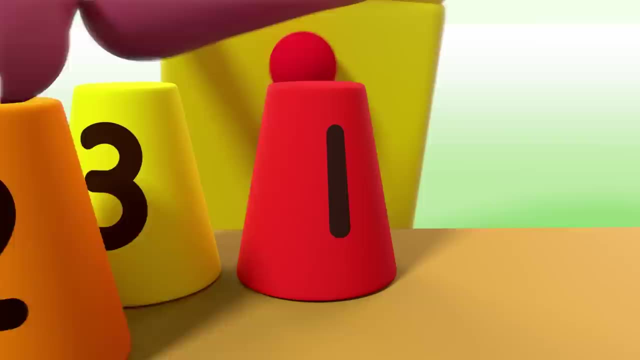 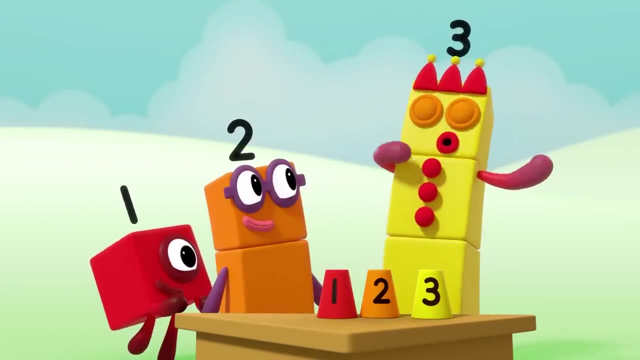 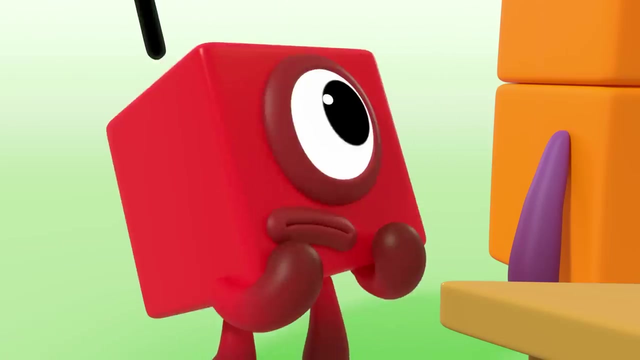 Or three, Let's play. find the apple Round and round and round, Round and round And round. Ready, steady, stop. So which cup is the apple under One? You're the first number, so you can have first guess. 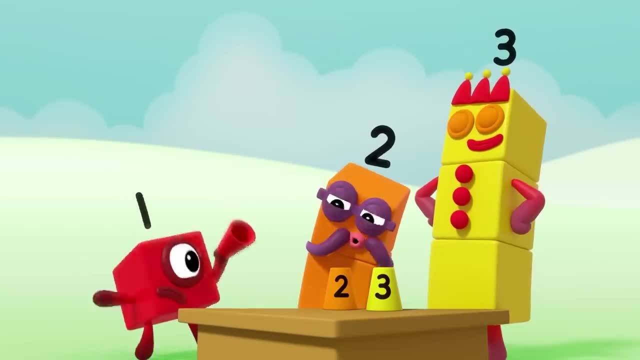 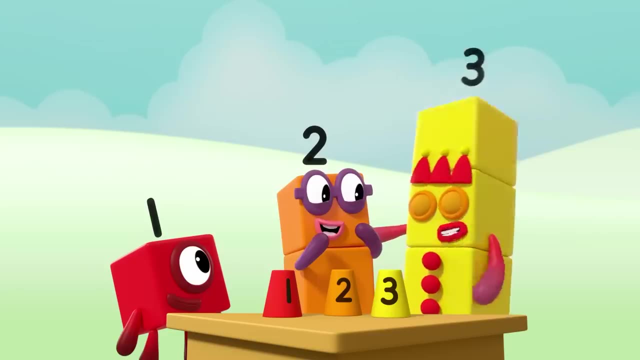 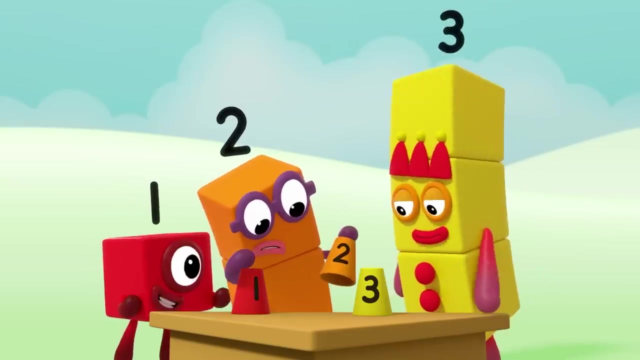 This one the first cup, Oh, Bad luck. one, Two: you're the second number, so you get second. go, Ooh, This, No, that, Ooh. Oh, My turn. Three is the third number. 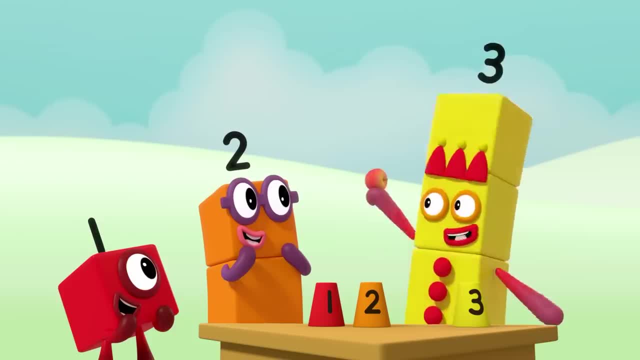 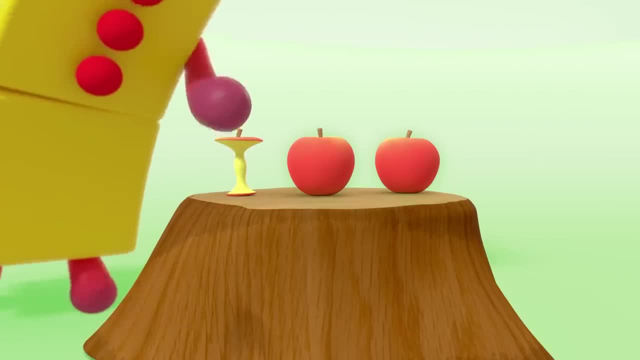 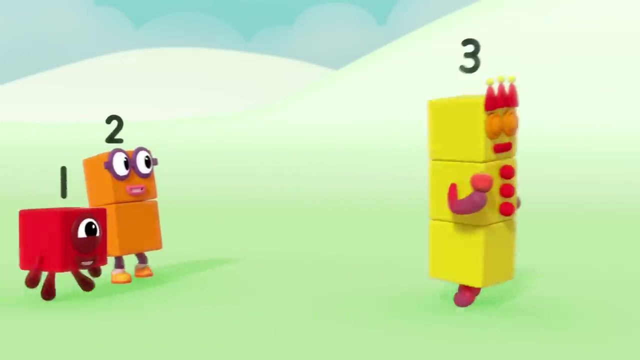 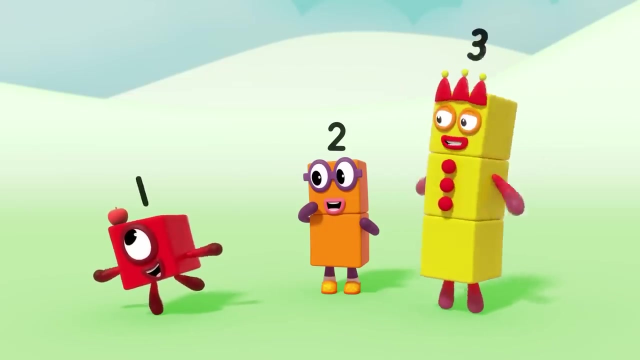 Add one, two, three, Third time, lucky, Yay, Well done. One apple gone, Two apples left, Let's play again. Let's play apple on top. Oh, Three simple rules: Apple on top, Don't let it drop. 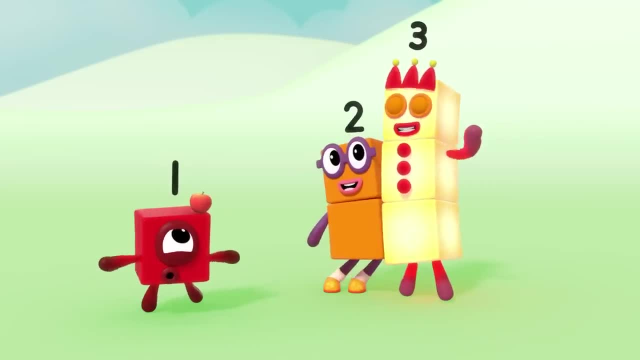 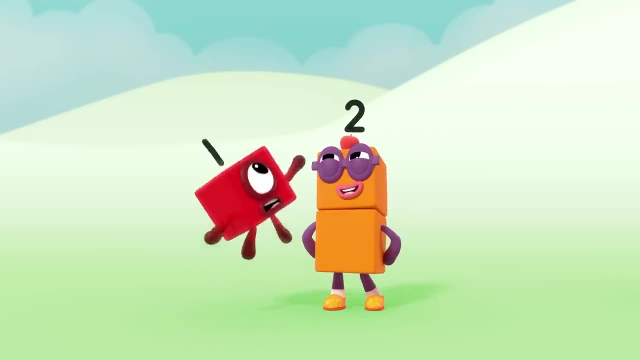 Ooh, Ooh, I can't reach. I'm smaller than you. I'm the smallest number, Then I'm bound to win. I'm bigger than you. Oops, Silly me. I'm bigger than one, but smaller than three. 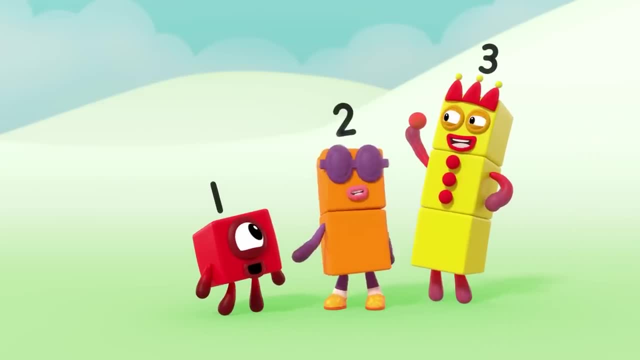 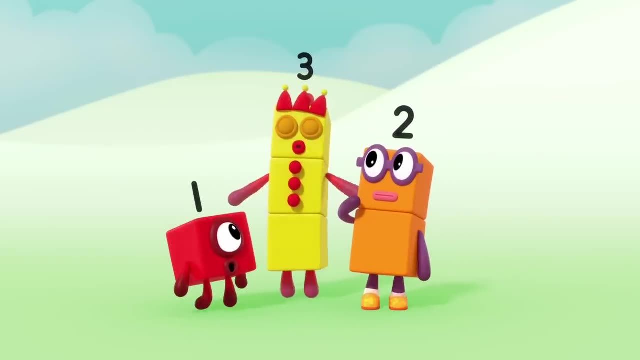 I'm bigger than both of you. I'm the biggest. So I guess I'm the biggest. I'm bigger than both of you. I'm the biggest. So I guess I win again. One, two, three, Two apples gone. 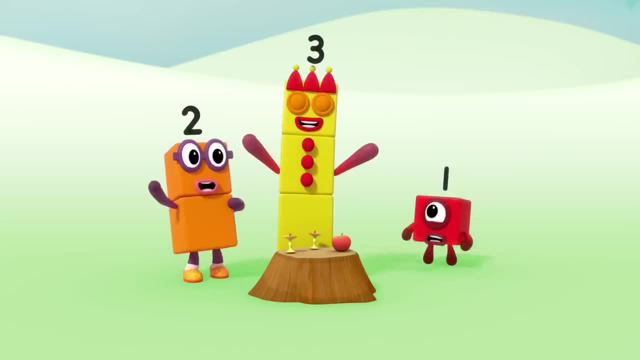 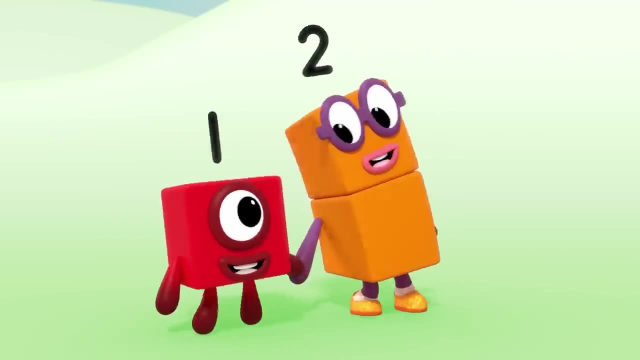 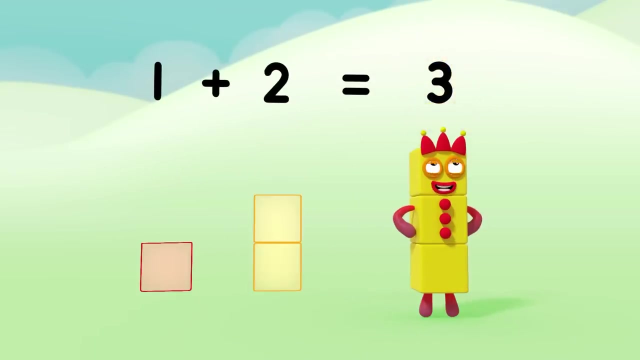 One apple left. Surprise. It's the final game. The biggest surprise wins: One plus two. Two equals three. One, two, three, Three equals Two plus one. Wow, But how Very good, You win best surprise. 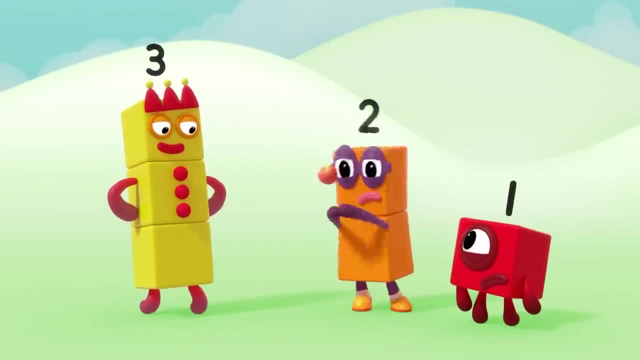 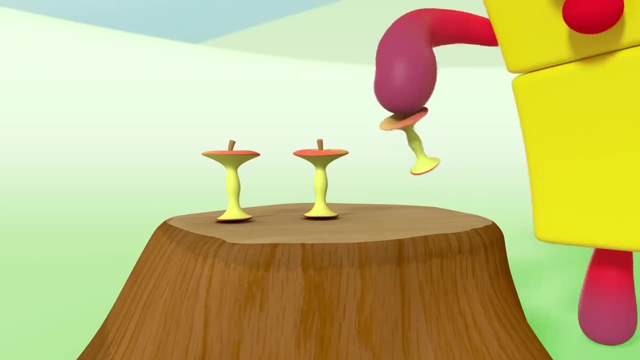 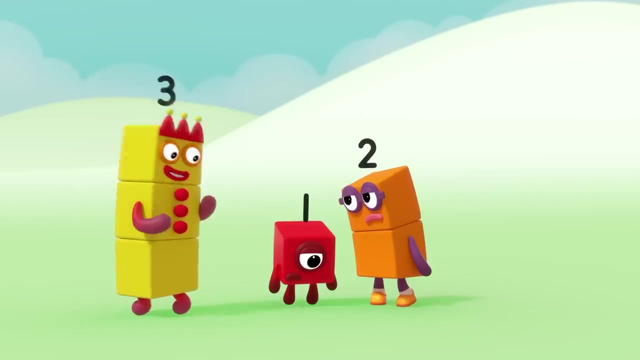 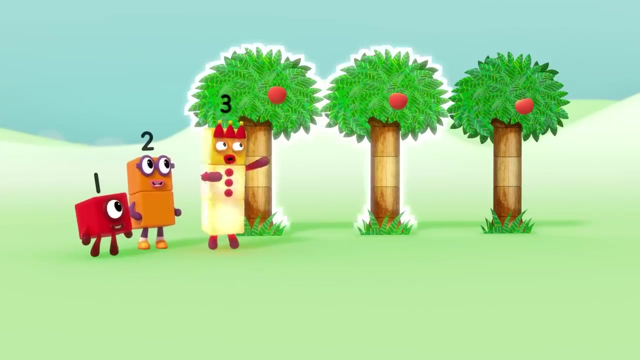 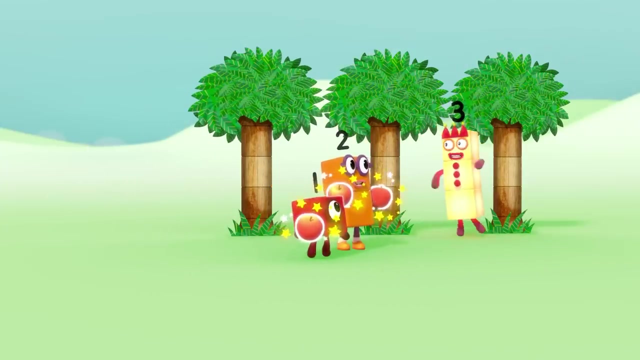 Three. One, two, three, All for me. Oh, That was the last one. Don't be sad, Don't be mad, Be glad. One, two, three, Three trees With one, two, three, Three apples. 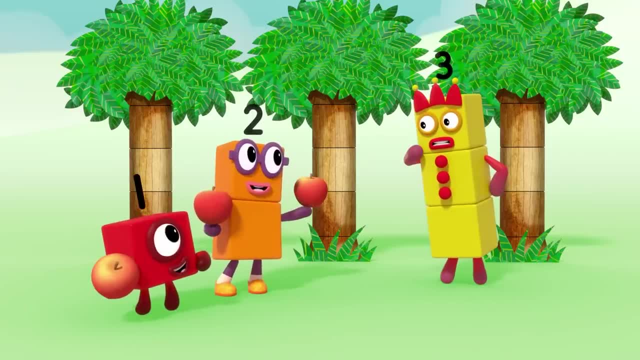 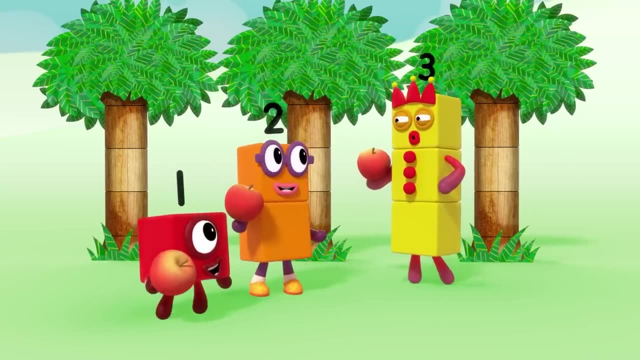 One for me and two for me. Two for me and two for me. I've already eaten three. I don't mind sharing. I've already eaten three. I don't mind sharing. Thank you two, Thank you two. Now for my final trick. 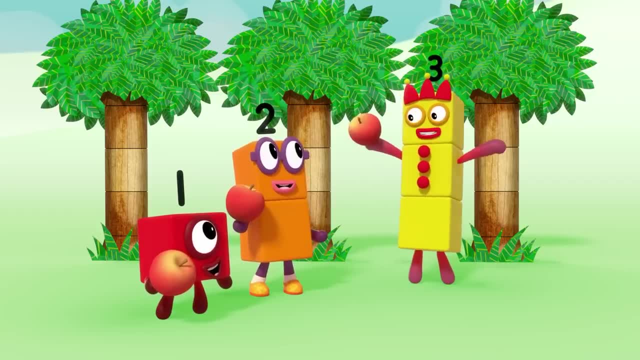 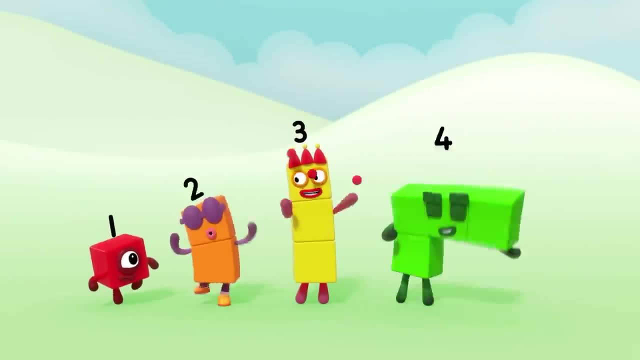 Now for my final trick. Let's make these apples vanish. One, two, three, One, two, three, Two for me and two for me. One, two, three, Two for me and two for me. I can do my exercises. 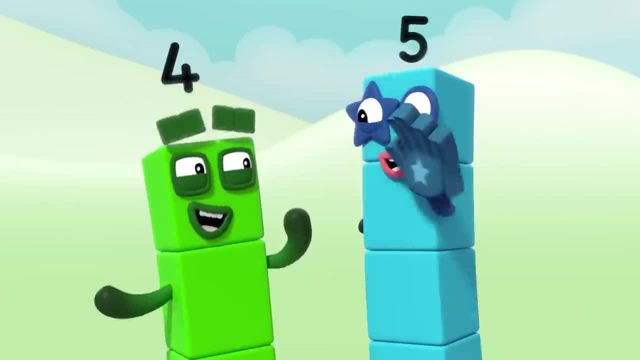 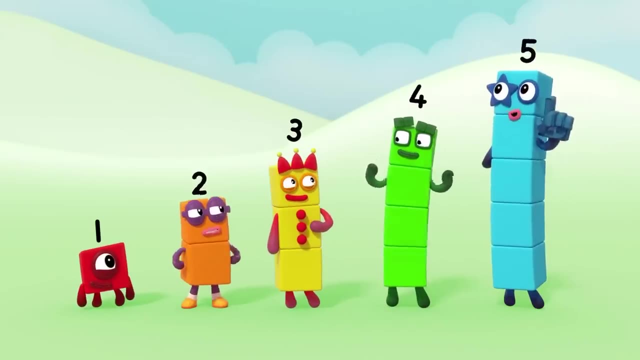 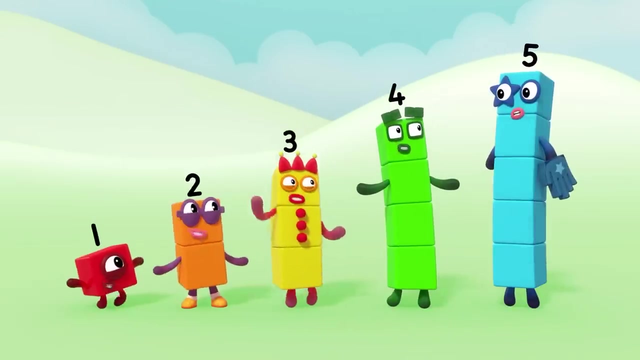 Hi team. So are we all here? Um Well, how can we tell? I know just the thing: Ready, steady, sing One, two, three, four, five. That sounds right. What shall we do today? 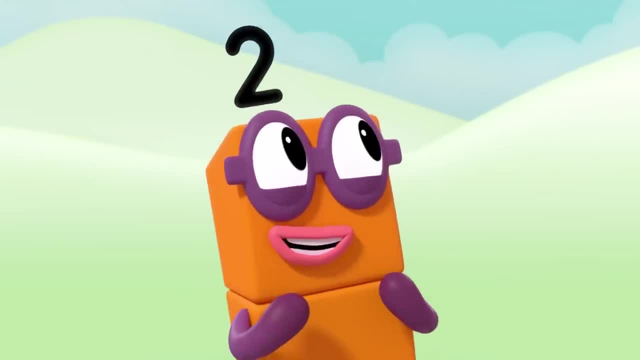 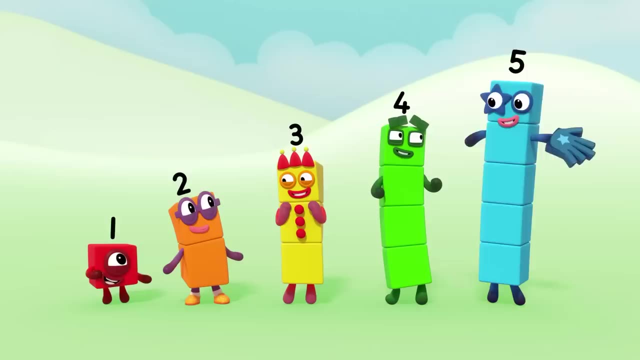 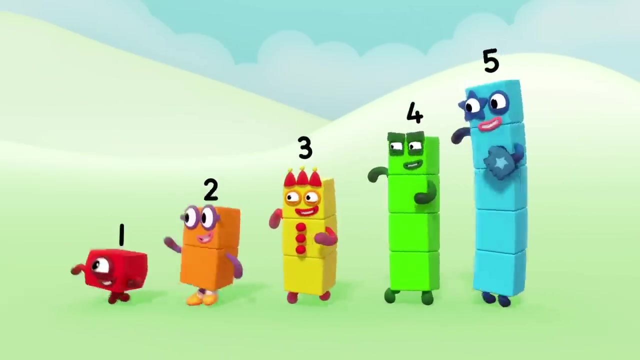 Walk in the sunshine, Run through the forest, Climb to the top of a tree, Pretend to be pirates, Discover a whole new world. Let's have an adventure. Hooray, Everybody ready? Off, we go Off, we go on a big adventure. 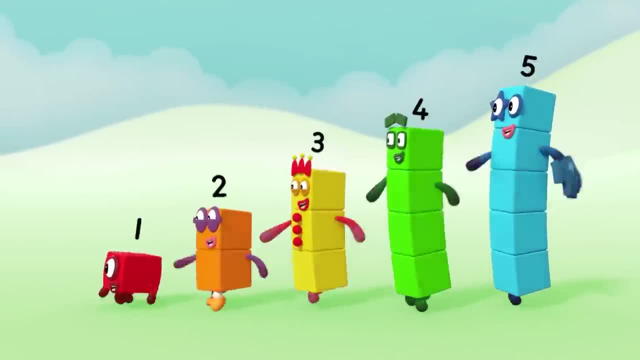 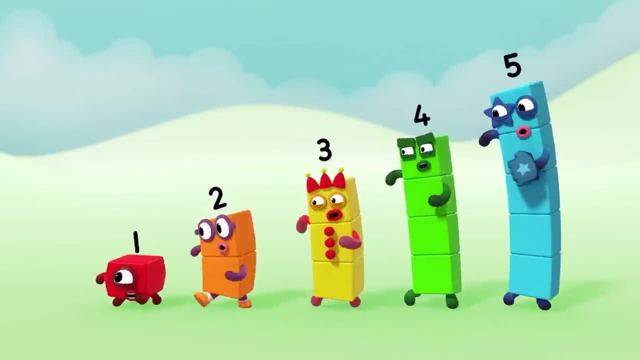 We don't know what the day will bring. Off we go on a big adventure, Ready, steady, sing One, two, three, four, five- That sounds right. And off we go again. Off we go on a big adventure. We don't know what the day will bring. 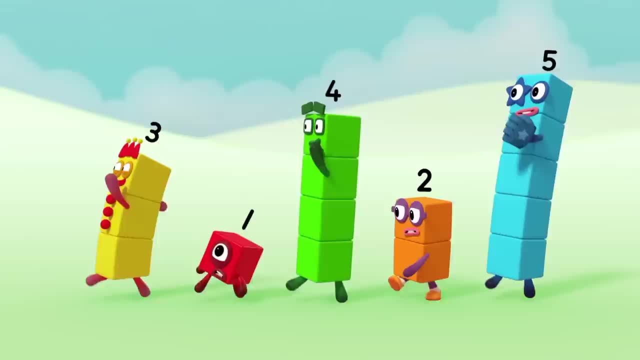 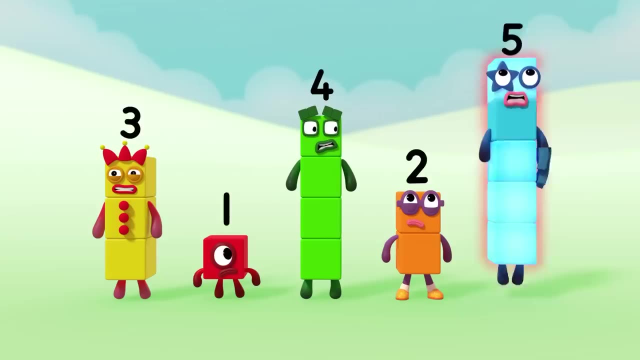 Off we go walking in the sunshine, Ready, steady, sing. Wait Too short, I can't see. Three, one, four, two, ah, That doesn't sound right. We're in the wrong order. I know what to do. 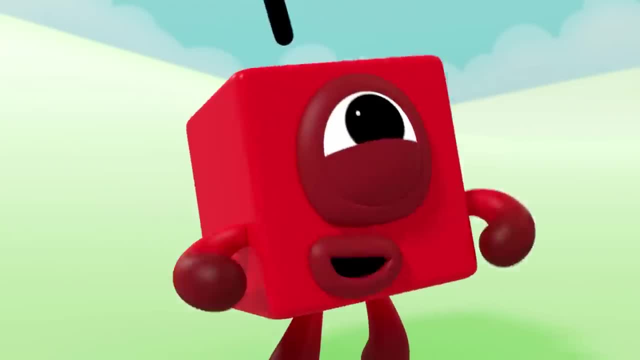 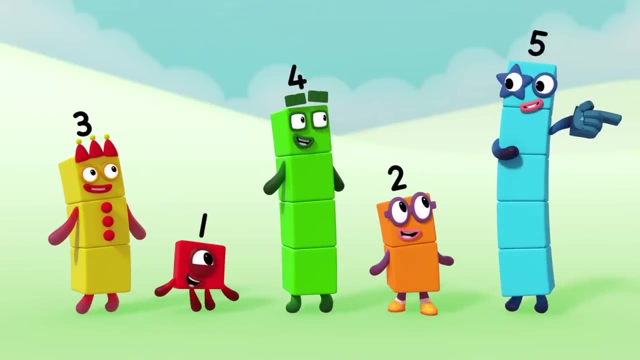 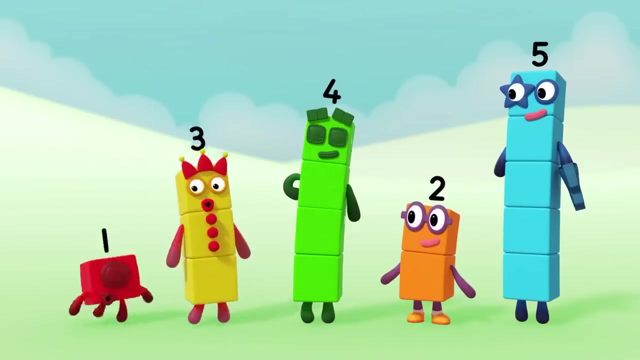 Diddly diddly do. Smallest that way, Biggest this way Go. I'm bigger than you. I'm smaller than you. Diddly diddly do. I'm bigger than you. I'm smaller than you. 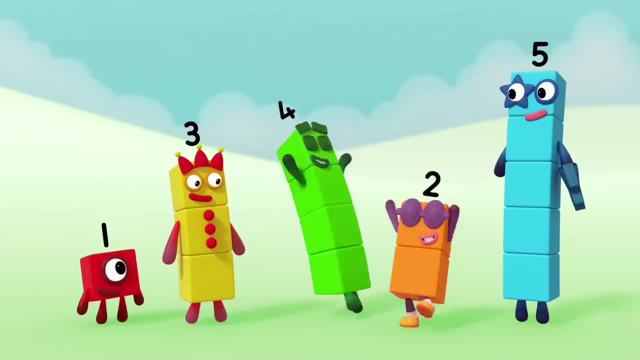 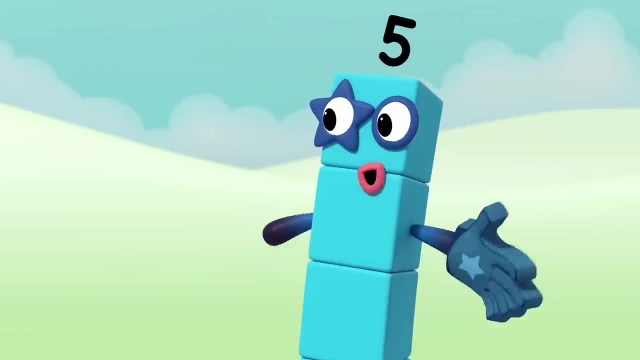 Diddly diddly do. I'm smaller than you Diddly diddly do. I'm bigger than you. I'm smaller than you Diddly diddly do. Are we all in order? 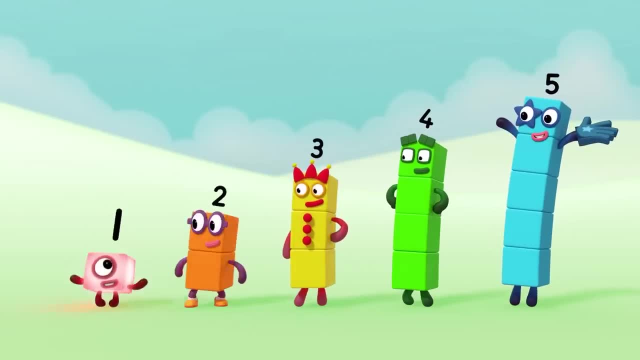 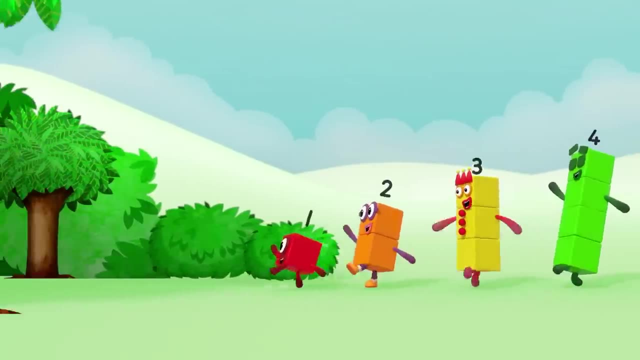 Did we all do the right thing: Ready, steady, sing One, two, three, four, five. That sounds right. And off we go, again Off we go on a big adventure. We don't know what the day will bring. Off we go running through the forest. 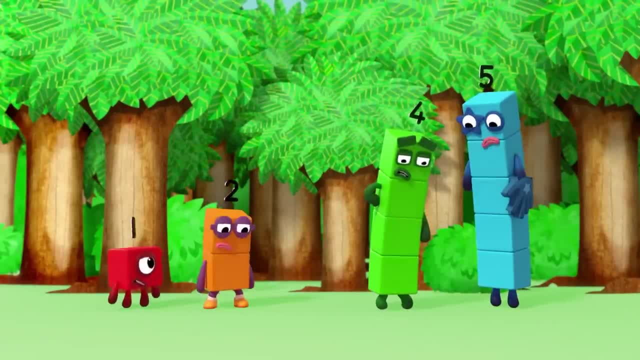 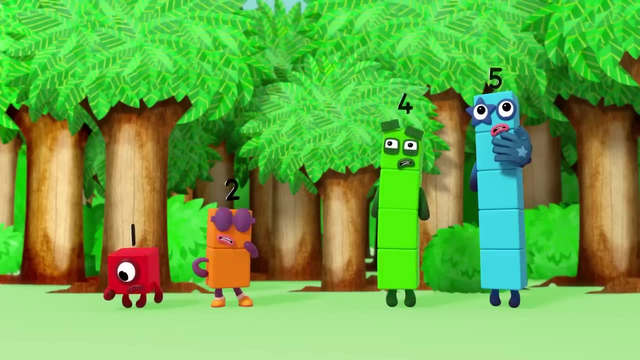 Ready steady sing, Ready steady sing. One two, three, four five. One two, three, four five. One two, three, four five. That doesn't sound right. Someone's missing. Who can it be? Let's see. 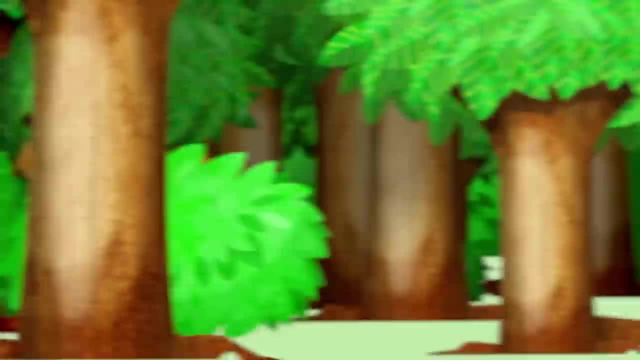 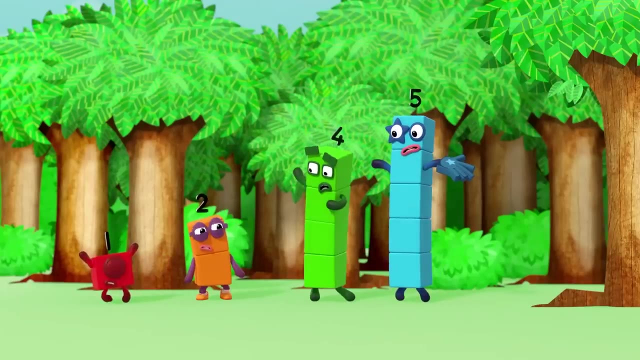 I'm one, Start with me. I'm two, I come after one. I'm four, I come after three. Three, Three's missing. Where is three? Where is three? Look at me, I'm number three, Three. 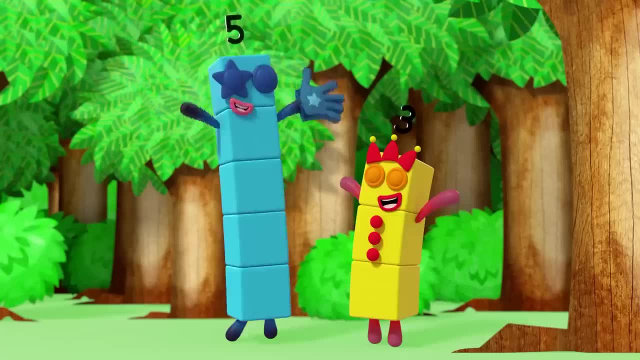 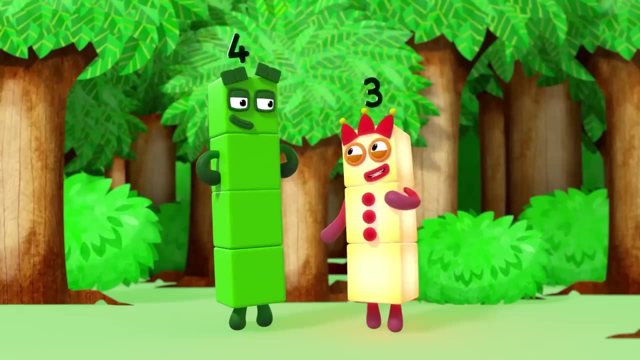 I don't know what to do. Diddly diddly doo. I'm bigger than you. I'm smaller than you. Diddly diddly doo, I'm bigger than you. I'm smaller than you. Diddly diddly doo. 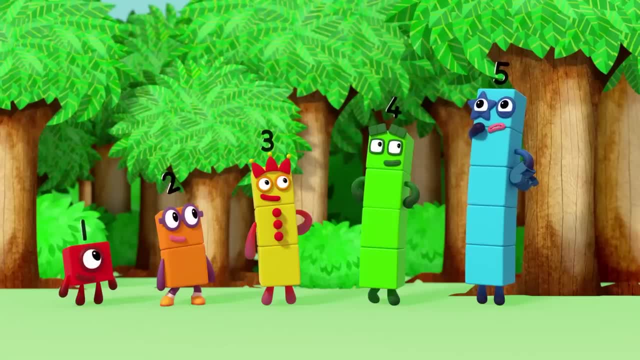 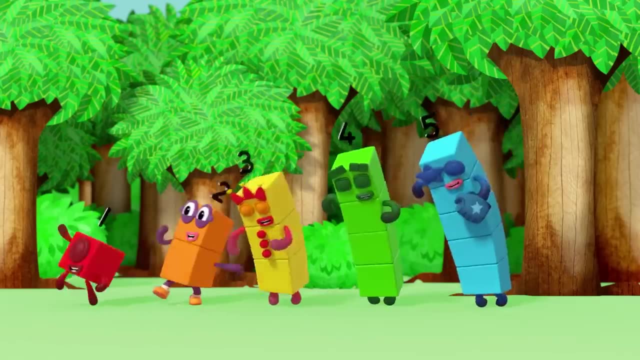 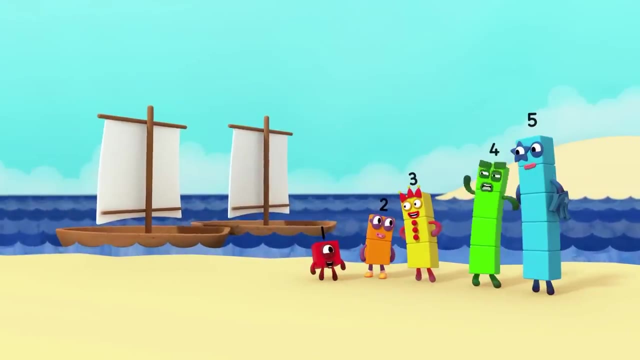 I'm smaller than you. Stop, Are we all here now? Did we all do the right thing? Ready, steady, sing One, two, three, four, five. Look One, two, two sailing boats. We can be pirates. 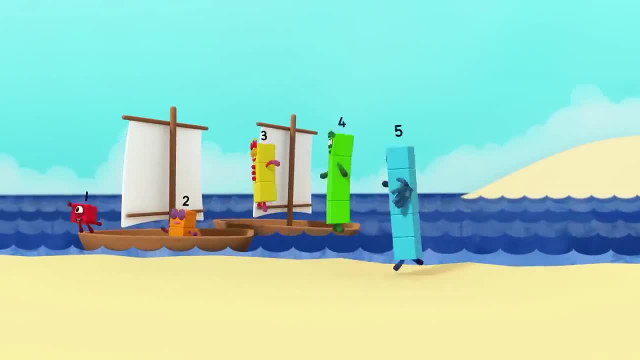 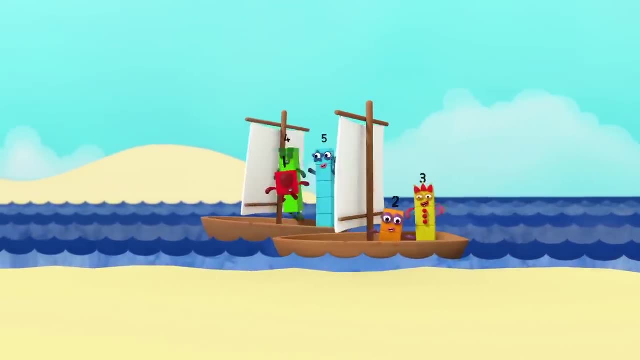 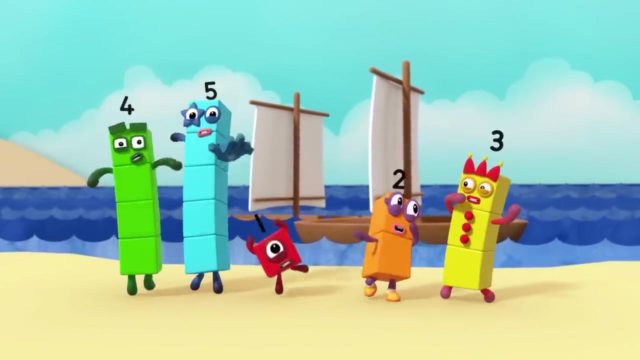 Ho ho, Off we go On a big adventure. We don't know what the day will bring. Off we go Sailing on the ocean, Ready, steady, sing Four, five, one, two, three. That doesn't sound right. 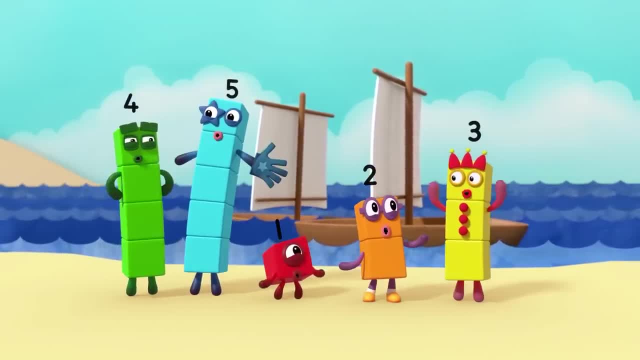 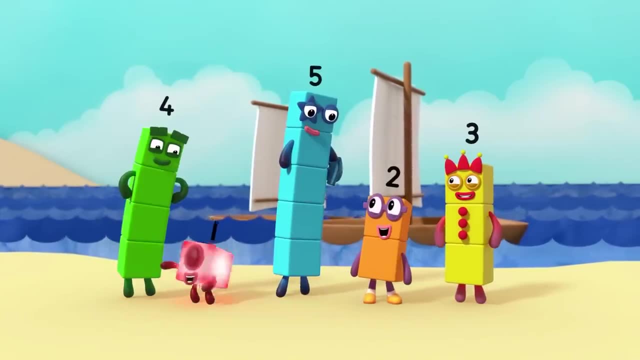 We're in the wrong order. We know what to do. Diddly diddly doo. I'm smaller than you. Diddly diddly doo. I'm bigger than you. I'm smaller than you. Diddly diddly doo. 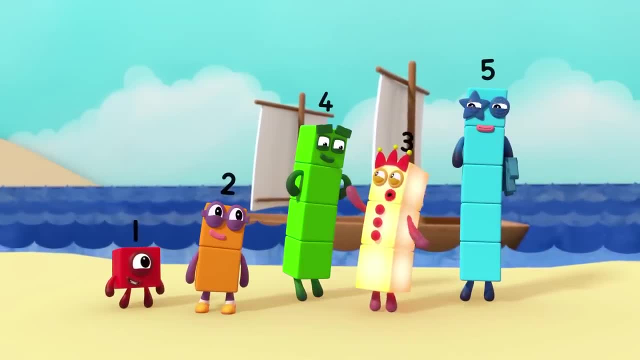 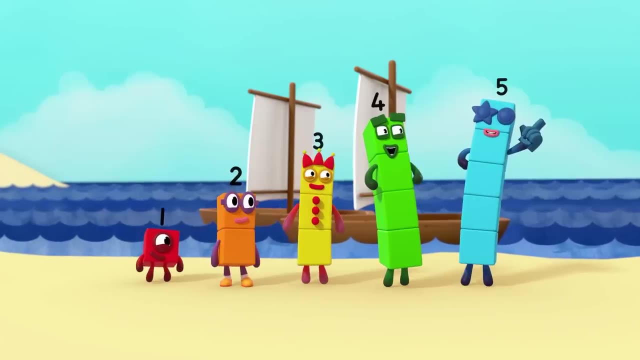 I'm bigger than you. I'm smaller than you. Diddly, diddly, doo, Stop. Are we all in order? Did we all do the right thing? Ready, steady, sing One, two, three, four, five. 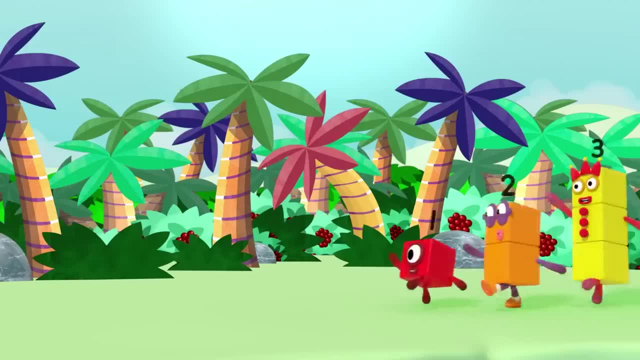 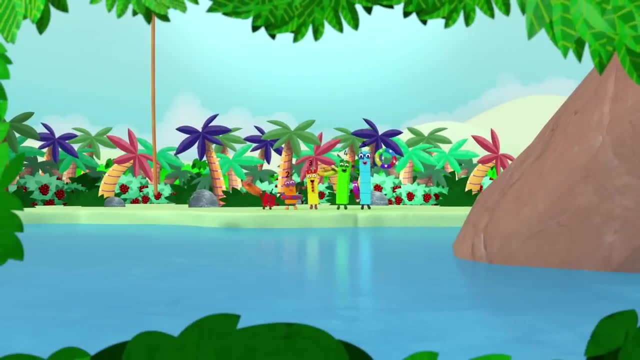 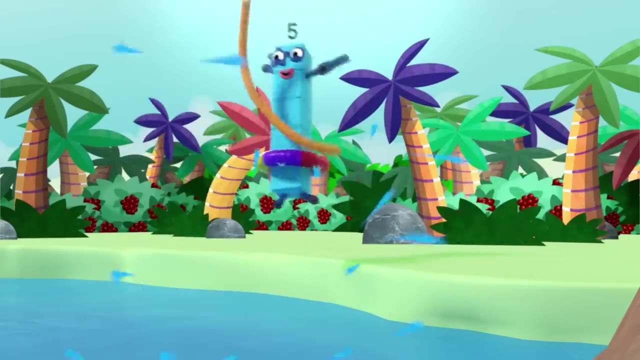 That sounds right. And off we go again, Off we go On a big adventure. We don't know what the day will bring. Bring Yay, Here we are Discovering a new world. Ready, steady, sing Yeah. 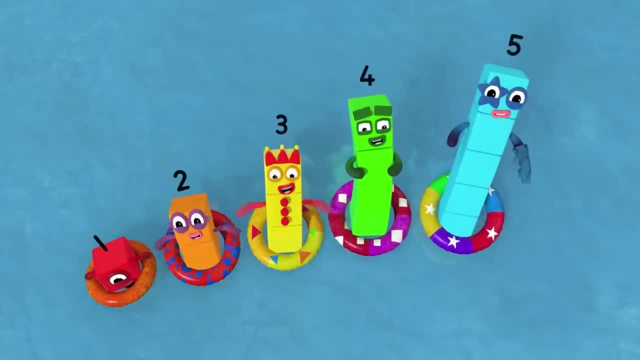 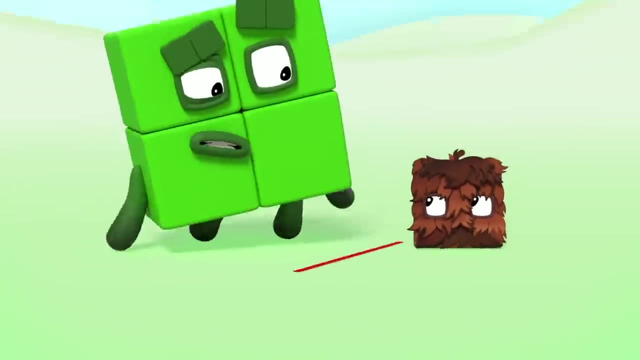 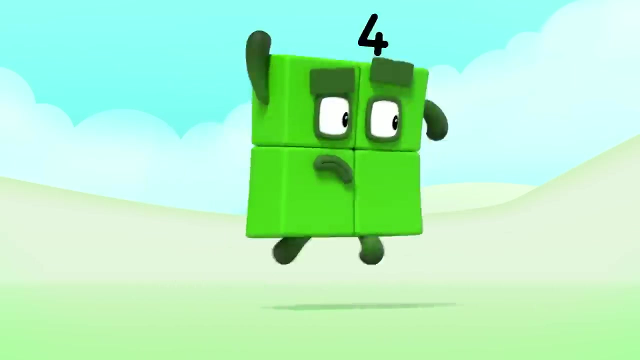 One, two, three, four, five. One, two, three, four, five. Oh, We're coming home. Hey, What is it Square? Ooh, a stick Fetch. Hey, Wait for me, Duh-duh-duh-duh. 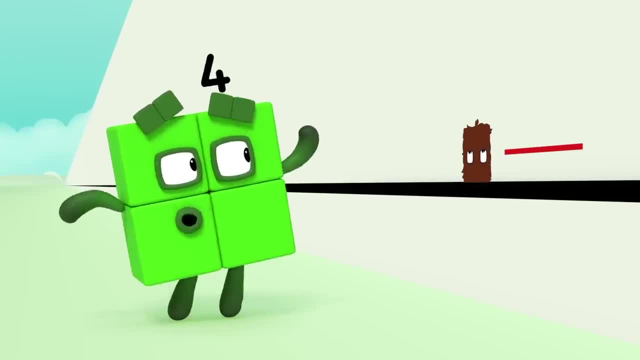 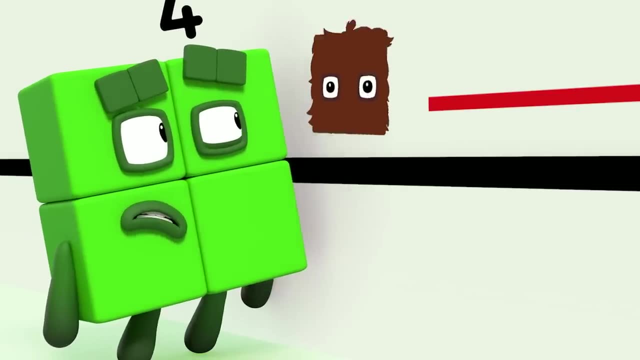 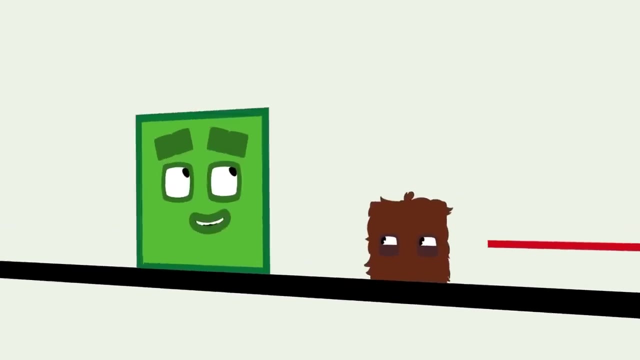 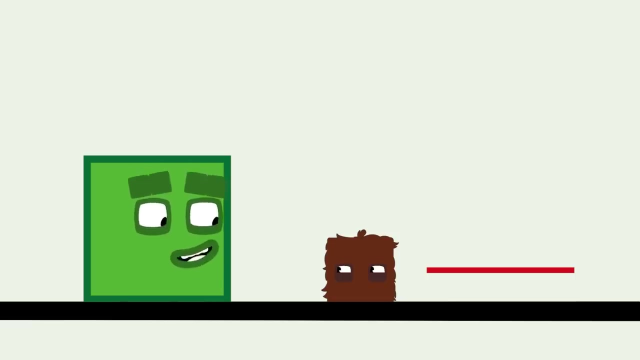 Oh, Oh, Square. Oh, You've gone all flat. Duh-duh-duh-duh, Ooh, that looks like fun. Hey, I'm all flat too. I'm a square, A real square, Ooh, squarey. 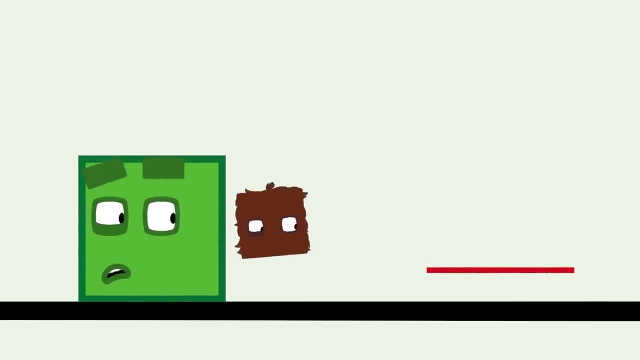 I've a feeling we're not in Numberland anymore. Welcome to Flatland, where all the flat shapes live. I am a line, One straight line, Two straight lines, And when three lines join together we make a triangle. 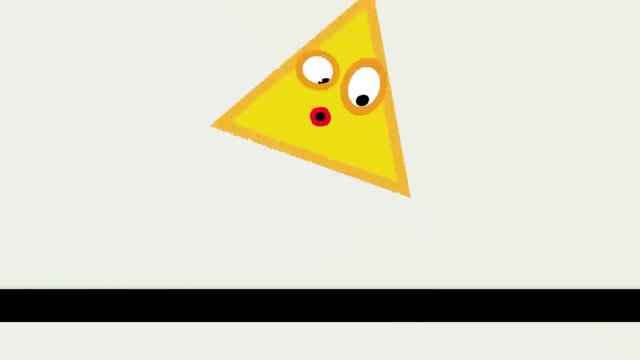 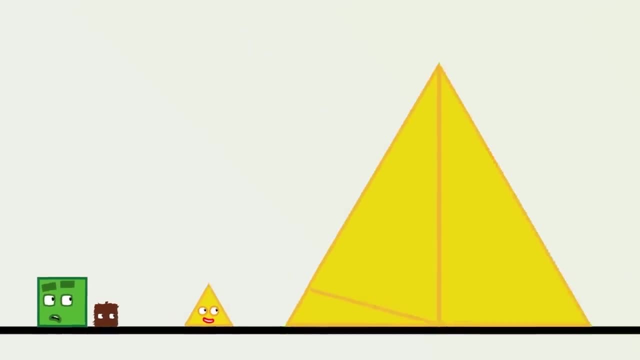 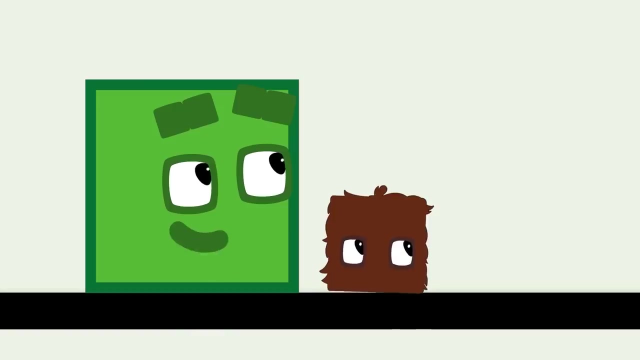 I've got one, two, three, Three sides And one, two, three, Three corners. Look at me, And at me, And at me, And at me. We're all triangles, Wow, But you're all so different. 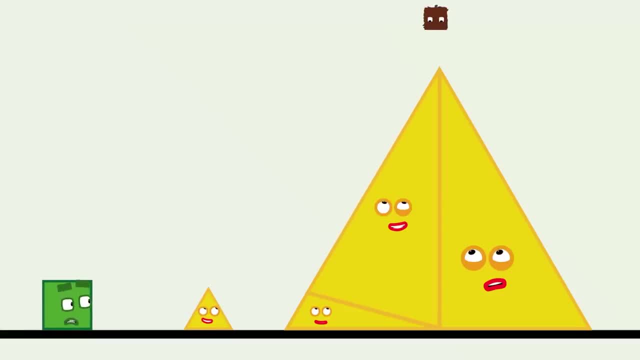 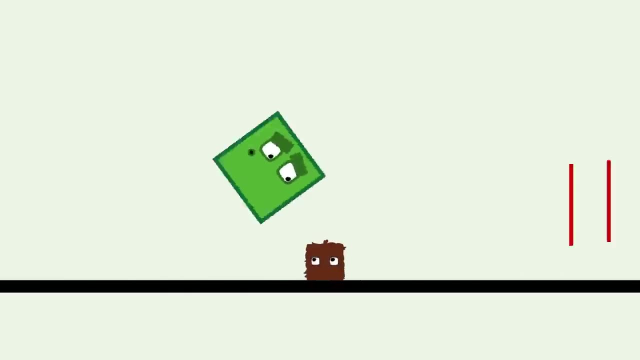 Squarey come back. Sorry, Sorry, Sorry, Really sorry Sorry. One, two, three, four, Four lines: Hello square. Wait, You're not a square, No, I'm a rectangle. Like you, I have four sides and four corners. 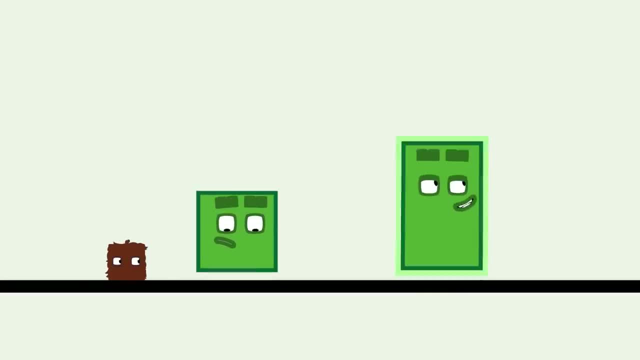 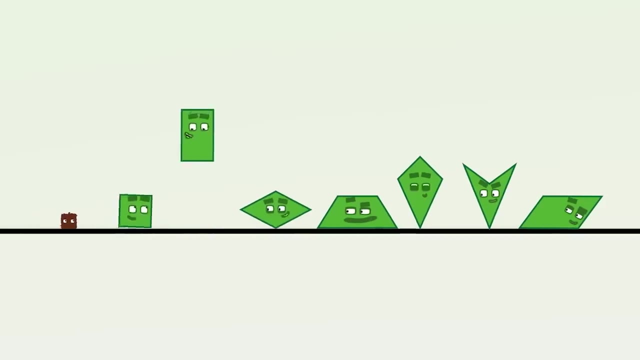 But your sides are all the same And mine are not, If I'm a surprise. wait until you meet the others. Hello Four-sided shapes, introduce yourselves. Rectangle, Rhombus, Trapezium, Kite, Dart, Parallelogram. 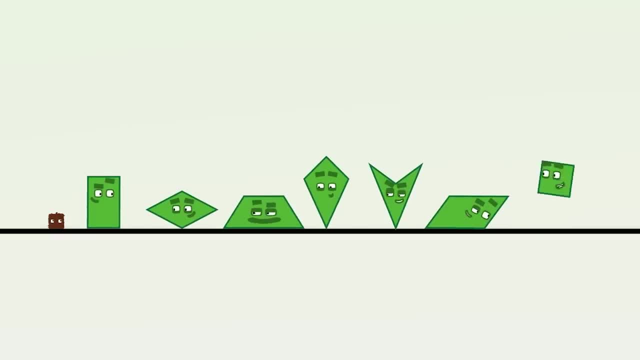 Swerve. Ooh, what wonderful names And what wonderful shapes: Rectangle, Rhombus, Trapezium, Kite, Dart, Parallelogram, Square. Ooh Squarey, come back. Oh, hello, Who are you? 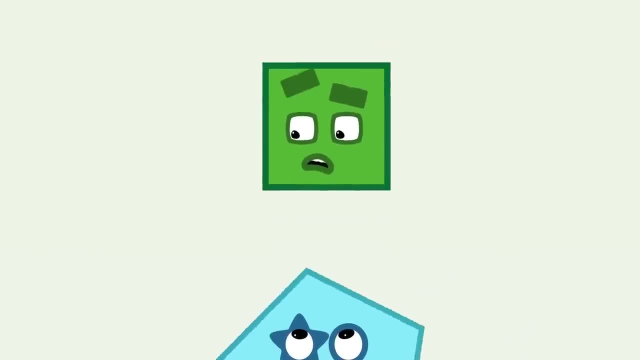 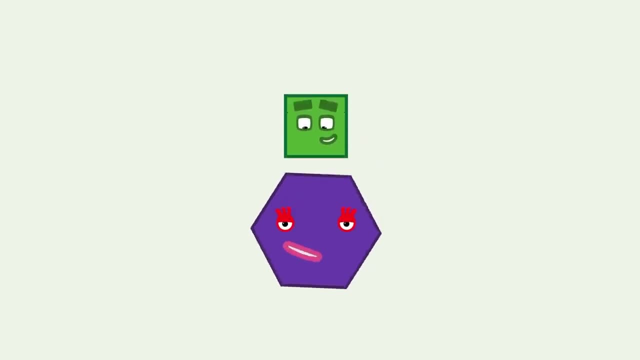 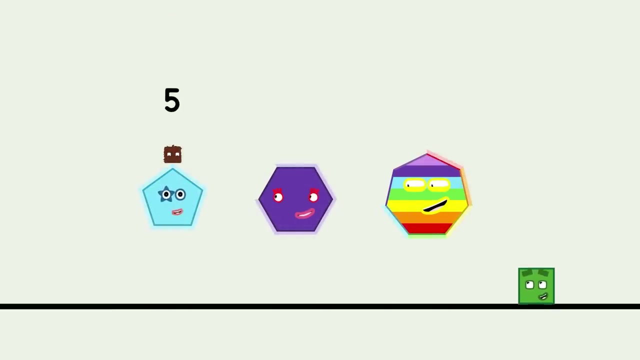 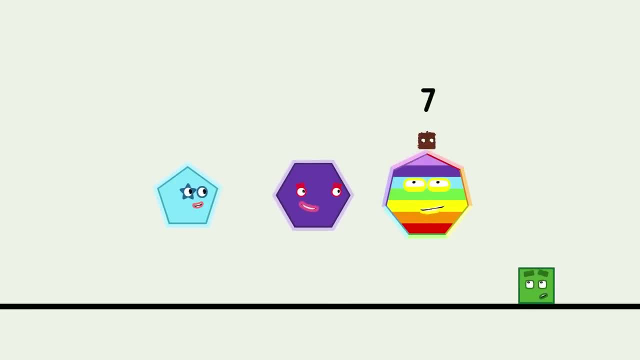 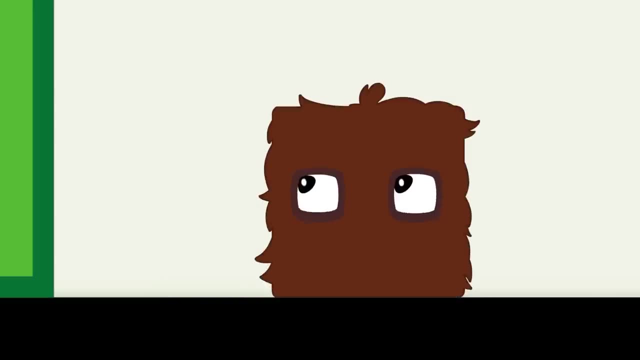 Oh, Oh, Oh No, that one, I saw that Really. What's that? It's a size and a hexagon. It's uh, Yip, yip, yip, yip, yip. What's that Squirry? 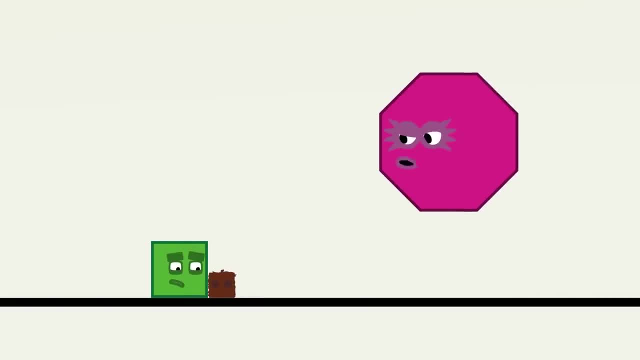 You're ready to go home? Hey, have no fear, Octagon is here. One, two, three, four, five, six, seven, eight, Eight sides. I will get you home, Octagon, make an eight-sided flying basket. 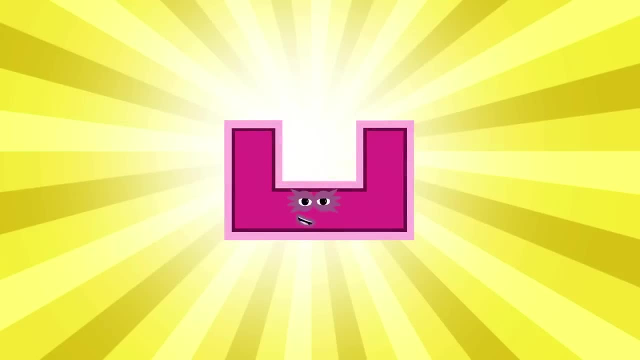 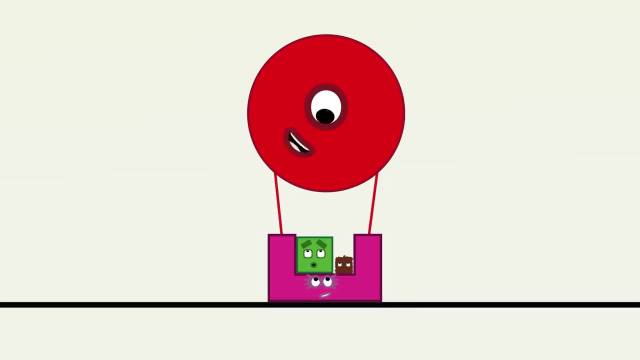 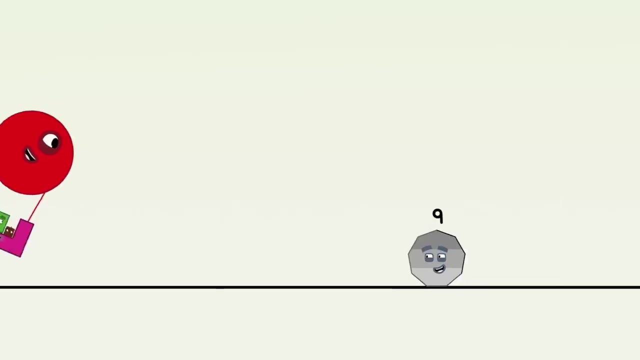 One, two, three, four, five, six, seven, eight. Basket. I'm a circle. I have just one curved edge. Hold tight folks, Here we go. Oh ho, ho, ho, hey, Ooh Wow. 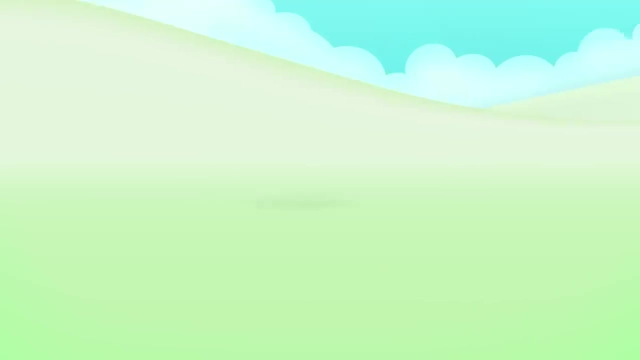 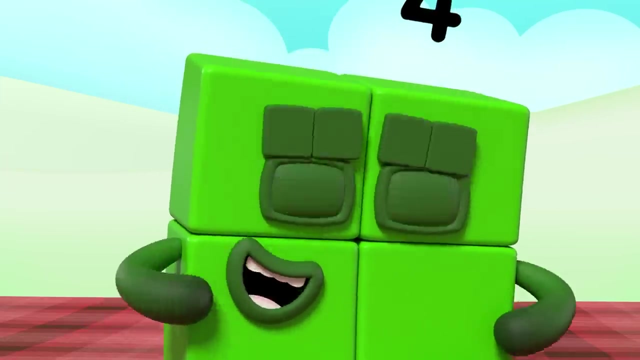 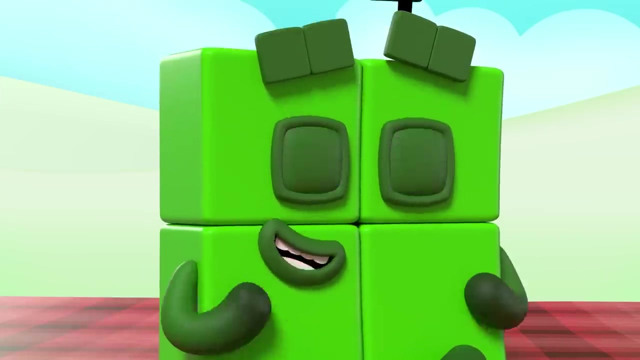 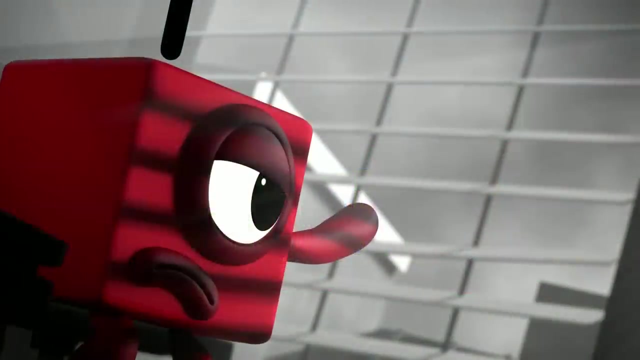 Goodbye, new friends, I'm me again And you're you. We went to Flatland and triangles were there and a rectangle and a pentagon and And I was a real square. Hooray, It was a great day in the big city. 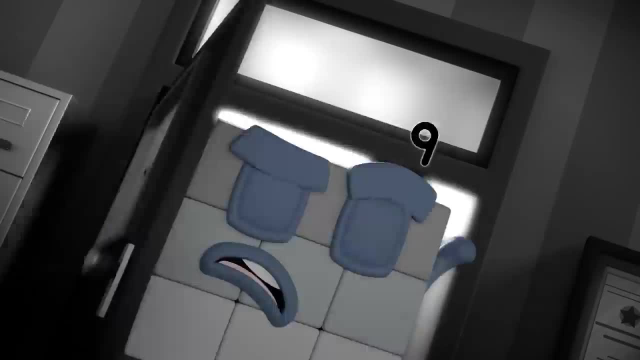 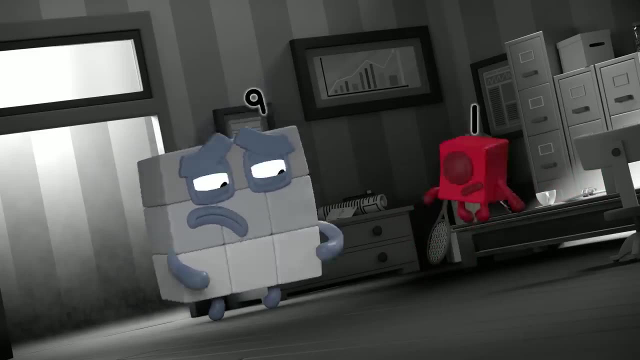 I was wondering where my next case would come from, when You've got to help me. One It's gone, Everything's gone. Slow down. Nine, Tell me what happened. I live in apartment nine on the ninth floor of numerical towers. 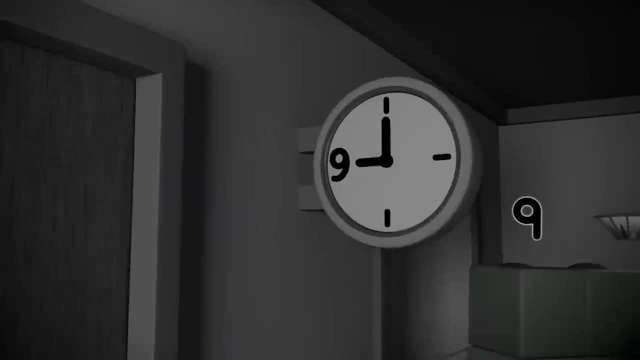 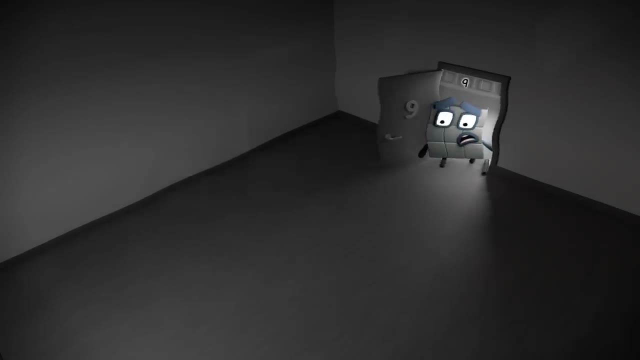 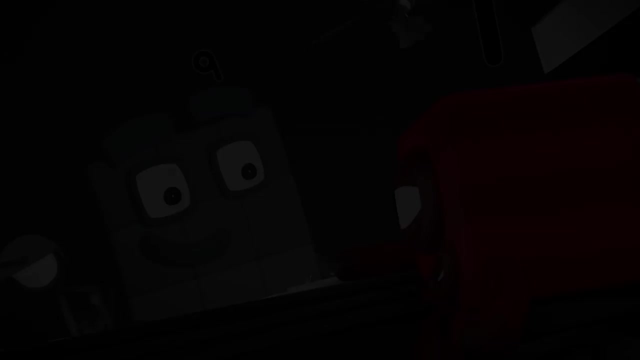 I left home this morning at nine o'clock to buy a newspaper. When I came back nine minutes later, the door was open. Everything was gone. A mystery indeed. I'll take the case. Let's look for clues. Did you notice anything strange or unusual when you got back? 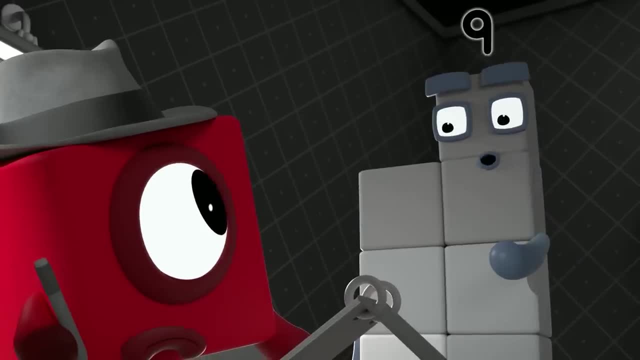 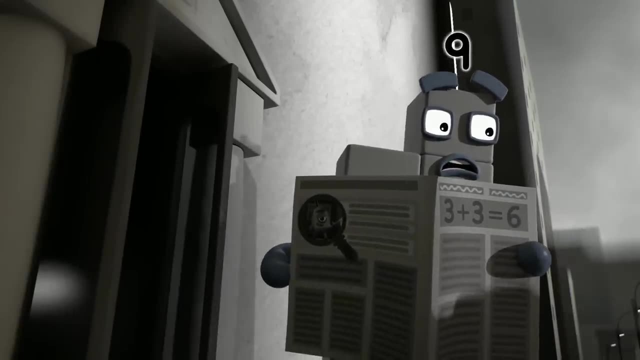 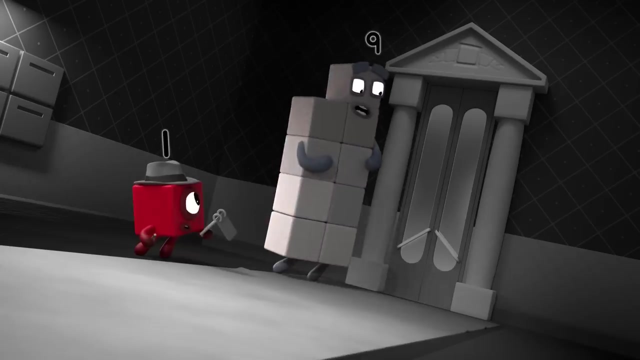 Uh, no, nothing. Oh, there was one thing: A suspicious shadowy stranger in a coat and hat pushed past me and ran out of that door, But apart from that, nothing. Can you describe this stranger? They were as wide as the door, so two blocks wide, with a flat head. 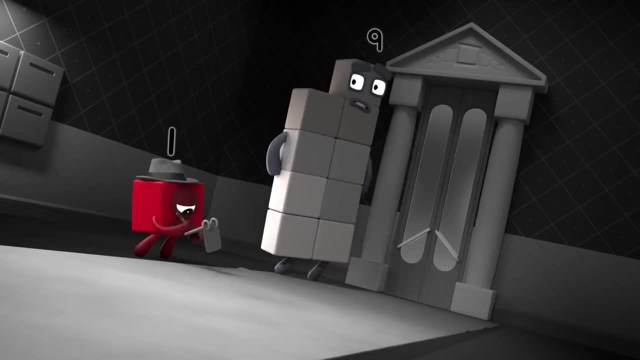 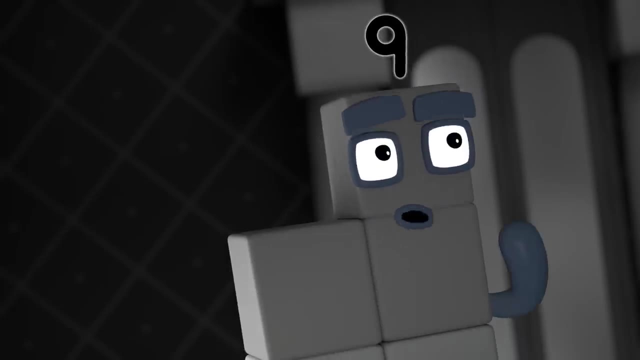 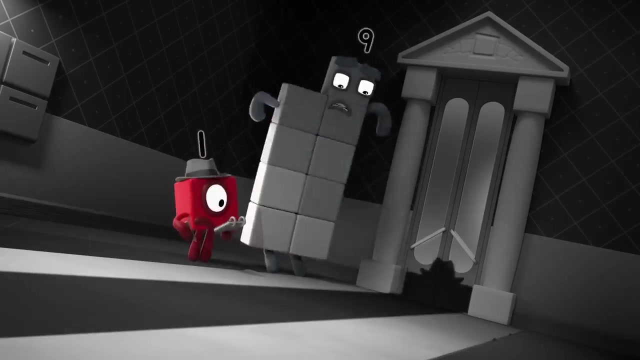 Clue one: flat head when standing two blocks wide. Anything else I could see over their head when we were both two blocks wide, so they must have been smaller than me. Clue two: smaller than nine. Look, Hat, Coat, It's them. 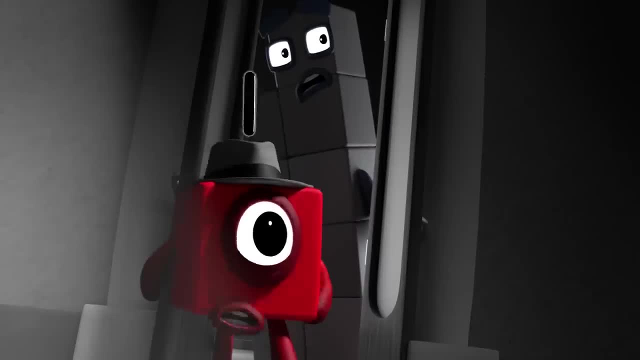 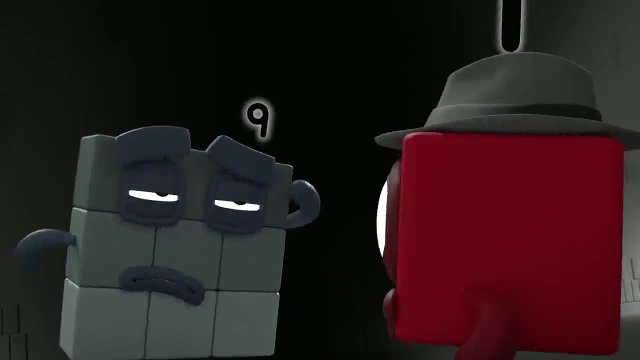 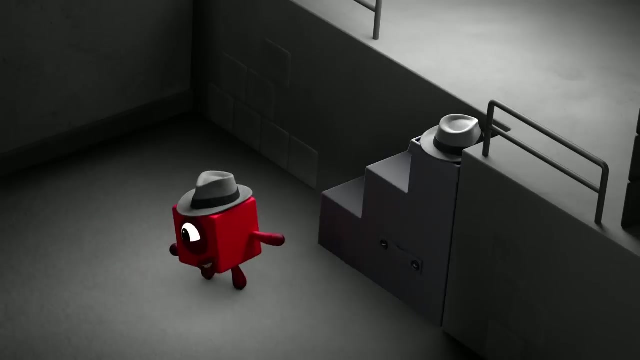 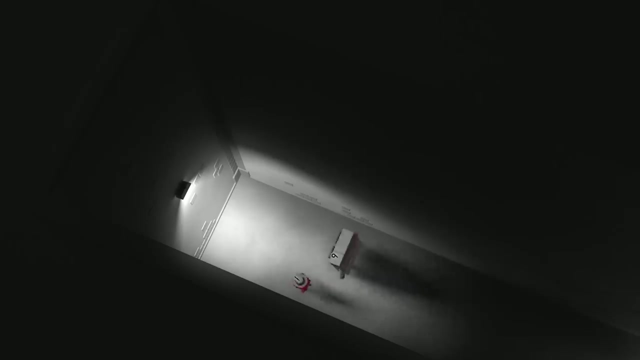 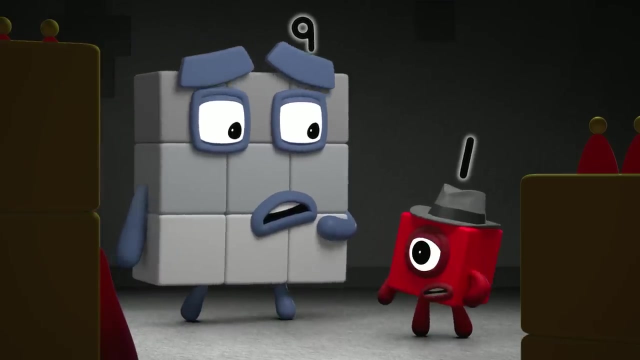 Clue three After them. quick There on the steps. The hat. These aren't steps, It's Did either of. you see a suspicious step-shaped figure in a coat and hat? No, Sorry, friend, No one else down here? 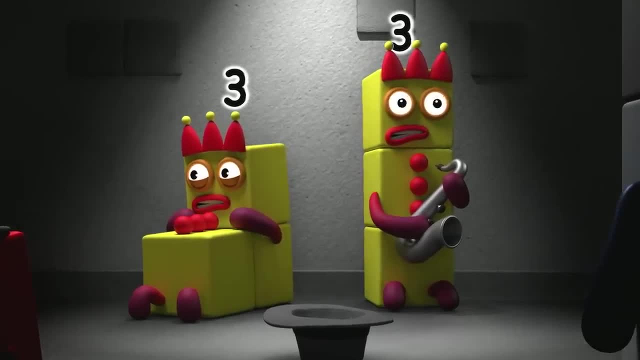 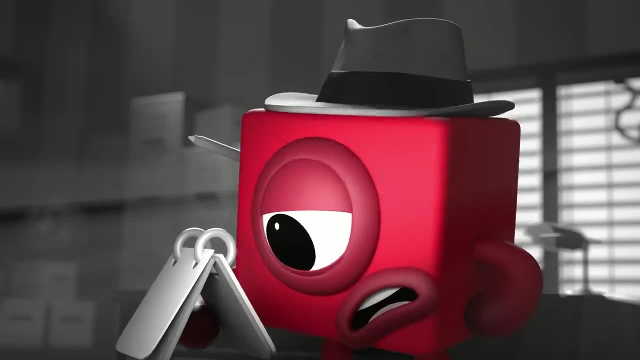 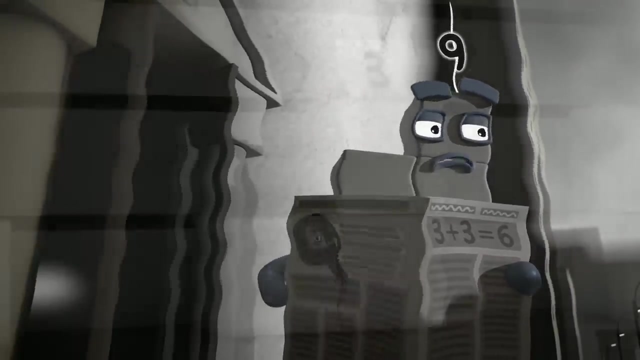 Just us. Something didn't add up, Ordid it. Let's look at what we know. Clue one: The suspect had a flat head when standing two blocks wide, So it can't have been three, five, seven or nine. 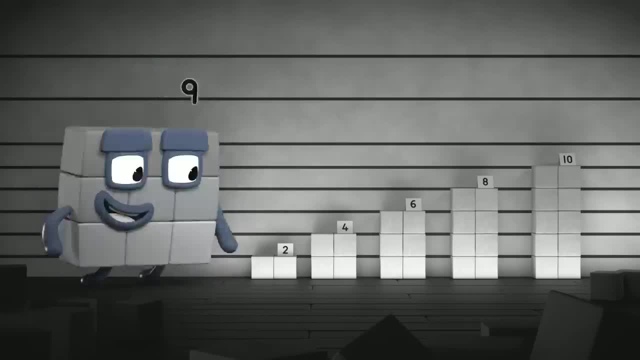 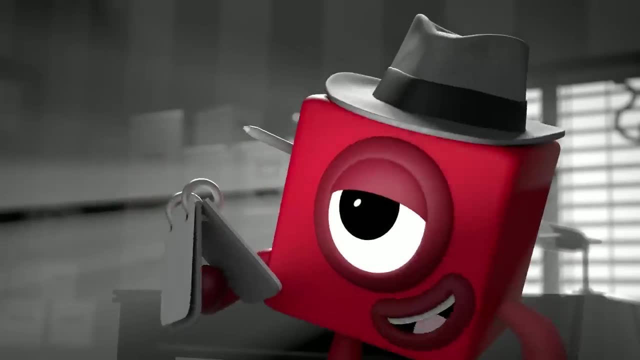 And it wasn't you, because you can't stand two blocks wide. Two, four, six, eight, ten. The suspect must be an even number. Bingo, And remember clue two. The suspect was smaller than nine, so it can't have been ten. 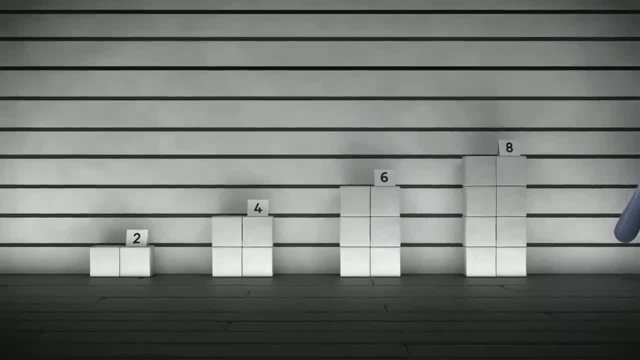 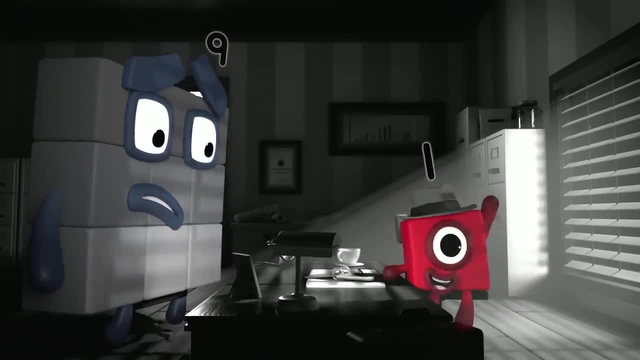 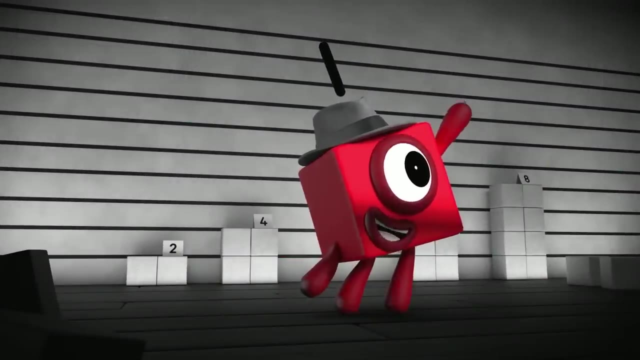 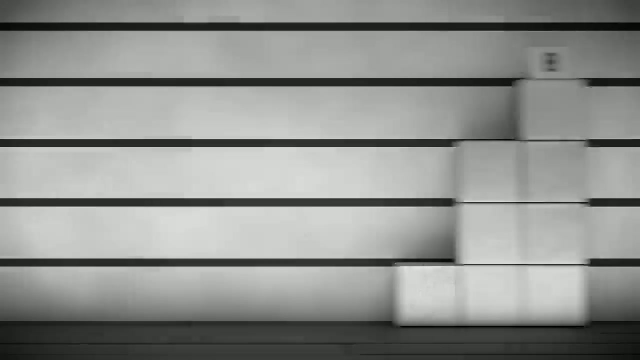 That still leaves two, four, six and eight. But which was it? Hmm, Wait, There's one more clue. we nearly forgot Clue three. The suspect can make a step shape, Not two or four or eight. 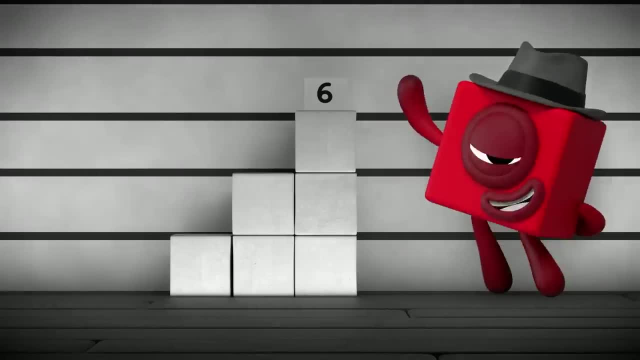 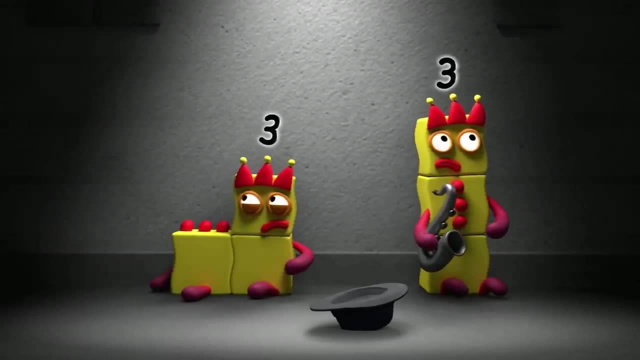 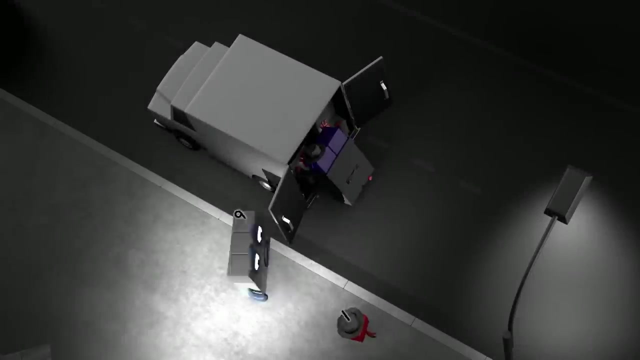 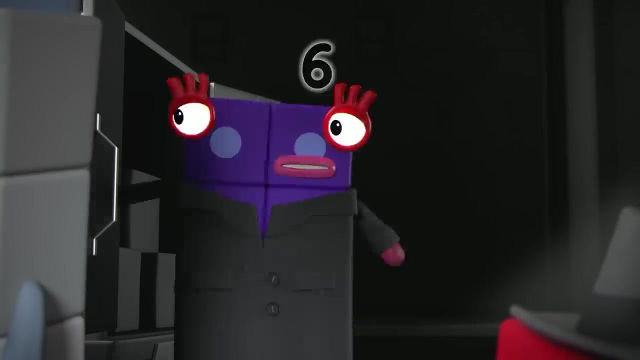 So it must have been Six. And who did we meet in the alley? Three And another three Equals six. Stop, thief. Ha, You've got it all wrong. Oh, where to begin? I'm not taking these things. 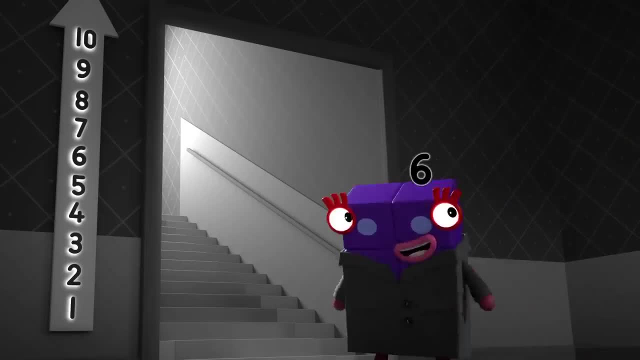 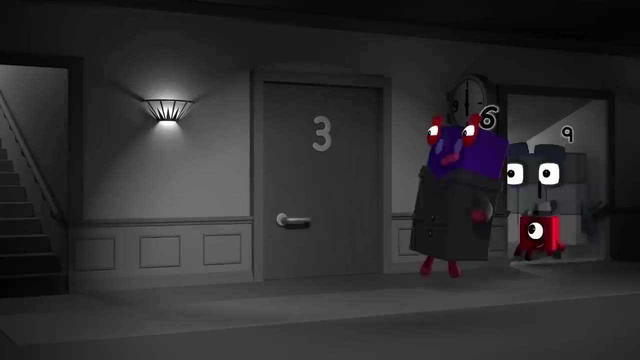 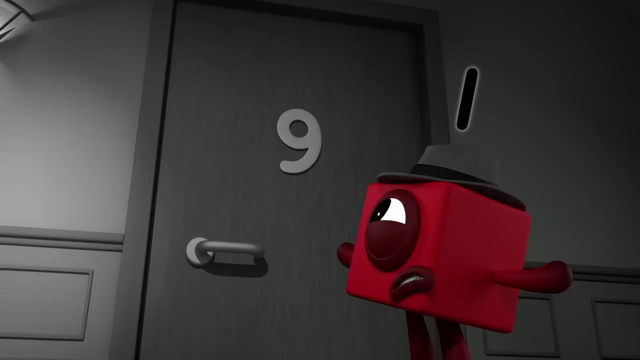 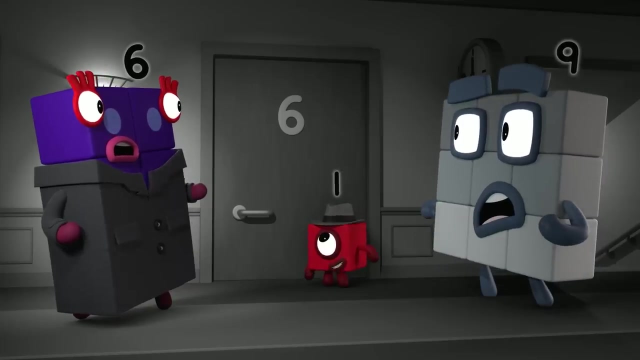 I'm moving them in, Moving in. Come up and I'll show you One, two, three, four, five, nine. Wait, Nine doesn't come after five. This isn't apartment nine, It's apartment six. Oh, 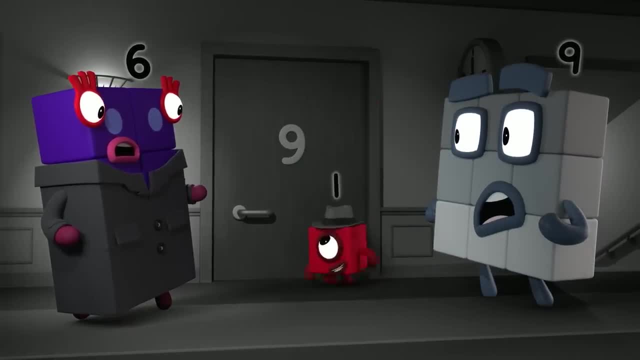 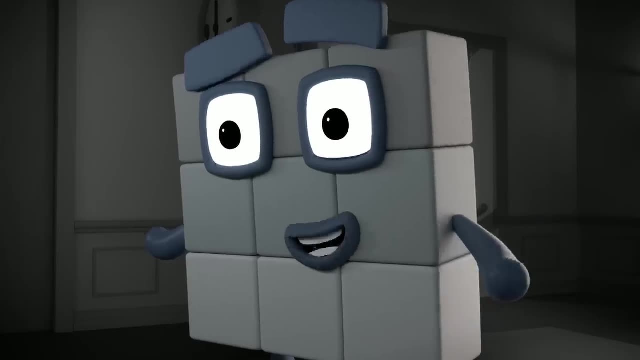 Look, The room that's turned upside down looks like a number nine. Oh, No, one stole your things. Nine: You went into Six's empty apartment, So my things must be Ha, ha, ha, ha, ha ha. 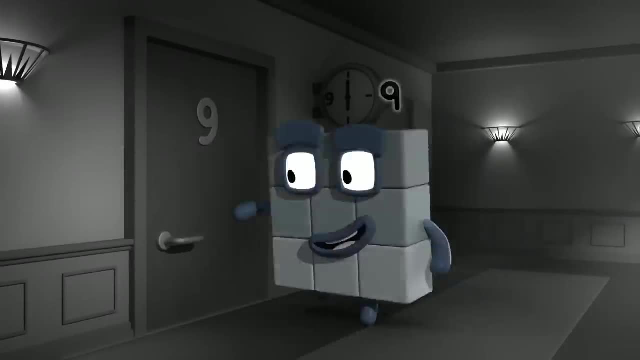 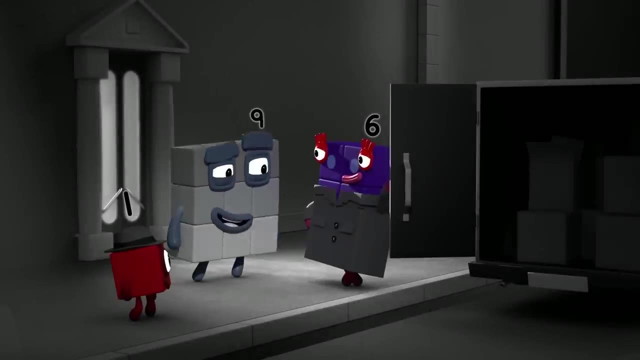 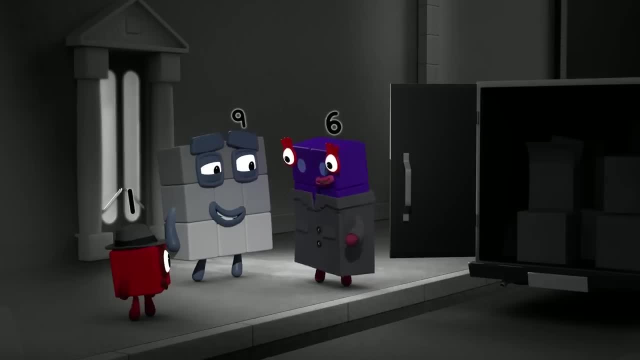 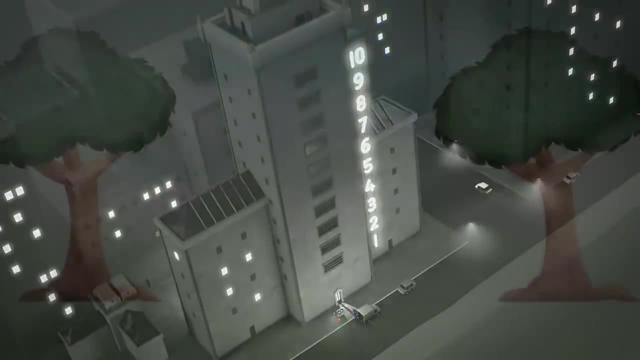 I thought that you were after me. That's why I hid the three-plus-three. Let's make it up to you by helping you move in. Welcome to the big city. No one's there and it's no fun. You can get the party started. 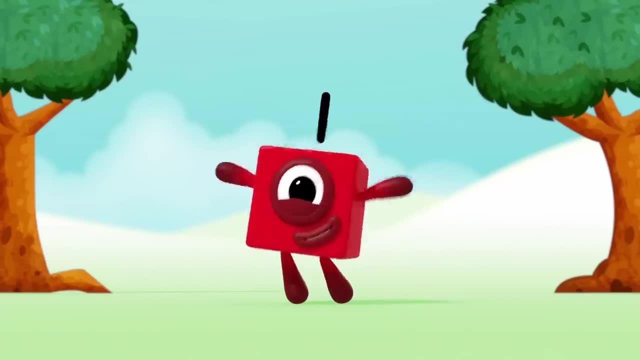 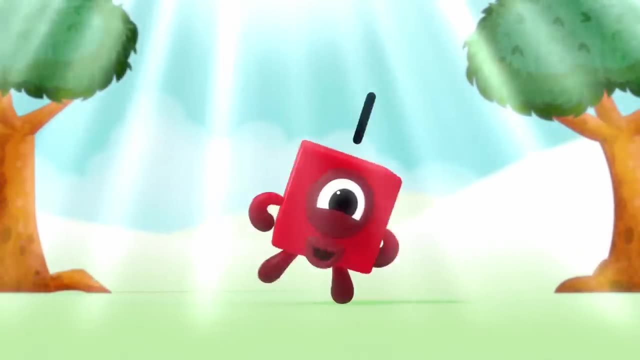 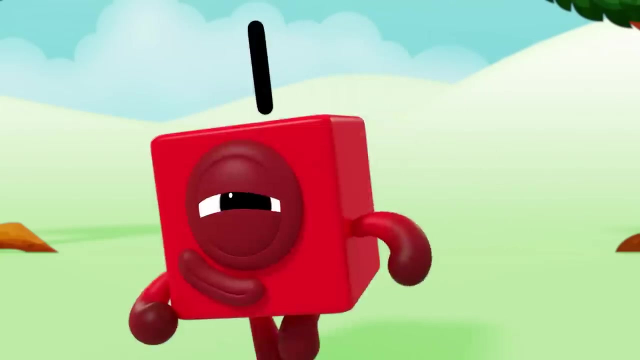 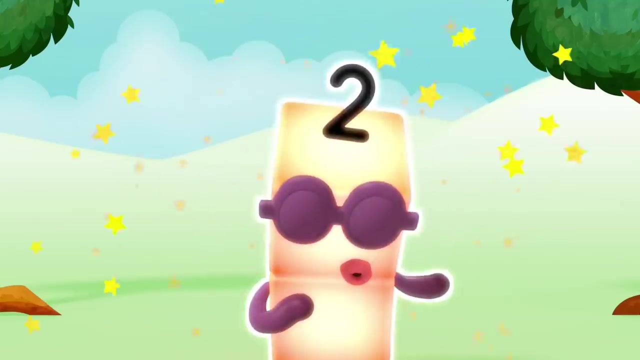 with a bang by adding one. I am one and I'm playing in the sun. Being one is my idea of fun. One, one little block. Now let's add another one. One Plus one equals two. I am two and I'm playing in the sun. 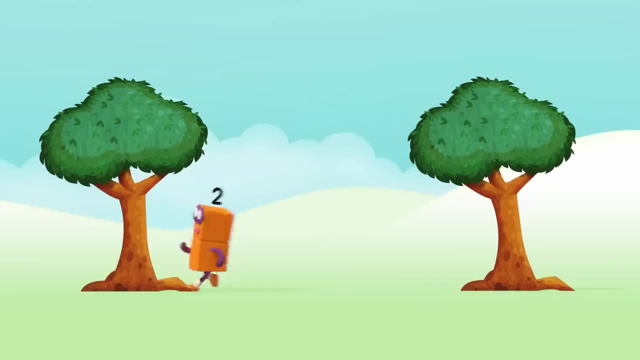 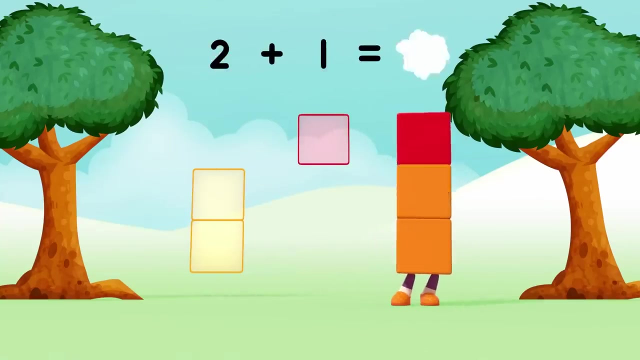 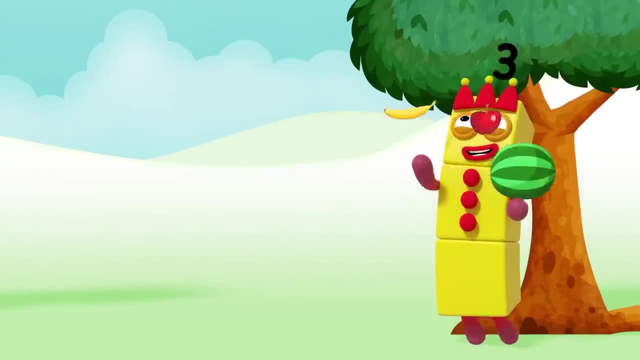 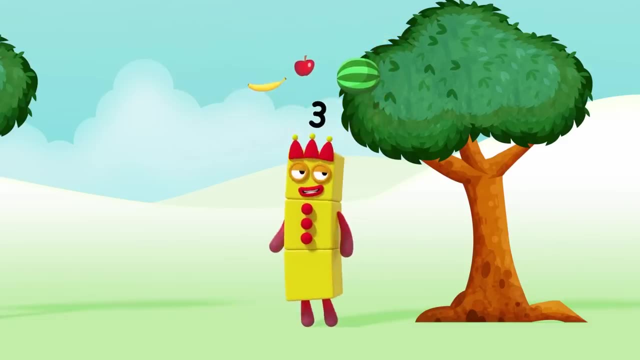 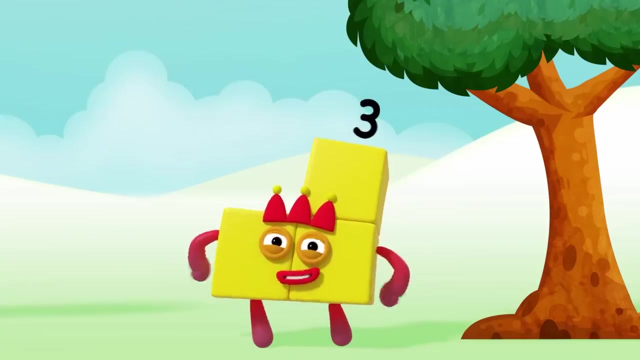 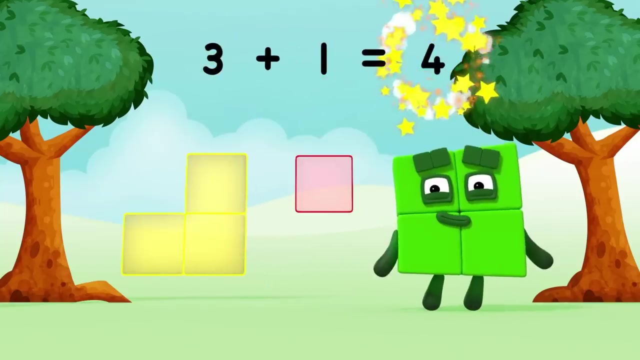 And I'm playing in the sun. Juggling things is my idea of fun. One, two, three, Three things. Look at me: One, two, three. Now let's add another one. Three plus one equals four. I am four and I'm playing in the sun. 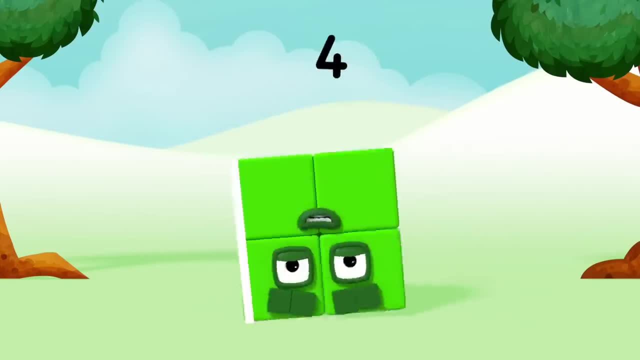 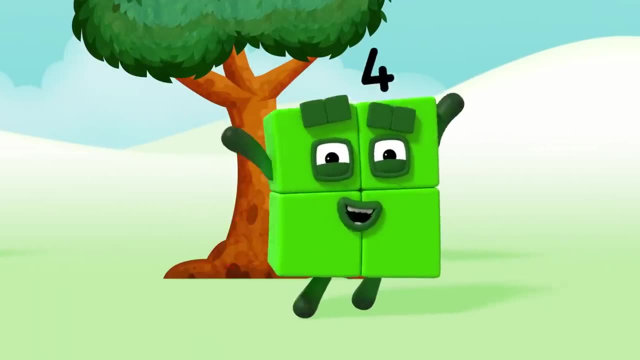 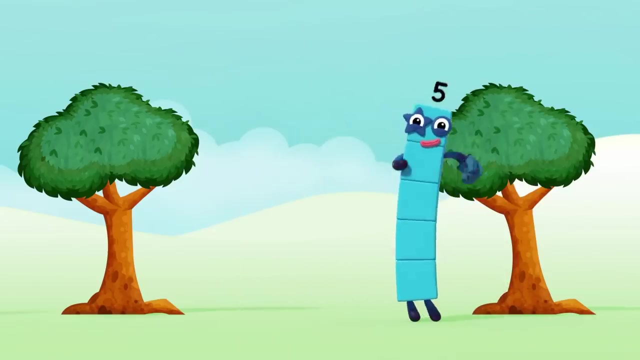 Being square is my idea of fun. One, two, three, four, Four sides Out out, out out Four corners. Now let's add another one. Four plus one equals five. I am five and I'm playing in the sun. 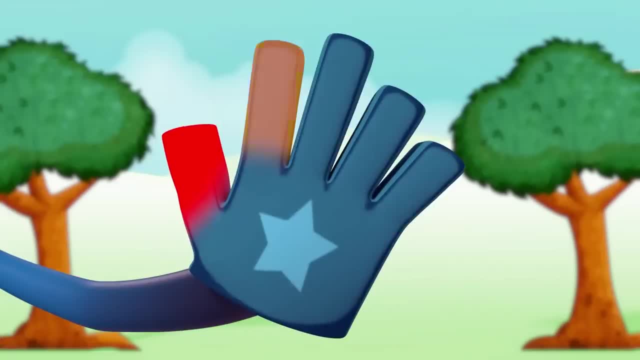 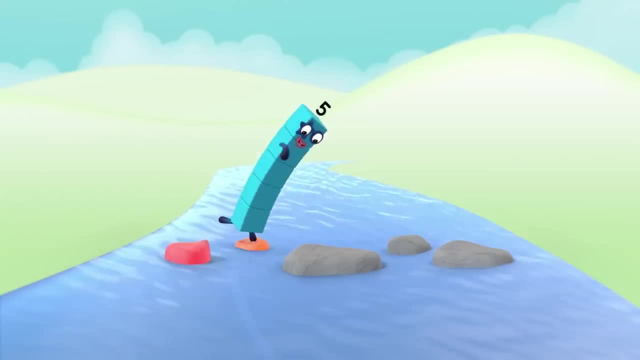 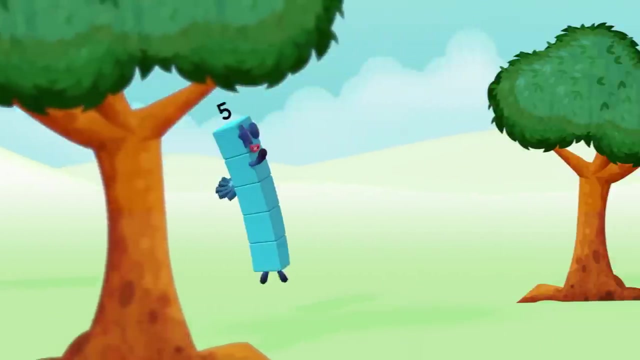 High five are my idea of fun: One, two, three, four, five, Five fingers: One, two, three, four, five. If you add another one the number gets one bigger, And if you keep on adding one you can get to any bigger. 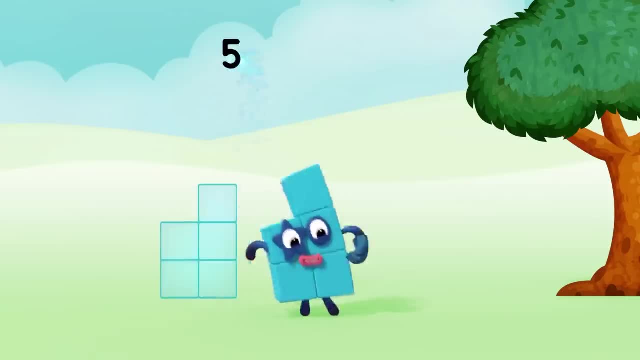 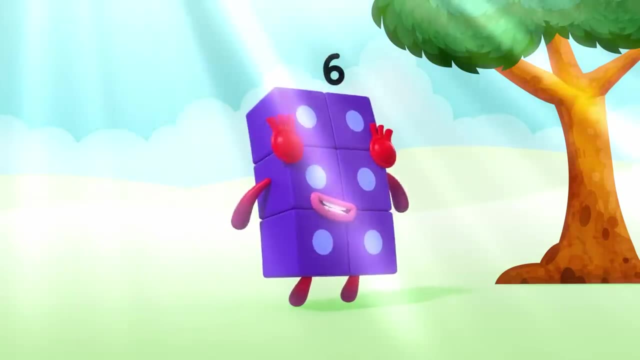 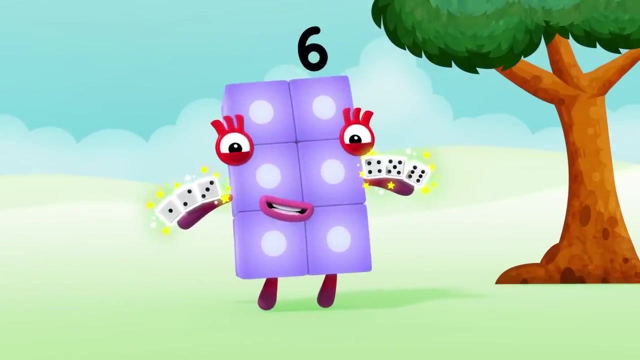 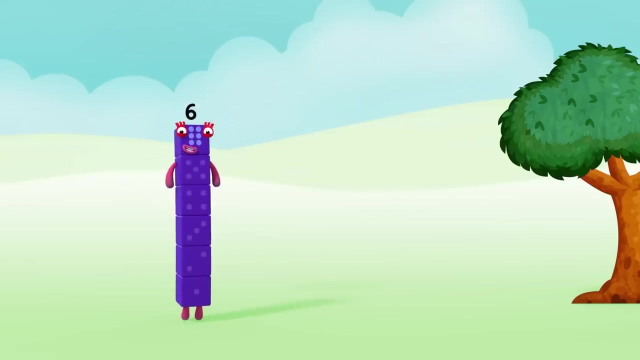 Now let's add another one. Five plus one equals six. I am six and I'm playing in the sun. Playing games is my idea of fun. One, two, three, four, five, six, Six dice. Now let's add another one. 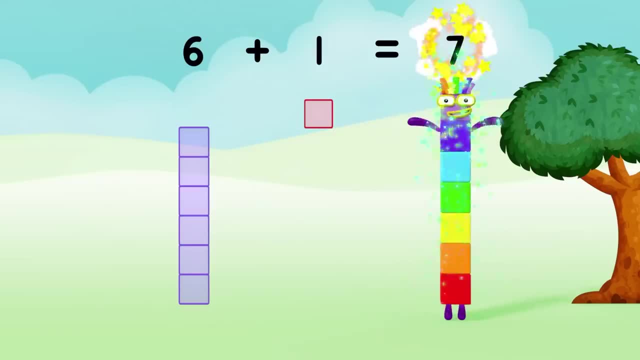 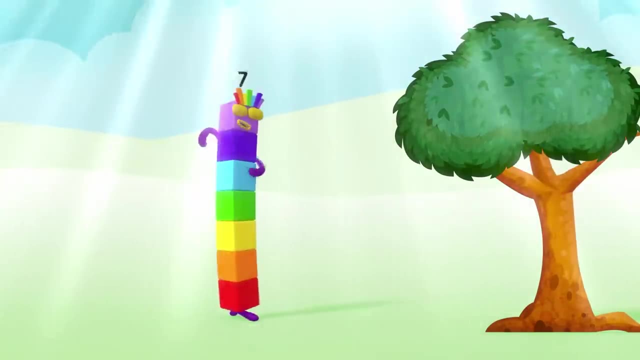 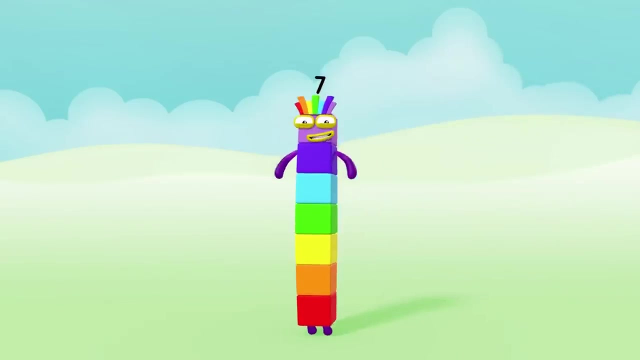 Six plus one equals seven. I am seven and I'm playing in the sun. Making rainbows is my idea of fun. One, two, three, four, five, six, seven, Seven colors. Now let's add another one. 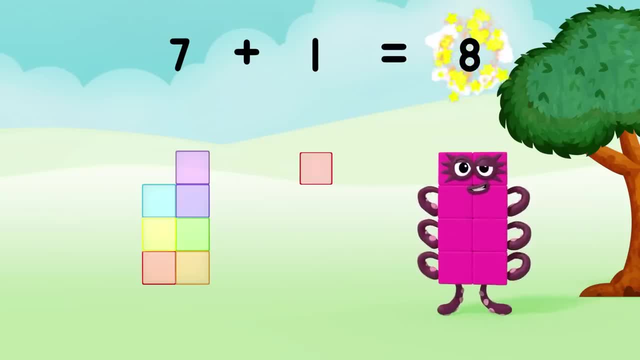 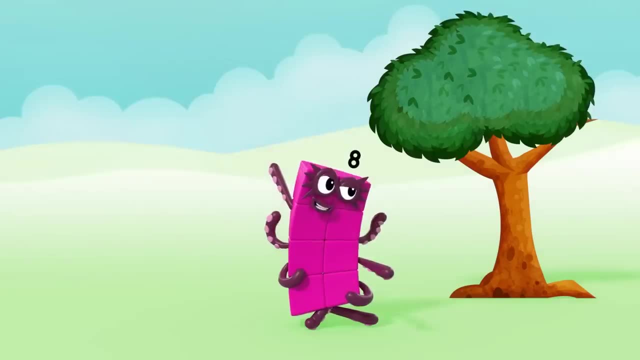 Seven plus one equals five. Seven plus one equals eight. I am eight and I'm playing in the sun. being Octoblock Is my idea of fun. Octoblock run: One, two, three, four, five, six, seven, eight run. 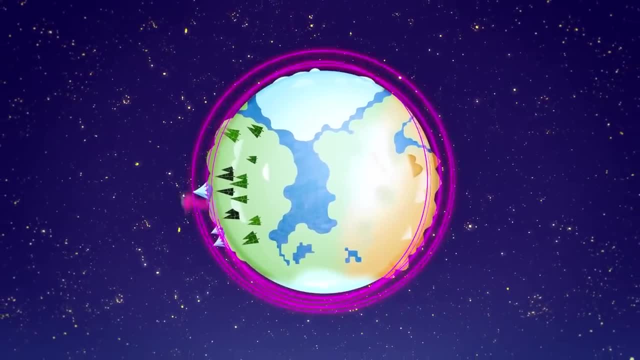 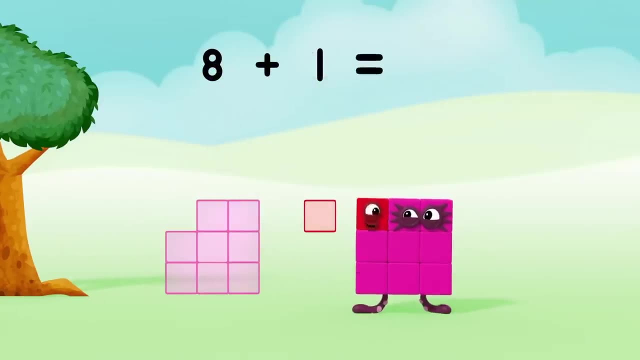 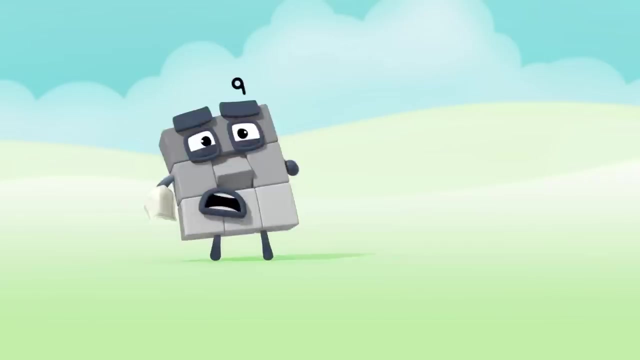 Ha-ha. Now let's add another one. Eight plus one equals nine. I am nine. Uh-huh, Uh-huh, I am nine and I'm playing in the sun. not sneezing Is my idea of fun. 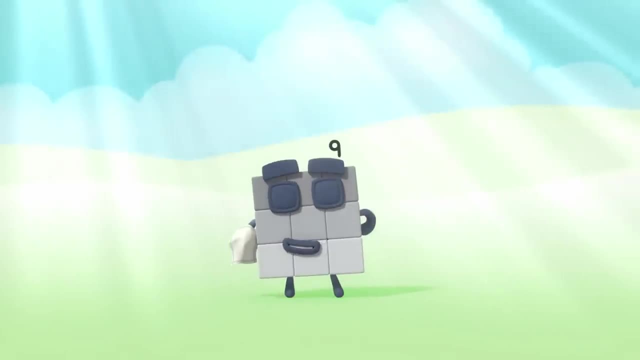 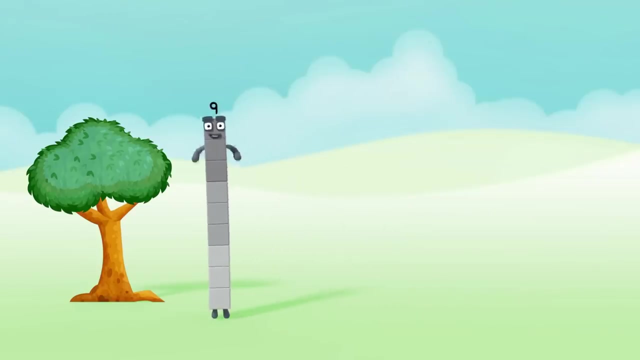 One, two, three, four, five, six, seven, eight, nine, Nine hankies. Now let's add another one. Nine plus one equals ten. I am ten and I'm playing in the sun being ten. 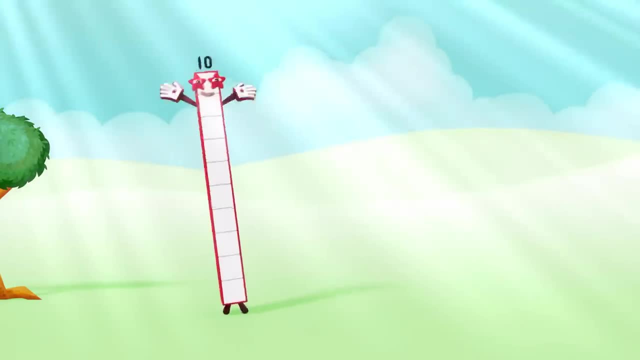 Is my idea of fun: One, two, three, four, five, six, seven, eight, nine. I am ten and I'm playing in the sun being ten. One, two, three, four, five, six, seven, eight, nine, ten. 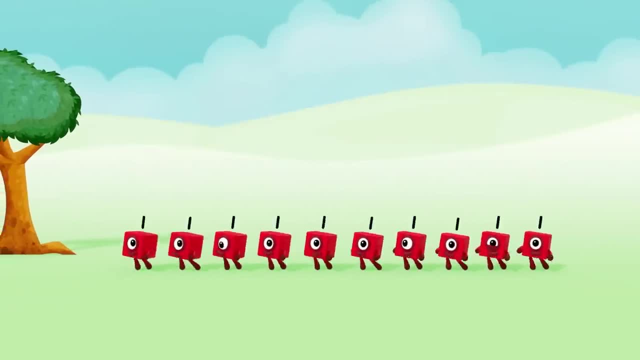 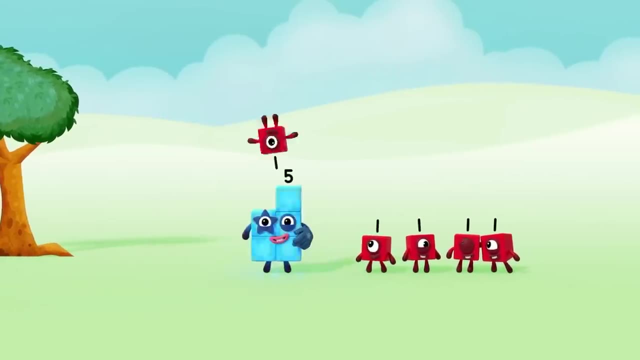 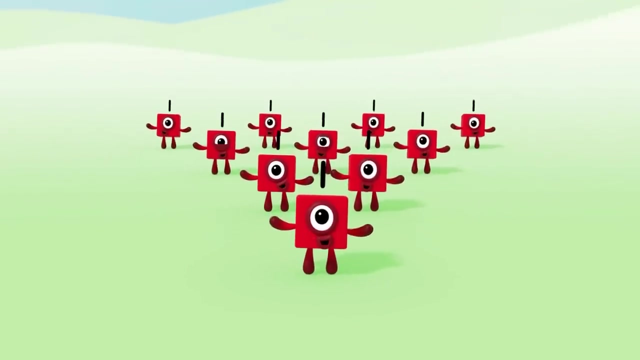 Ten blocks. We're ten ones and we're playing in the sun. Making friends is our idea of fun. One, two, three, four, five, six, seven, eight, nine, ten. Remember this forever. You can do what we've just done. 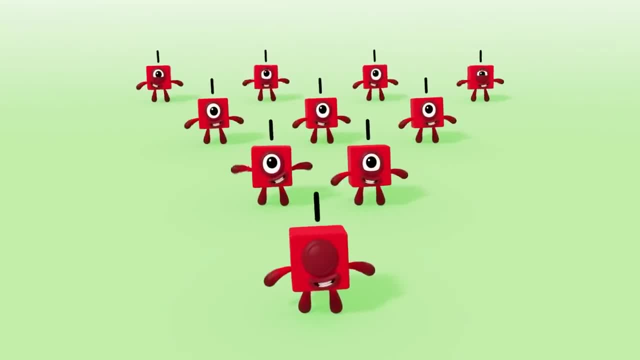 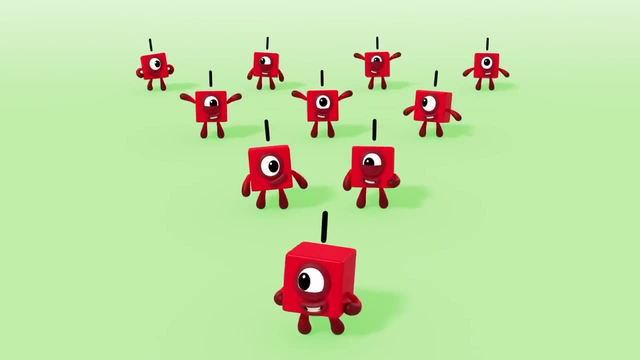 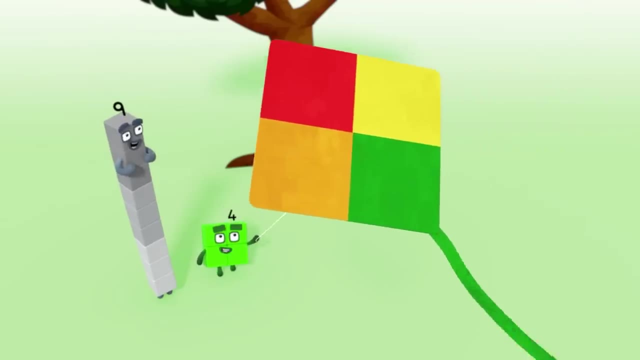 You can make any number and you'll keep on adding one. This way you have 10 blocks to make. You're a ten, So a point goes to you. Eight blocks per question, Two blocks for me, I. That was fun. 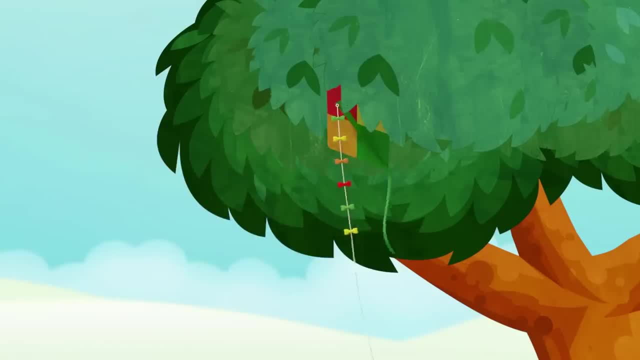 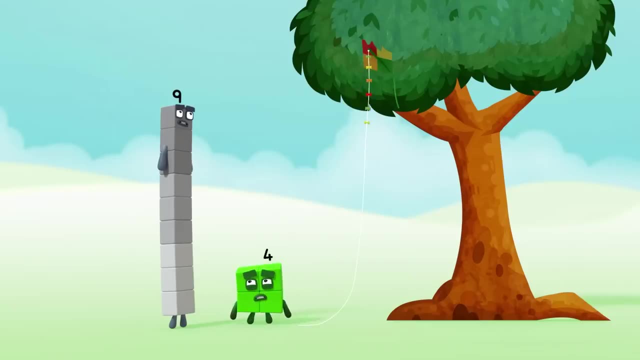 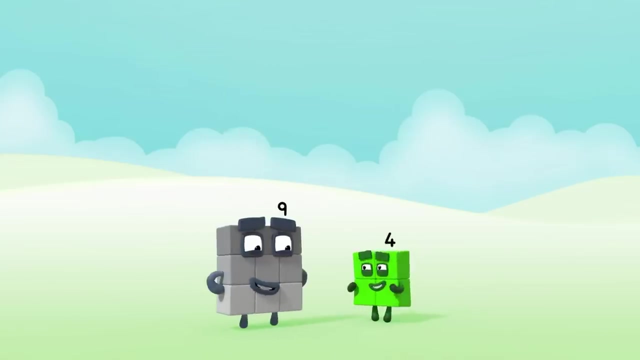 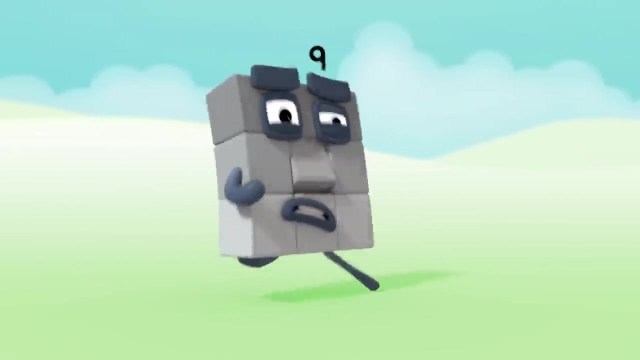 Yay, Look at it, go. Oh, mind that tree, Can you get it down? You're a big square, You can do anything, Right? Well, maybe if I take a run up, That's it Go nine Achoo. 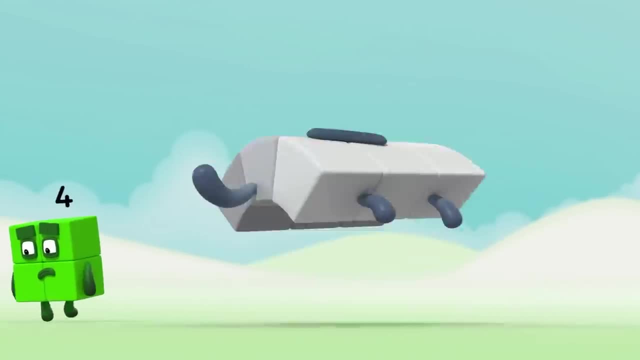 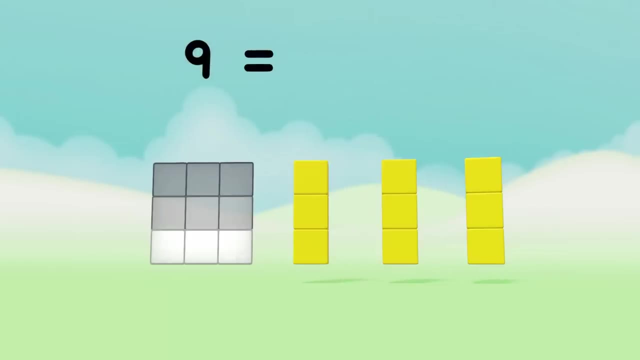 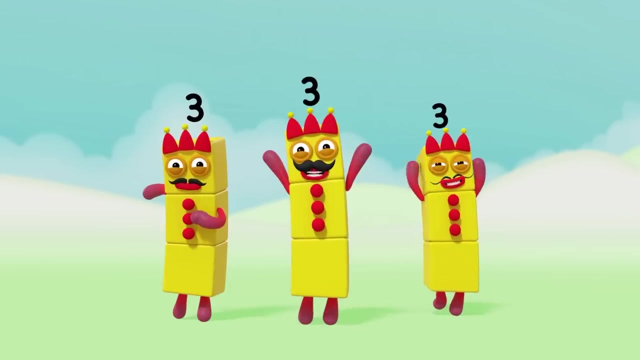 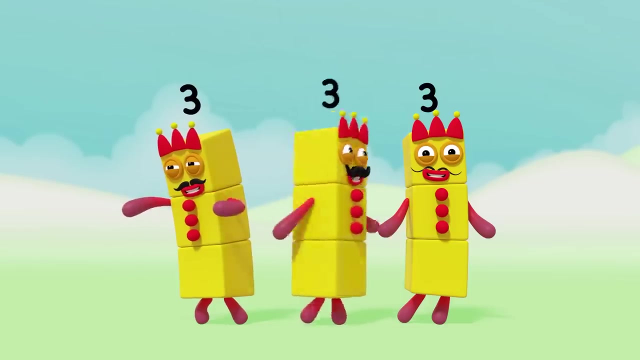 Maybe we should get ten. Nine equals three Plus three plus three. Roll up, roll up, roll up. We three are the Three Threes The most amazing, the most incredible, the most extraordinary acrobats in Numberland. 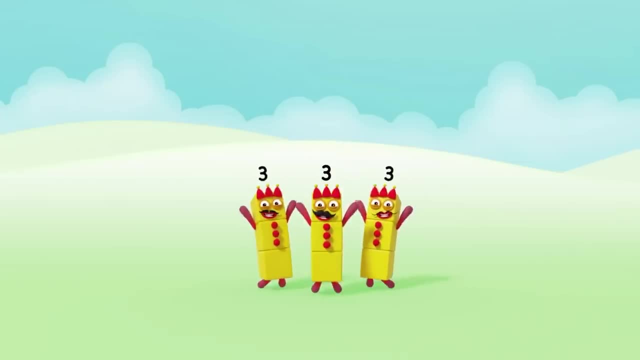 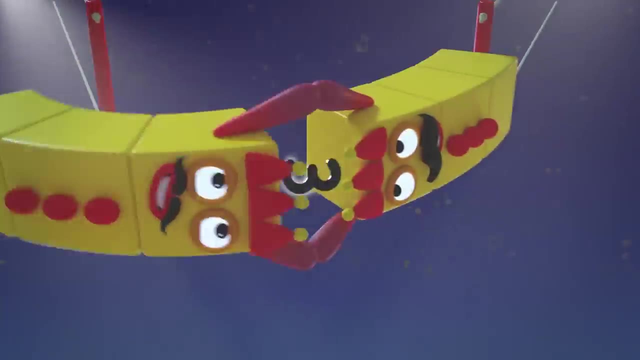 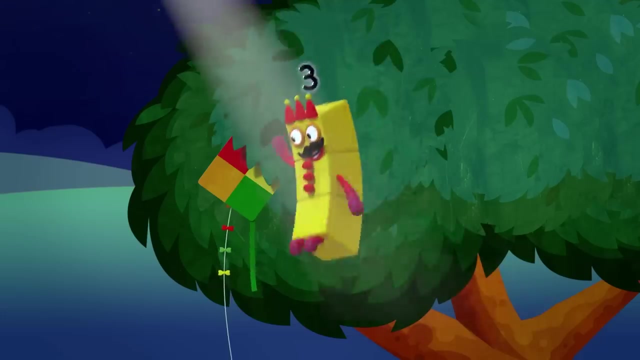 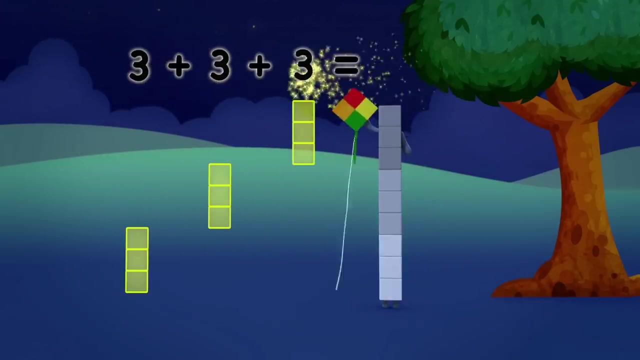 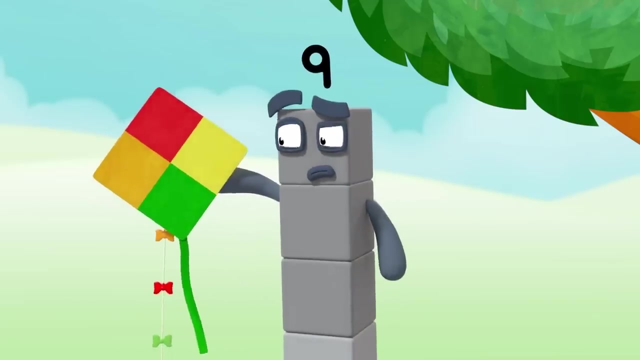 Drumroll please, as we present The Three Threes On the flying trapeze. Three plus three plus three equals Nine. Nine, You did it. Did what? Oh yes, It was nothing really. 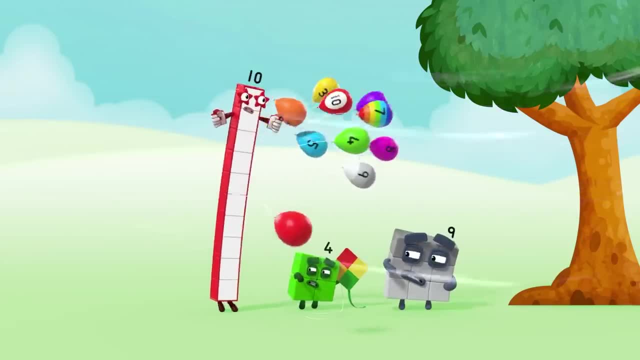 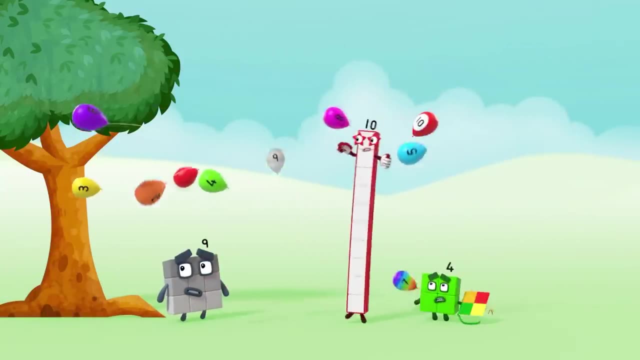 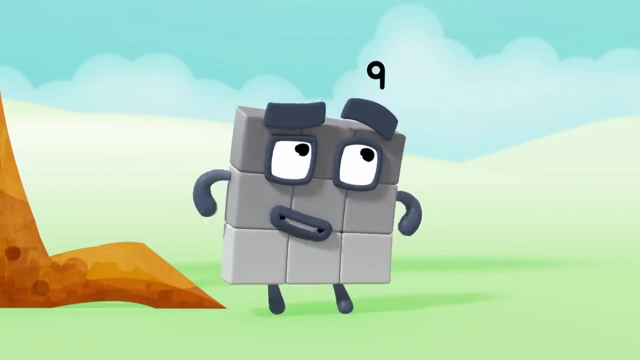 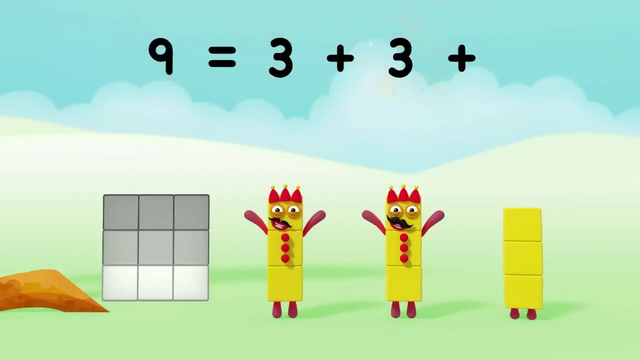 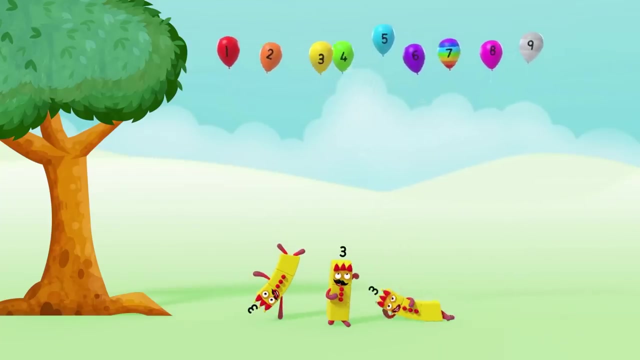 Really Quick, Quick, Stop them. There are too many. We need help. Help, I can do this myself. Nine equals three plus three plus three. The Three Threes will seize these with great ease. Drumroll, Drumroll please. 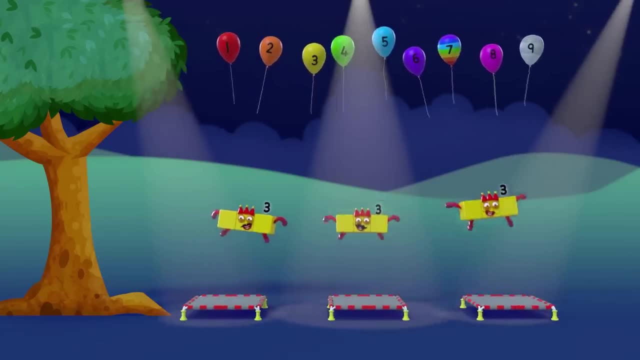 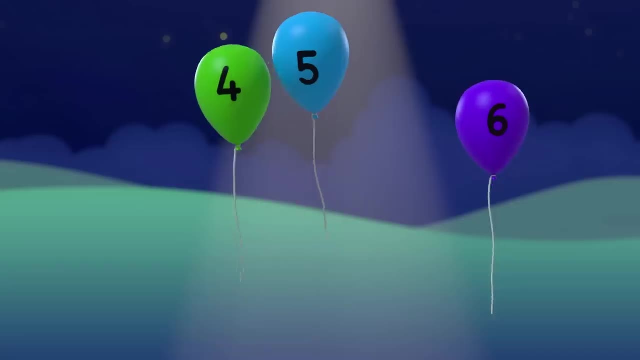 Three, two one. One. two, three, Four, five, six, Seven, eight, Nine. Three plus three plus three equals Nine. You did it again. I did it. I did it. Three, two, one.